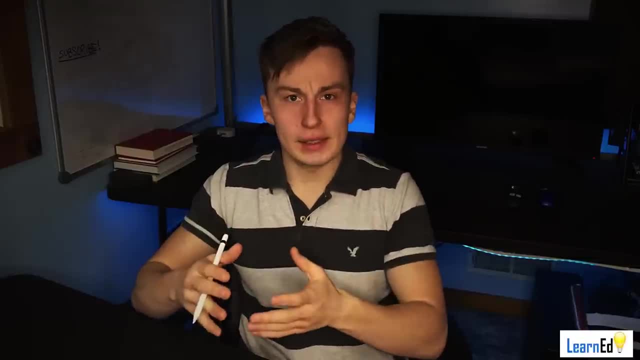 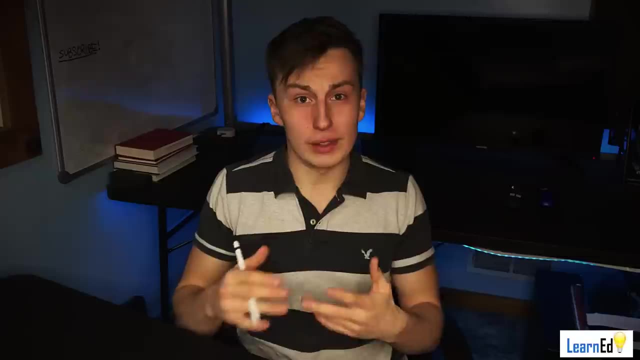 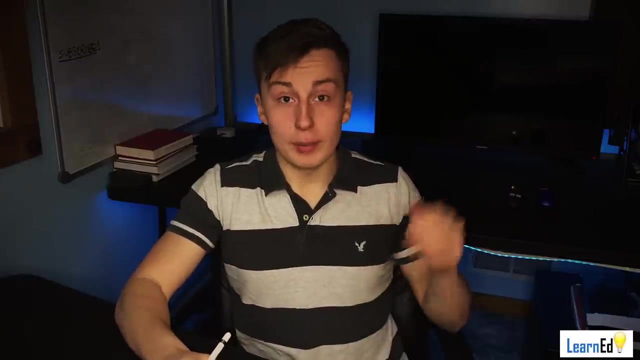 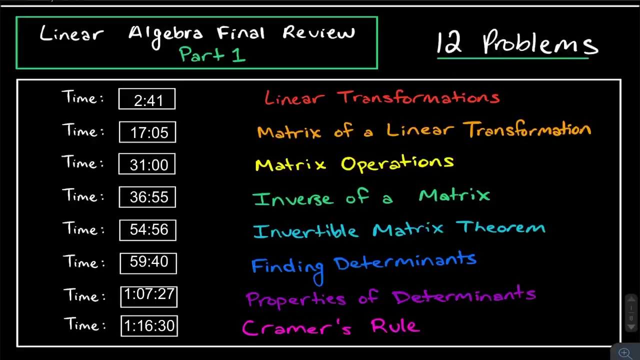 talking more about vector spaces, bases and, of course, doing change of bases as well- dimension rank, And in the third video, we'll talk about eigenvalues and vectors and all the stuff that comes with that. Okay, so now let's get a more in depth look on what we're going to be doing in this video And, as you can see, we're going to be doing 12 problems, Okay, And these 12 problems are going to consist of the following topics, The first one being linear transformations, and then 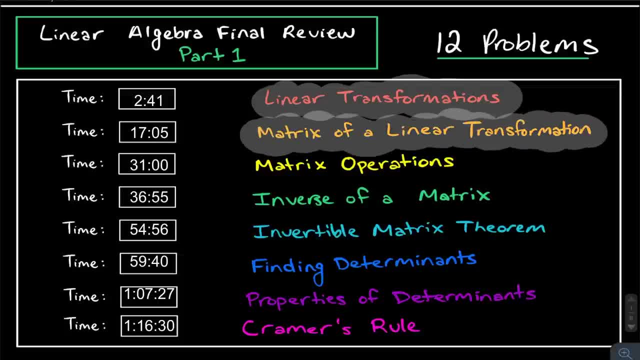 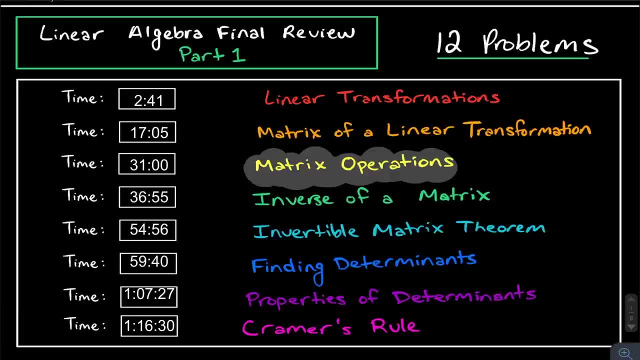 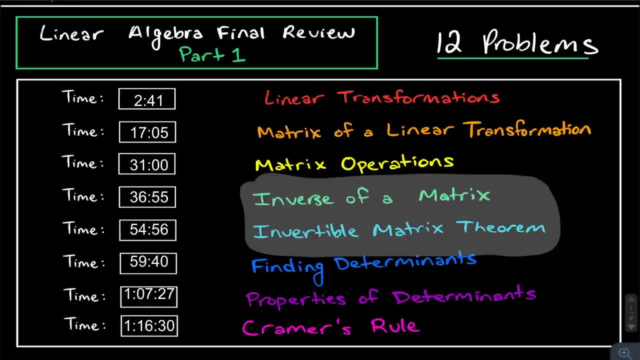 we'll talk about the actual- like the standard- matrix of a linear transformation. We'll dive in a little deeper there. We'll talk about matrix operations. So basically that's just going to be a problem on matrix multiplication And then we're going to dive a lot deeper into the inverse of a matrix. We'll do a few problems there, Just finding the inverse of a matrix and using the invertible matrix theorem to see if a matrix is invertible or not. We will then talk about finding determinants. 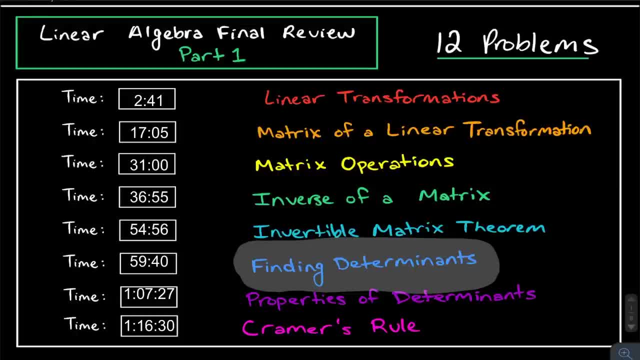 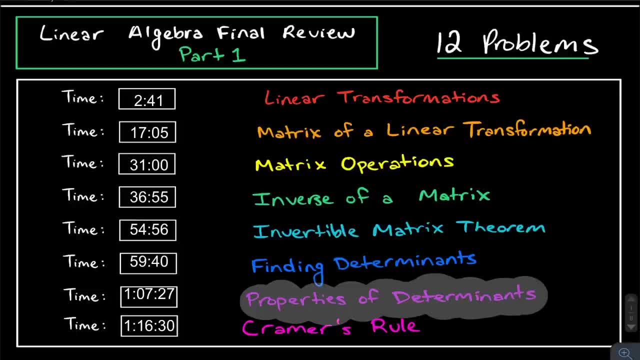 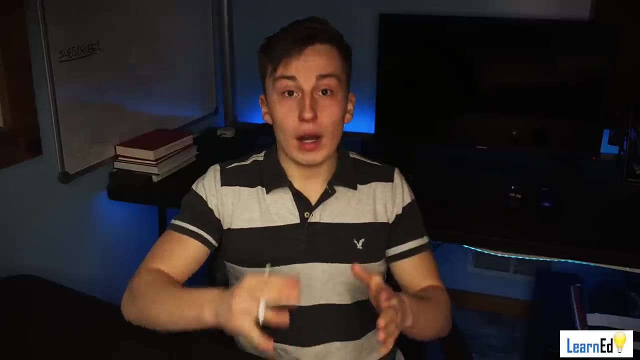 Okay, so we'll use a couple methods, such as cofactor expansion, And we'll also talk about properties of determinants. We'll talk about you doing a row reduction to find determinants, And we will talk about other things such as being upper triangular And, lastly, we will touch on Kramer's rule. Okay, Now, a big thing to note in this video before we get started is that we're going to be doing, of course, a lot of 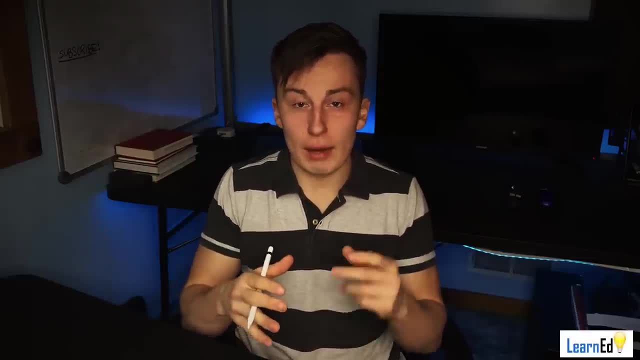 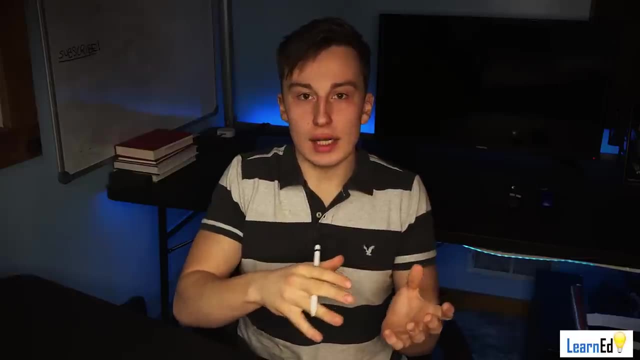 a lot of row reduction. that's kind of at the heart of linear algebra. okay, and while i will try to go a little bit slower with the row reduction to start off with, i, you know, i want to note that it's going to be, you know, at a, at a good pace, right, i'm not going to be slowing down and 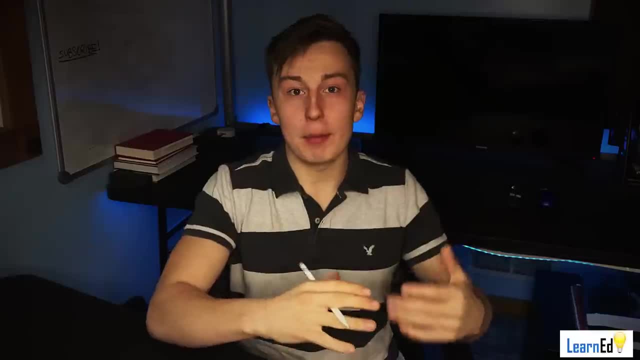 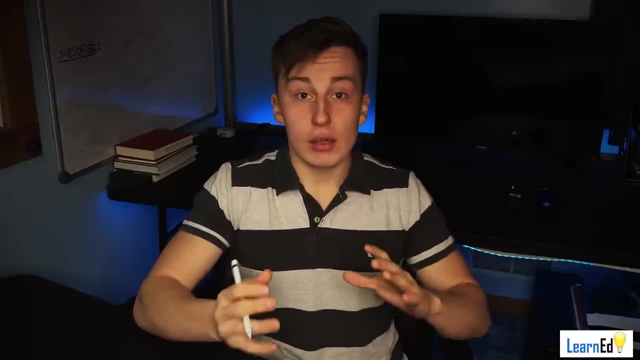 explaining each step you know in in a lot of depth, because i'm assuming that we're all kind of on the same page. as far as row reduction goes, okay, if that's something that you feel you need to work on, you know i can uh link in the description. hopefully, uh, i'll have a row. 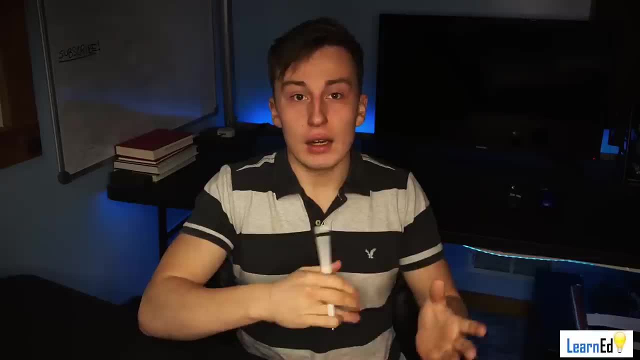 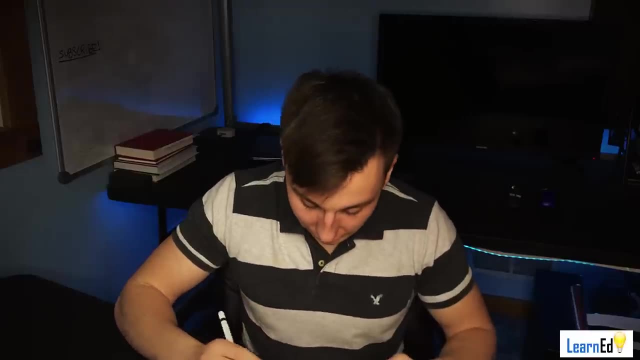 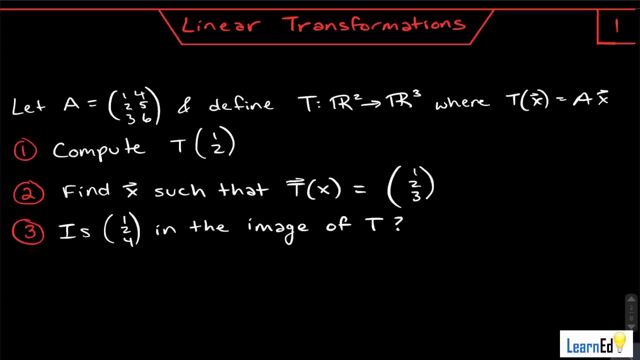 reduction video up by the time that you watch this, but if not, then, uh, i'll be in the process of making one, okay, so, anyways, let's get in to this video and start with our first problem, which is on linear transformations. and our first problem is saying: let a, we have a, we have a. 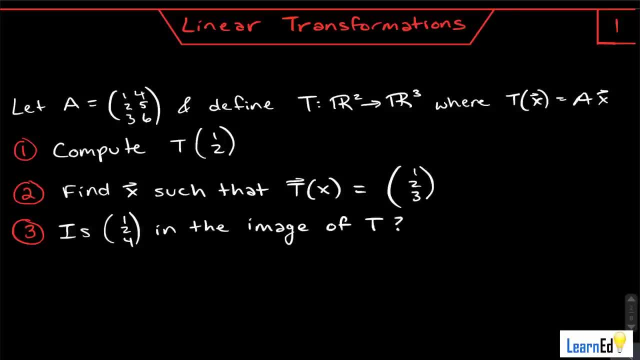 standard matrix a, and i'll talk about why it's it's called a standard matrix in a second. but we have a and we are defining a transformation from r2 to r3 where t of x is equal to a times x, and that's some notation that i also will mention in a second. 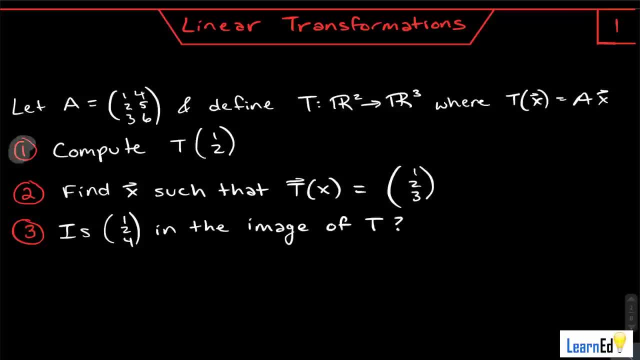 because that is very confusing. now we're asked to three things. we're asked to compute t of one, two. we're asked to compute uh, we're asked to find an x such that t of x is equal to one, two, three. and lastly, we are asked to find if one, two, four is in the image of t, and we'll have to also talk. 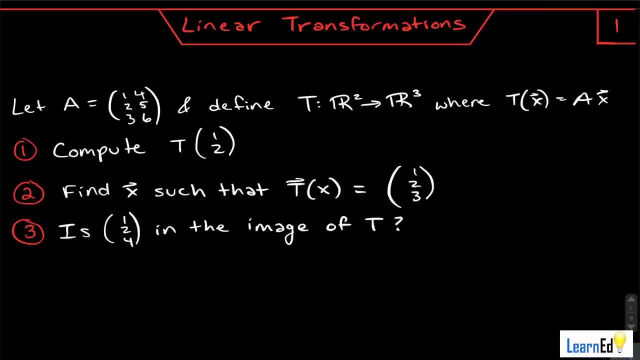 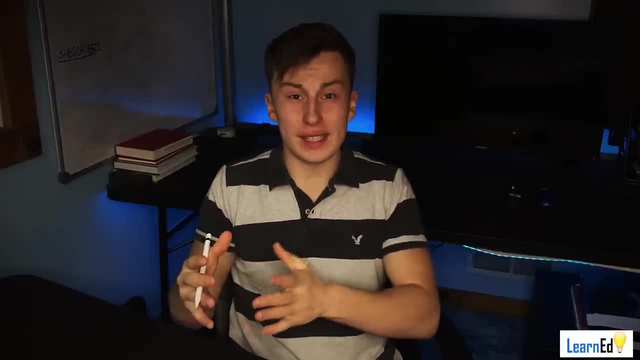 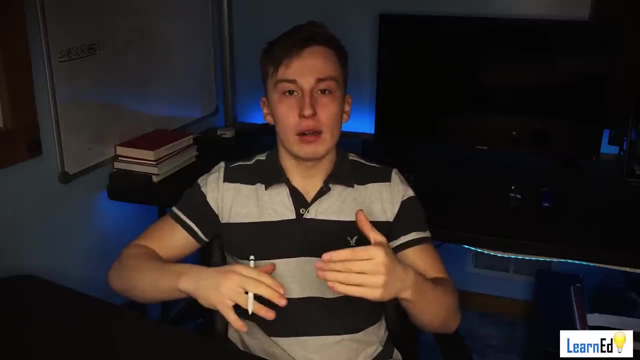 about the whole image idea of what that means. okay, so first talk about the notation of a transformation, and that's why i wanted to go over this again, because, of course, this is something that pops up again and again as you go through your linear algebra course. however it's, it's a 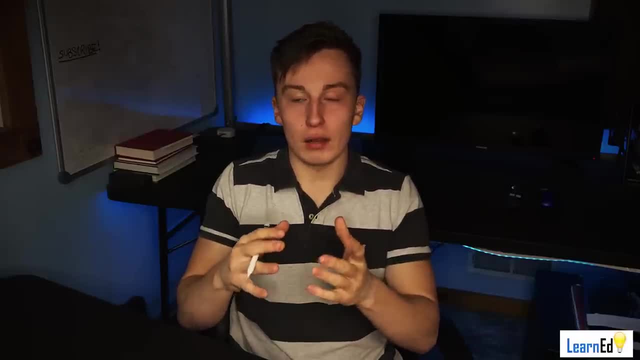 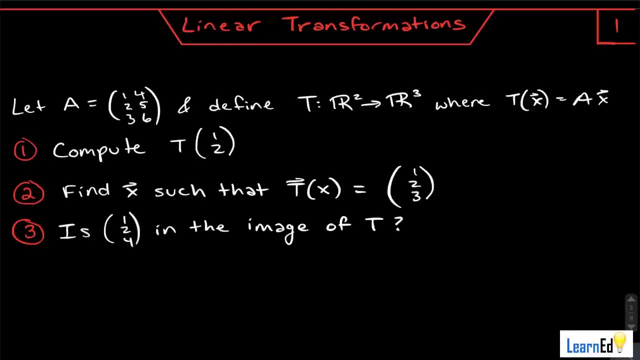 tough topic to start out with, and i think that's the. the first thing that i wanted to talk about is the first point that a lot of students struggle with: to begin linear algebra. okay, it was definitely the first thing in linear algebra that i ended up struggling on myself, okay. so here's the 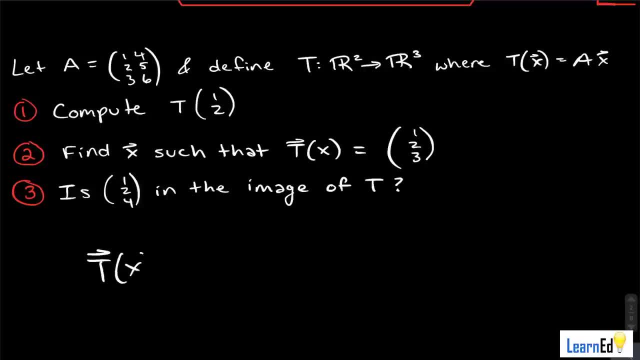 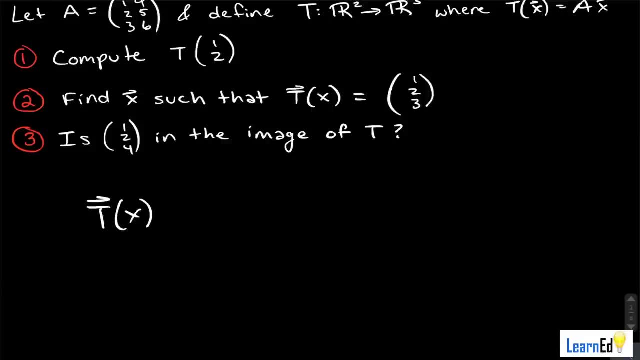 idea, this, this notation here, this t of x, kind of think of it as, and, by the way, t of t of x equals a x, right, and we know that a x equals b. okay, you to think of this as is. y equals a function of x. okay, and basically the f lines up with the t. 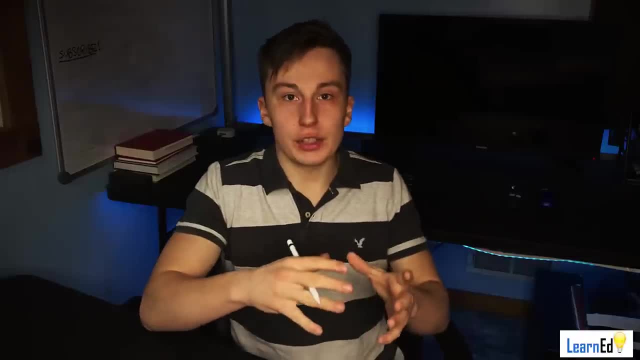 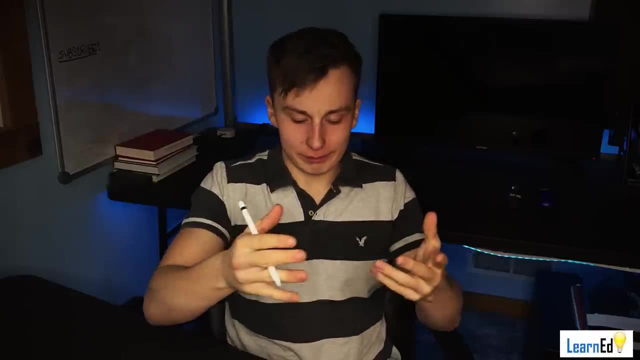 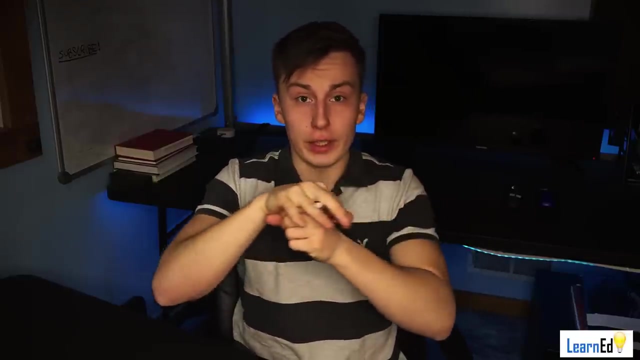 okay. so it's kind of like the t tells you what kind of what kind of dimensions you are are transforming your vector into right. so we're taking in this example, we're taking a vector from two space and converting it to a vector in three space. okay, 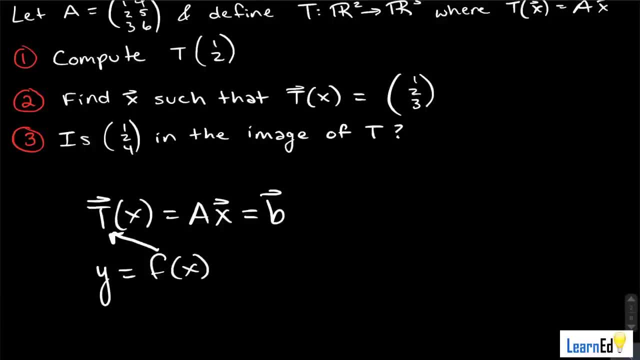 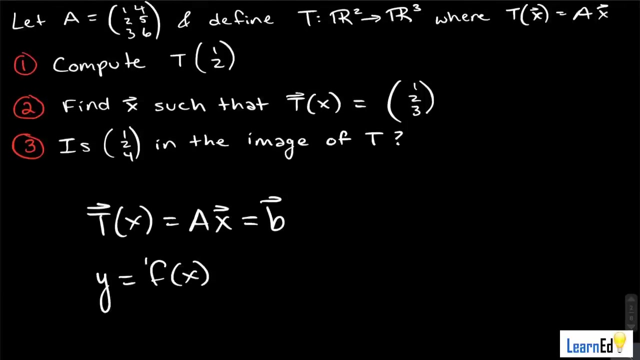 and that's kind of the purpose of t. now, your b, right, this b is just y, right, and the actual contents of t of x, right, that is a of x. okay, so where you know where t of x is kind of just this notation of f of x. so f of x actually equals, you know, like, let's say, x squared plus x plus one or something. 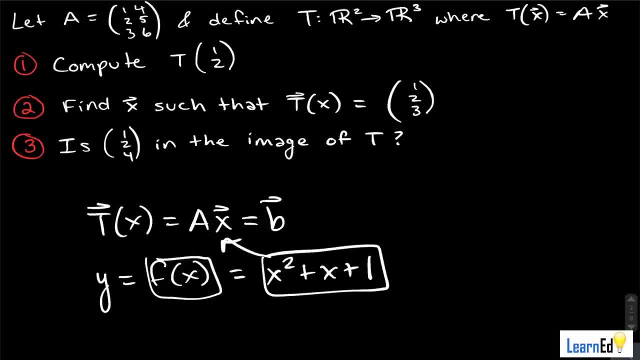 like that. this is kind of like a x. it actually tells you what the function is. so you know, i kind of apologize because this is in a. uh, i said kind of apologize, that's funny. anyways, let me actually move these things around, because these are in the wrong order and i can probably 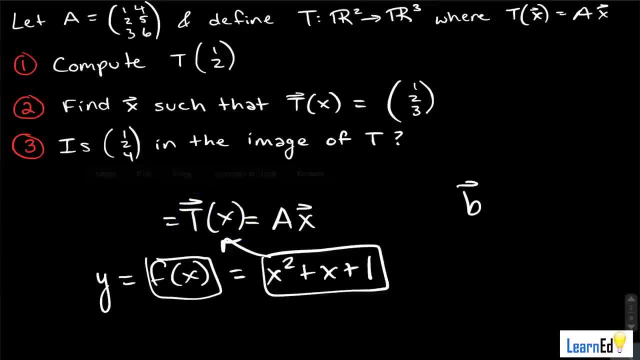 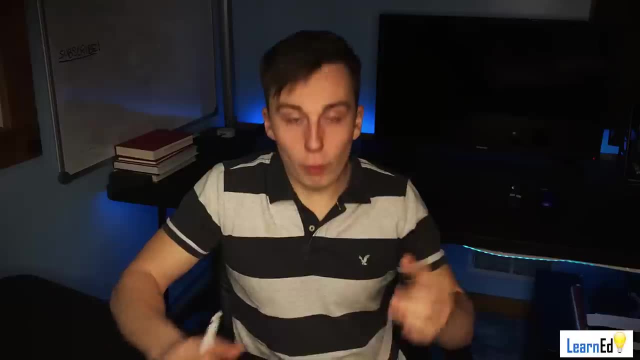 show this a little bit better if i just show it like this: okay, so this is actually what's going on. it's more like this, and then these things correlate exactly with what you see above all right, so there's kind of a better way to put it now. hopefully that makes. 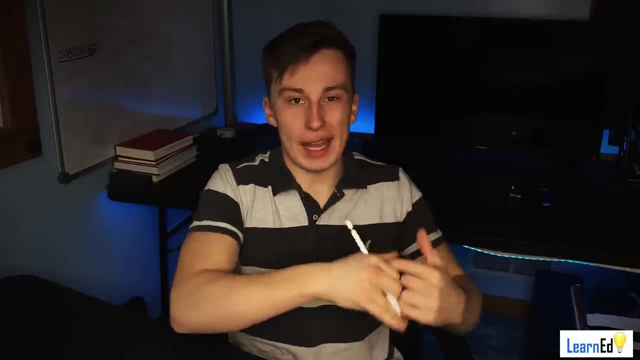 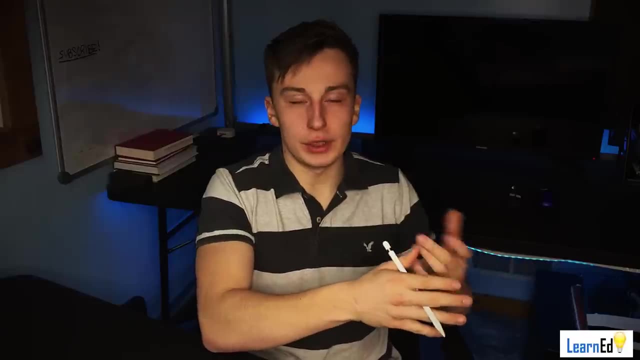 more sense now. okay, so the t of x is kind of just like f of x. your your vector b right, your your d. you can kind of think of it as your dependent variable, which in this case is a vector, all right, and that's the result of your function of. 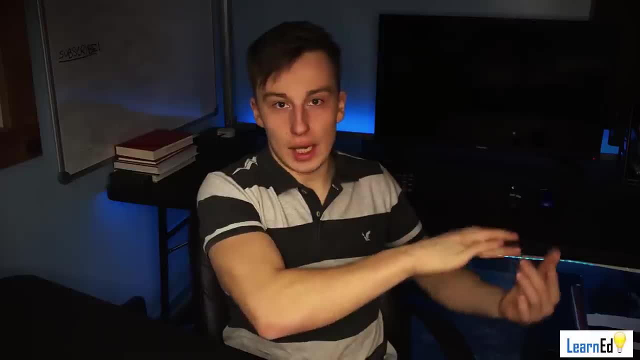 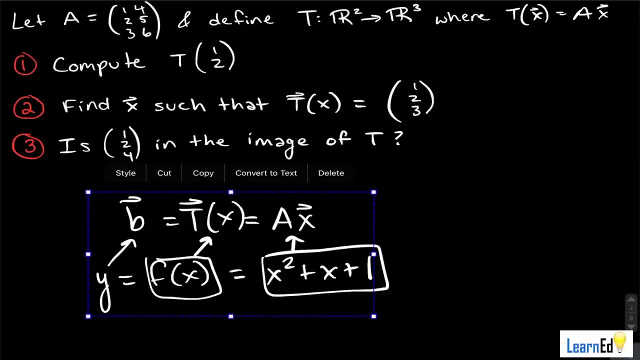 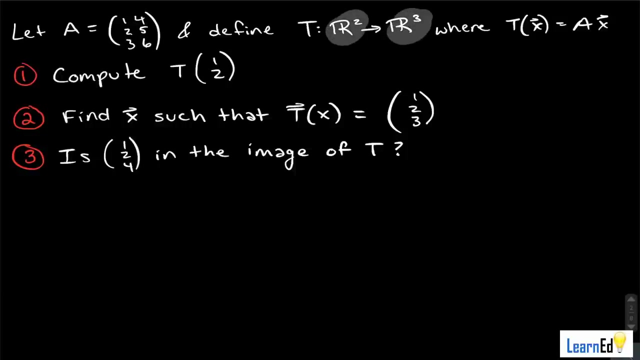 of x. you input some vector x and you output a, b, okay. so that's the idea of the matrix equation. now we're performing a transformation. we're taking a vector x, okay, and we're transforming it to, from a variable into space, to a vector in three space, okay, and you know i mentioned 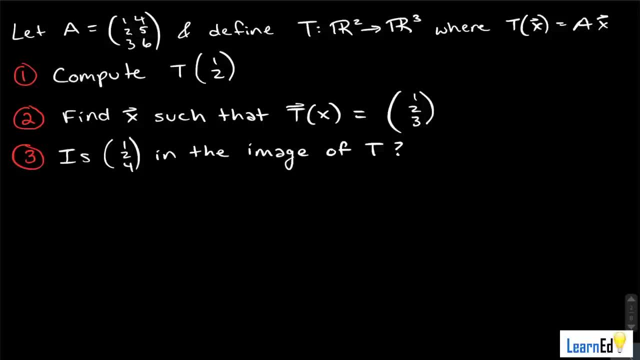 that previously now, as i also said, this a right here. this is called a, a standard matrix. okay, and that is what operates on the, the x vector right in in our first problem. it is one, two. so now, with that knowledge, we should be able to go ahead and start our first problem. all right, and 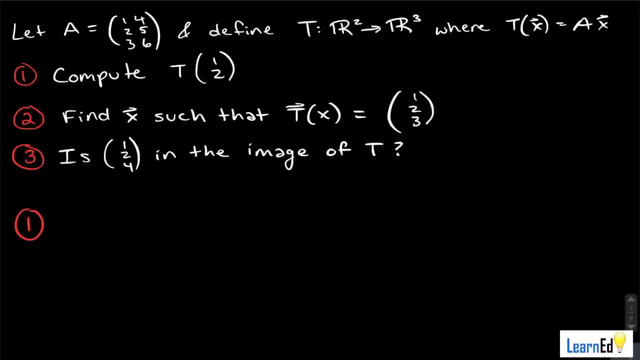 that's to compute the, the t of one, two. so let's write down our equation. we know that a x equals b right and t of one two just means that we're plugging in x, or we're plugging in one two for x. so let's do that. we have one four. 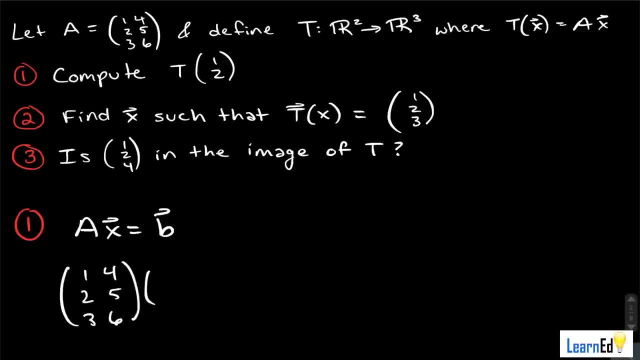 two, five, three, six, and we multiply by that vector one, two, and well, let's see what we get now. the next thing about multiplying by a vector with when you do some matrix multiplication, is that you'll just end up getting something like this right, which is a lot nicer than having to do it all out, uh, with, like you know, a two by two. 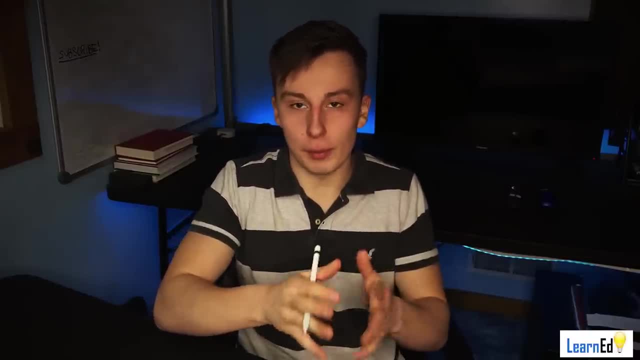 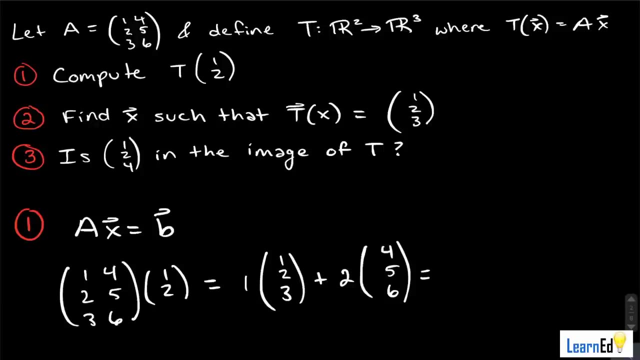 multiplied by a, two, by two, that can get really gross, but of course we will have to be doing an example of that a little bit later. anyways, you can now see that we will end up getting a one, two, three plus a eight, ten, twelve, and that will give us a nine, uh, 12, and then a 15 below, and that is the answer to number one. 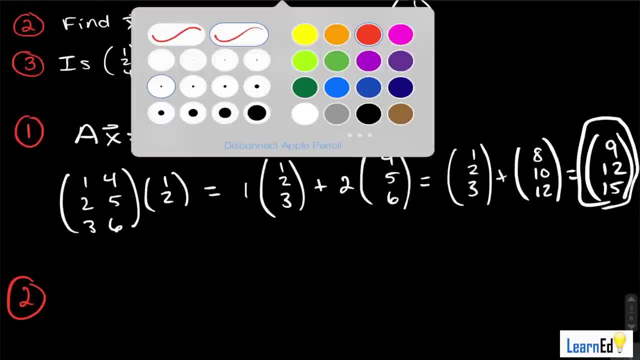 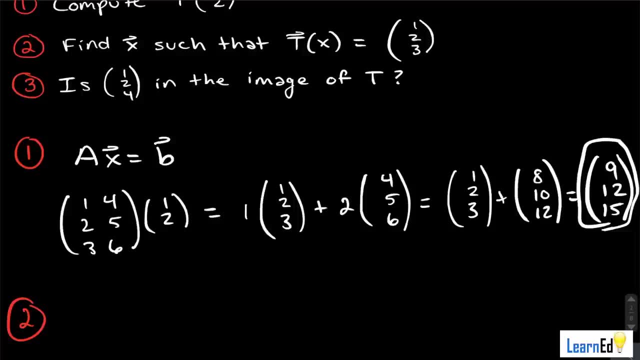 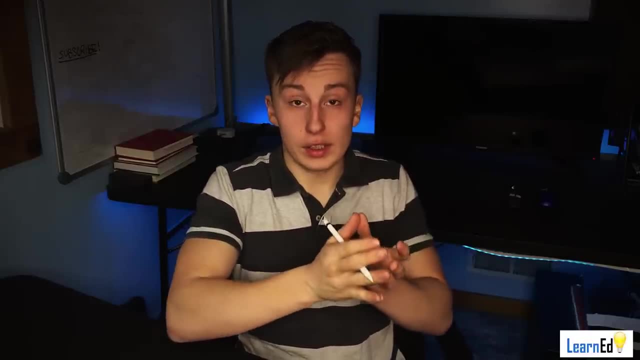 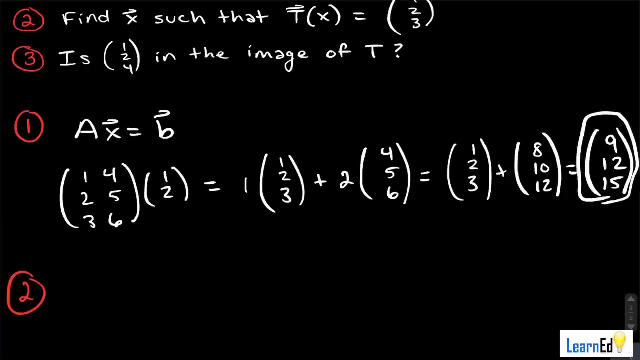 okay, now for the second part of the problem. we want to see. we want to see if- uh, we can- we can find a x where t of x can equal one, two, three. so we want to basically transform some x to get one, two, three. we want to find what x we can transform to do that. okay. so, instead of having one, four, two, five, three, 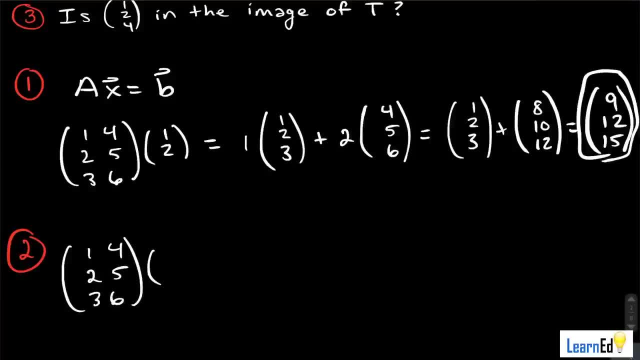 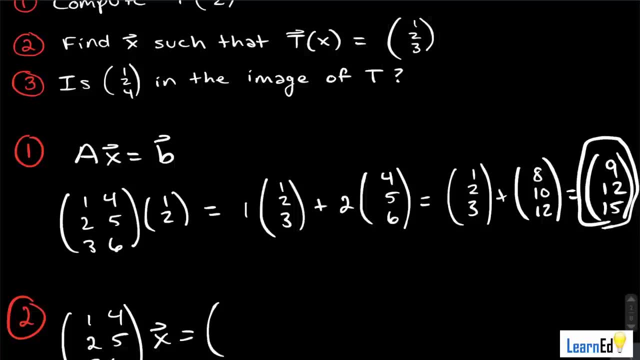 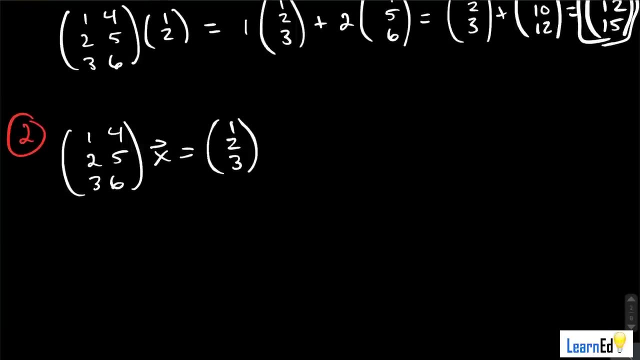 six, uh times some known vector. we don't know this vector, but we do know b, right. b is one, two, three, right. here we write one, two, three and you can guess what we do here. we are going to use row reduction to find what x actually is. so we can do that, we can augment this matrix. 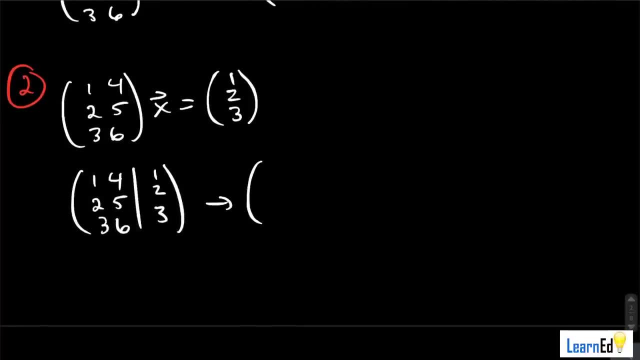 okay, we get a one, two, three. now let's start row reducing, okay. so i will zero out the rows below the first pivot- okay, and or the the, the two positions below the the first pivot- okay, and that we'll see how that ends up affecting these things. so we know that the 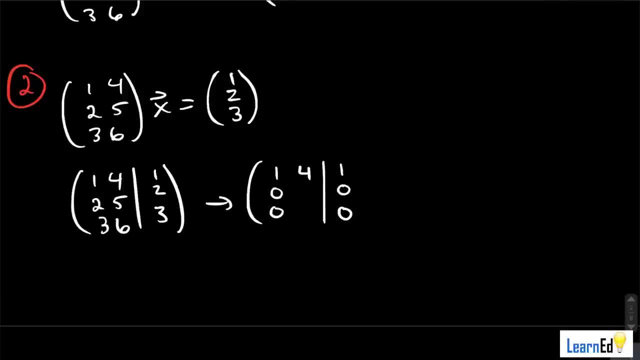 third column will actually go to zeros, because it it is identical to the first column, but for our second column in the, the position in the second row, well, we have to get to this zero here. we had to multiply by negative two and add. so we multiply four by negative two to get negative. 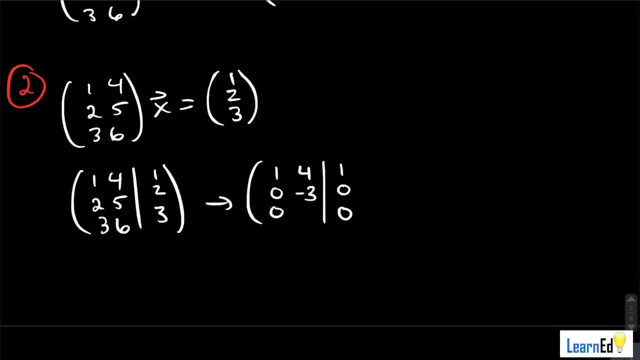 eight and add five to get negative three, and then doing the same exact idea, but now with negative three, because we have to multiply by negative three to get this zero here, we will end up getting a negative six here. okay, now you can see that we can do a scalar multiplication to reduce this. 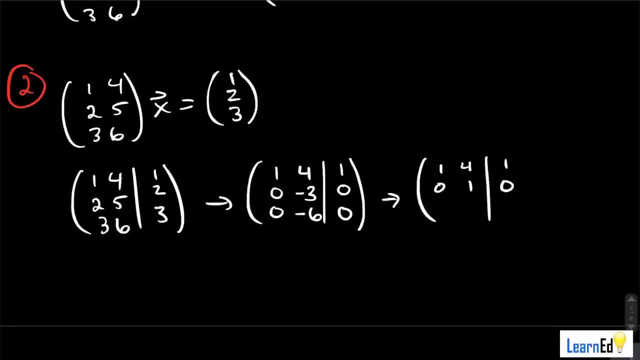 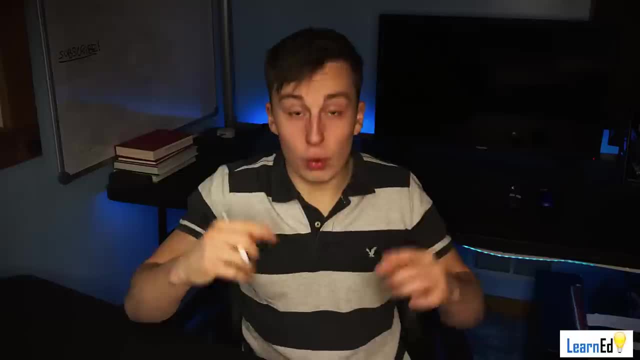 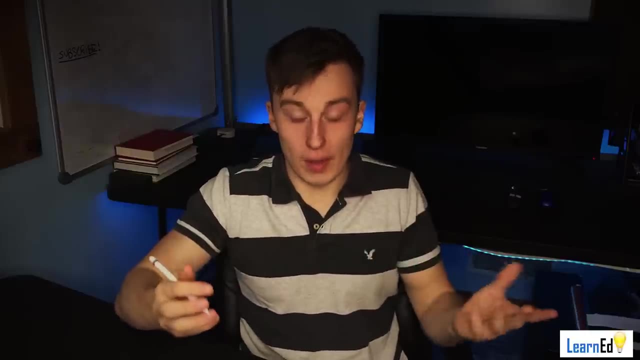 second row to zero one, zero, right, we just multiply by negative one third. you can also think of it as dividing by negative three. okay, and since the uh, the whole, the third row, the third row as a whole is a scalar multiple of the second row. we can also just zero that out. 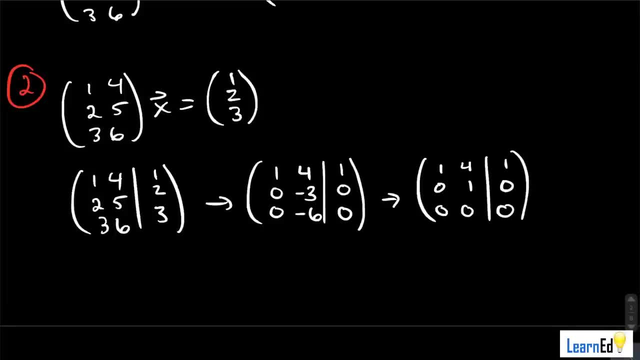 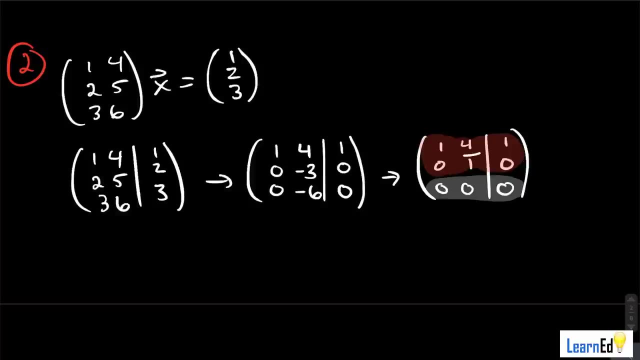 all right in that, since that we zeroed out that row that gives us a two-dimensional vector. right, because the only things that actually matter at this point are right here. okay, all we have to do now is get rid of that four right here and we can actually do that. uh pretty. 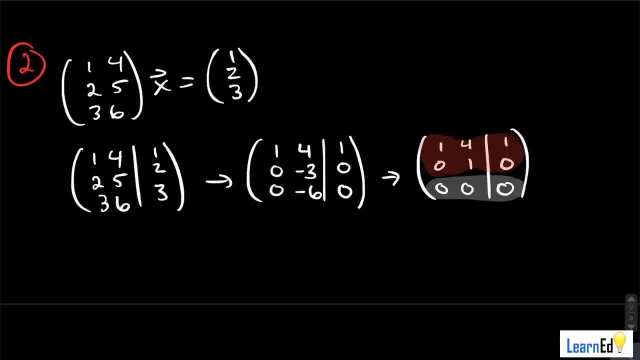 easily. we can multiply the the second row by negative four and add it to the first row. however, you you can just write it now as one zero, zero one and then have a zero, zero, zero, one, zero. so you can write it like this and not even really bad an eye, because you can see here that we have a zero. 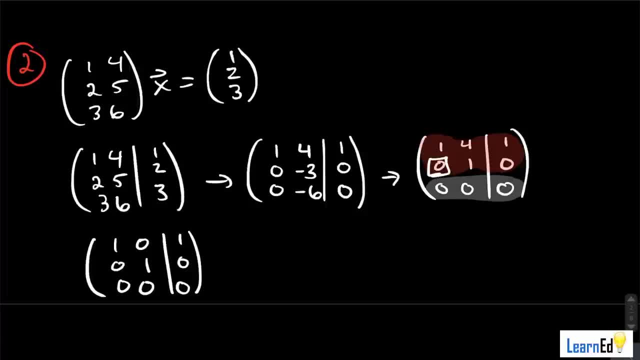 zero, zero, one, zero. so we can write it like this and not even really bad an eye, because you can see here here that all other entries in row two are zero. so there's not going to be any other effect, not on these other entries in row one. right, and that's a nice little trick that i, you know, i kind. 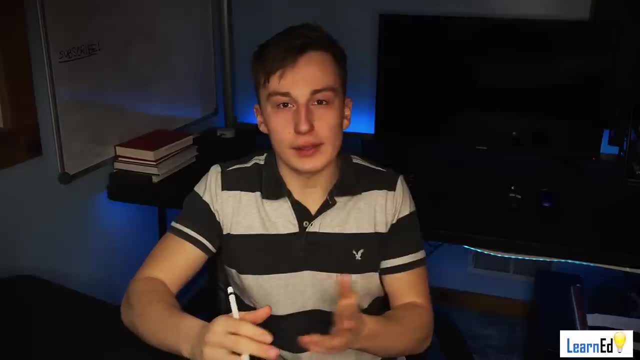 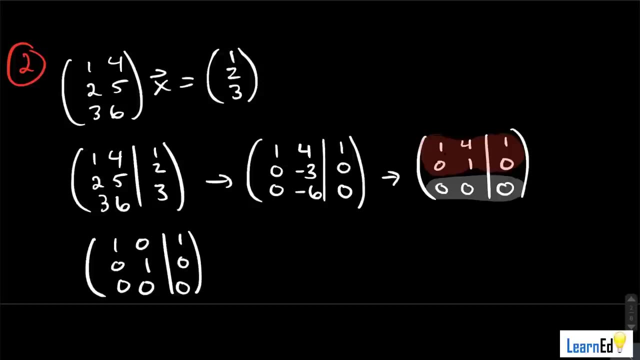 of figured out. when i was on working my way through linear algebra, i was like: oh, okay, so this makes row reduction a little bit nicer, okay, so a little bit less work. now what this tells you is that your vector is one zero, that that x, that will give you one, two, three is one zero. and that makes sense, right? because if 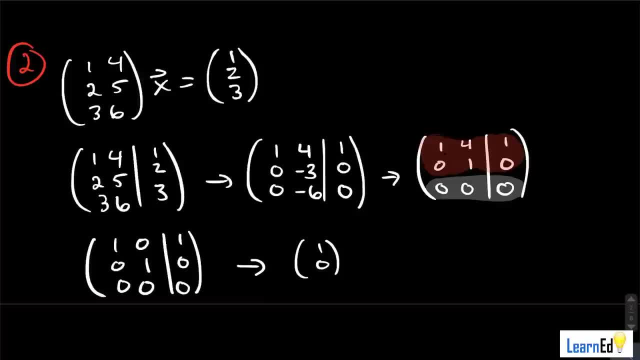 you put in right. let's say that we have one, two, three, four, five, six times one zero. you will get one times one, two, three, right, which is one, two, three. okay, just so. that that's kind of a check from the information, that, or from from how we know how to plug in at x from part one. 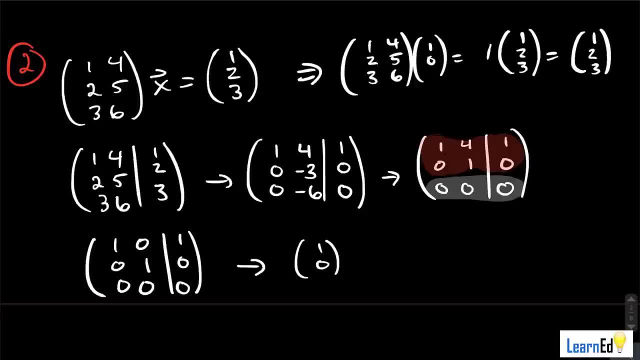 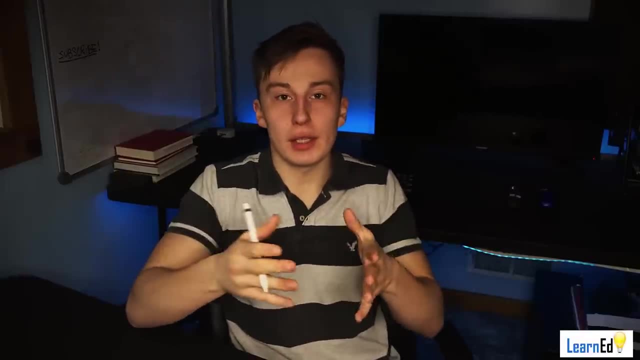 one. okay, now you gotta realize, though, that this is not one zero, zero. if you were wondering why it's not, it's because, like i said earlier, this row, when it zeroed out, you lose that dimension, and you lose that dimension because there's no longer a one. if there was a pivot there, you still have a dimension. 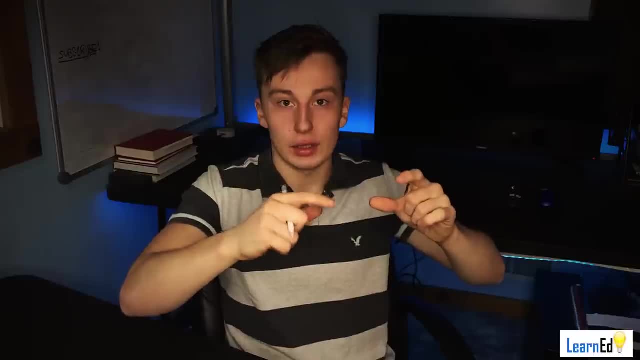 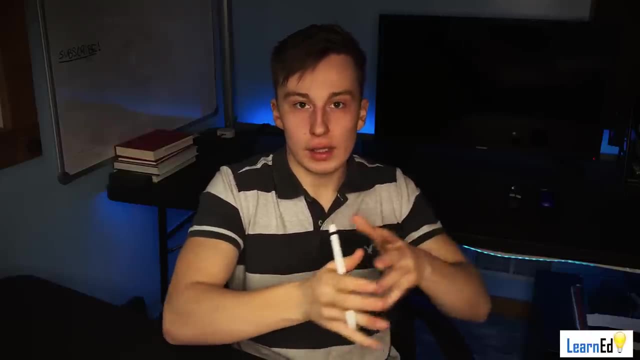 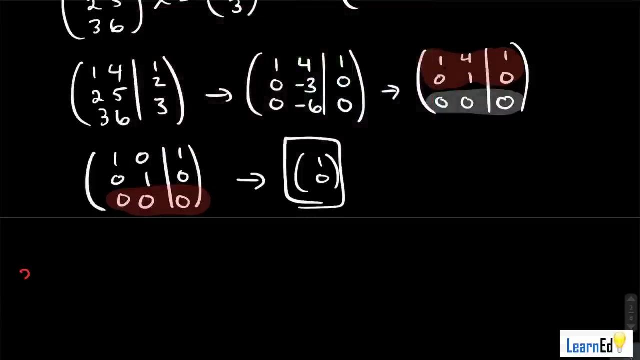 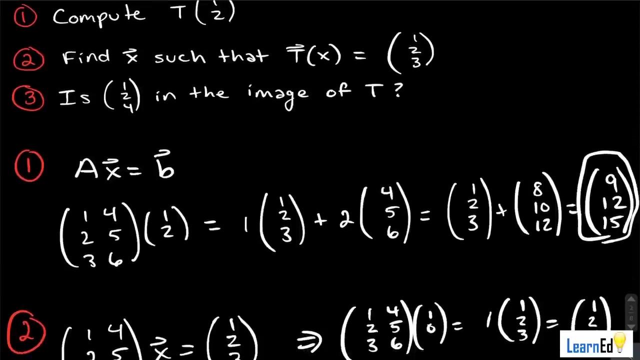 but you've lost that pivot, so you've lost that extra dimension. so now you have gone from a, a vector in three dimensions, to a vector in two dimensions. right, so you reversed the transformation. that's our answer. moving on to the third part, we want to see if one, two, four is in the image of t. 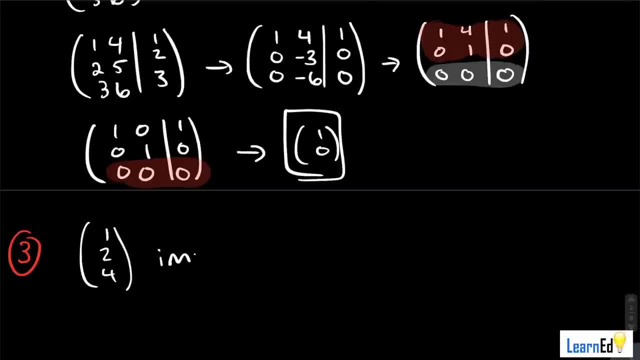 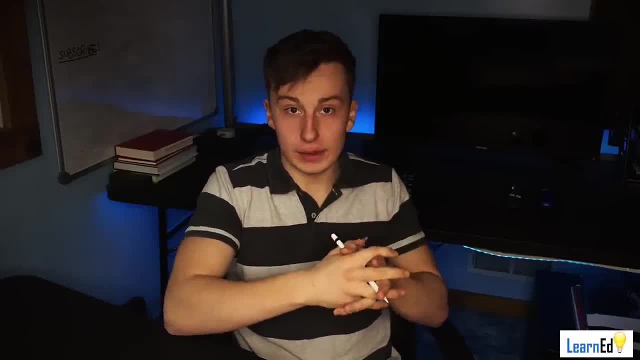 what does that mean? okay, all right. what does it mean for a vector to be in the image of t? okay. so what does that mean for a vector to be in the image of t? okay, well, to do that, we can actually look at some problems that we've already done. 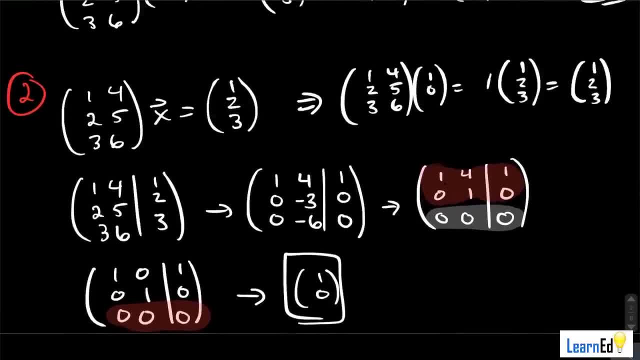 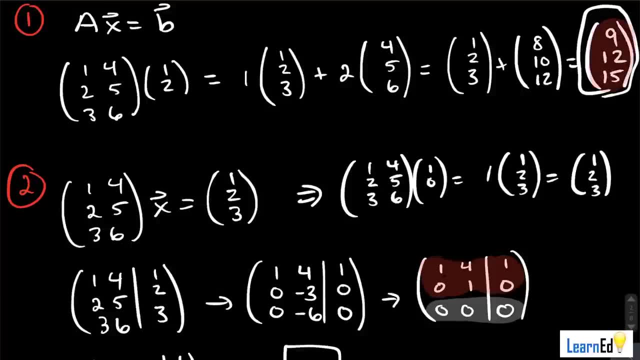 with this, with this question. okay, we can say that 9 12, 15 is in the image of t, because there is a vector that we can transform to get 9 12, 15.. okay, at the same as the same, in the same sense, we can say that: 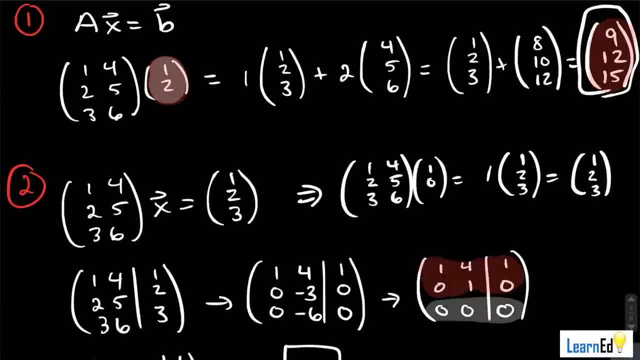 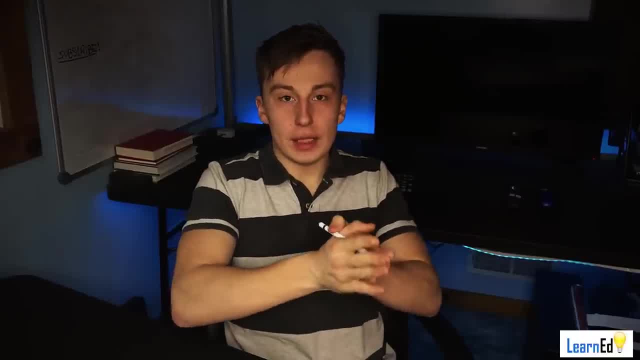 The image of 1, 2 through this transformation is 9,, 12,, 15.. So that's the idea of how the image thing works. okay, The image of 1, 2 was the resulting vector after you apply the transformation. 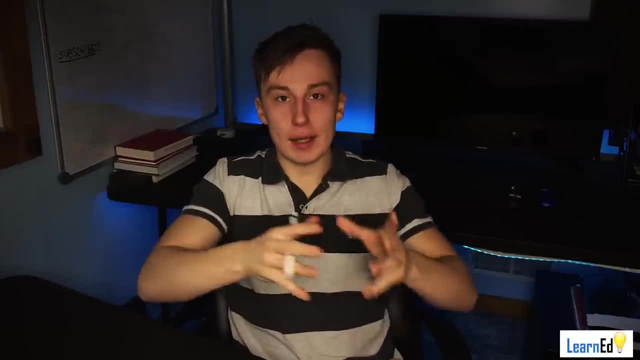 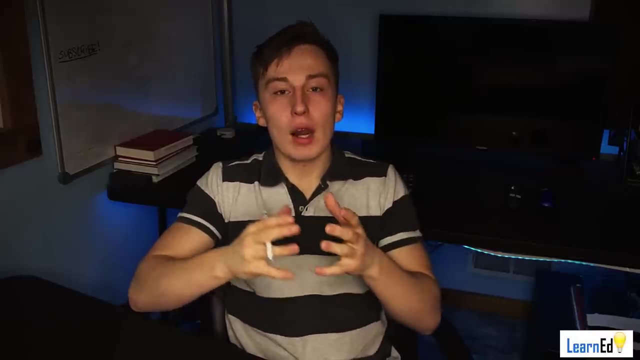 And so you could say 9,, 12,, 15 is in the image of t. So what does that mean for our problem? now that we have a random b vector and we need to see if it's in the image of t, We need to see if we can apply that transformation t to some two-dimensional vector. 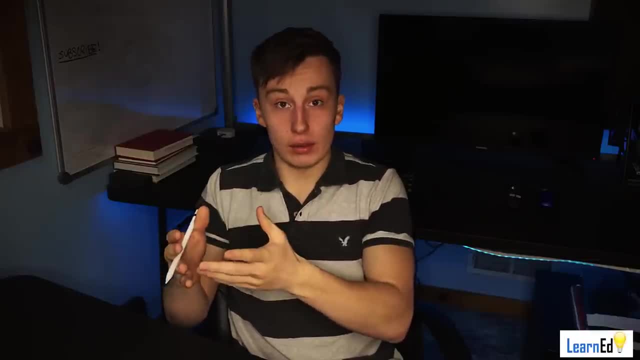 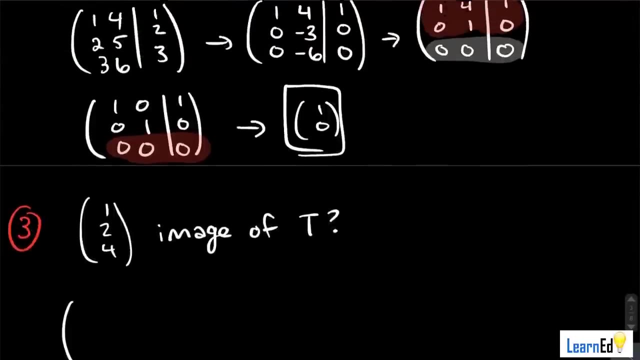 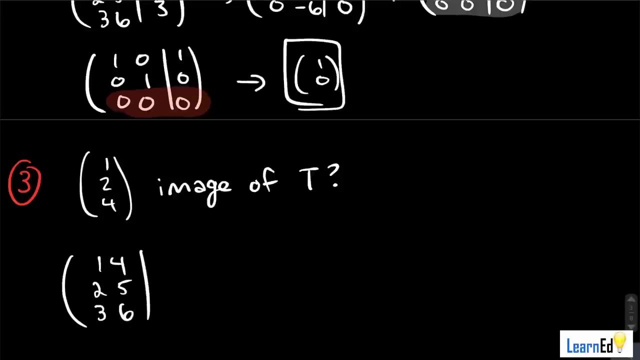 and get 1,, 2,, 4 as a result. That is what that question is saying. So all we have to do is basically the same thing as we did in problem 2.. We set up what we know our standard matrix to be. 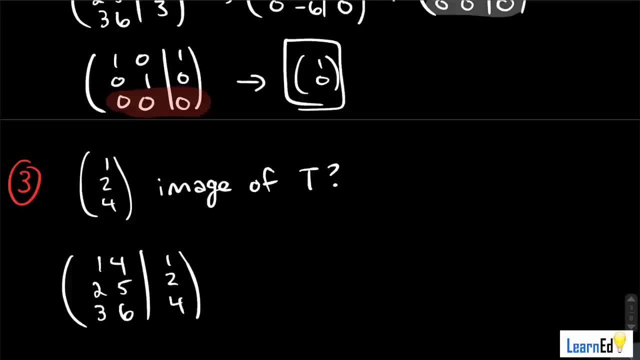 We augment it with 1,, 2,, 4 and see if there is an actual x vector that we can apply to the image of t. We can get out of this all right. So we zero out the two entries below the first pivot. 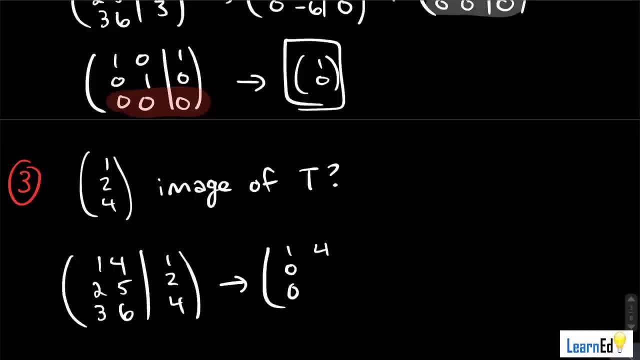 in the same fashion as we did before. okay, And this will become 0. And now, instead of having a 4 here, what we're going to get? we multiply by negative 3 on the top and add it to the bottom. 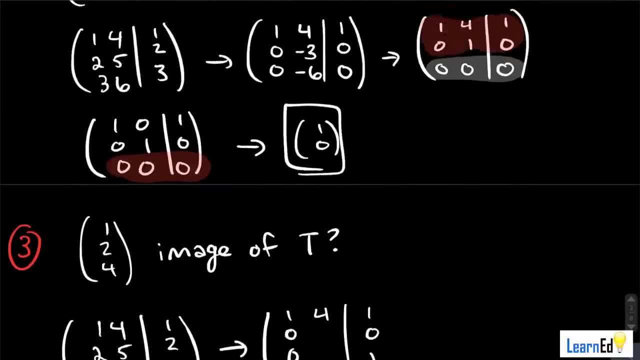 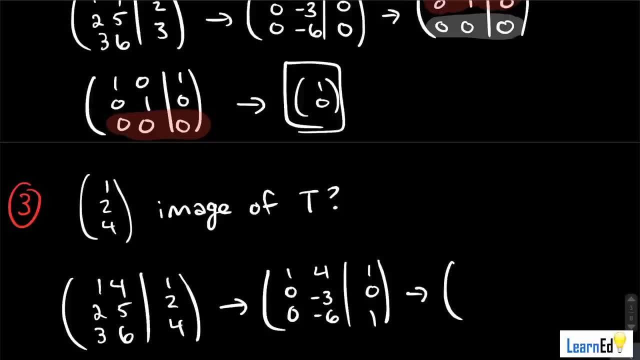 So we get a 1 here, all right. And then the 5 and 6, we know that those become negative 3 and negative 6, respectively. So we can scale down the second row and get 0, 1, 0.. 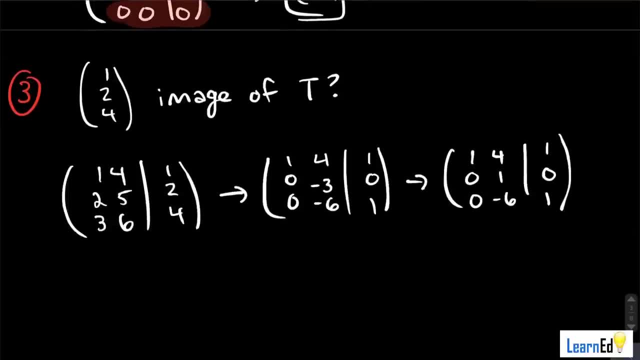 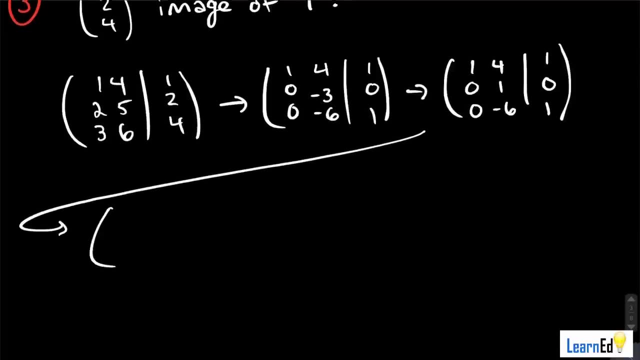 And we can just keep the other third row, because we can't scale that down or zero it out. now that we have this 1 here, That 1 entry is going to kind of mess with us, and that's fine, Because what you'll see here is that when we 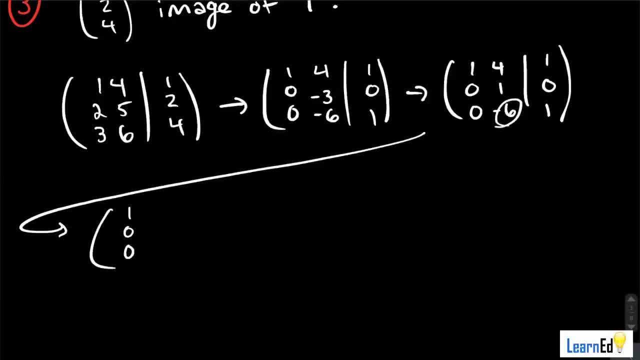 zero out this negative 6 in the bottom middle entry. what ends up happening? And note that we can do that with the second row, because there's two 0 entries here, as I mentioned before. So what we can do is just zero out that 6. 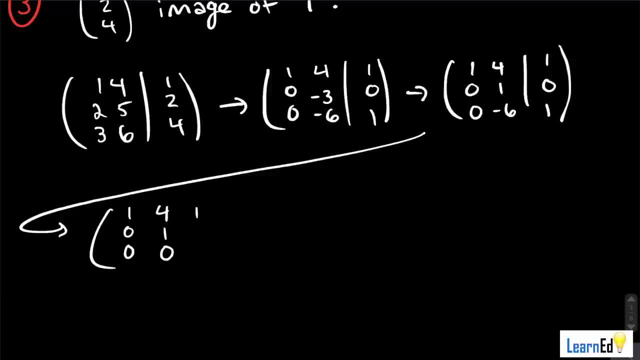 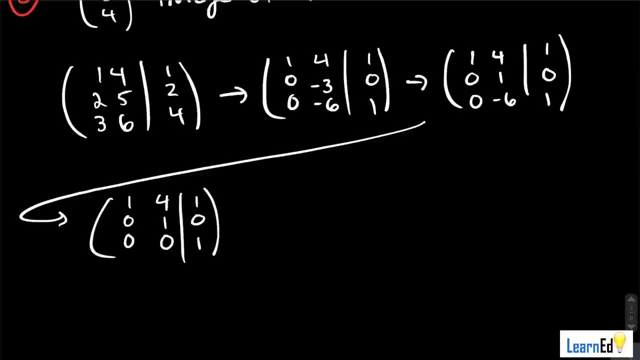 without having to worry about anything else being affected. So we get 1, 0, 1, okay. So here's the problem, though Remember this is augmented. We have a 0 equal to 1, right. 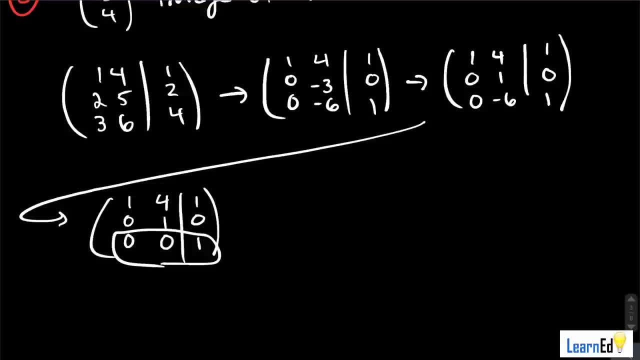 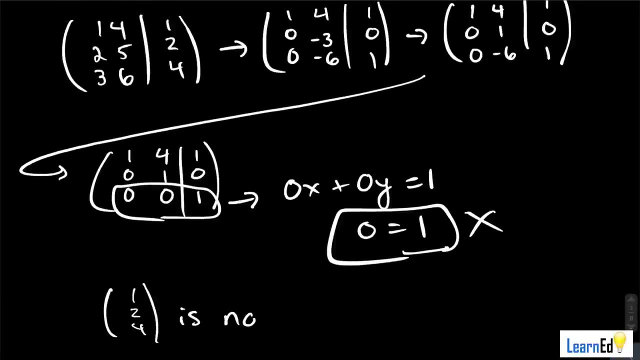 That's essentially what this is saying. This bottom row is saying that 0x plus 0y equals 1. And that means that 0 equals 1, which we know is not true. Okay, So our answer is that 1,, 2,, 4 is not in the image of T. 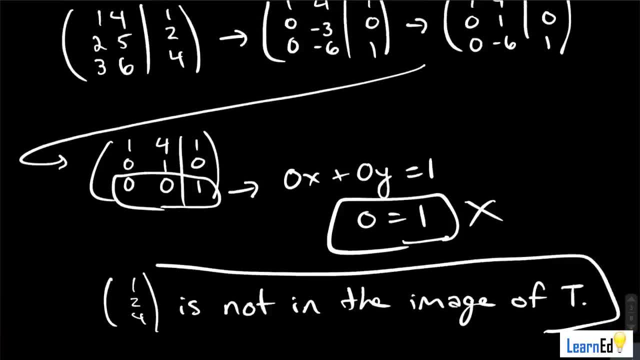 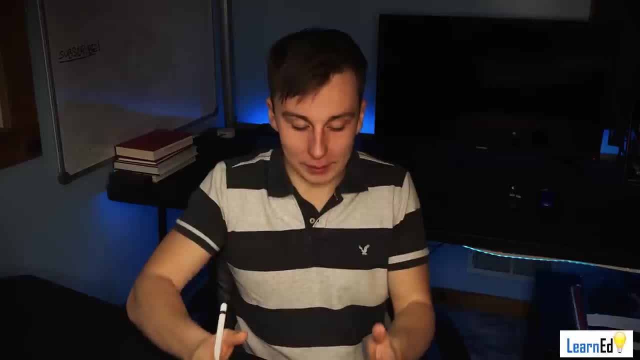 All right, And that's the. That's the answer to the last part of our problem. So hopefully that example makes you, helps you to understand transformations a lot more. I know if I had somebody sit down and explain it to me like this: 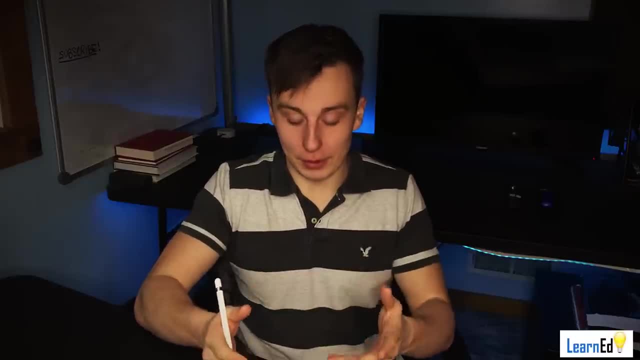 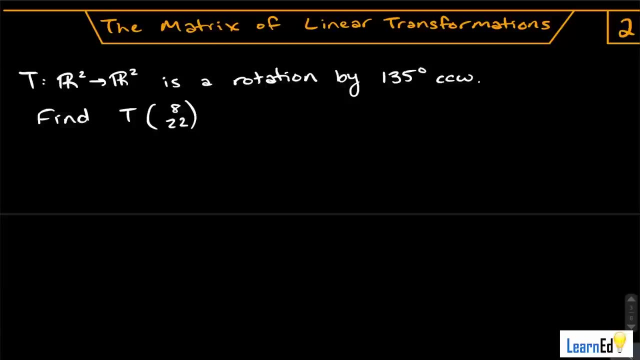 I think I would have understood transformations a lot better, So I really hope that's the same for you. Now let's move on to talking more about transformations. when we talk about the matrix of linear transformations, Okay, So we have a transformation from R2 to R2,. 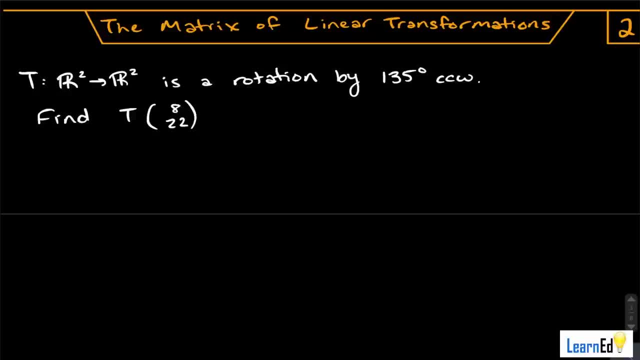 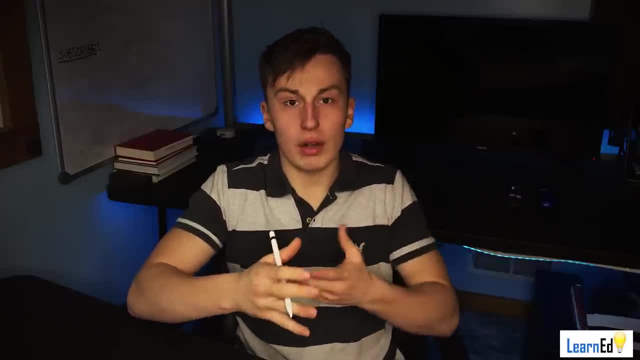 and it's a rotation by 135 degrees, counterclockwise, And what we want to find, what we want to find is T of 822.. Now, when we're talking about a counterclockwise rotation, okay, or we're talking about any rotations at all. 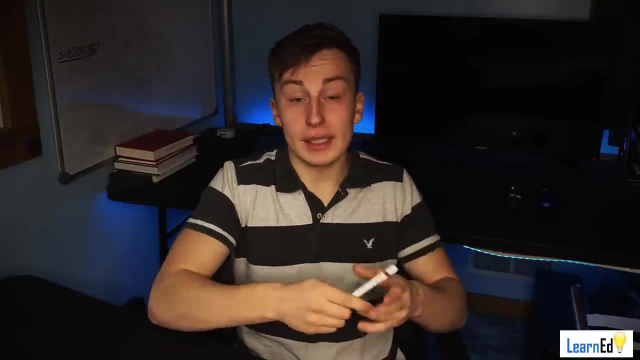 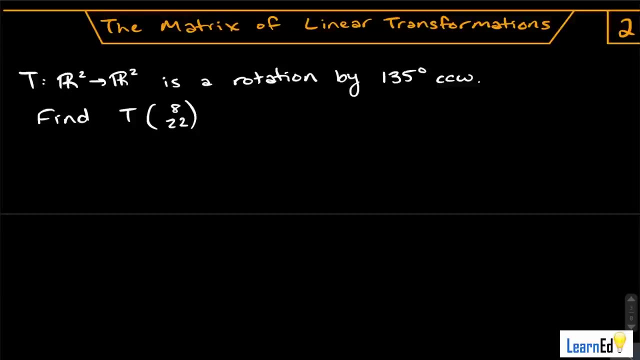 we can kind of think of the unit circle to help find our standard matrix here, Because, as you notice, that's what we're missing in this problem. Okay, So let's go through and do that, But where do we start? And that's a valid question, right? 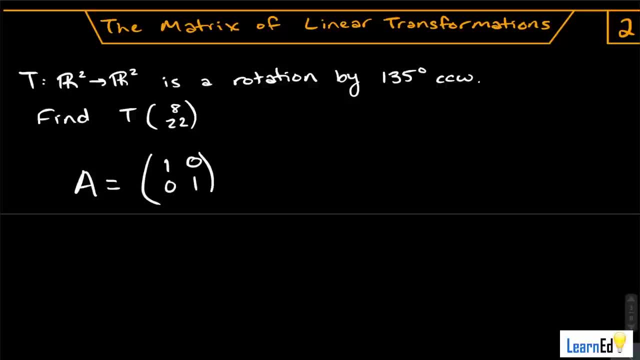 If we said that our standard matrix was 1, 0, 0, 1.. Well then, if we multiply this by 822, you'd be able to see that we get the vector 822 back. Right, Right. 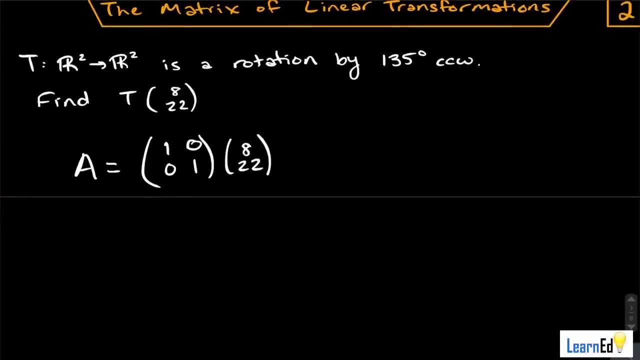 Because that's just the, just an identity matrix. So what we want to see to get our standard matrix is: well, what's going to happen to this, this a, when we do 135 degrees counterclockwise rotation? Okay? 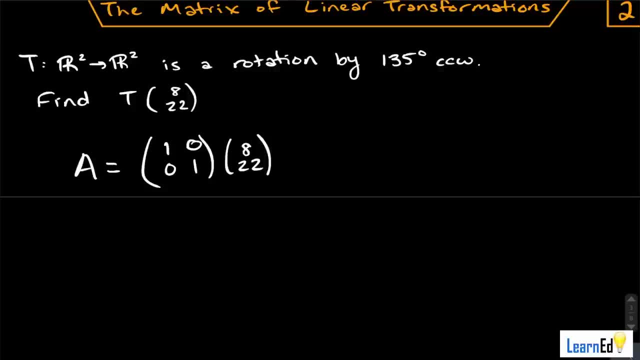 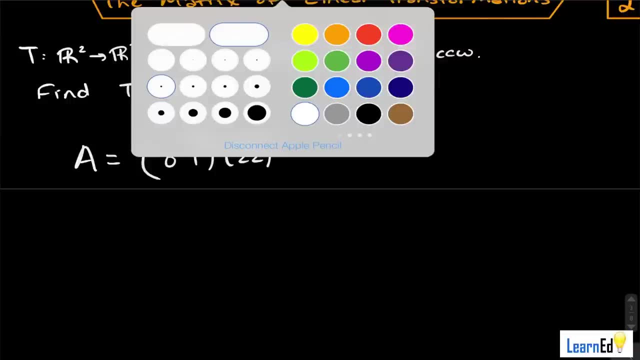 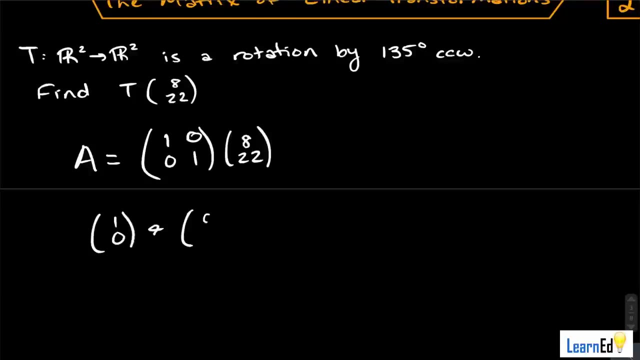 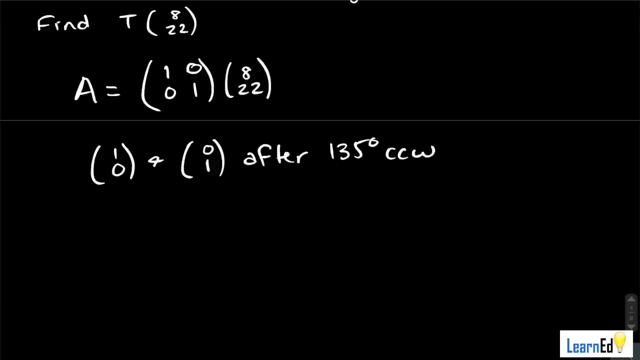 And if we can figure that out, that out and figure out what our new a will be, well then we've found our standard matrix. we apply that to 822, we solve the problem. okay, so let's first examine one zero and zero, one after 135 degrees of counterclockwise rotation, and to do that we'll graph them. and this is where 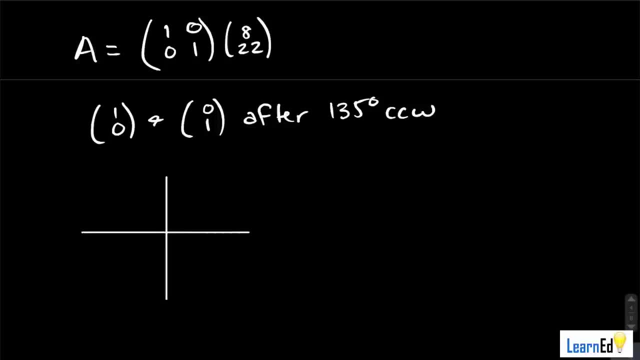 you can kind of see the unit circle idea coming to play. let's color. and I saw I know I've kept this like color menu open for a while, so I will tone that down. I'm so indecisive sometimes honestly. but let's say we have that vector one, zero, okay, and we rotate 135 degrees counterclockwise. 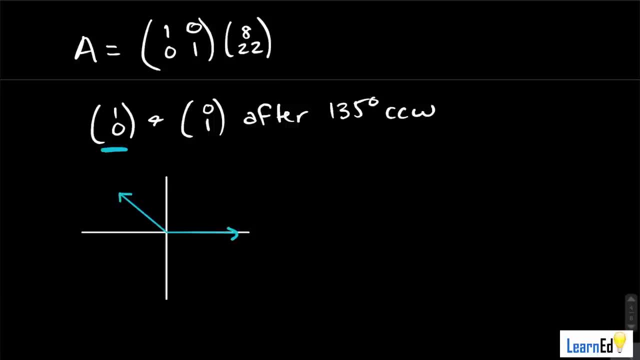 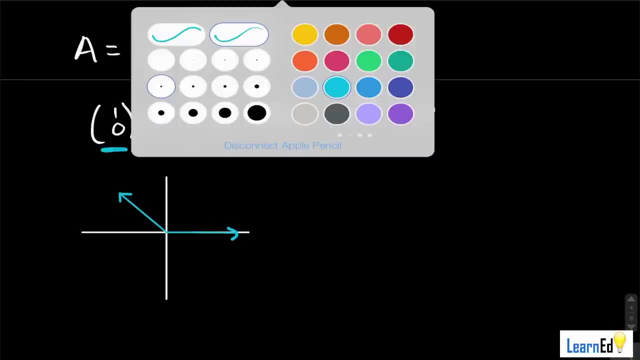 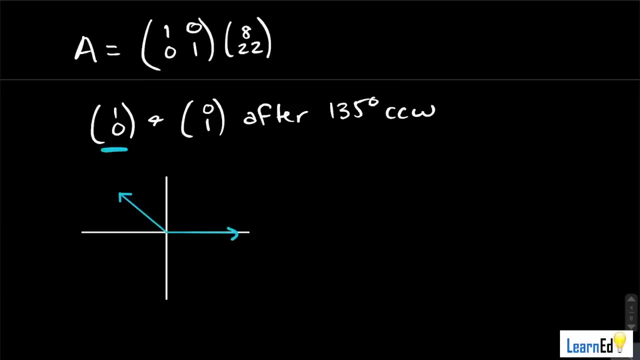 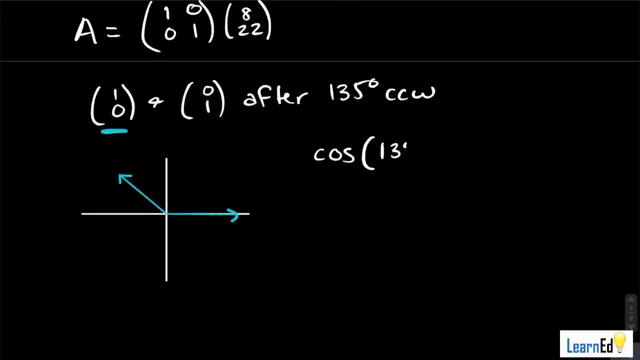 so our resulting vector is over here, okay. well, now what are the x and y components of our vector? new vector: well, we know, that that's. we know from like. what's that? like algebra 2, pre-calculus, or something like that? that our new components? we just take the cosine of 135 right, and then that's. 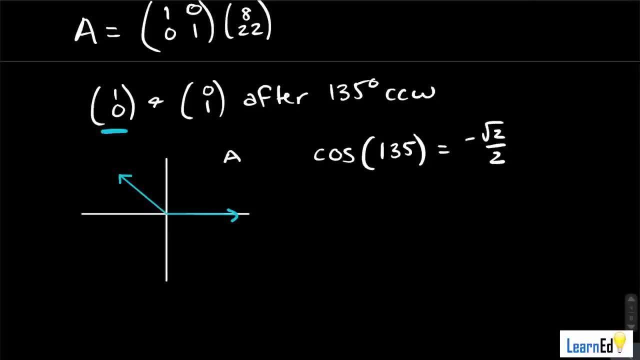 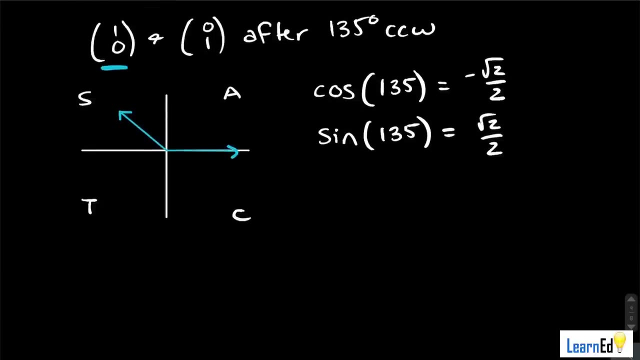 equal to negative rad 2 over 2. right, we know that cosine is going to be negative in the second quadrant. and then, if we do sine of 135, we know that's equal to rad 2 over 2. okay, and so there's, there's your components, and that's going to be the the. 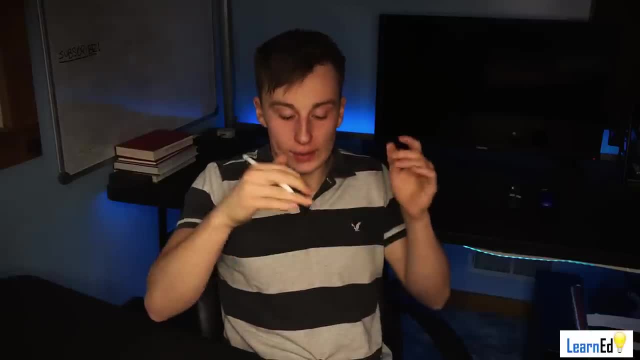 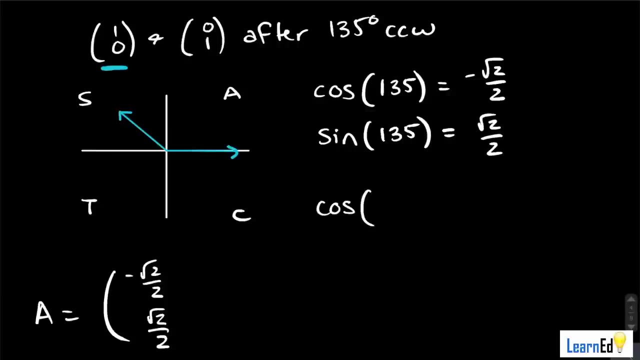 resultant- uh, that's the resultant vector from one zero. so that's what we put in our standard Matrix. okay, so now we can do the same exact thing for our zero one vector, and that will just end up going down here when we do an 135 degree rotation, and that will now be. 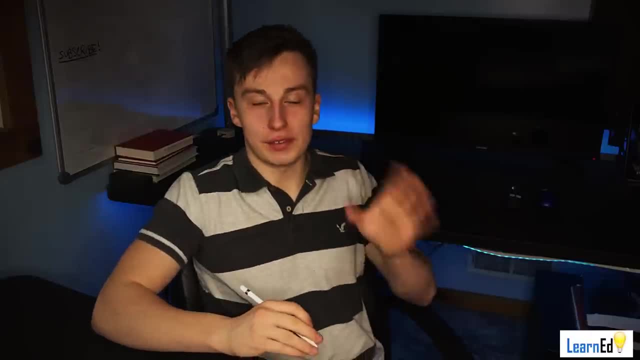 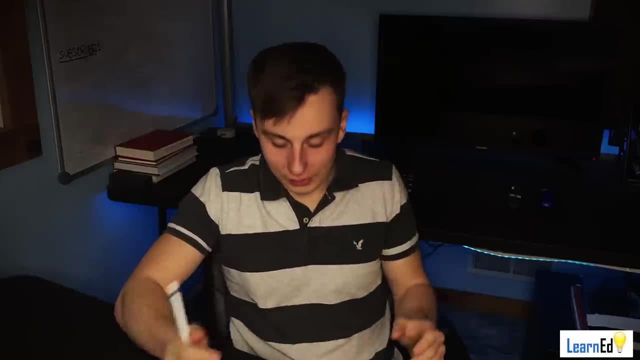 at a 225 degree rotation. and guys, I apologize for some background noise. I have no idea what's going on downstairs and it's. I hope it's not ruining the video, so I apologize if that's been bugging you. um, I don't want to stop the video to tell him to tone it down, but sorry. 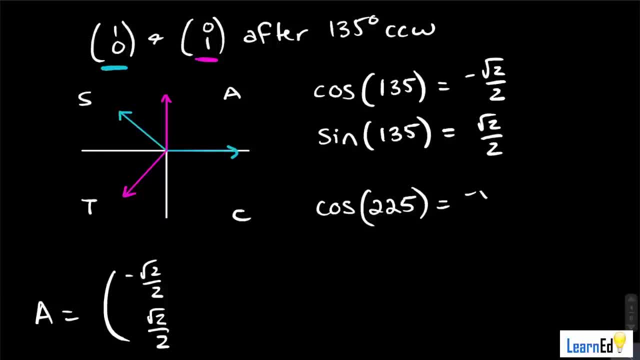 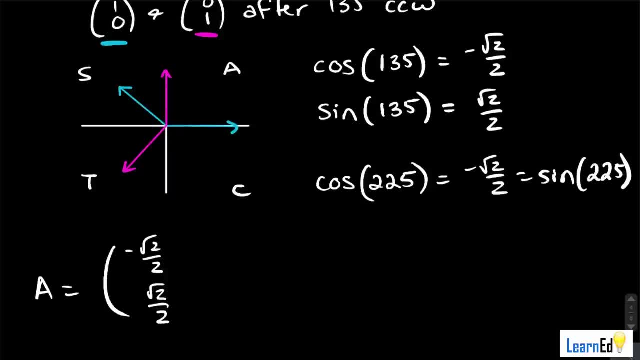 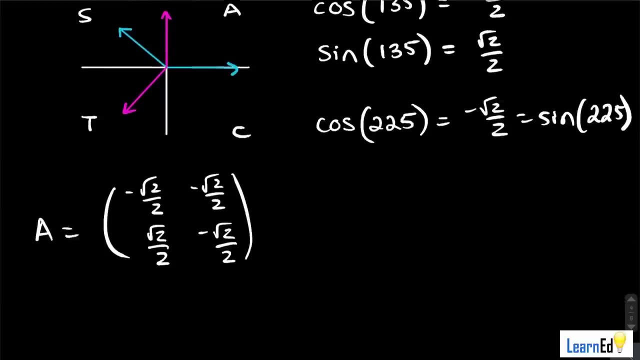 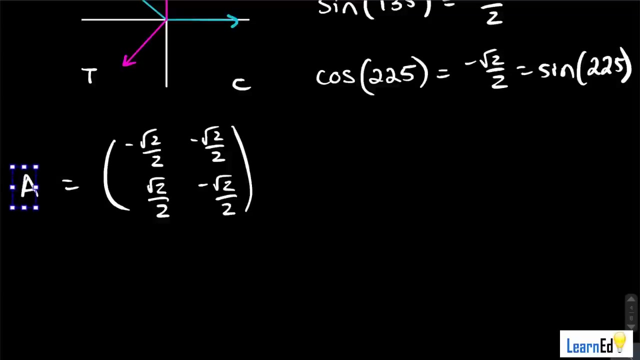 uh, so anyways, cosine of 225 is negative, rad 2 over 2 and so is sine of 225. So I'll just write it, like to save space. okay, putting those in. we now have our standard matrix. we can now multiply this standard matrix by, and we'll instead write this as a of x, right, because we know that our x here. 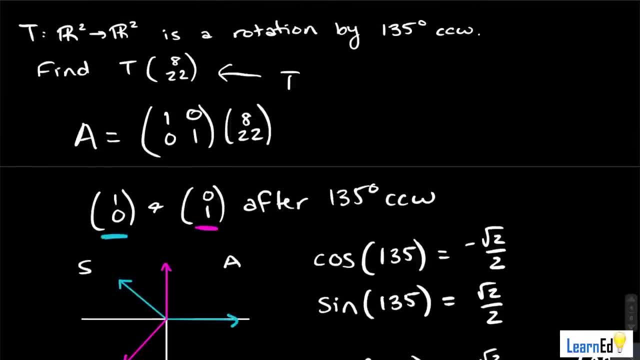 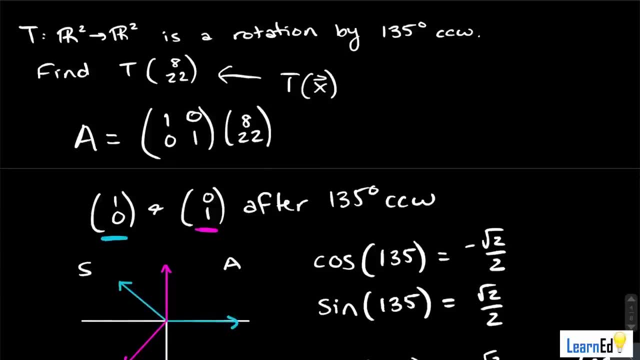 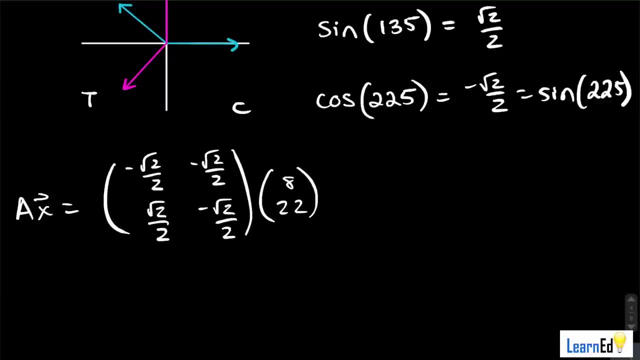 is 822. right, we know, because this is t of x. right, there you go. that's how that should be noted, right? so we plugged in a vector x of 822, so we have 8 and 22 there. so now we can multiply 8 by. 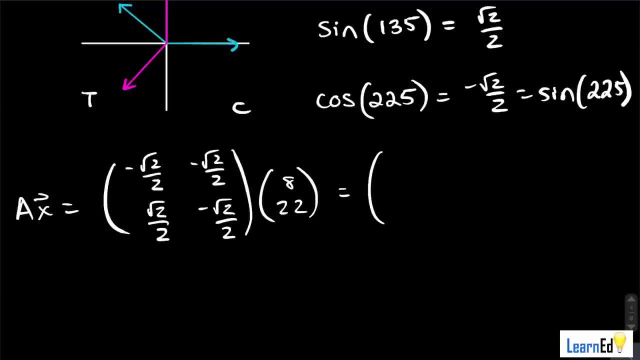 the the first column, and we'll get a negative 4 rad 2. and we multiply, uh, by the the sorry, the second column, and we'll get a negative 4 rad 2. and we multiply by the the sorry, the second entry in the first column, and we get a 4 rad 2. then we do the same exact thing for the. 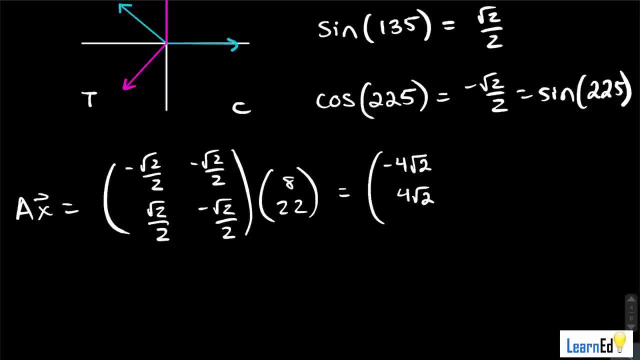 second column, but now with 22 and we have a negative 11 rad 2 and a negative 11 rad 2, so we can- and sorry, this is not in the correct. uh, yeah, this is not correct. hang on, i'll figure this out. plus, there we go. sorry about that. so this is now equal to: 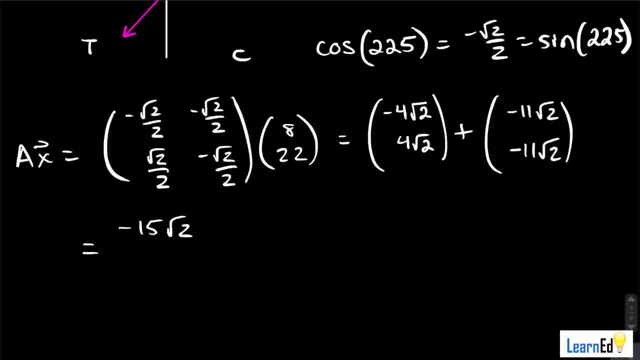 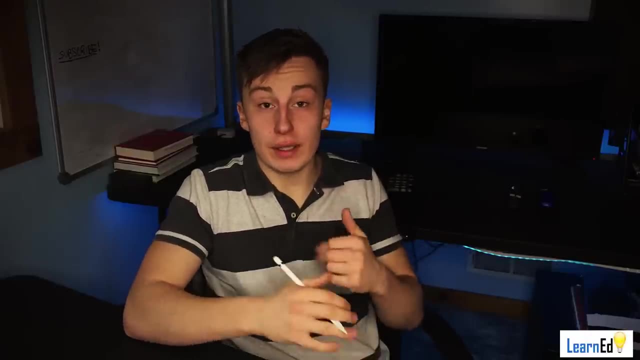 negative 15, rad 2, and we multiply these two entries and we get a negative 7, rad 2. okay, and now we can circle that. that is our answer, okay. so you know, the hardest part about a problem like that is really just finding the standard matrix. if you can do that, then the problem. 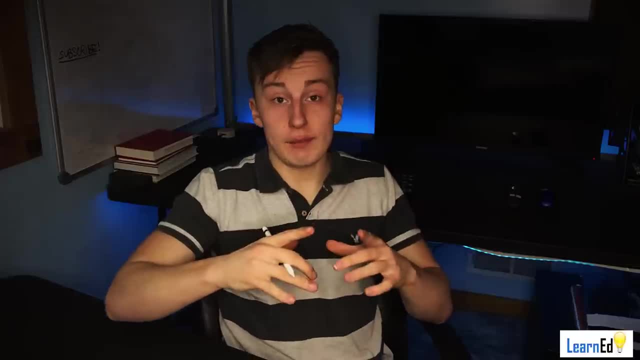 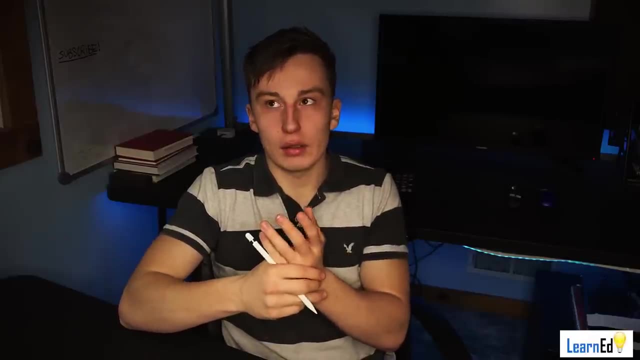 is all downhill from there. you multiply by your, your x vector. that's your input and our output, you can now see, is a 2d vector and we're going to get a negative 7 rad 2 and we're going to get a negative 7 rad 2, and we can also check that, by the way. i mean, if there was ever a situation where 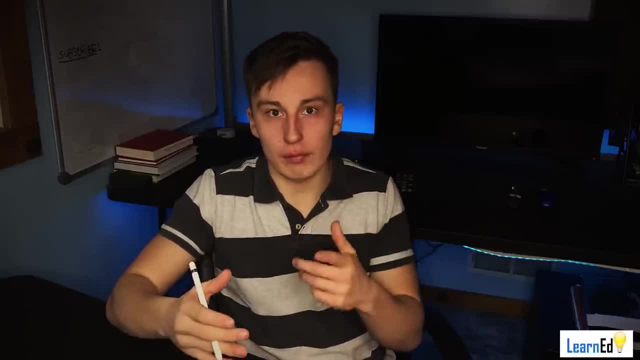 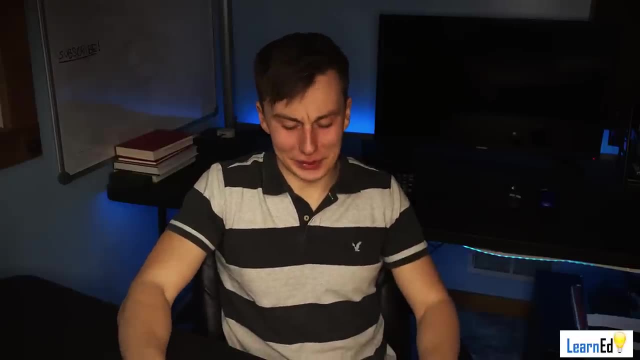 your transformation is from r2 to r2 and you end up with the three-dimensional vector. well, you know, something's up and you can correct that. okay, so you know, there's just some- hopefully helpful- insight into a problem like that. let's move on to the next problem, and the next problem is asking us: 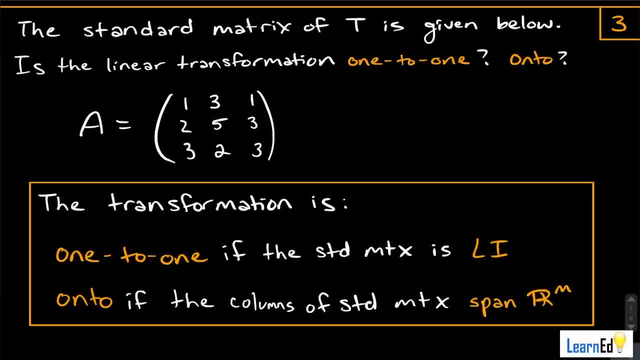 if the standard matrix of- or sorry, it's saying the standard matrix of- t is given below, is the transformation one-to-one and is it on two? so we know that we have a right here. we have our standard matrix, right, that's our standard matrix of t and we're asking if it is one to one and if it is on two. now, 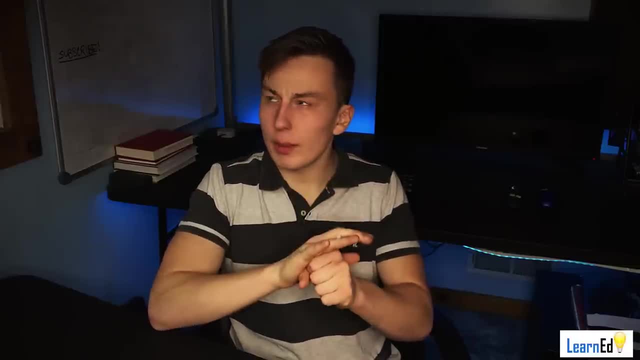 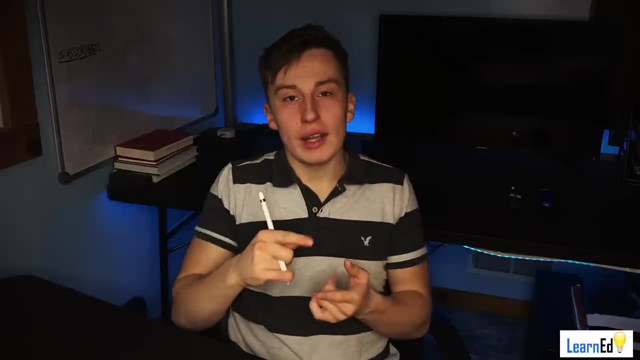 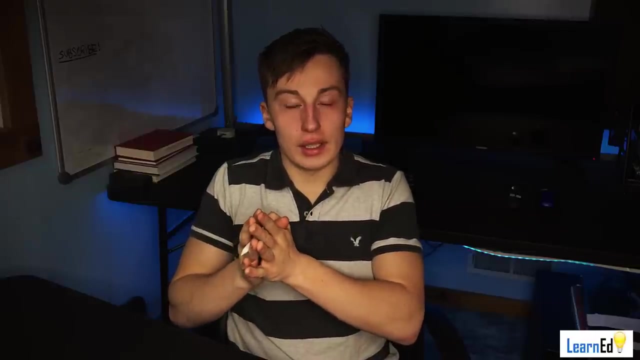 these are big terms. when you talk about, uh, we talk about invertible matrices, right? we'll actually do a problem with that later, trying to see if a matrix is invertible. a matrix is invertible if, if it did this, if it is one, sorry, a linear transformation is: uh, if it is one to one and on two, then the standard matrix is invertible. 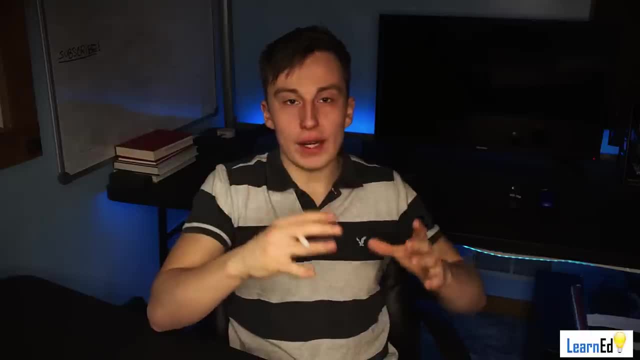 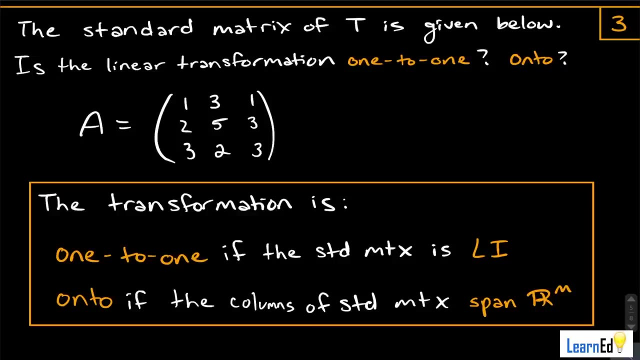 okay, so if an and you find out if your linear transformation is one to one and on two from the standard matrix itself, okay, and i'll show you how, so that that might seem confusing, because i'm throwing a lot of like- probably not new terms, but terms that you probably 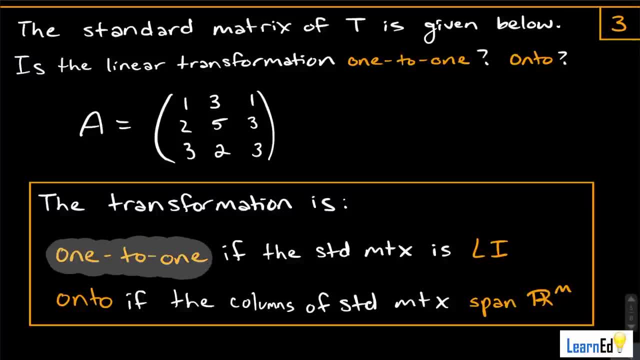 haven't heard in a while, perhaps. anyways, the transformation is one, two, one if the standard matrix is linearly independent. okay, so if you end up with something like this, where you have, uh, you know some, let's write this like like this: so we have some, we, we have some entries, some non-zero entries and we have a zero row, okay, we know now that this is. 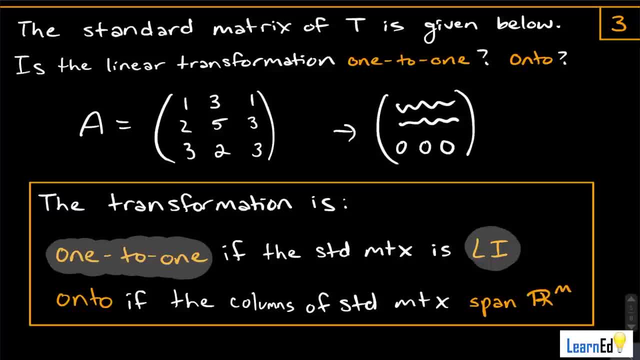 linearly dependent. okay, and that would make it so we end up not having a one-to-one transformation. now the transformation is on two if the columns of the standard matrix span rm. okay, so remember, if that terminology is confusing to you, that a matrix has is m by n, so it has m. 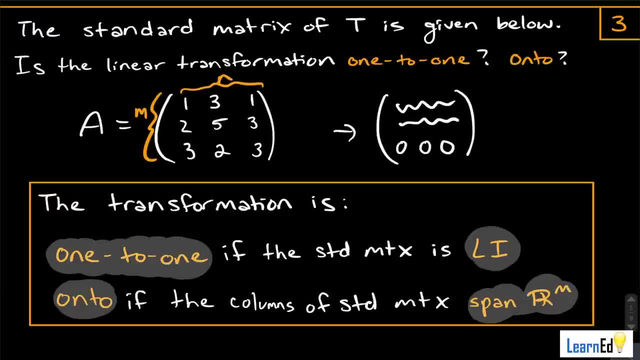 rows and it has. that's a terrible curly bracket- but it has n columns. okay. so if we, if let's say that we do our row reduction and all these columns go to zero, okay, well then we only have two valid columns left, and that does not equal. 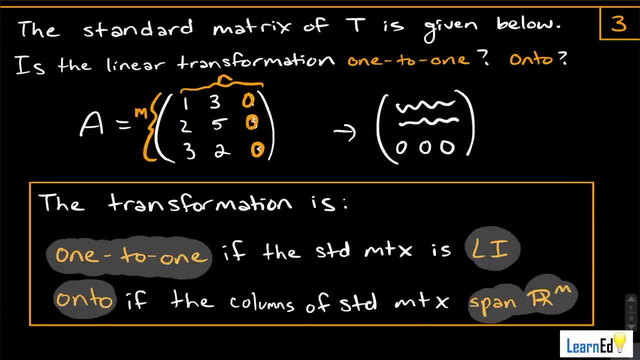 the three rows that we have, so it doesn't span rm. okay, so that's the idea. and if you're wondering, okay, how do i remember, m by n is row by column. well, how i like to remember it, r by c is rc car. that's what, that's what always, uh, that i used and that also helps with matrix multiplication. it also 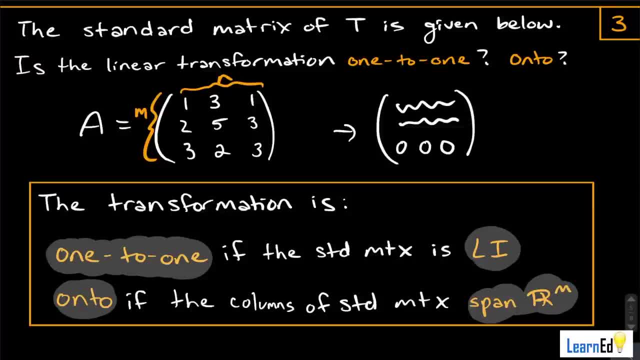 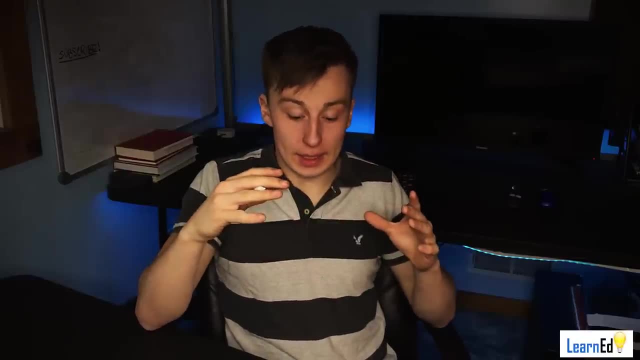 it helps in a bunch of different areas actually, but anyways, that's how that works. now, yeah, i already showed you a, a matrix that would have not been onto, and also, if you get any type of matrix that is not a n by n matrix, okay, if it's not an n by n matrix. 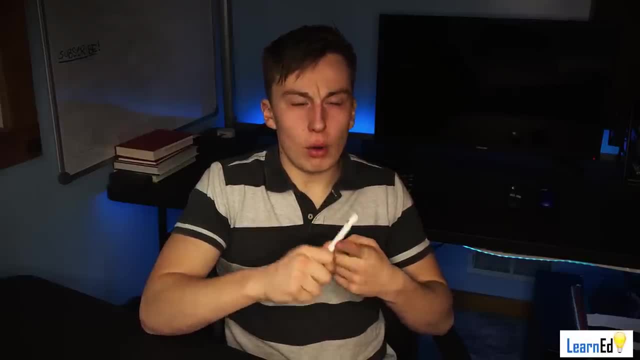 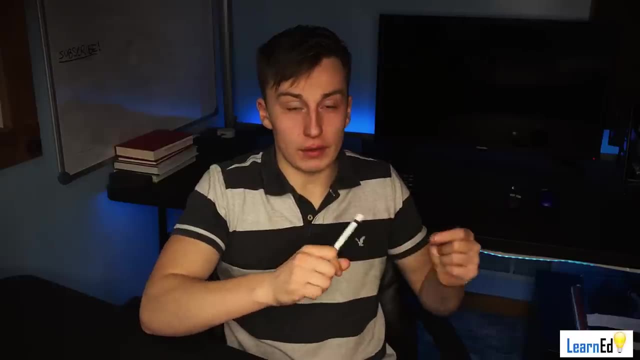 then you will, i believe, always have a matrix. that is, yeah, you will. you will never have a matrix that is both one to one and on two. okay, because you always have either a zero row or a zero column. i believe, and- and you can correct me if i'm wrong, but i believe that's true, because i don't think. 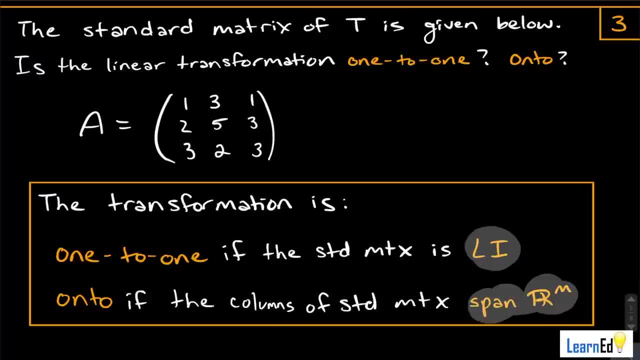 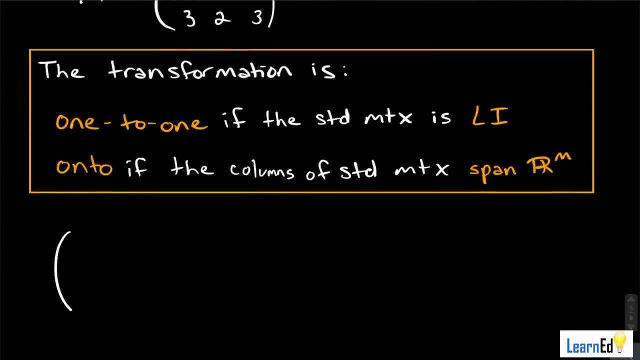 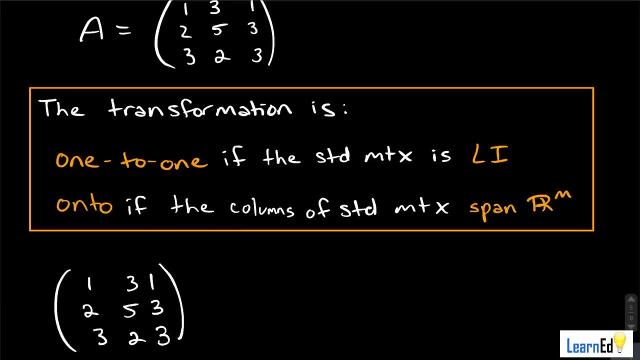 you can invert a matrix that is not n by n. we'll figure out probably later in this video. so anyways, let's get into this problem here. let's just start row reducing our standard matrix and we can again zero out the first the, the first two entries under the first pivot. okay, and we will. 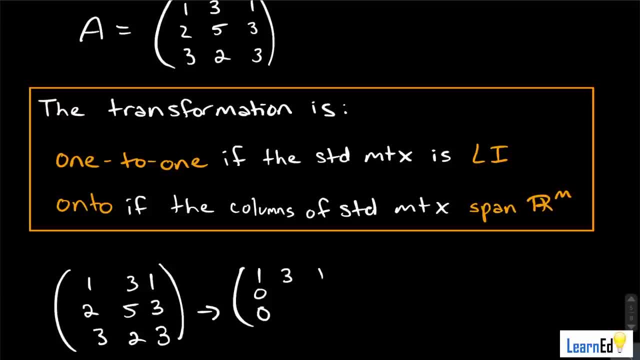 get a. since this is a five here, we will get uh times negative two, three. we'll get a negative one here and then in this entry, here this will be- we have a negative two times one, so we'll get a one here, okay, and we for our, for this entry: here we have negative three times the. the top plus two is: 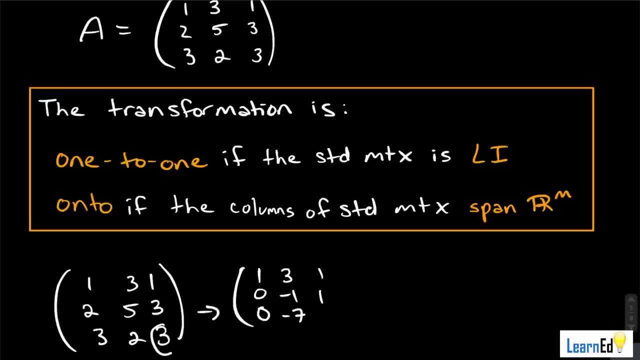 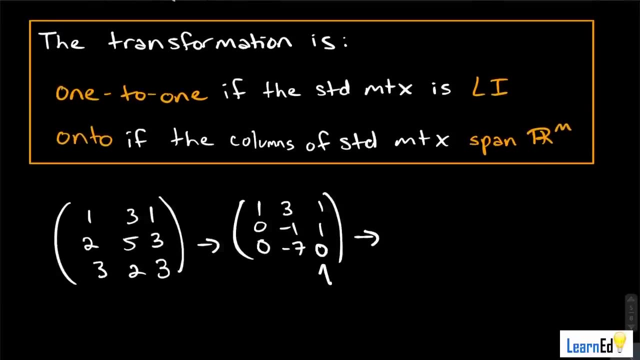 negative seven. and then for this bottom entry here we have negative three times one is negative. three plus three is zero. now a big thing to note here. don't write this off right away as being linearly dependent, because you see a zero here. okay, because, as as you're going to see later in this problem, a non-zero. 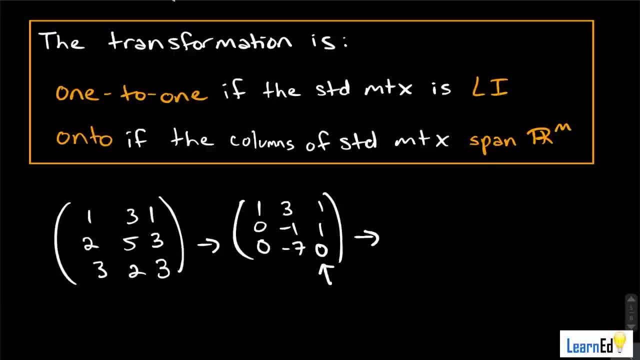 entry is going to pop up there and it's going to end up being linearly independent spoiler alert. okay, so don't try to jump to conclusions too early. and, by the way, we could also perform a row swap, so we don't deal with something like that anymore. okay, and we actually will have an entry. so if we 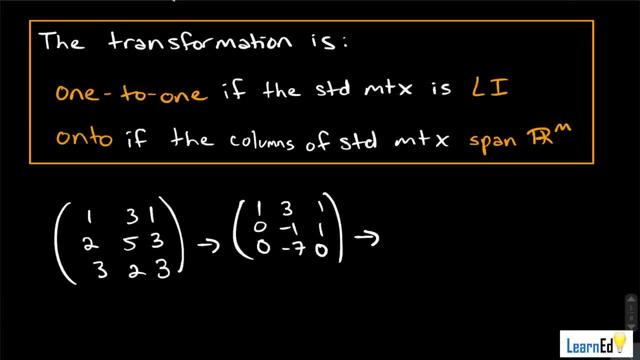 did a row swap between the second and third rows, we wouldn't have that situation anymore. okay, and actually i might do that here. it might be a little bit simpler to do something like that here, okay, so let's go ahead and do that. one, three, one. we'll do zero and we'll make this negative seven. 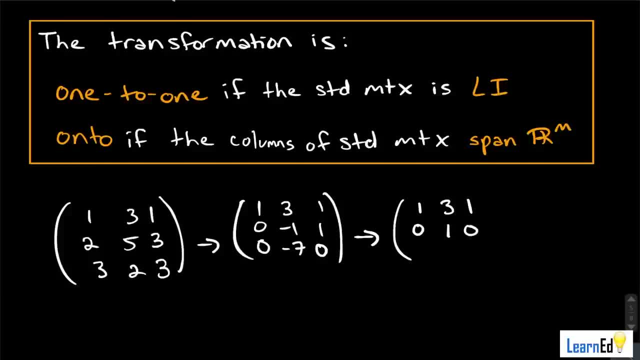 eight, we'll scale it down to be a one and we'll put it in the second row. and then we'll have zero negative one and one and then we'll spell it as negative seven and then we'll put it in the second row. i will put that in the third row, okay, so now you can see again that we have a non-zero entry. 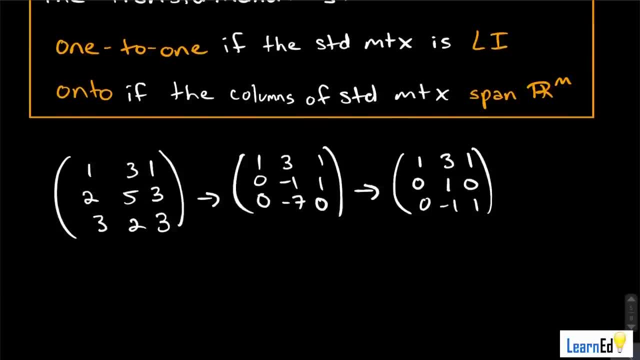 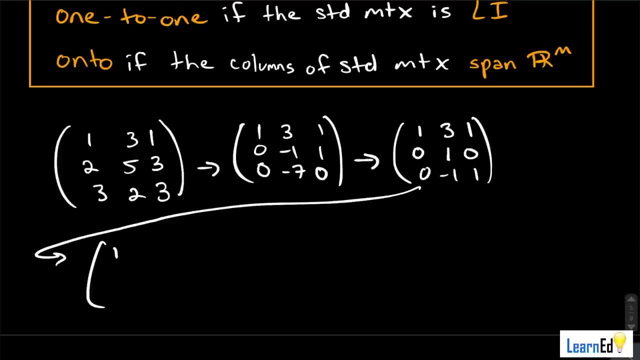 in the bottom right, so this will still end up being linearly independent. okay, so we have one. we can actually. well, let's not do anything yet to this three in the the top row, because we still have this- sorry, this is not there, you go one. we still have this negative one here that we had to. 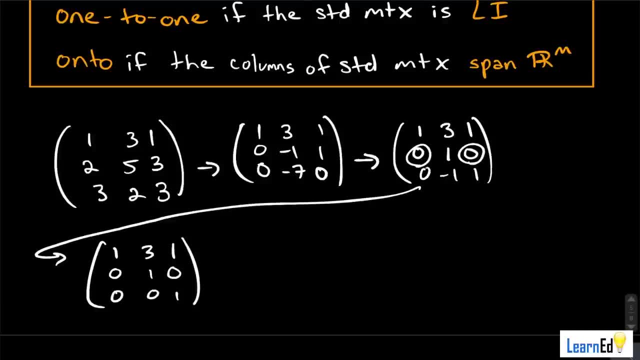 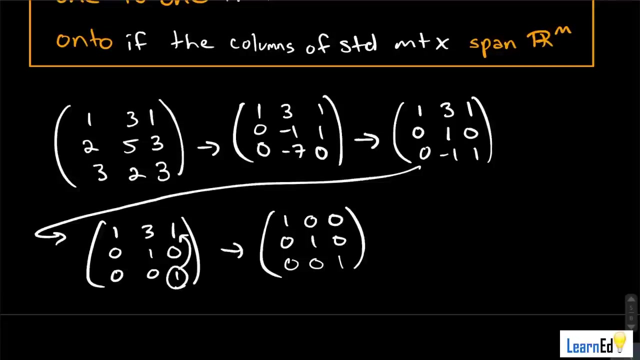 zero off and again we had a zero and a zero here. so no effect, no other effect. on the third row, we can zero off the three and the one in the top row because this one will be able to zero off three- three for the reason I mentioned before, and also this one will be able to zero off this one. 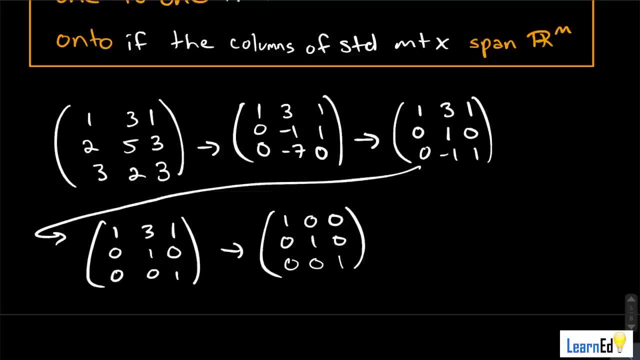 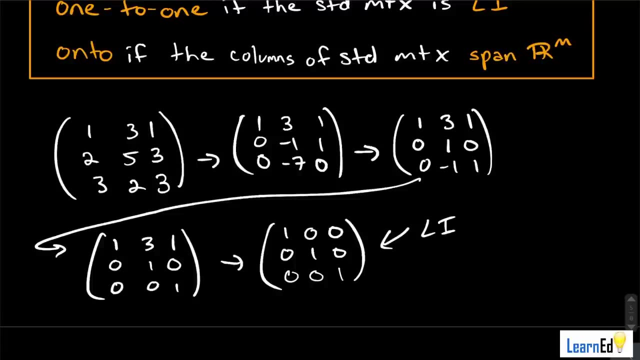 because all other entries in the row are zero, so there's no other effect on row one. so you see, here we have a linearly independent matrix and also you can see that it's onto because all of these columns span rm okay. so spans rm, columns span rm okay. 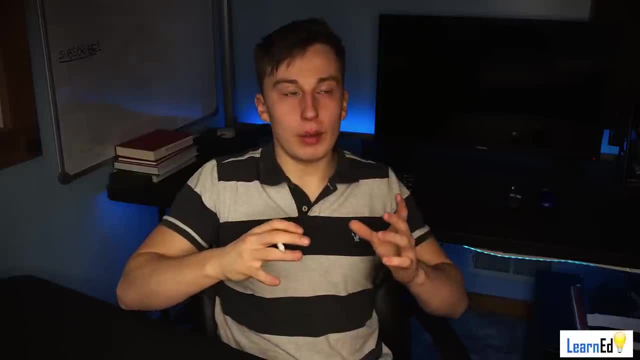 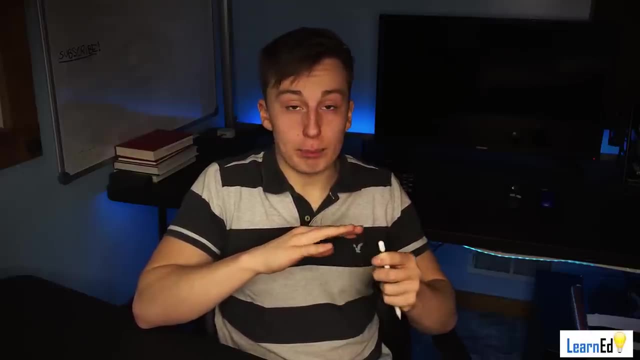 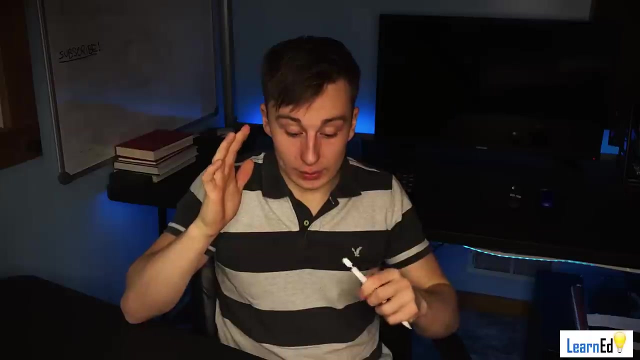 so you know probably a way to generalize this. I guess it's going to be one to one and on two, if there is a pivot position in each column- okay, there's a pivot position in each column- then this is going to be linearly independent and it's going to span rm. so it's going to be. 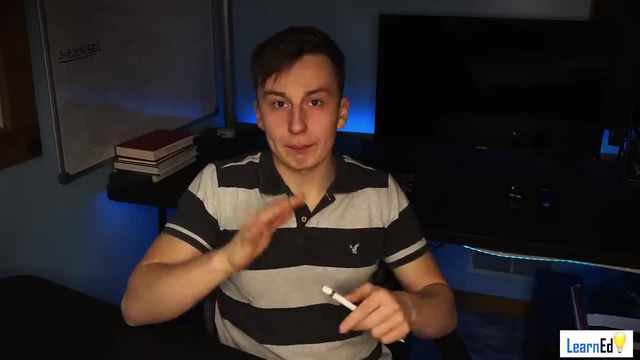 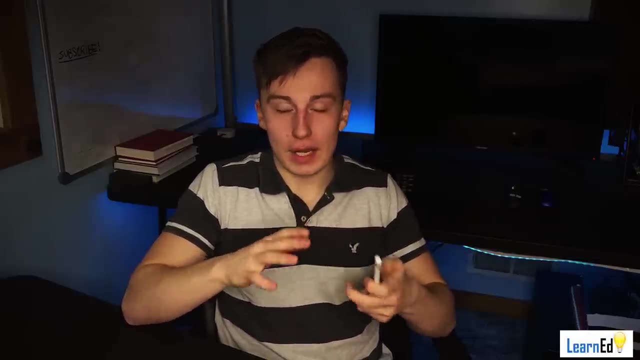 both one to one and on two and, as you may remember from the characterization, characterizations of invertible matrices, we're going to have a linear, independent matrix and we're going to have a linear if it has a pivot. if a standard matrix has a pivot position in every single column, then it is. 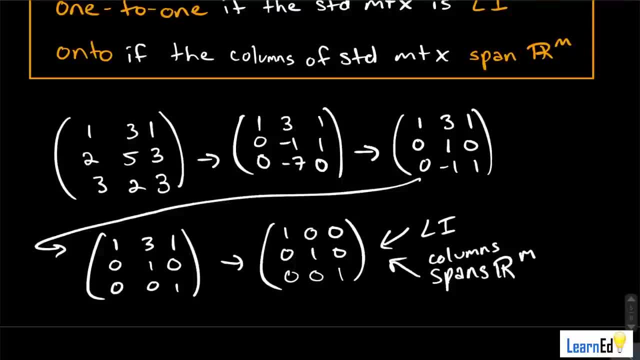 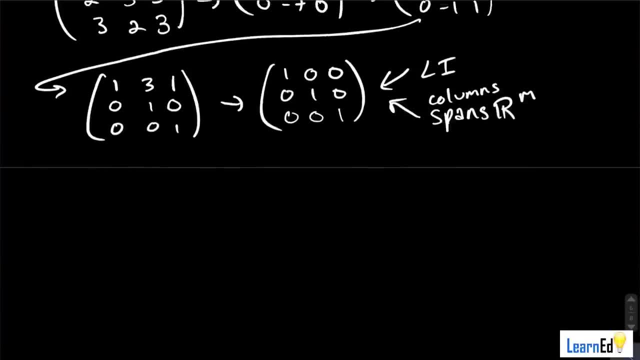 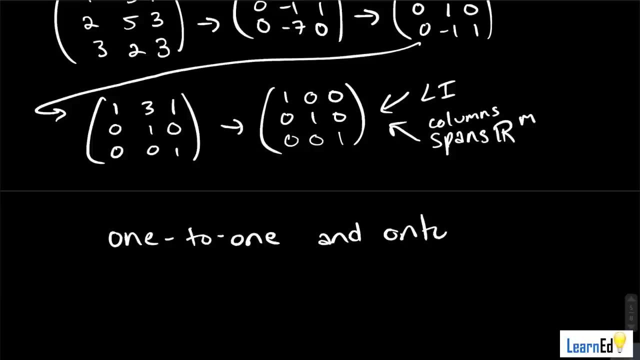 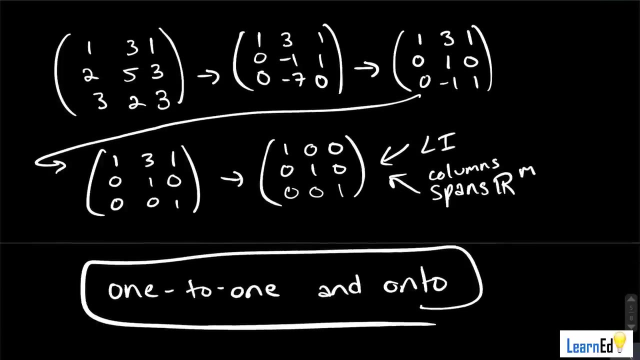 invertible. okay, that's one of the conditions. so that's that, anyways. moving on to and. did I actually write down the answer? uh, no, I didn't. so let's just say one to one and on two. all right now. I mentioned that rc car thing before. okay, that rc car, I guess rc being an acronym, you could use this acronym. and I also mentioned 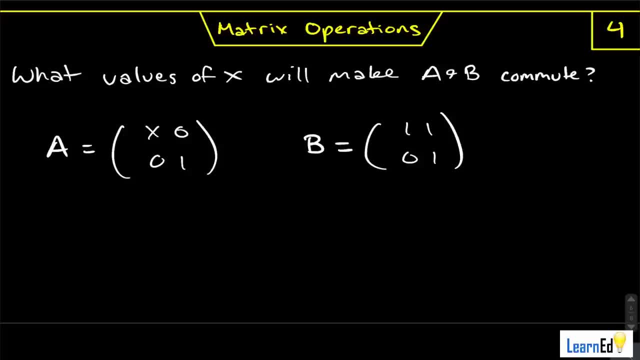 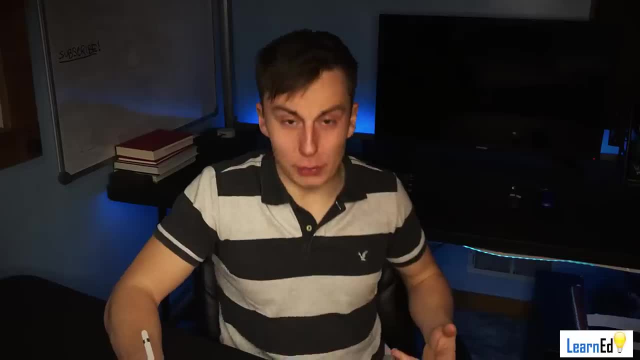 that you could use it in matrix multiplication, and that's exactly what we're going to do for this problem. we're asking what values of x will make a and b commute. now, this problem is going to be relatively impossible if you don't know what that means, what, what the word commute. 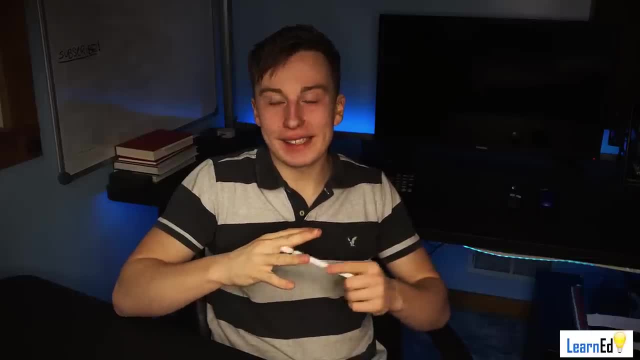 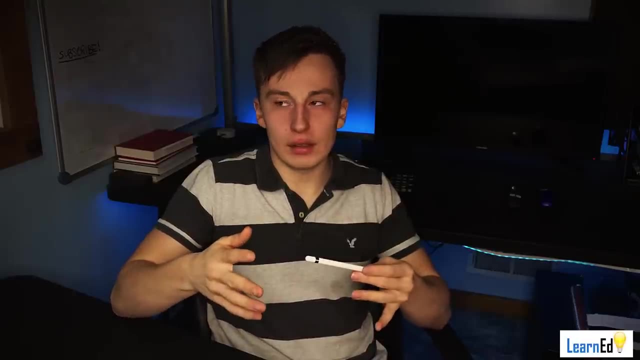 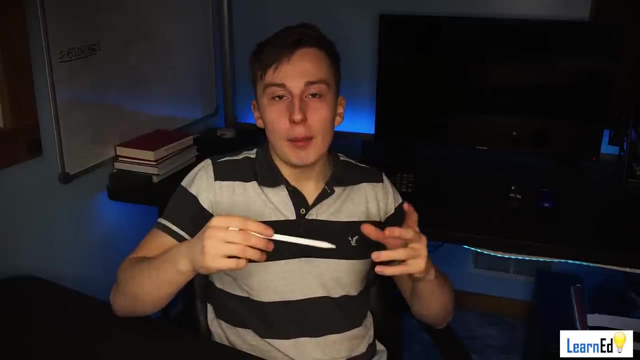 means okay, and you know that's the biggest thing about linear algebra is that they're not necessarily a new term. okay, used in linear algebra fashion, yes, you could say it is, but there's a lot of different terms that get thrown around in linear algebra that you need to keep track of. 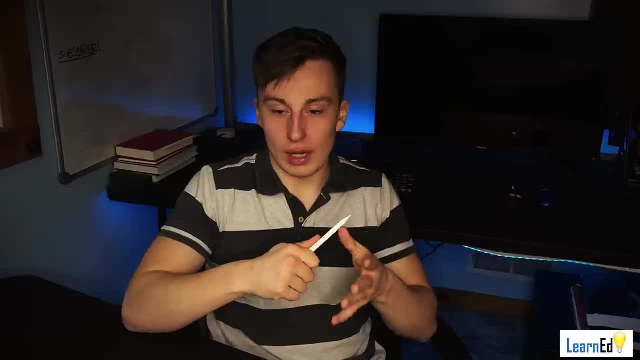 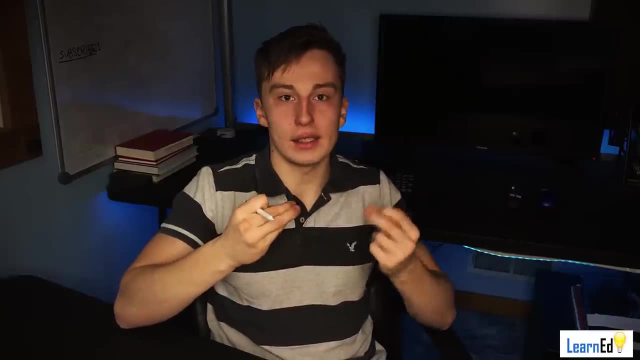 okay, you know you have commute, you have image kernel, you have, you know, vectors, or you have column space and null space and all that stuff and you need to all remember what that is okay. so I'm going to be doing examples of that in a little bit. but I'm going to be doing examples of that in a little bit. 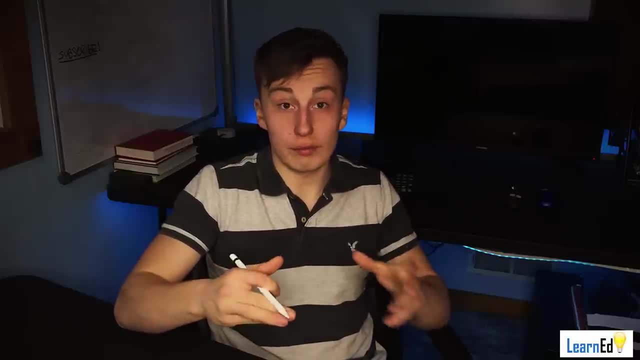 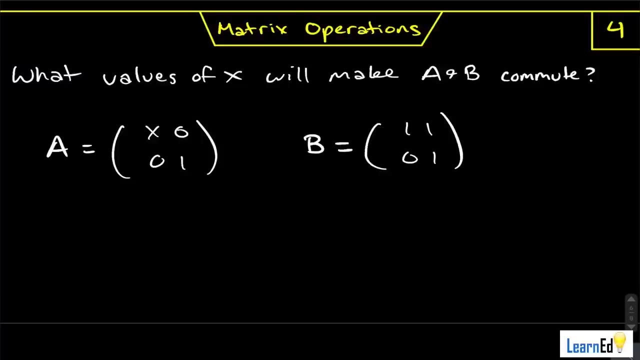 all this stuff just to help you jog your memory on on all of these different terms to all this terminology that gets used in linear algebra. so basically, if a and b commute, that means that a b equals b, a right kind of like the commutative property. okay, that's where this whole thing. 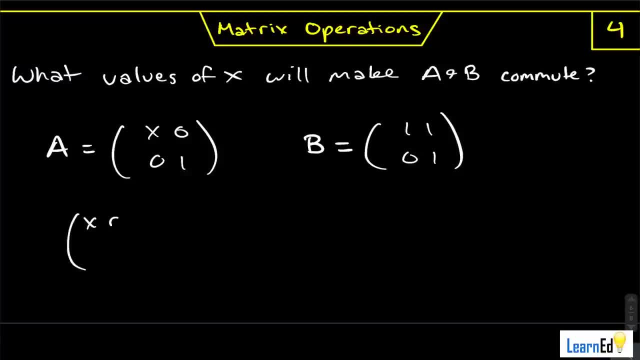 stems from now, what we have to do first- let's multiply a times b, okay- and what we can do first off, what's going to be the dimensions of our resulting matrix. well, this first matrix is a two by two and the second matrix is a two by two: the inners, the inners, the. 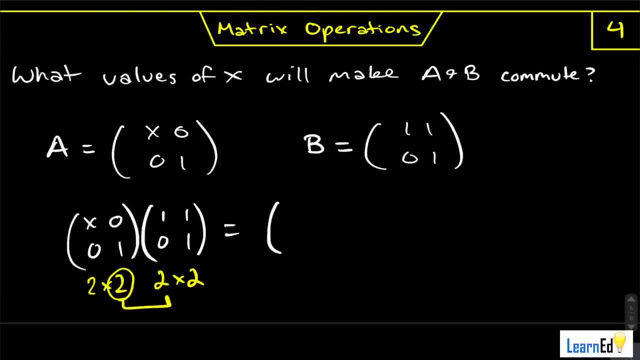 the, the two guys that I just did right here. right this, this and this: they tell you if you can actually perform a matrix multiplication. those two values have to be the same- they are in this case- and the outer numbers, this two and this two, tell you what the dimensions of your final matrix will be. so these, this will be a two by two matrix. 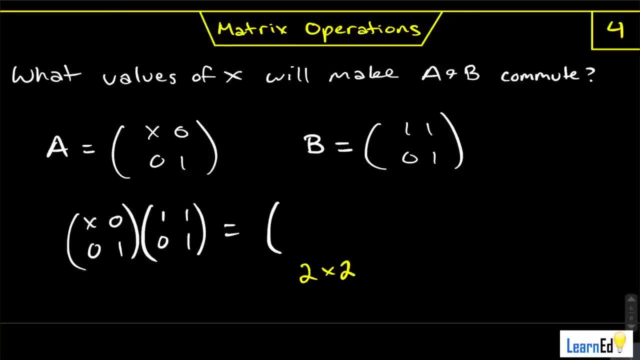 okay, so how do we actually go about multiplying here? well, in where this acronym comes in is in the, the first matrix. you use the row that the entry that you're trying to find is in. okay, we're trying to find the top left entry, so that's in the first row and we're also going to. 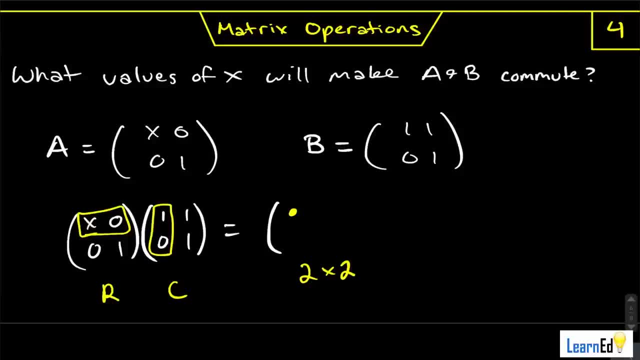 then box the the column that that entry is in. okay, but that's going to be in the second matrix, okay, and what we do is we first section this off in two pieces. okay, and we're going to multiply x times one, all right, and we get x. we'll add that to our second piece. zero times zero, and that's zero. 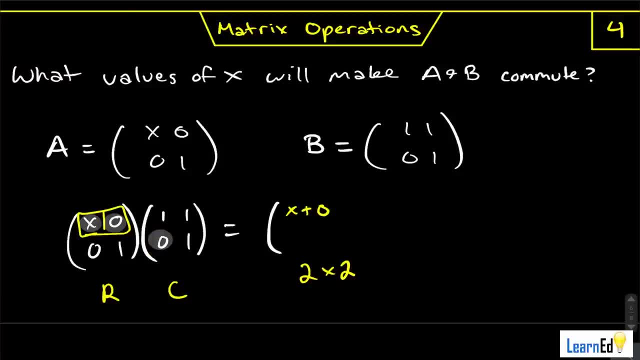 and we're just going to continue doing that for the rest of of our multiplication process. okay, now for our second one. I'll just do these boxes one more time. if we're trying to find this entry, that's in the bottom row and it's also in the first column. so now we have a zero times at. 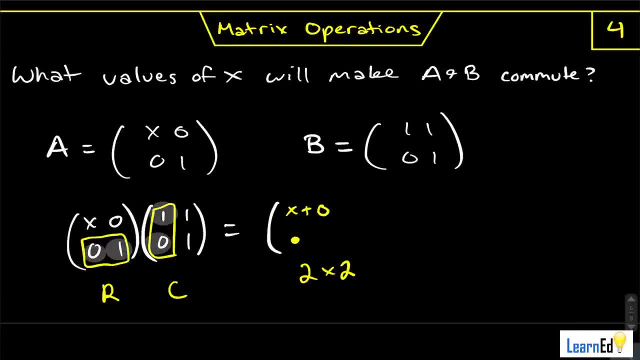 one and then a 1 times a 0, okay. so, as you can see, those are both 0, so we get a 0, okay, and now that should be fairly straightforward, so we'll go through that and then we're going to go through and do the rest of these entries. so, for our top right, we're going to have a X times 1 and a 0 times. 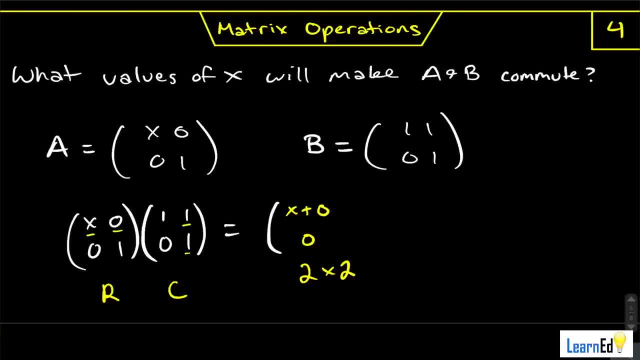 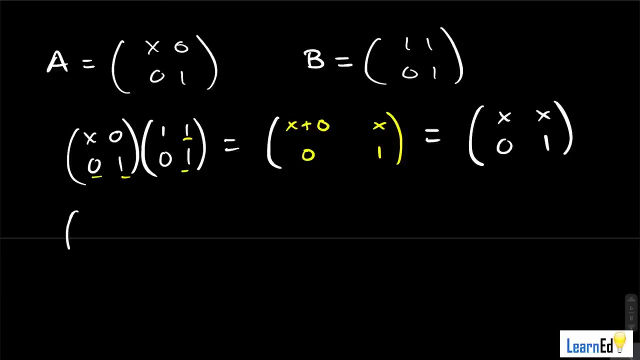 1. so we'll just end up with X and for our final multiplication we're going to have a 0 times 1 and a 1 times 1, so we get 1. okay, now we have to see, and I'll actually rewrite this here: this will be x x 0, 1 and we have to see now. 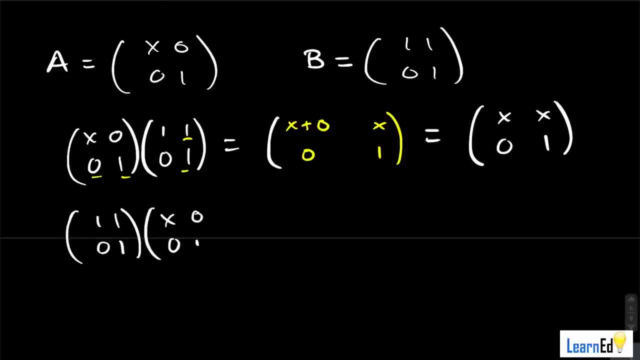 if we're, what, what? all right, let me get my words together here. we have to see, when we switch around these matrices, what will our answer actually be when we multiply these things. so first we're going to have a, we have a 1 times x and a 1 times 0, so we get x here. 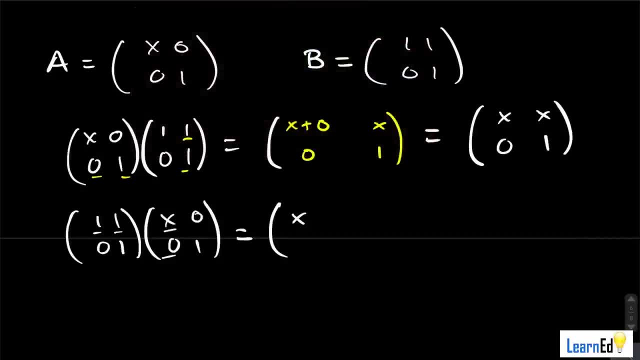 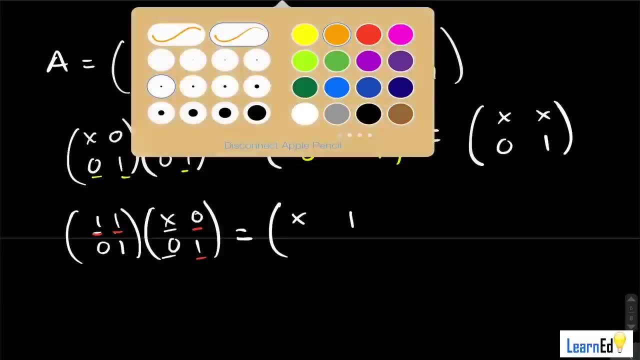 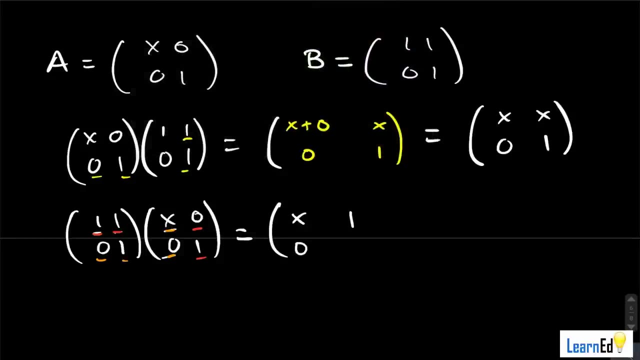 we have a 1 times 0 and a 1 times 1, so we get a 1 here. we have a 0 times X and a 1 times 0, so we get a 0 here. and we have, lastly, 0 times 0 and a 1 times 1, so we get a 1 in the bottom entry. okay, 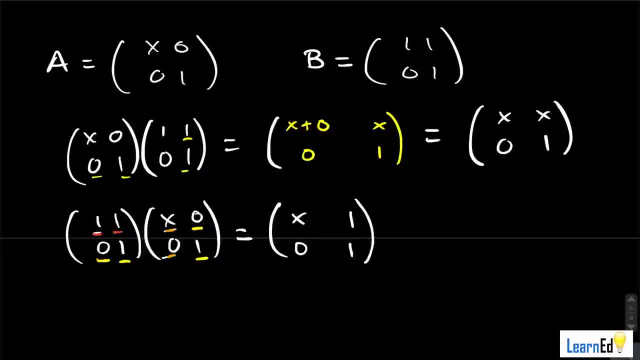 now we can actually finally see what our X's need to be, and you may look at these X values in the top left entry and be like, okay, well, they can be anything. however, the restriction on X comes in where you see the X in the top right entry and the one in the top right entry. so you see. 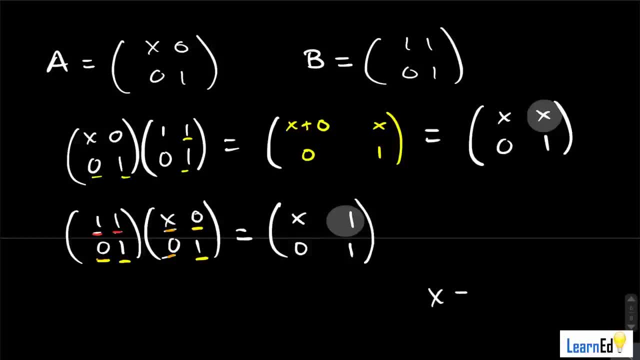 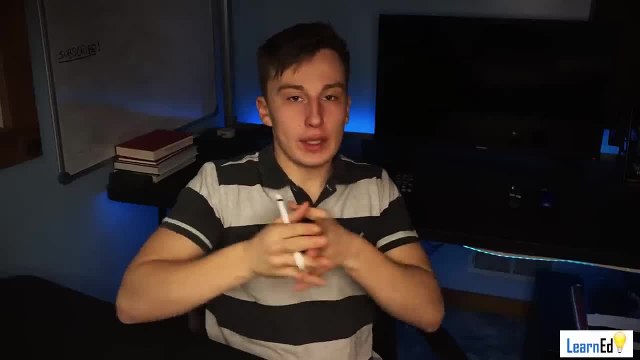 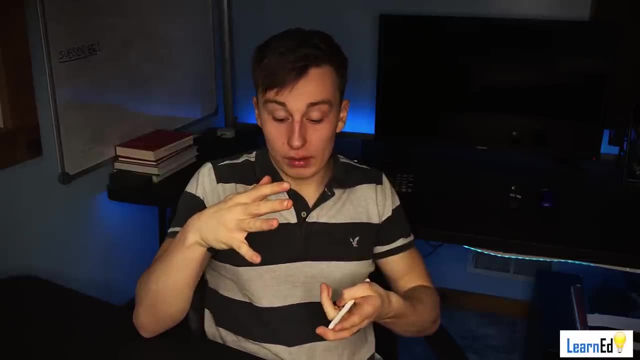 for these matrices to be equal, X needs to equal one, and that's your answer. okay, so while the X is in the top left could be anything. they're restricted by the what the X has to be in the top right. okay. now, if you saw something where you didn't have that restricted X, okay then X. 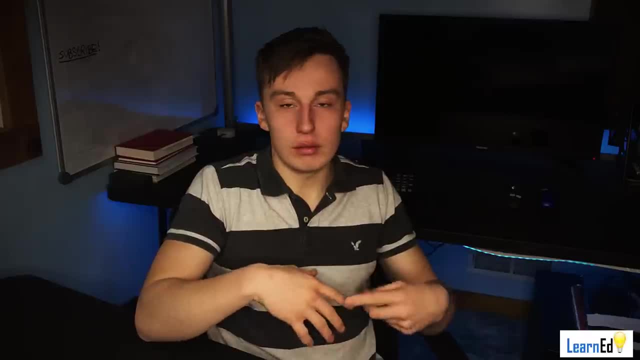 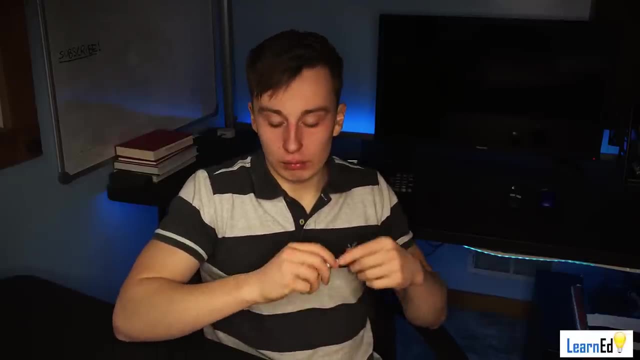 could be anything right. you could pay X as any number and then you would, you know, have have a nice time doing that, but here that X is restricted, and you see what our answer is. so, now that we've talked about linear transformations and we've talked about matrix, 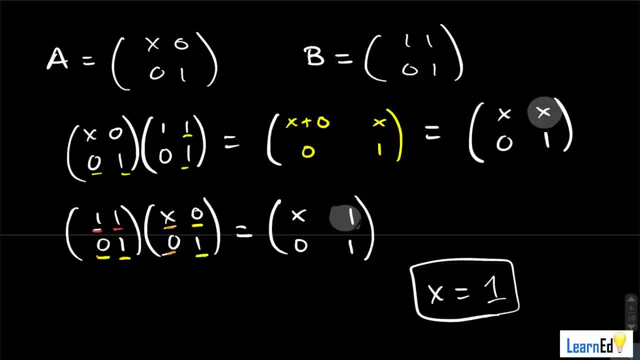 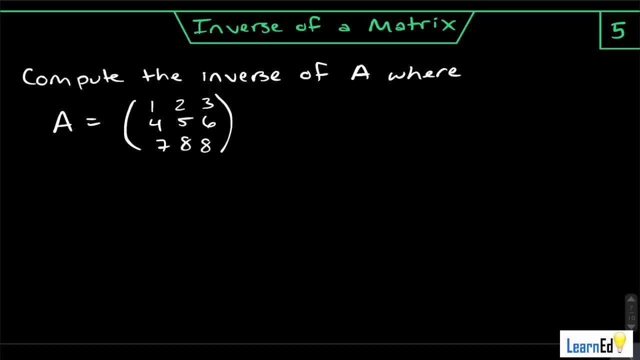 operations, you know, like matrix multiplication. we've done some addition and other stuff in previous examples. now we're going to talk about the inverse of a matrix. okay, and problem five is asking you to convert, compute the inverse of a where a is equal to, and you have your three by 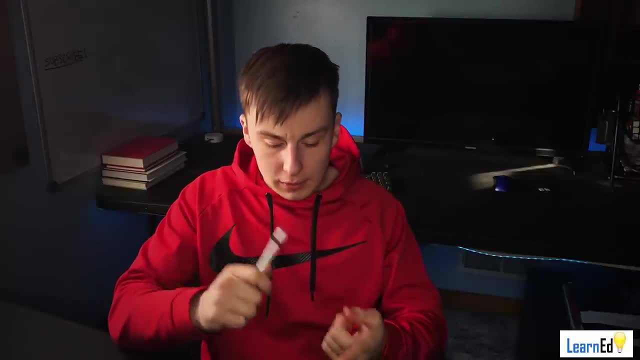 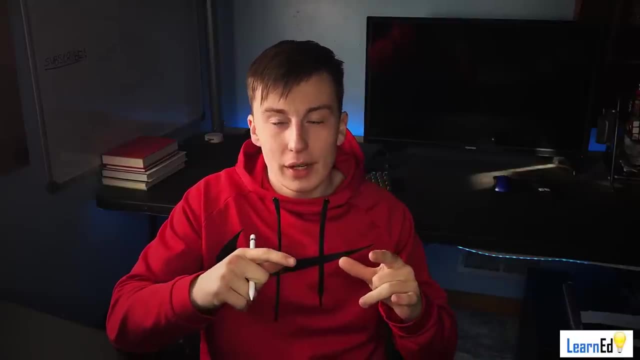 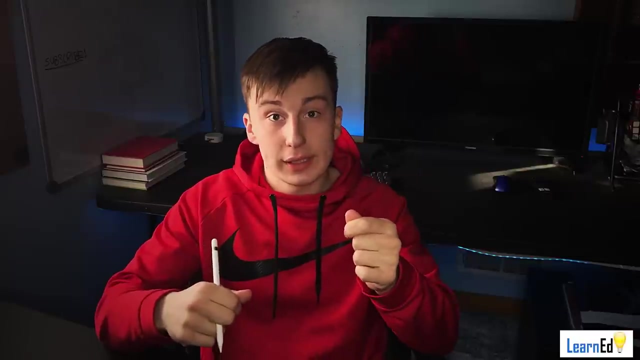 three matrix there. now how do we compute a, the inverse of a three by three matrix? we know how to do it for a two by two right. for a two by two matrix, all you have to do is switch the two X's entries in the main diagonal and then just negate the entries in the reverse diagonal right. but how? 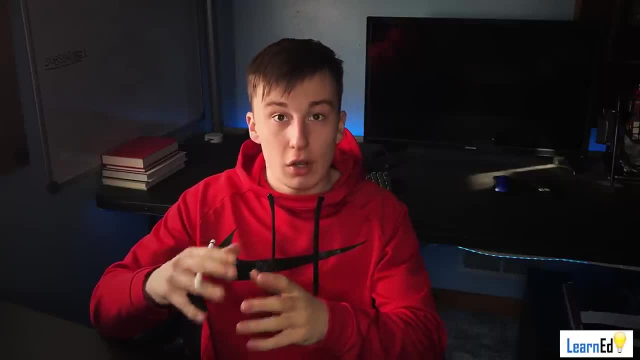 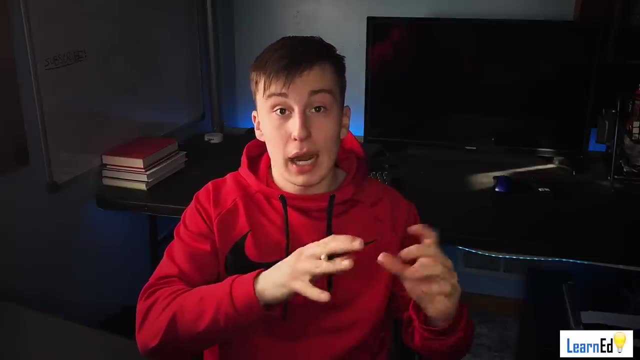 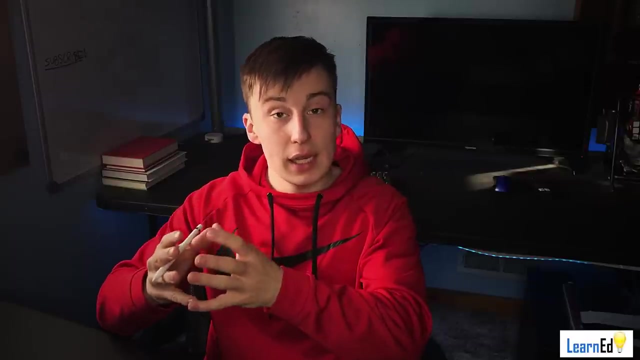 are you going to compute the inverse for a three by three? all we have to do is augment this three by three with the identity matrix. for a three by three, right, I, three, and then we're going to row reduce and once we have the identity matrix on the left side, instead, our augmented side will show. 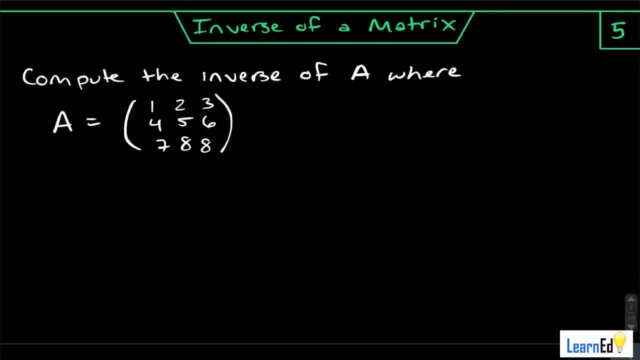 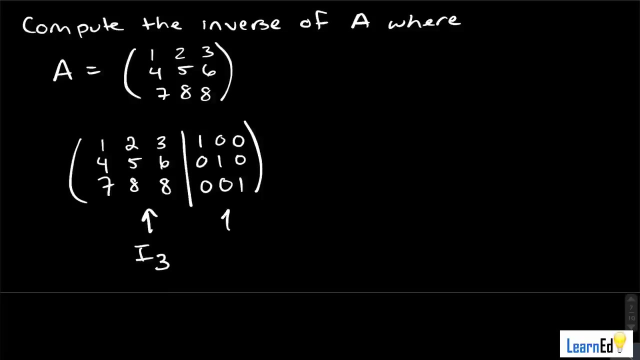 what a inverse actually is right. so what we're going to do is set up our a and we augment it with the identity matrix. okay, now what's going to happen is we get the identity matrix on this side when we row reduce and this side will be a a to the negative one. negative one will be up there, okay, so. 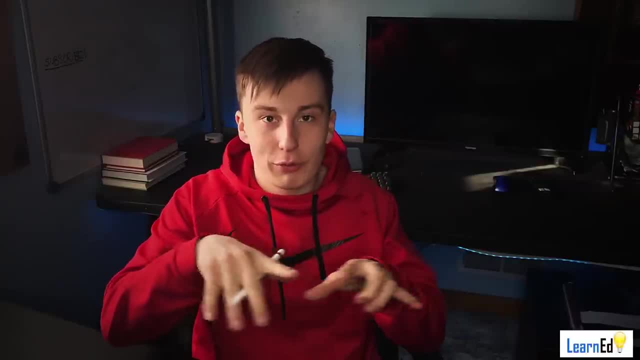 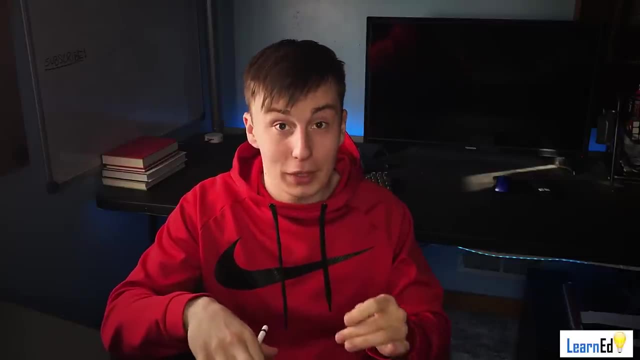 and, by the way, I know that these numbers you know- one, two, three, four, five, six- but it will not be that easy to reproduce, right? this is actually going to be probably a hardest row reduction example, and I think it's good to have one of these where you're going to have, you know. 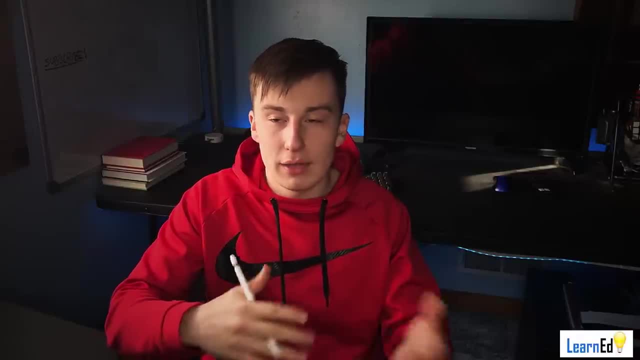 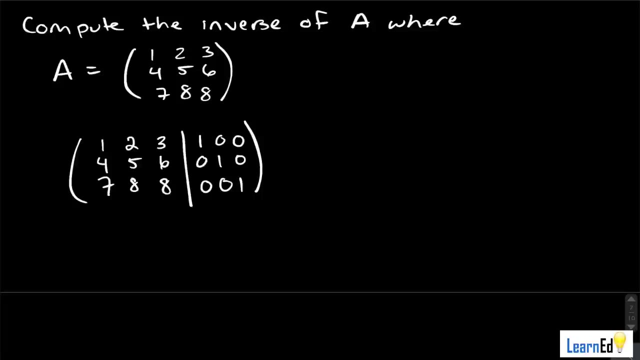 some fractions and stuff like that, just so you are practiced with that, even though it's not really that big of a step. but anyways, let's get into this, and the first thing that we're going to be doing is, like always, we're going to zero out the two entries below our first pivot. okay, so we get one, two, three. we have one zero, zero. 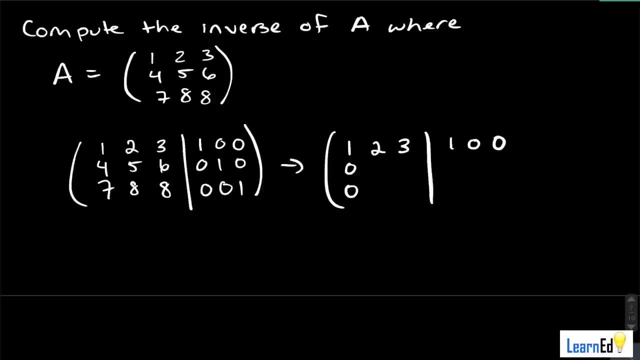 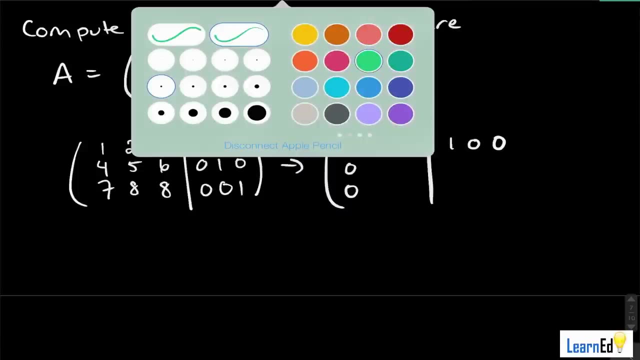 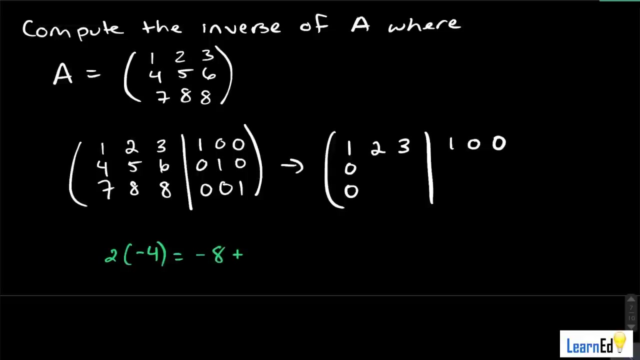 and then what will be our entry here? well, to zero out this thing right here, we need to multiply by the first row by negative four and add to our second row. so if we multiply two by negative four, okay, two times negative four is going to be negative. eight plus five is negative 13.. or not? no, it's not, it's negative three. 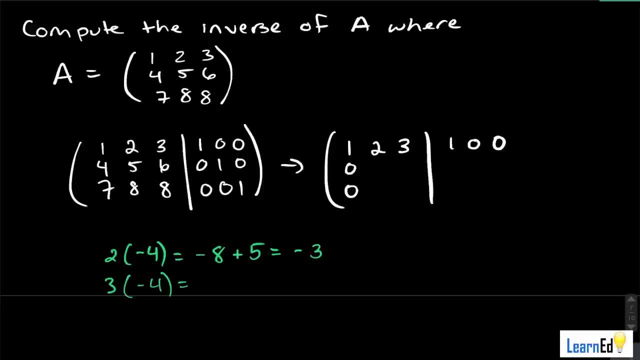 okay. and then we have a three times negative four, which gives us a negative 12, and that plus six is negative six. okay, so we can fill those in negative three and negative six. now we also have to deal with this, this one affecting this entry here. so one times negative four equals. 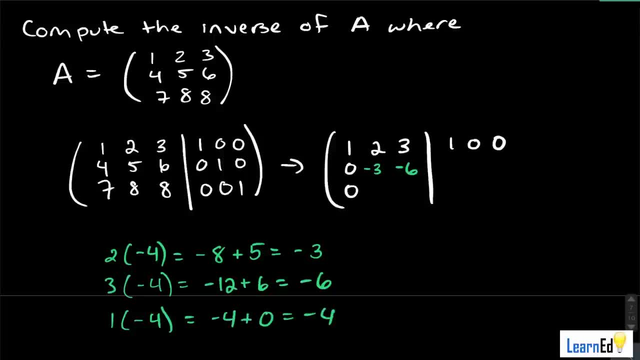 negative four plus zero equals negative four, so we get that there, and then we have a one zero. and then, lastly, we have to do our third row, and so we're going to have to get a zero there. we're gonna have to multiply by negative seven and add, so we get a two times negative. seven is negative 14. 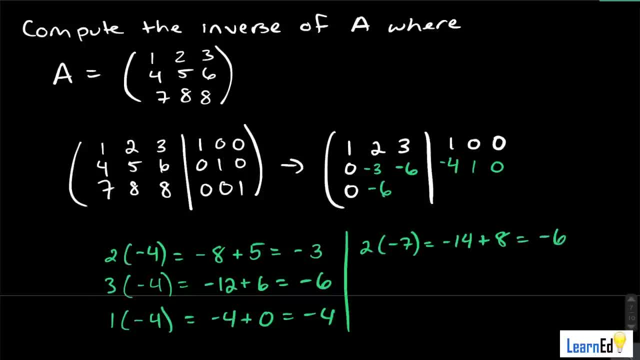 is negative 6. we have a 3 times negative. 7 is negative. 21 plus 8 is negative. this is negative 13. and then we have a 1 times negative. 7 is negative. 7 plus 8 is going to be 1, so this will. 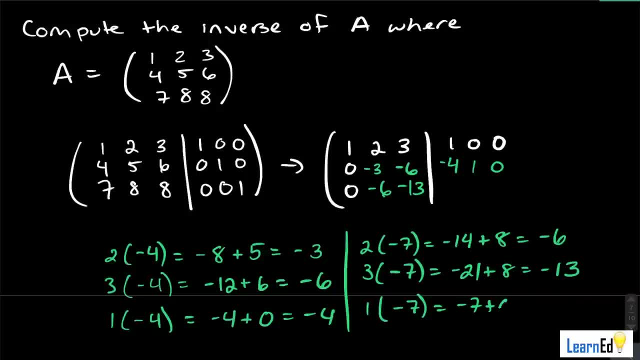 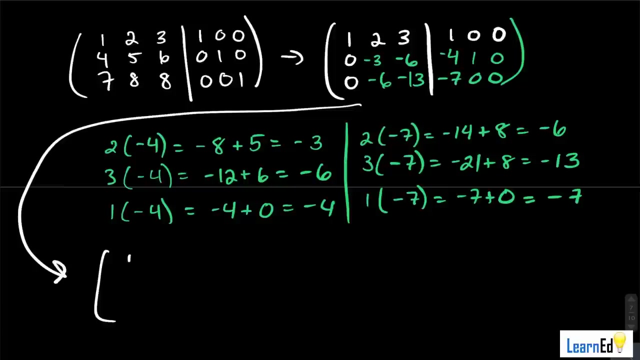 or sorry, not plus 8, plus 0, because there's a 0. there was previously a 0 there. I'm thinking about this entry, but no, so we're going to get a negative 7 over here. okay, so there's everything that we changed in green. so now let's bring this matrix down, okay, and let's keep going. so we have. 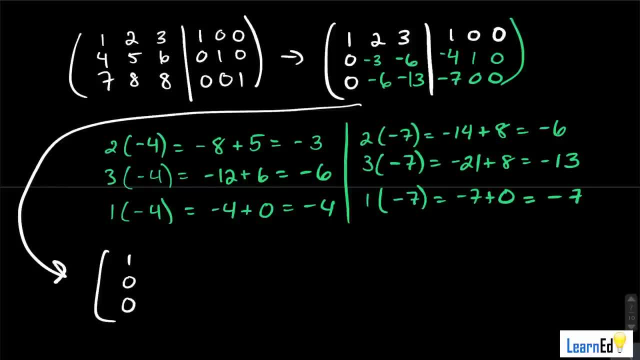 our first column pretty much figured out. the next thing I want to do is get this entry right here zeroed out. okay, so to do that we have to just multiply by negative 2 on the second row and then add to the third row. okay, so we got to figure out. 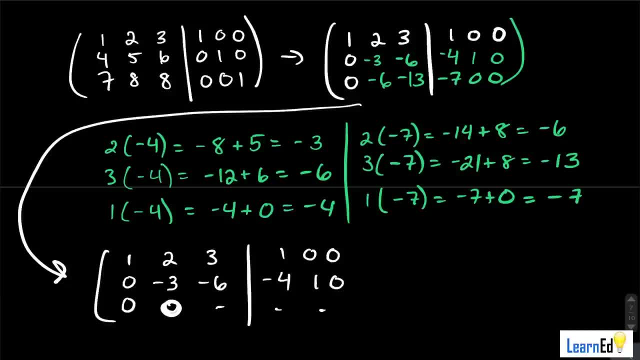 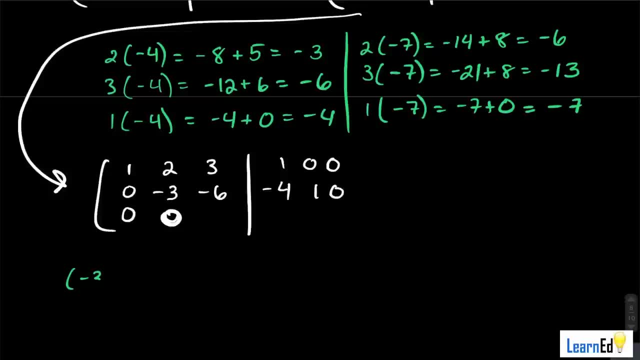 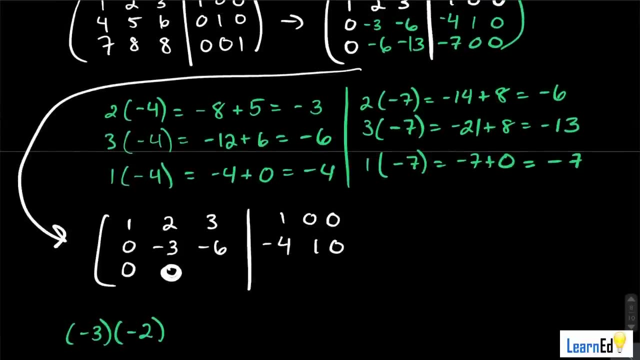 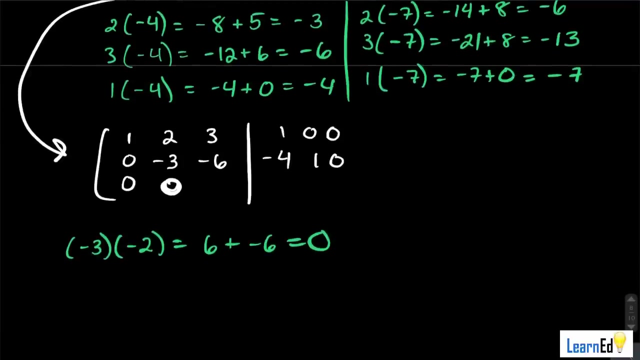 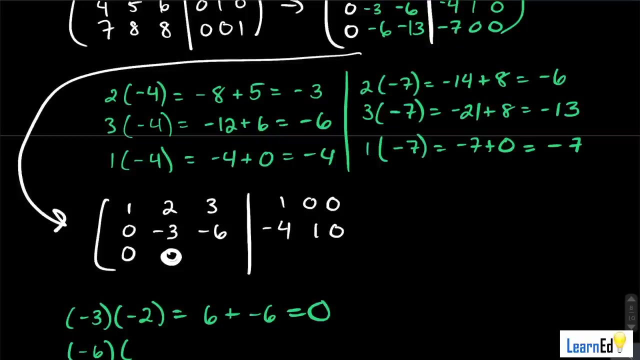 what these four entries will be right here. okay, so we're going to get, like I said, we have to multiply by the second row, by negative 2 to get. this will be 6, and then if we added to negative 6, we get zero, so that that does make sense. then what we'll do is we have a negative 6, we have to multiply that. 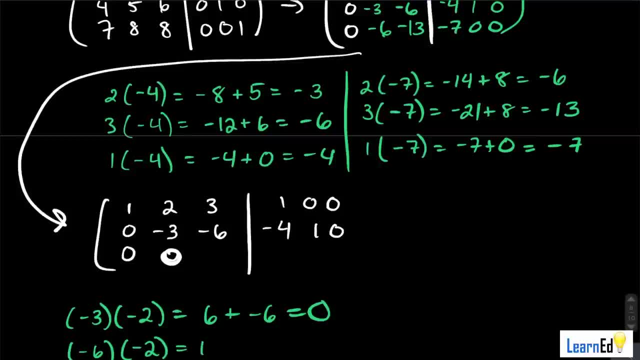 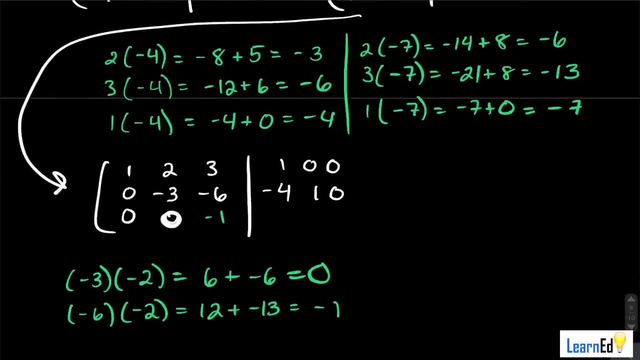 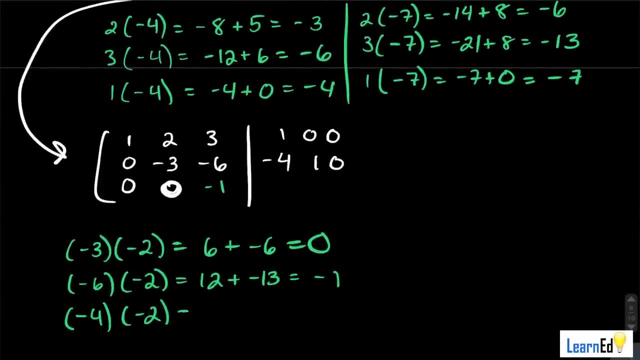 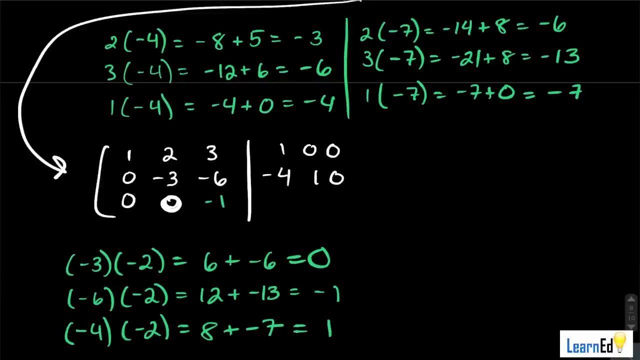 by negative 2 and we get a 12. we'll add that on to negative 13, get a negative 1. so negative 1 goes here. then we have a negative 4. multiply that by negative 2, we get 8. we're going to add that on to negative 7 and get 1, and then we have a 1 multiply. 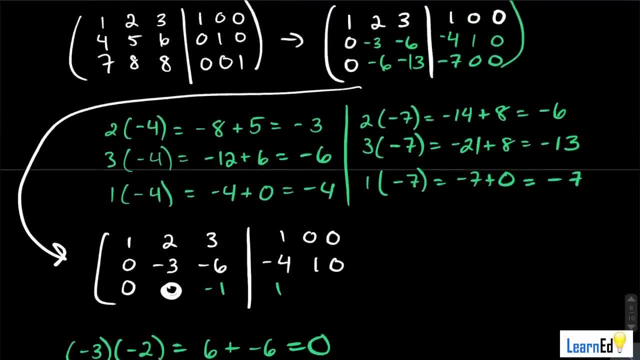 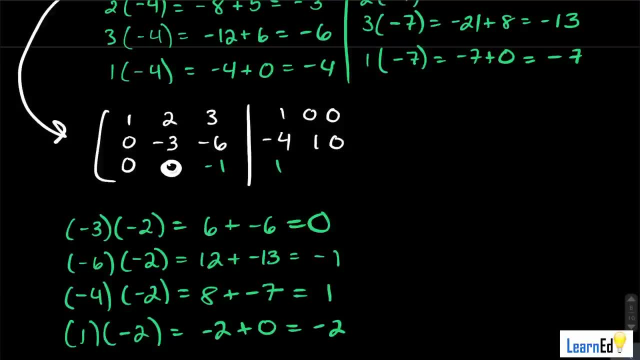 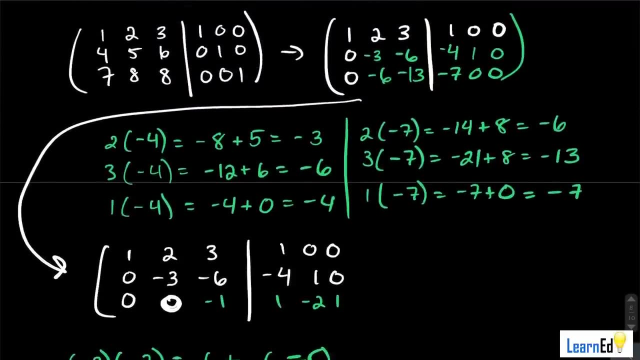 that by negative 2, get negative 2, and we're going to add that to 0 and get negative 2, so we'll have a, a negative 2 here, and then this entry will remain unchanged, because- and did I? yeah, I zeroed that out by accident, sorry guys. 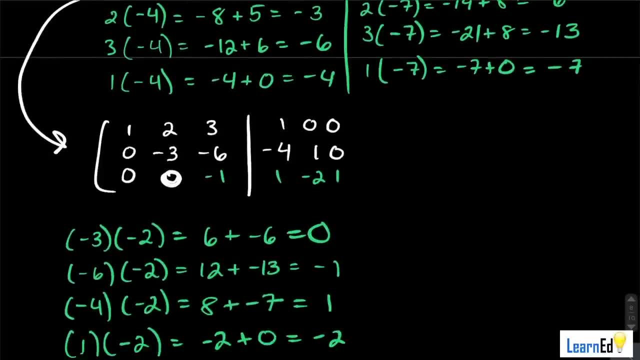 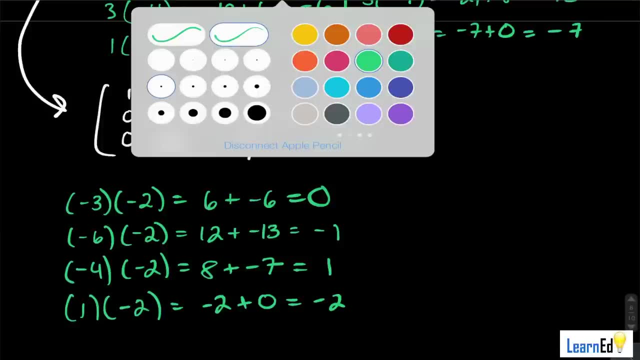 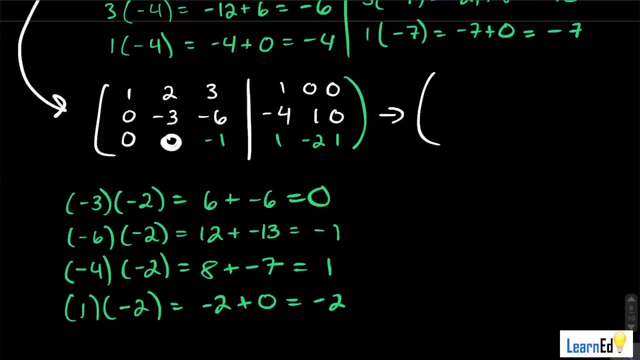 that's going to be a 1. so there you go, so that that's going to stay as a 1, because this entry zero, not there's going to be no effect. okay, so moving on, we can, Since we have now this matrix in row, echelon form right. 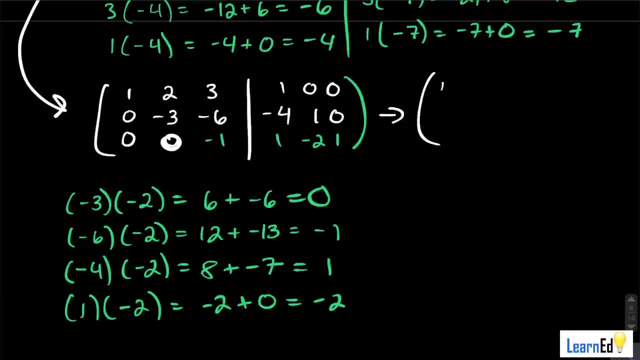 We have this kind of upper triangular look. What we're going to do is start zeroing out the tops, the top above our pivots. Okay, so I'll try to write down everything that's going to stay the same. We're going to have this piece stay the same. 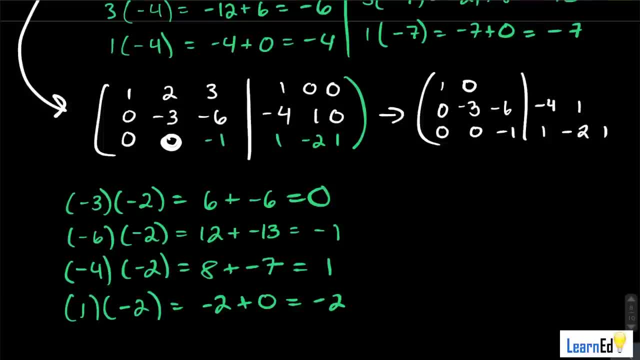 Our second row will stay the same, And our first row is the only thing that's going to be changing. Okay, so what piece is going to go here? Well, to get this thing zeroed out, here's where the fractions are going to come in. 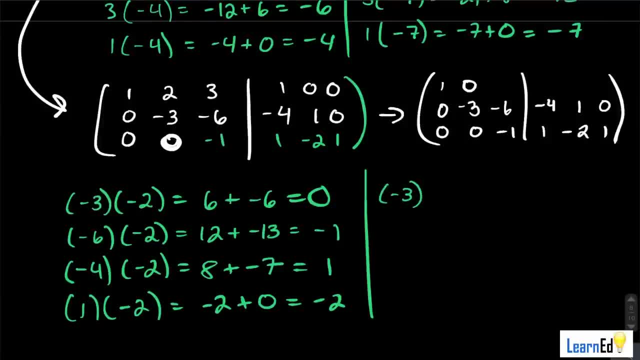 Because we would have to multiply, we'll do row 2, right, Because row 3 won't be of any use here. So we multiply row 2 by 2 thirds, And that gets us to row 2.. And that gets us to row 2.. 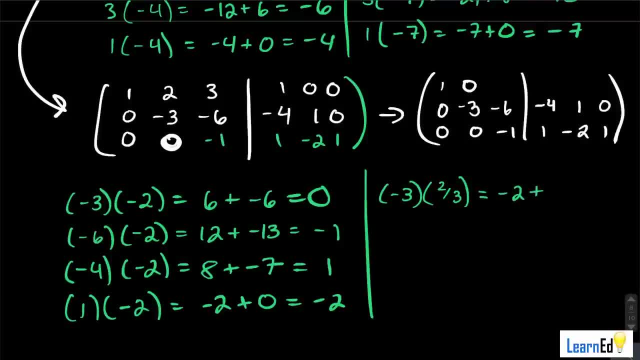 And that gives us negative 2. We add that on to 2, and we get 0. So our multiplying factor is 2 thirds. Next we're going to do that with negative 6. Multiply that by 2 thirds. 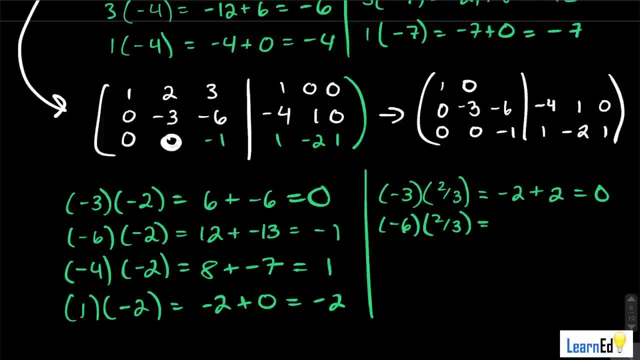 And we're going to get a. We'll get a negative, We'll get a. Why can't I figure this out? This is going to be a 4, negative 4.. Okay, and then we add that on To 3, and we get negative 1.. 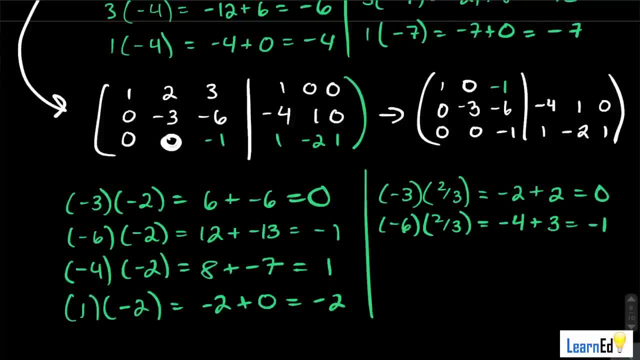 So we'll have a negative 1 right here. Alright, awesome. We have a negative 4 times 2 thirds, Which gives you a negative 8 over 3. And we add that on to the 1 that is there And we get a negative 5 thirds. 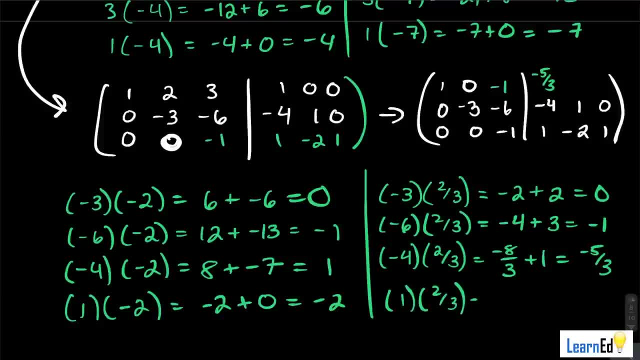 We will have a 1 times 2 thirds And that will give us 2 thirds, And then we add A 1. Or sorry, we add 2. 0, and get 2 thirds off of that. So now we have 2 thirds and then this will stay as a 0. 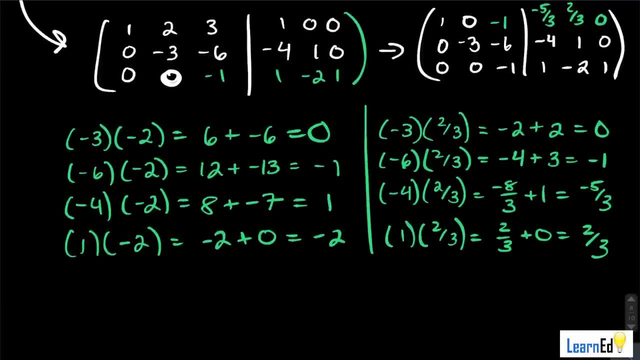 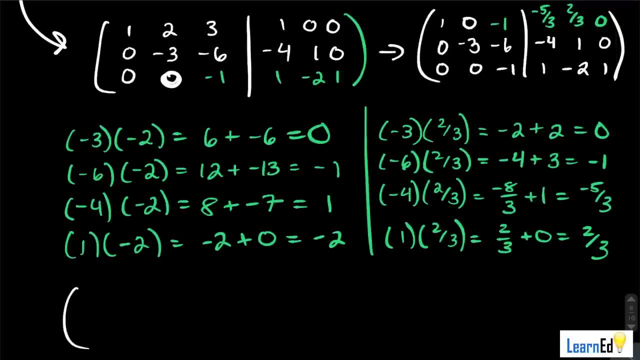 Alright, So now we can actually Get our. Since we now have our second column done, we can get our third column done, And then all we have to do is scale and we'll be set with this problem. So, last step: we're going to zero out these two things right here. 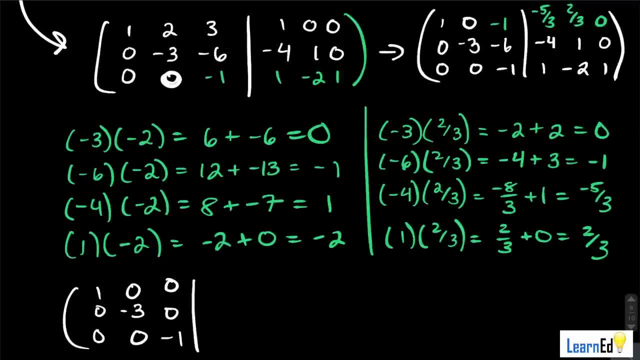 And so we know that our bottom row will stay as 1, negative: 2, 1.. Okay, and to get our second column to be zeroed out in the Or to get our third column to be zeroed out in the second entry, we have to multiply the third row. 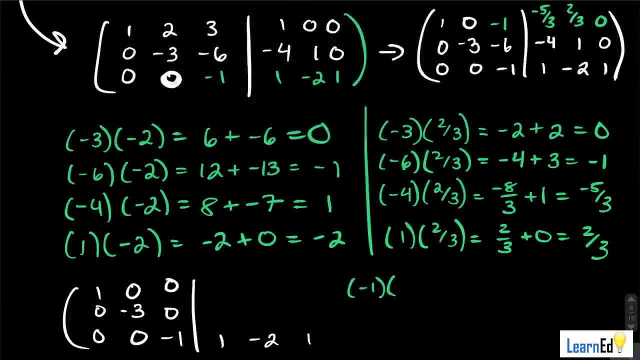 Okay, Third row. so negative 1, times negative 6. And that will give us 6.. We'll add that to negative 6. And we will get 0.. Okay, Now we can do that for 1.. 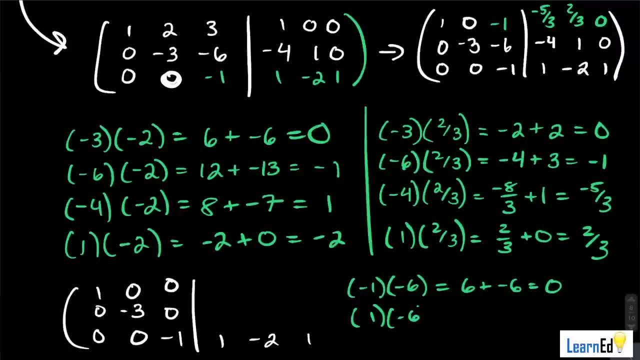 We can do that for this 1 right here. Multiply it by negative 6.. Get negative 6.. Add it on to negative 4.. And get negative 10.. So a negative 10 goes here. We can do that for negative 2.. 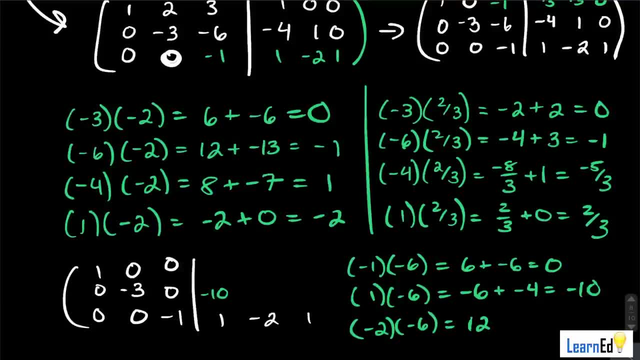 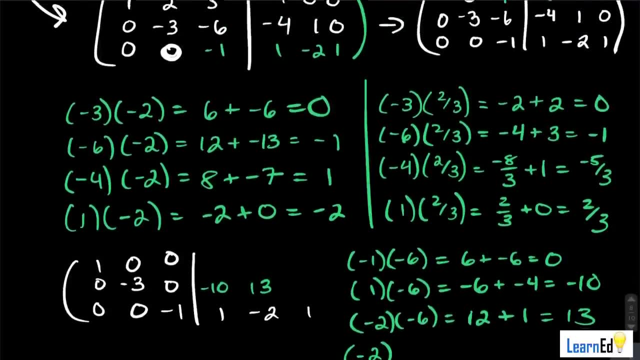 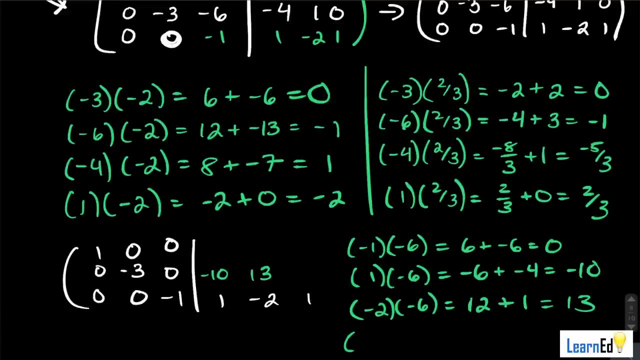 Get 12.. And then we can add on to the 1 that was there and get 13. And we can do that for Multiply negative, Not negative 2.. We'll multiply 1 by negative 6, again Negative 6.. 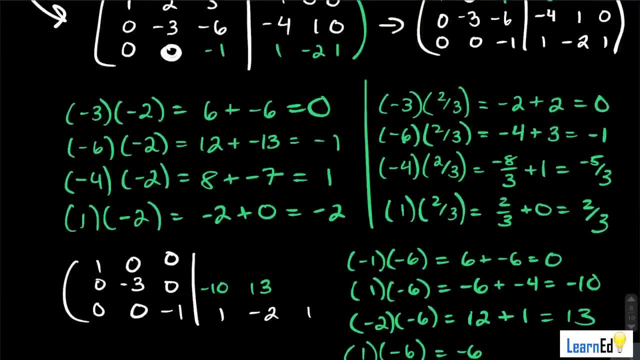 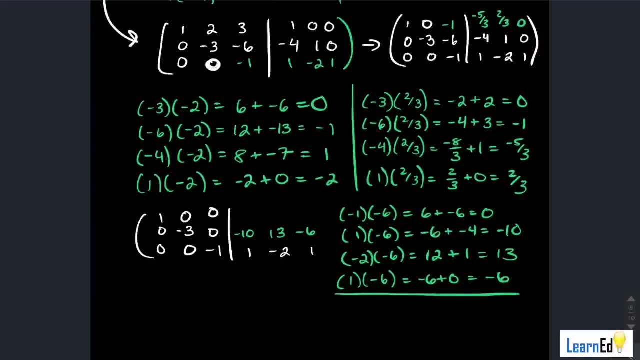 And Then this time we're adding on to a 0.. So we just end up with negative 6.. Okay, So the last thing that we have to do is get our first row in check, And well, all we have to do- we can look over here to get this negative 1 that I'm highlighting right now zeroed out. 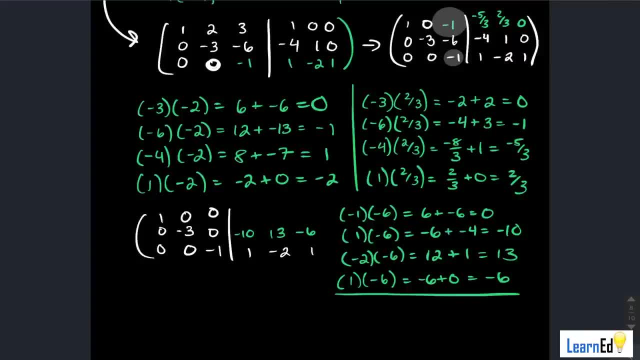 So we would have to multiply the negative 1 on the bottom by negative 1 and then add Okay. So we multiply row 3. By negative 1. We get a 1. And then we add it to the position in row 1.. 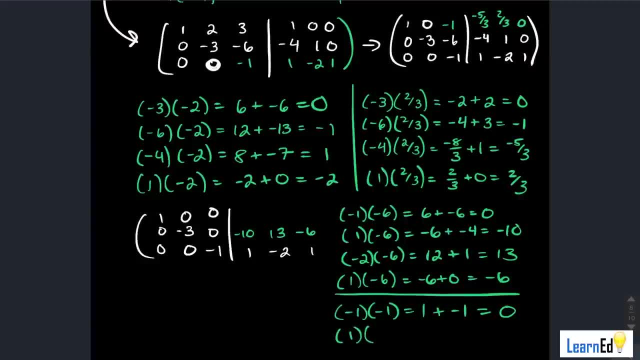 And get 0.. So we're going to do that for all entries in row 3.. If we do it with 1, we get a negative 1 when we multiply And we subtract 5 thirds and get negative 8 thirds. 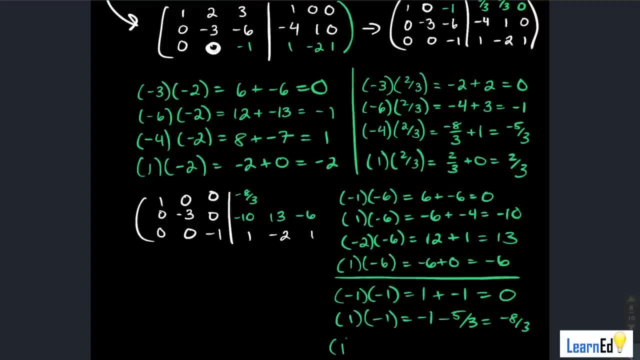 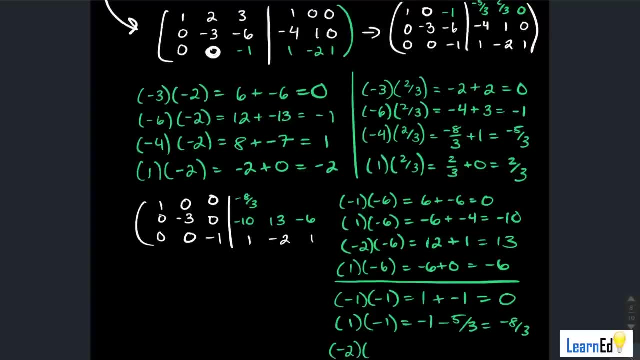 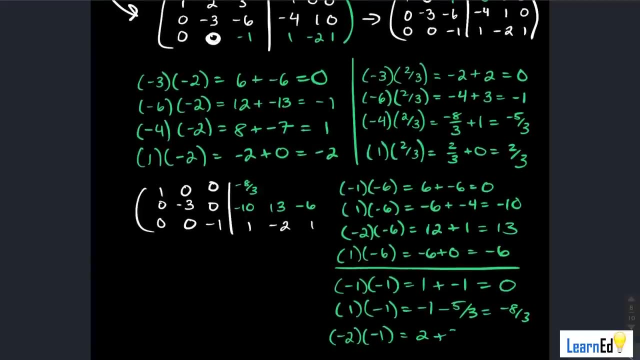 Next we can do that. Next we can do that. Next we can do that with a negative 2.. And we multiply that by negative 1 and get 2.. We add on 2 thirds and we get 8 thirds. 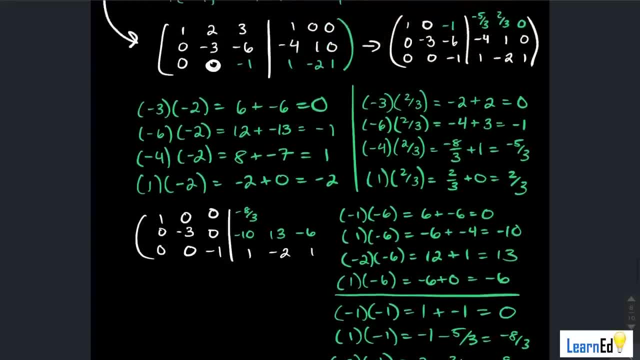 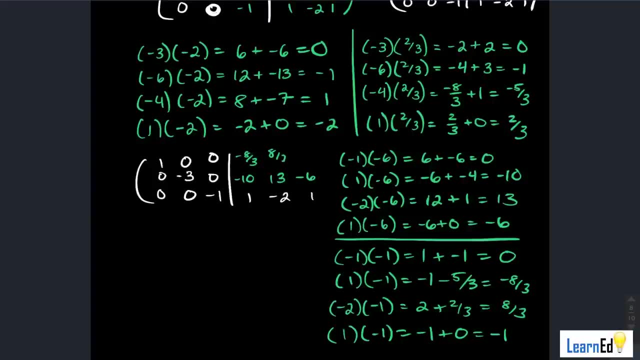 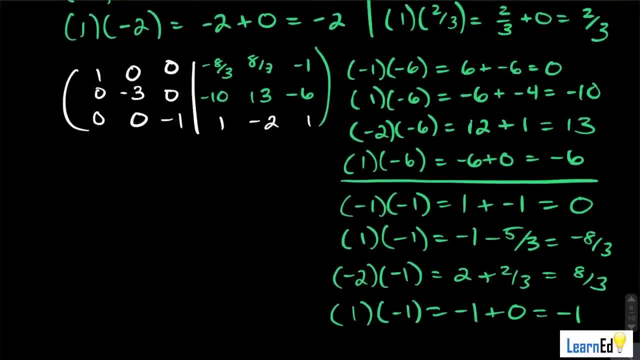 And then we're going to do that with 1. And we get negative 1.. We add that on to 0 and we get negative 1.. So we have 8 thirds And negative 1.. Okay, So almost done here. 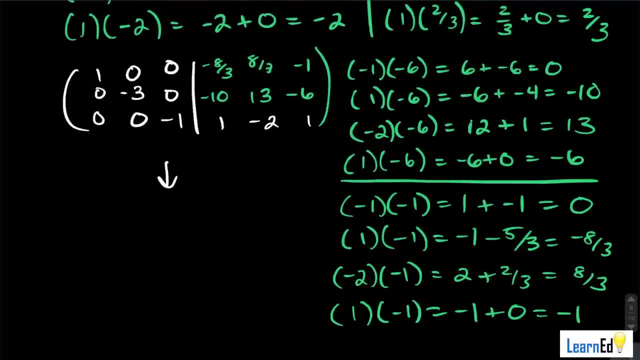 All we have to do now is just scale the rows. Row 1 is fine, So that will be your answer there. Row 2 needs to be scaled by a negative 1 third, So we'll get a 10 thirds here. 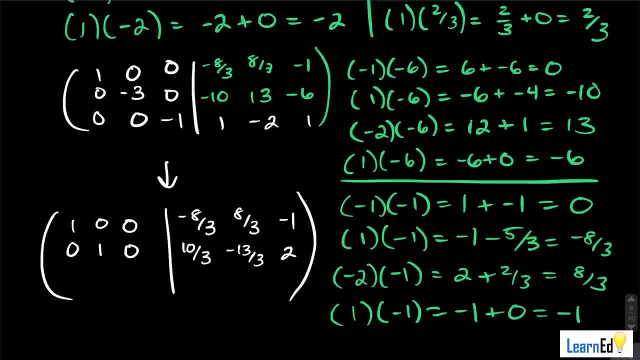 We will get a negative 13 thirds here And we'll get a 2. then in our third row we'll get a zero, zero one. so we have to scale by negative one, and then we get a negative one, two negative one. all right, so that is going to be a inverse and you're going to 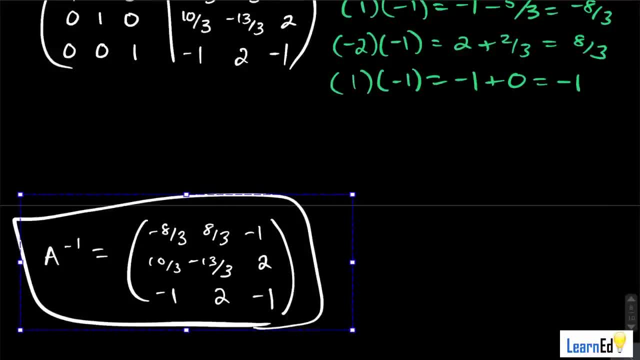 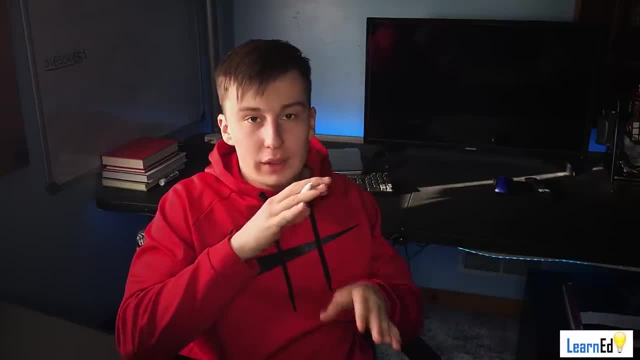 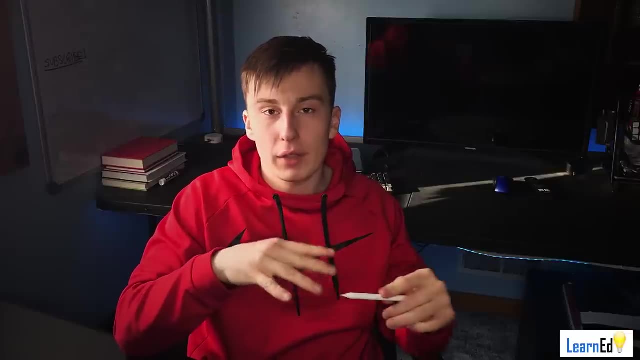 get that right here. okay, so that is your a inverse, all right. so you know it is definitely a lengthy problem, especially when you have a matrix that's really gross to row reduce. i don't know how many of those you'll actually have in your final, because you know, i know, that most professors are. 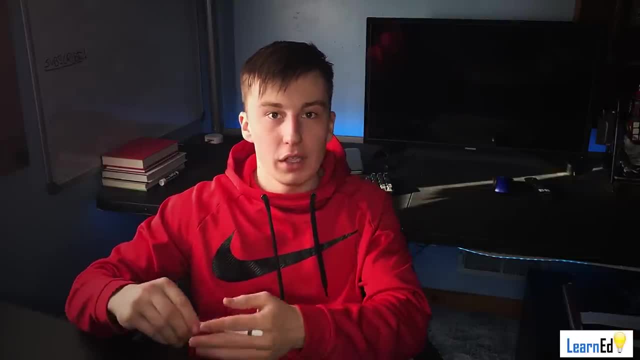 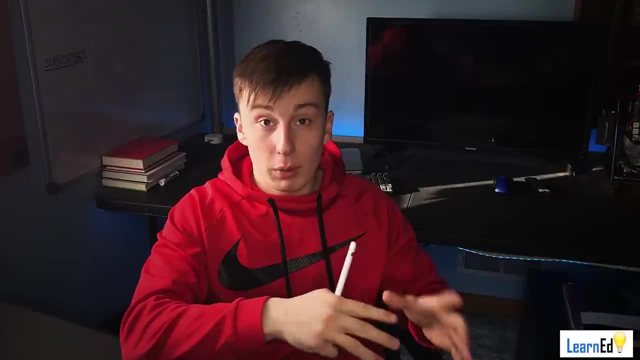 going to want you to focus on the important stuff. you know row reduction is important, but you have to do it for pretty much every single topic in linear algebra. so i don't think they're going to have you focus on row reduction as much as they're going to have you focus on 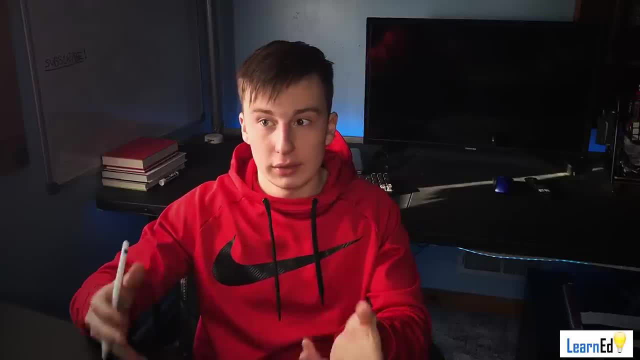 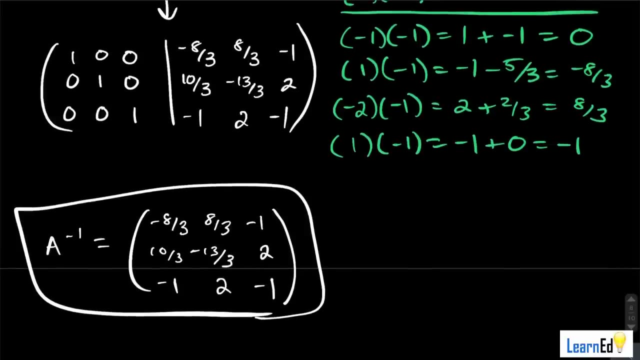 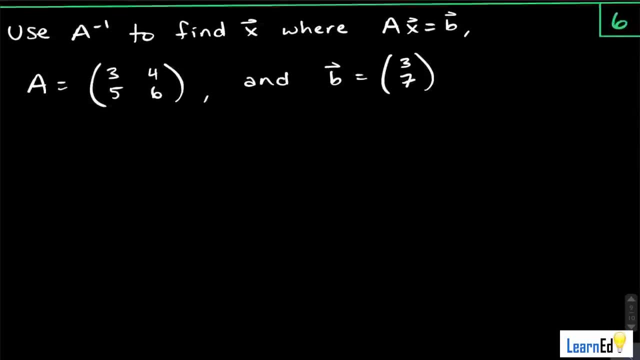 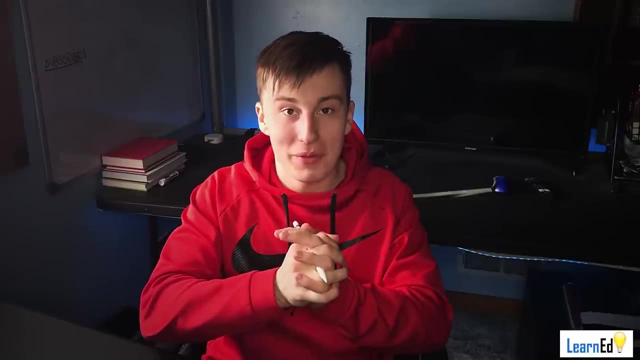 them better than me. so, moving on to number six, and number six is asking us to use a inverse to find x, where a x equals b. okay, now for this problem. this is going to be impossible if you don't know where to even start. right, and i think that might be the hardest part of this problem is just 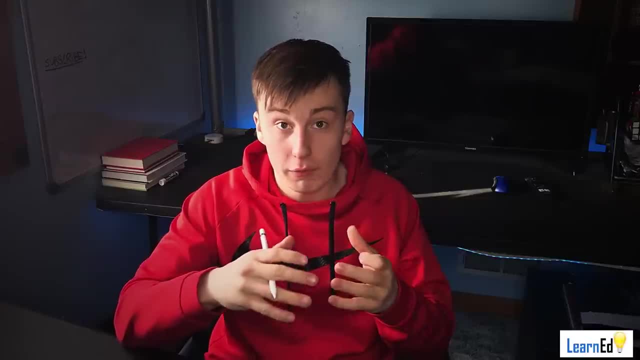 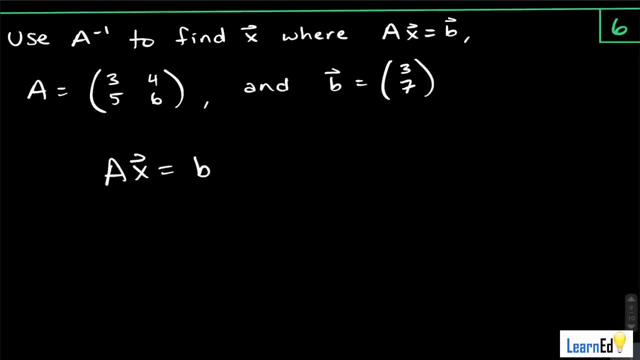 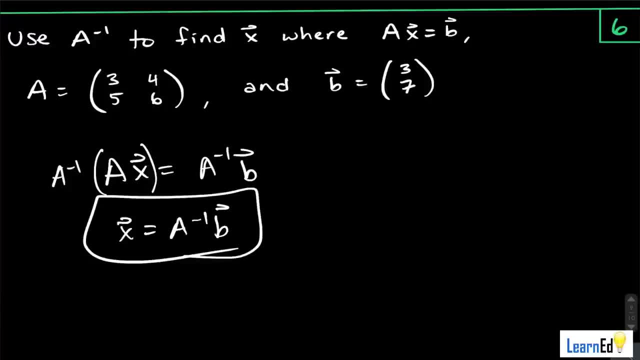 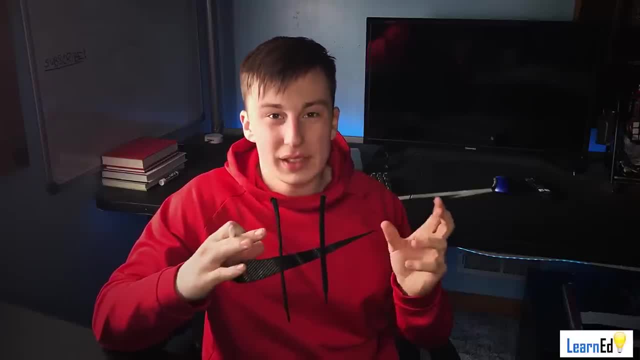 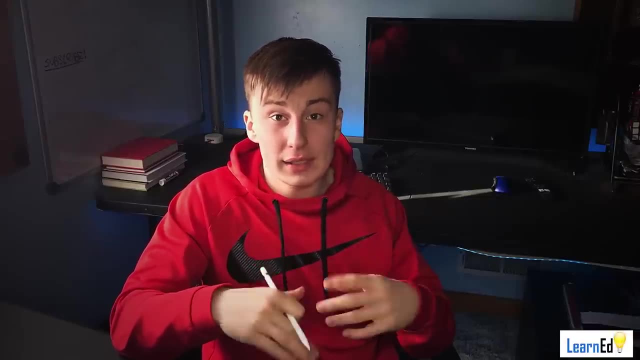 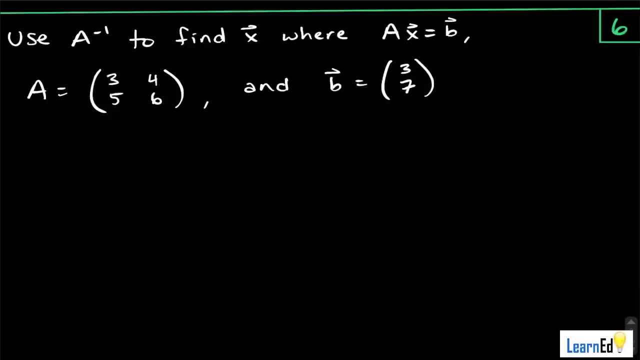 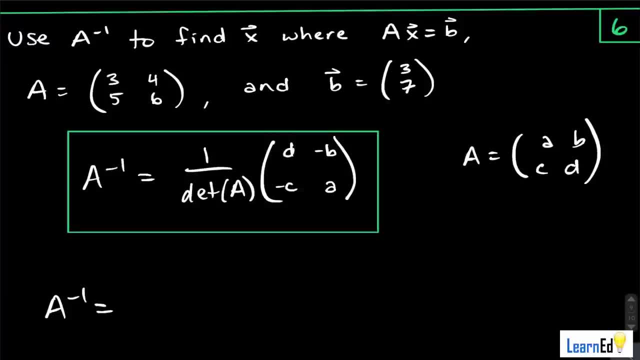 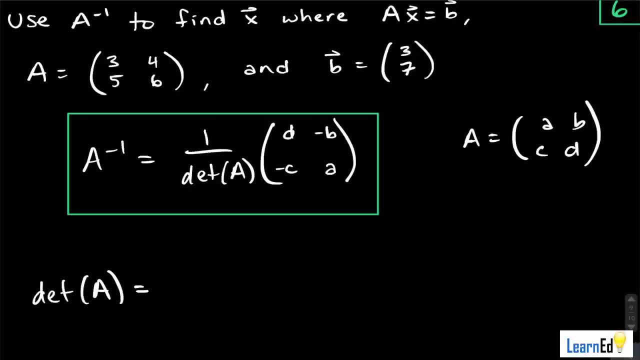 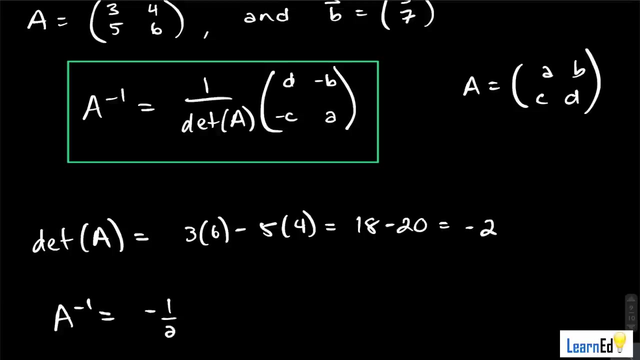 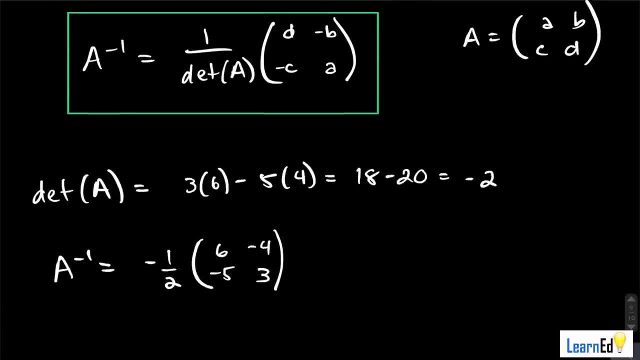 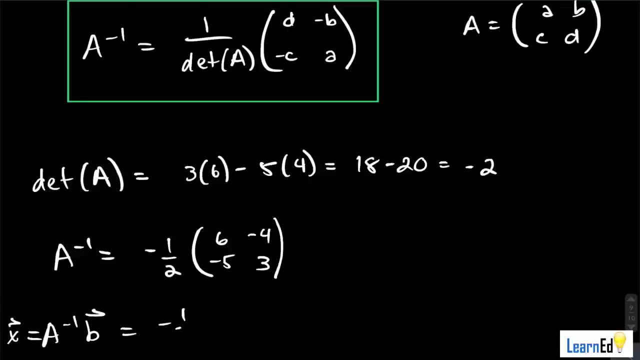 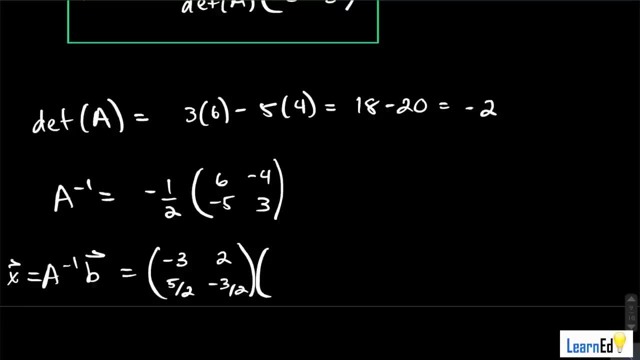 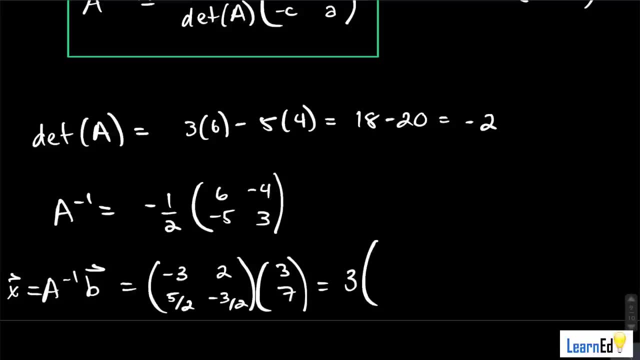 afterwards and actually maybe that would have been a little bit easier. anyways, we can multiply by our B vector now, which is 3- 7, and then we get a 3 times negative- 3, 5 halves, plus a 7: 2 negative 3 halves. okay, so we get equals and we get a. 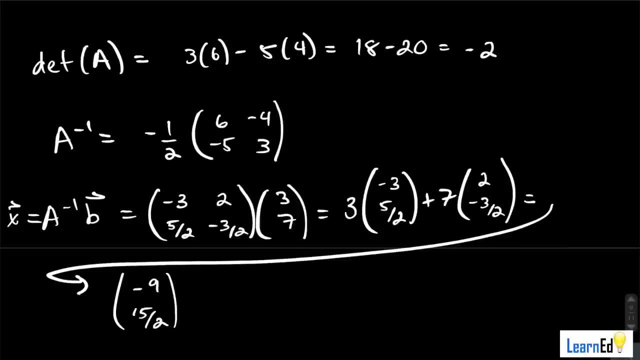 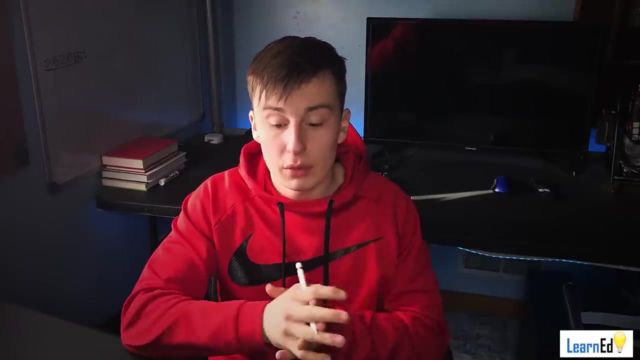 negative 9, 15 halves plus a 14, and then we have a negative 21 over 2 here. okay, so in the end we get a 5 on the top and then we get a negative 6 halves on the bottom, which is negative 3. okay, so definitely a really nice method to use. 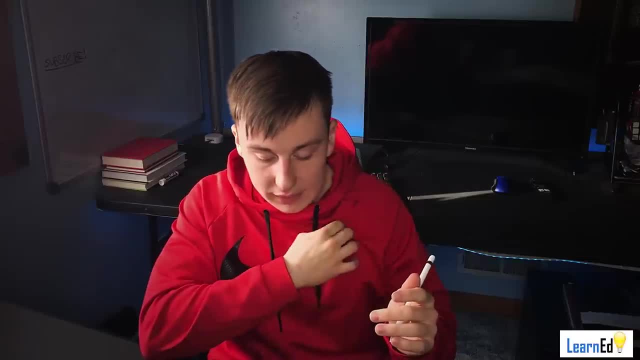 you know, especially in- I mean in this case- we probably would have been able to, you know, especially in, I mean in this case we probably would have been able to, you know, especially in, I mean in this case we probably would have been able to row reduce somewhat. simply, I mean we 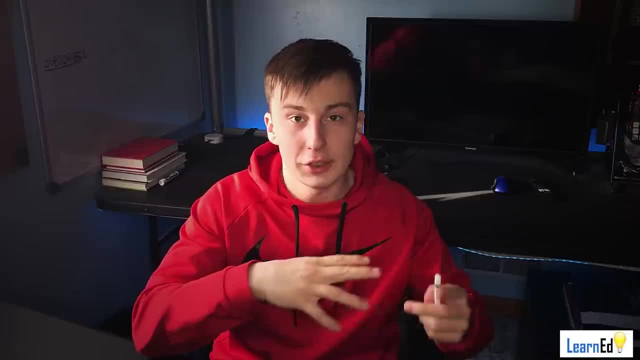 row reduce somewhat simply. I mean we row reduce somewhat simply. I mean we have some some higher values in there, have some some higher values in there, have some some higher values in there, like not just a bunch of zero ones and like not just a bunch of zero ones, and 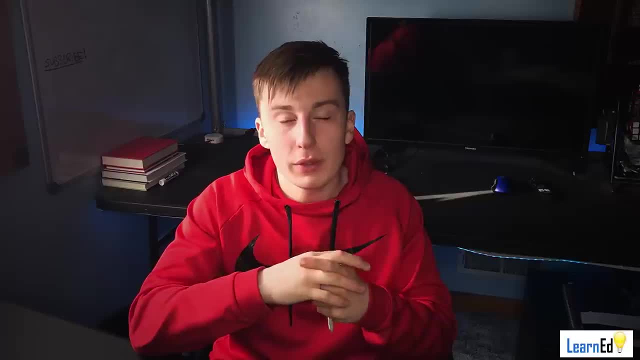 like not just a bunch of zero ones and twos, so it might have been a little bit twos, so it might have been a little bit twos, so it might have been a little bit more difficult to row reduce, but you you more difficult to row reduce, but you you. 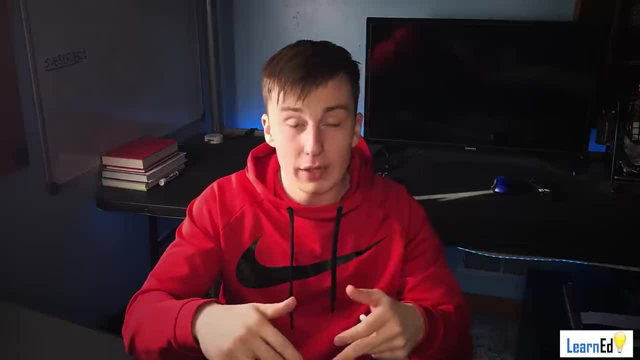 more difficult to row reduce. but you, you know, especially if you have something know, especially if you have something know, especially if you have something with you, know even larger values, like with you know even larger values, like with you. know even larger values, like maybe double digit values. you definitely 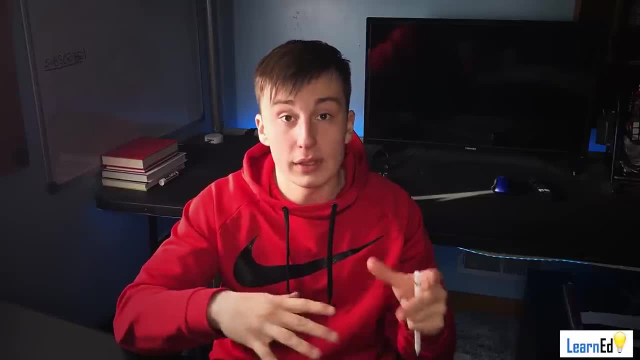 maybe double digit values. you definitely maybe double digit values. you definitely want to consider using this method using, want to consider using this method using. want to consider using this method using a inverse. so moving on to question seven: a inverse. so moving on to question seven: a inverse. so moving on to question seven. now we're going to talk about the 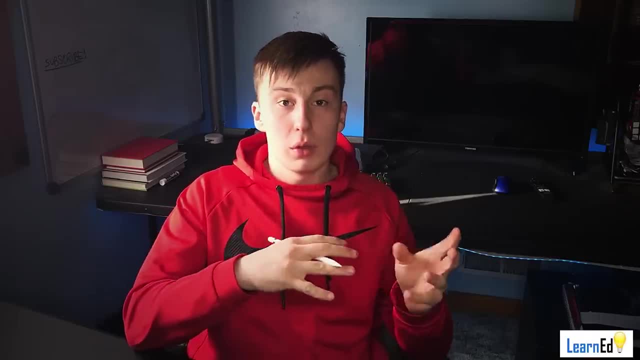 now we're going to talk about the. now we're going to talk about the characterizations of in verbal matrices. characterizations of in verbal matrices, characterizations of in verbal matrices, and if you don't remember that was, and if you don't remember that was and if you don't remember that was basically the invertible matrix theorem. 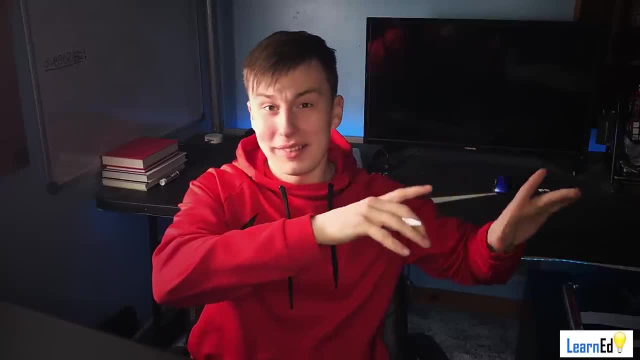 basically the invertible matrix theorem, basically the invertible matrix theorem. okay, and I'm not sure what I actually okay and I'm not sure what I actually okay and I'm not sure what. I actually talked right when I talked about the- the talked right when I talked about the- the. 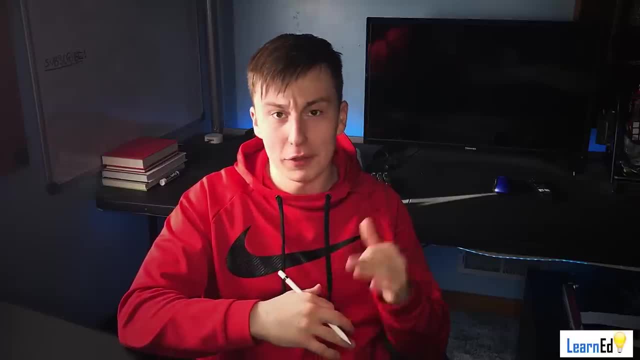 talked right when I talked about the the menu. in the beginning of all the menu. in the beginning of all the menu, in the beginning of all the different topics. I'm not sure if I different topics. I'm not sure if I different topics. I'm not sure if I called this the invertible matrix. 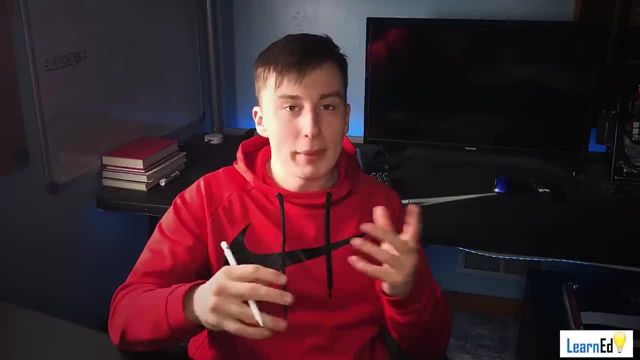 called this the invertible matrix, called this the invertible matrix theorem, or if I called this theorem, or if I called this theorem, or if I called this characterizations of invertible, characterizations of invertible, characterizations of invertible matrices. but basically that's what this. 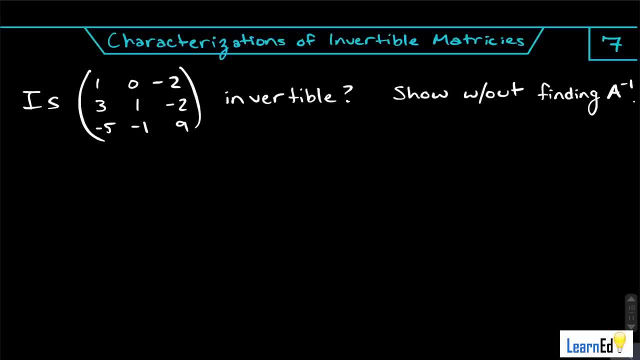 matrices, but basically that's what this matrices, but basically that's what this problem is going to be about, okay, so problem is going to be about. okay, so problem is going to be about okay. so we're being asked: is this 3x3 matrix? we're being asked: is this 3x3 matrix? 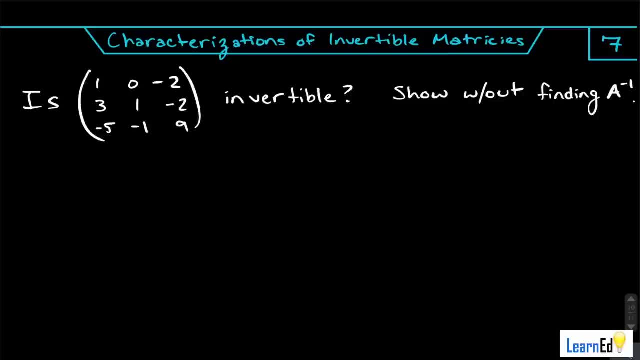 we're being asked: is this 3x3 matrix invertible? okay, and we want to show invertible? okay, and we want to show invertible, okay, and we want to show this without finding a inverse? okay, so the this without finding a inverse? okay, so the. 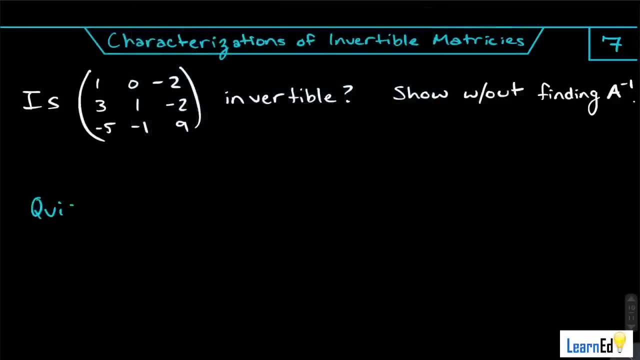 this without finding a inverse. okay. so the quickest check for the invertible, quickest check for the invertible. quickest check for the invertible matrix theorem: okay is to see if it is matrix theorem. okay is to see if it is matrix theorem. okay is to see if it is linearly independent, and onto and. 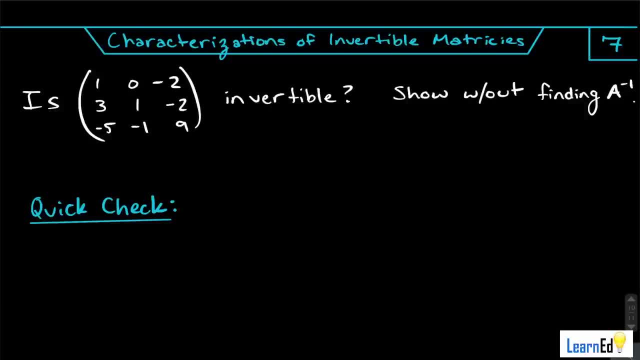 linearly independent and onto and linearly independent and onto, and basically what that means is that we basically what that means is that we basically what that means is that we need to see if there's n pivot positions, need to see if there's n pivot positions. 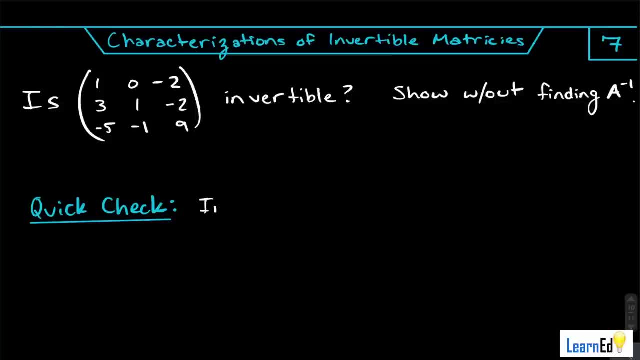 need to see. if there's n pivot positions- okay, so invertible. if okay, so invertible. if okay, so invertible. if there is a pivot position in every column: there is a pivot position in every column. there is a pivot position in every column- okay. so if there's a pivot in every. 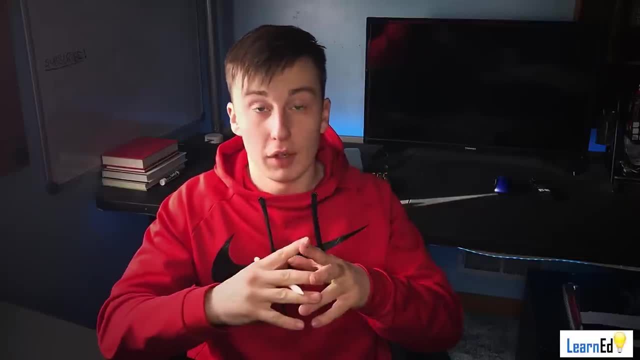 okay. so if there's a pivot in every, okay. so if there's a pivot in every column, then your matrix is invertible column, then your matrix is invertible column, then your matrix is invertible, okay. so all we need to do is row reduce. okay, so all we need to do is row reduce. 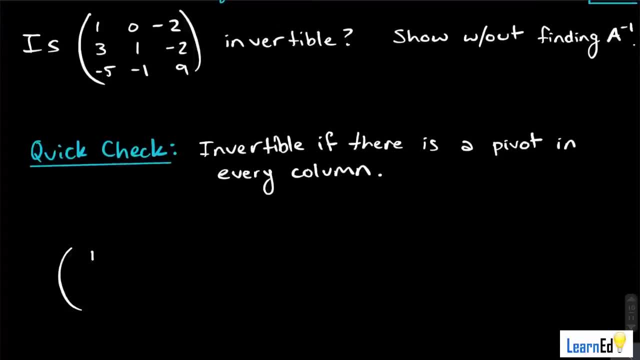 okay, so all we need to do is row reduce and see what we get. let's do that quick and see what we get. let's do that quick and see what we get. let's do that quick. we have 1: 0 negative 2, 3, 1 negative 2 and 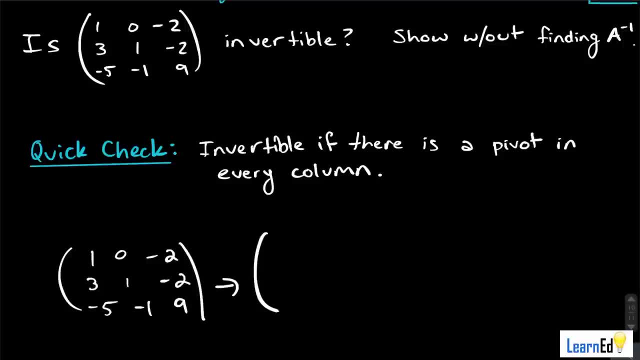 we have 1: 0 negative 2, 3, 1 negative 2 and we have 1, 0 negative 2, 3 1 negative 2 and negative 5. negative 1 and 9 we can start. negative 5, negative 1 and 9: we can start. 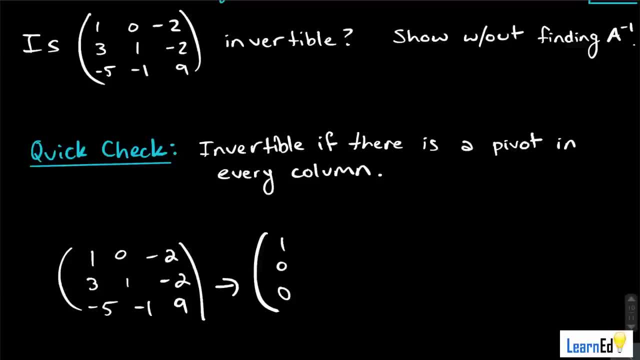 negative, 5 negative 1 and 9. we can start off by zeroing out the first column off. by zeroing out the first column off, by zeroing out the first column, except for the pivot. okay, we'll keep the, except for the pivot. okay, we'll keep the. 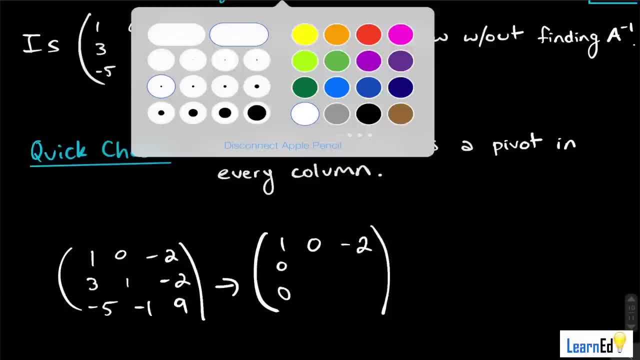 except for the pivot. okay, we'll keep the first column, the second row and third first column, the second row and third first column. the second row and third row are going to be the ones that change. row are going to be the ones that change. row are going to be the ones that change, since we have a 0 entry in the first. 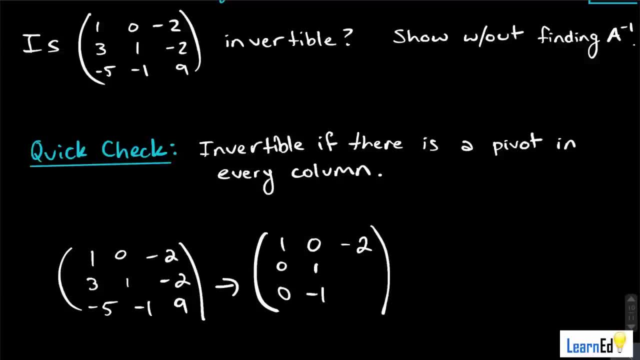 since we have a 0 entry in the first, since we have a 0 entry in the first column, here we know that our second column here, we know that our second column here, we know that our second column will stay the same, and now we'll column will stay the same, and now we'll. 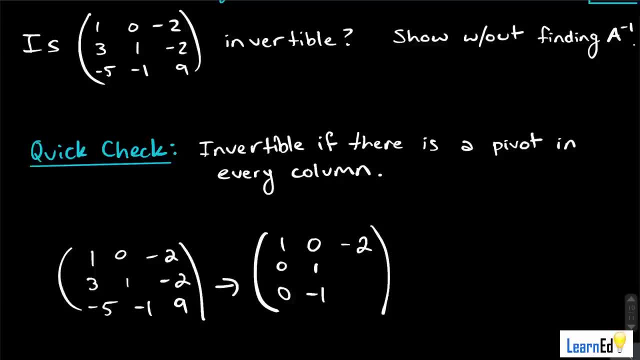 column will stay the same, and now we'll actually have to worry about our third, actually have to worry about our third, actually have to worry about our third column. so our negative 2 needs to get column. so our negative 2 needs to get column. so our negative 2 needs to get multiplied by what? well, for our 1 or 1? 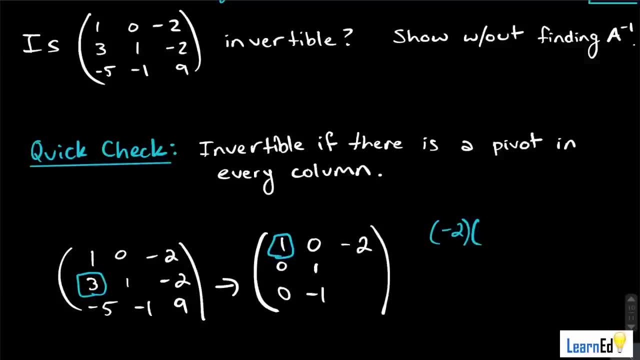 multiplied by what well for our 1 or 1, multiplied by what well for our 1 or 1, multiplied by negative 3, and add it on to multiplied by negative 3, and add it on to multiplied by negative 3 and add it on to this 3 here to get 0. so we multiply. 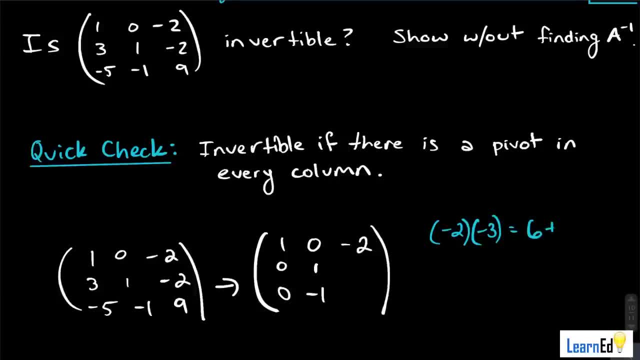 this 3 here to get 0. so we multiply this 3 here to get 0. so we multiply this negative 2 by negative 3, we get 6. this negative 2 by negative 3, we get 6. this negative 2 by negative 3, we get 6. and we add it on to the negative 2 to. 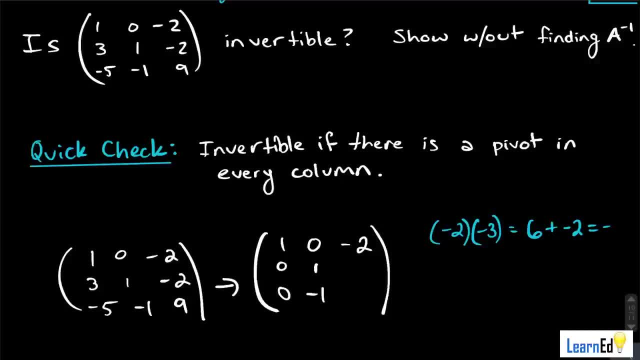 and we add it on to the negative 2 to and we add it on to the negative 2 to get a a start, not negative 4. we get a 4. get a a start, not negative 4. we get a 4. get a a start, not negative 4. we get a 4. okay, so we get a 4 here. then we're going. 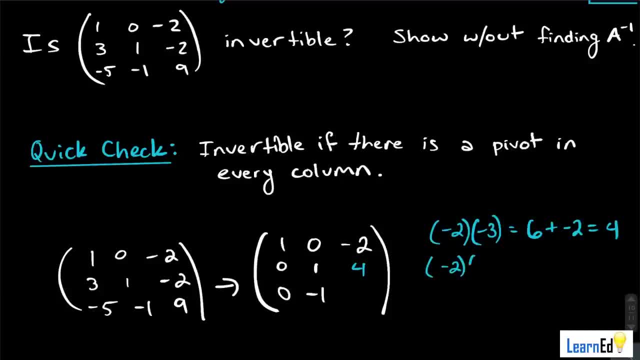 okay, so we get a 4 here, then we're going. okay, so we get a 4 here, then we're going to move on to our last entry and to get to move on to our last entry and to get to move on to our last entry and to get that to be 0. in the first column we had 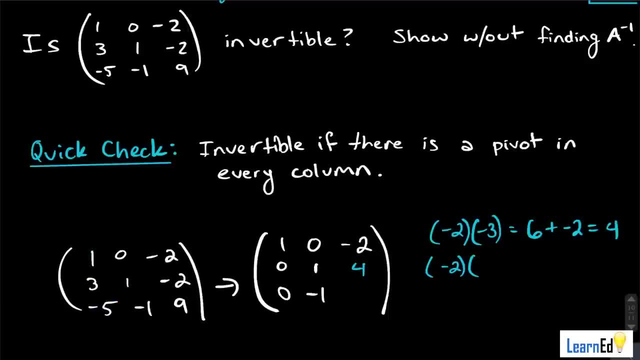 that to be 0 in the first column. we had that to be 0 in the first column. we had to multiply 1 by 5 and then add on. so we to multiply 1 by 5 and then add on. so we to multiply 1 by 5 and then add on. so we have to multiply negative 2 by 5 and we 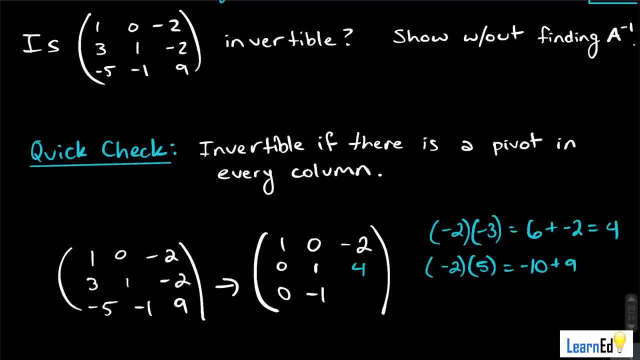 have to multiply negative 2 by 5. and we have to multiply negative 2 by 5 and we get a negative 10. we're going to add on, get a negative 10. we're going to add on, get a negative 10. we're going to add on to the 9 and we get a negative 1. okay, so, 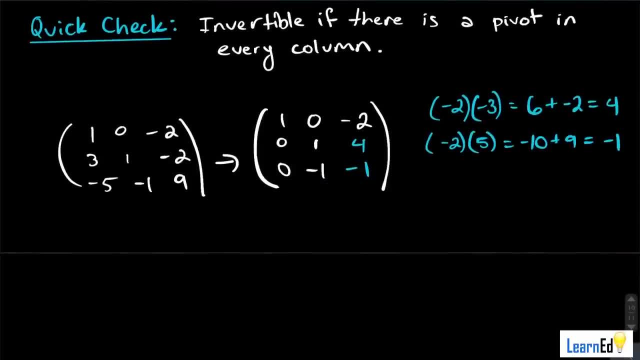 to the 9 and we get a negative 1- okay. so to the 9 and we get a negative 1- okay. so now all we have to do is zero out this now. all we have to do is zero out this now. all we have to do is zero out this entry, and then we're in a row. echelon. 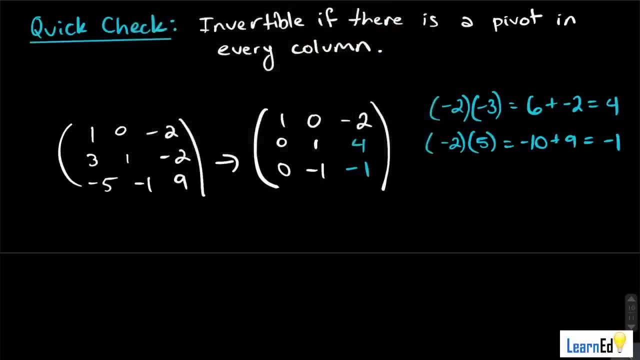 entry. and then we're in a row: echelon entry. and then we're in a row echelon form where we can make a conclusion: okay. form where we can make a conclusion: okay. form where we can make a conclusion: okay. so we get a 1: 0, we get negative: 2: 0, 1, 4. so we get a 1 0, we get negative 2 0, 1 4. so we get a 1 0, we get negative 2 0, 1 4, and then the only thing that's going to, and then the only thing that's going to. 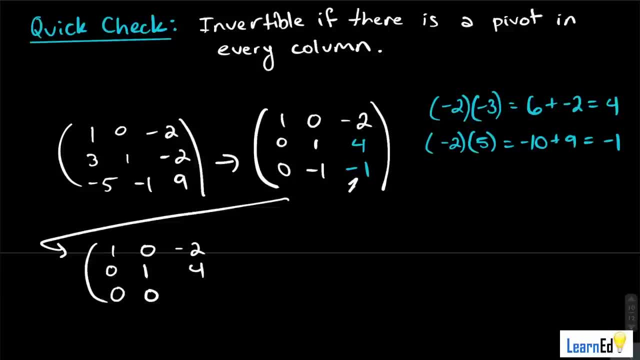 and then the only thing that's going to change is that 0 there, and then this change is that 0 there, and then this change is that 0 there, and then this negative 1 is going to change now to get negative 1 is going to change now to get. 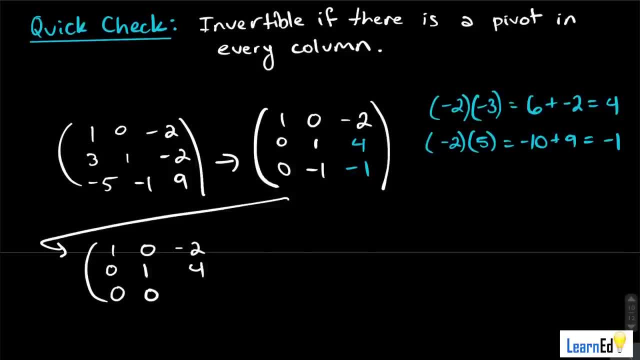 negative 1 is going to change now. to get this negative 1 to be 0, we can just do this negative 1 to be 0. we can just do this negative 1 to be 0. we can just do row 2 plus row 3, so we can say now that: 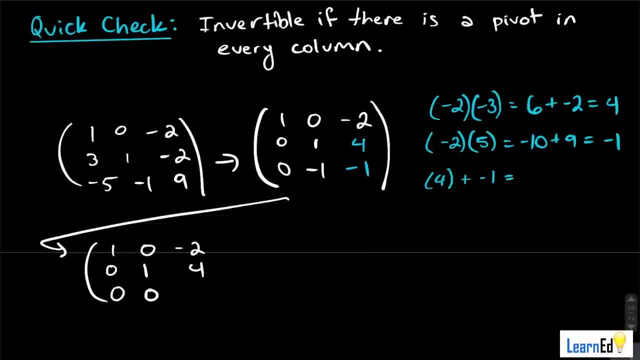 row 2 plus row 3. so we can say now that row 2 plus row 3. so we can say now that this is going to be 4 plus negative 1. this is going to be 4 plus negative 1. this is going to be 4 plus negative 1, which is 3, so this becomes 3. okay, now we 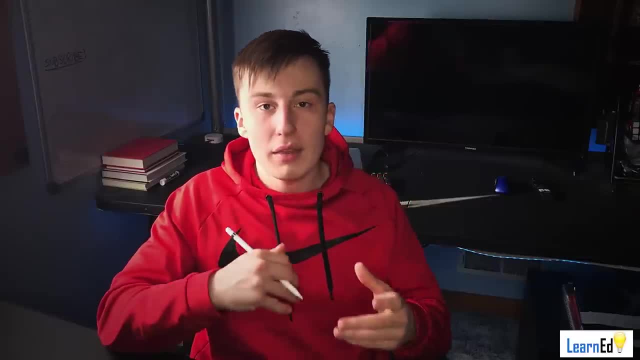 which is 3, so this becomes 3. okay now. we, which is 3, so this becomes 3: okay now. we can see that there's going to be a, can see that there's going to be a, can see that there's going to be a pivot position in every column and that 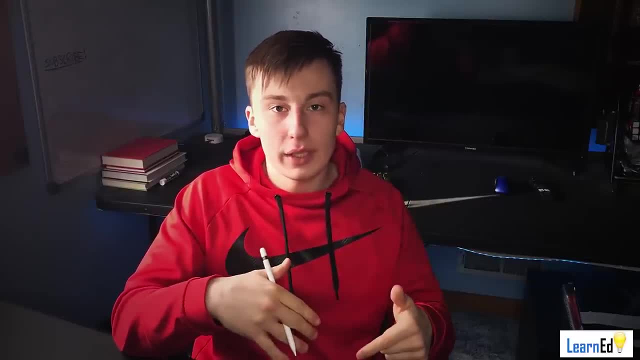 pivot position in every column and that pivot position in every column and that is kind of you can draw that conclusion, is kind of you can draw that conclusion is kind of you can draw that conclusion right now. but you know a lot of people right now, but you know a lot of people. 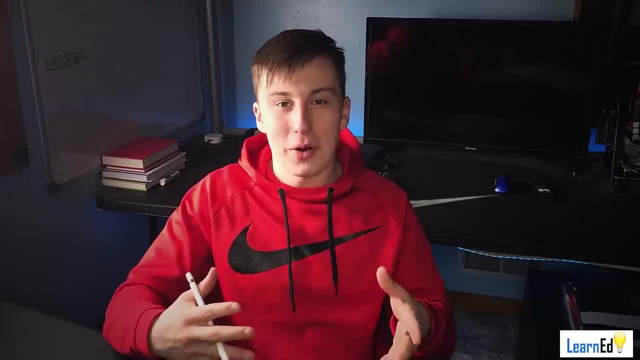 right now. but you know a lot of people like to get to reduce rush long form, like to get to reduce rush long form, like to get to reduce rush long form, just as a kind of a precaution, just as, just as a kind of a precaution, just as. 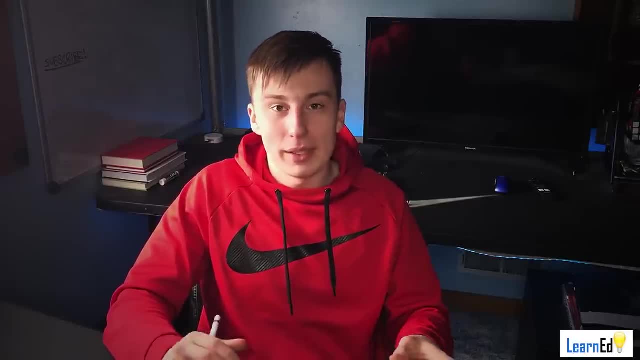 just as a kind of a precaution, just as like a safety measure, and I do like to like a safety measure and I do like to like a safety measure, and I do like to do that as well, just because it makes me do that as well, just because it makes me. 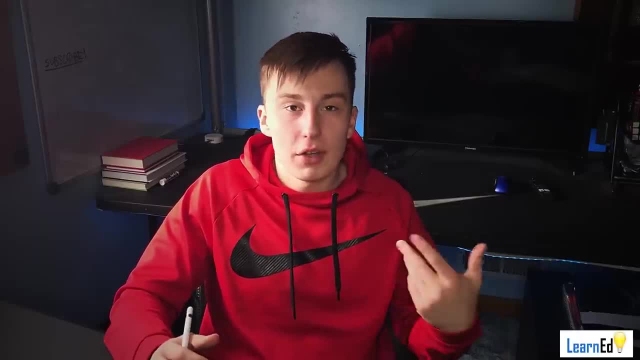 do that as well, just because it makes me feel better and makes me feel that I feel better. and makes me feel that I feel better and makes me feel that I definitely got the right answer, even definitely got the right answer, even definitely got the right answer, even though, if you get here, you are done, so I 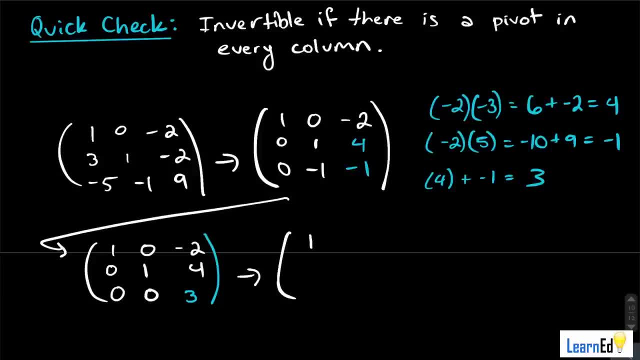 though, if you get here, you are done so. I, though, if you get here, you are done so, I can just get to reduce rush long form, can just get to reduce rush long form, can just get to reduce rush long form here, and what we can do is scale the. 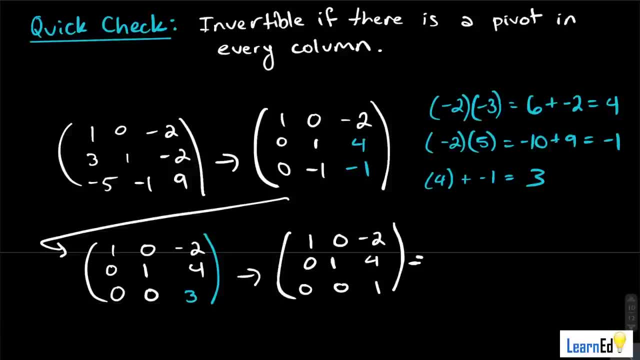 here, and what we can do is scale the here, and what we can do is scale the third row, and then we can zero out the third row, and then we can zero out the third row, and then we can zero out the the third column, except for the pivot. 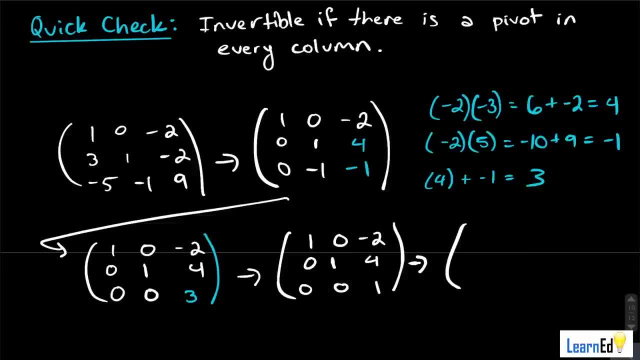 the third column, except for the pivot. the third column, except for the pivot, because we have a zero here and a zero, because we have a zero here and a zero, because we have a zero here and a zero here. so we get one zero, zero, zero, zero here. so we get one zero, zero, zero, zero. 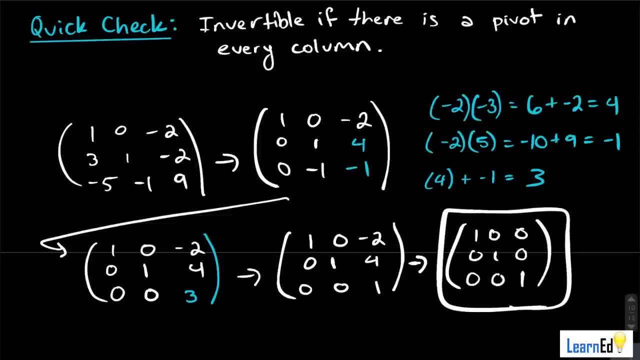 here. so we get one zero, zero, zero, zero, zero one, zero, zero one. and there you go: zero one, zero, zero, zero one. and there you go. zero one, zero, zero, zero one. and there you go, you have your identity matrix, and you have your identity matrix, and you have your identity matrix and you are now in reduced, rush line form. okay, 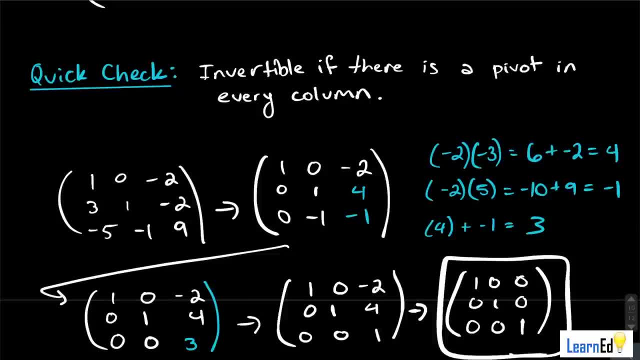 you are now in reduced rush line form, okay, you are now in reduced rush line form, okay. so now that we see we have a we, so now that we see we have a we, so now that we see we have a, we definitely have a pivot in every column. 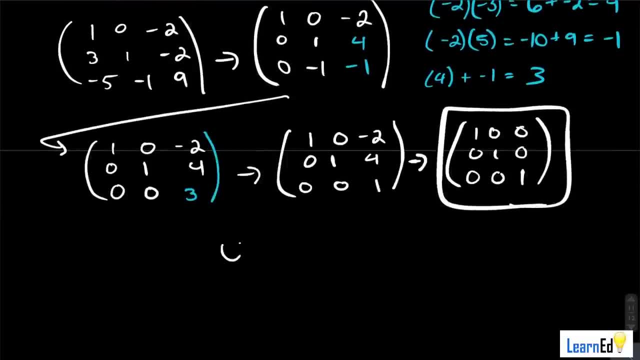 definitely have a pivot in every column, definitely have a pivot in every column. this matrix is invertible. so the answer: this matrix is invertible. so the answer: this matrix is invertible. so the answer is yes, all right. so moving on to our is yes, all right. so moving on to our. 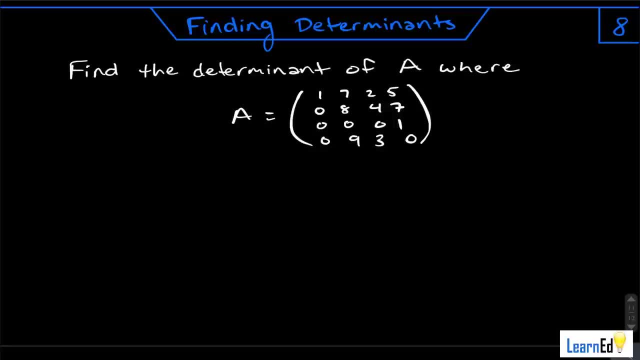 is yes, all right. so, moving on to our next problem on finding determinants. next problem on finding determinants. next problem on finding determinants: problem a is asking us to find the problem. a is asking us to find the problem. a is asking us to find the determinant of a where a is some. 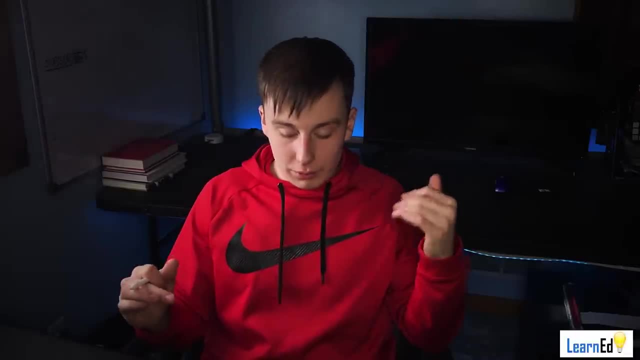 determinant of a where a is some. determinant of a where a is some 4x4 matrix. now we all know that you know 4x4 matrix. now we all know that you know 4x4 matrix. now we all know that you know finding a determinant of something that. 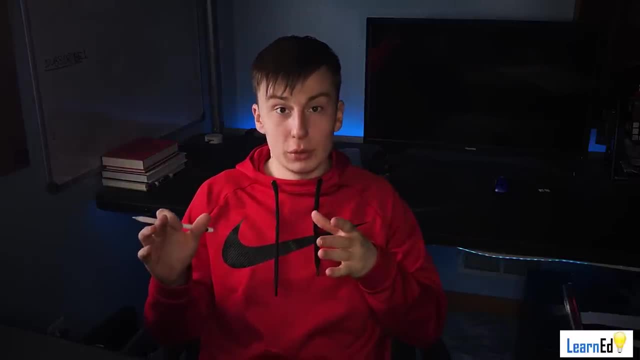 finding a determinant of something, that finding a determinant of something that is, you know, a 2x2 or sorry that is, is you know a 2x2 or sorry that is? is you know a 2x2 or sorry, that is greater than a 2x2, is really annoying. 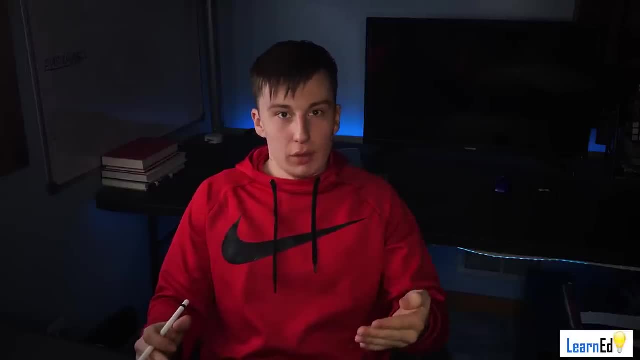 greater than a 2x2 is really annoying. greater than a 2x2 is really annoying, and especially with something like a, and especially with something like a, and especially with something like a 4x4- okay, but what we can do here since 4x4 okay, but what we can do here since. 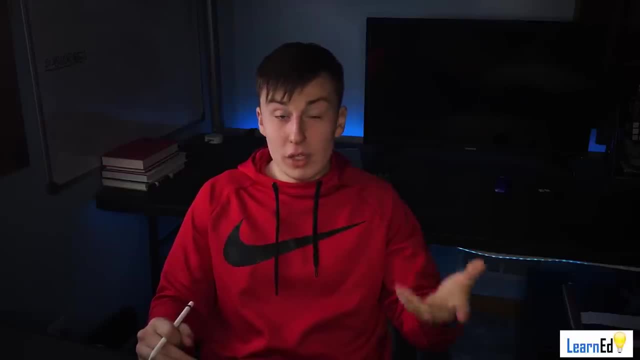 4x4. okay, but what we can do here, since we actually have a lot of zeros in? we actually have a lot of zeros in. we actually have a lot of zeros in certain rows and certain columns. we can certain rows and certain columns. we can certain rows and certain columns. we can do a cofactor expansion to make this a. 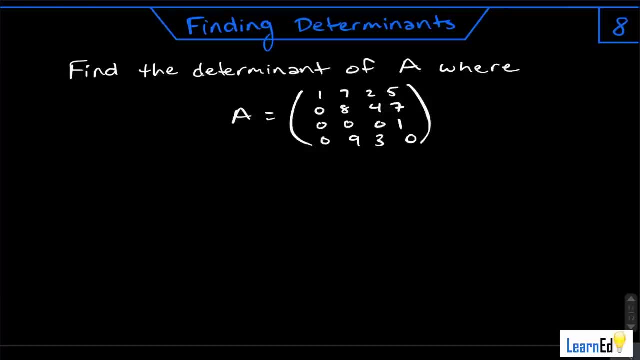 do a cofactor expansion to make this a do a cofactor expansion to make this a lot easier for ourselves. so you can see lot easier for ourselves, so you can see lot easier for ourselves. so you can see here that first off our first column, and here that first off our first column, and 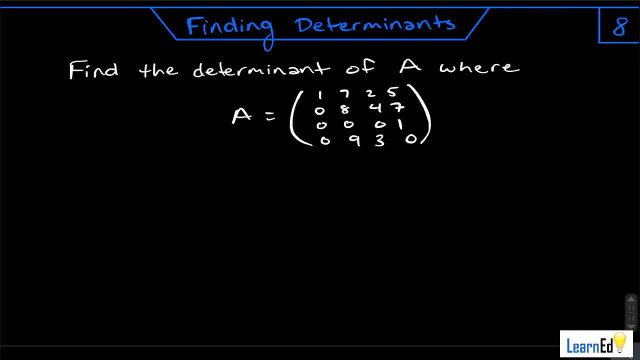 here that first off our first column and our third row. they have three zeros in our third row. they have three zeros in our third row. they have three zeros in them. so that's gonna be a great place to them. so that's gonna be a great place to. 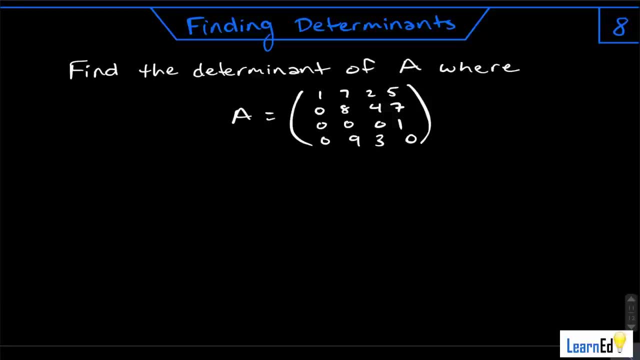 them, so that's gonna be a great place to do a cofactor expansion, okay, so remember, do a cofactor expansion. okay, so remember, do a cofactor expansion. okay. so remember that the formula for a cofactor, that the formula for a cofactor, that the formula for a cofactor expansion, right, is you? basically just 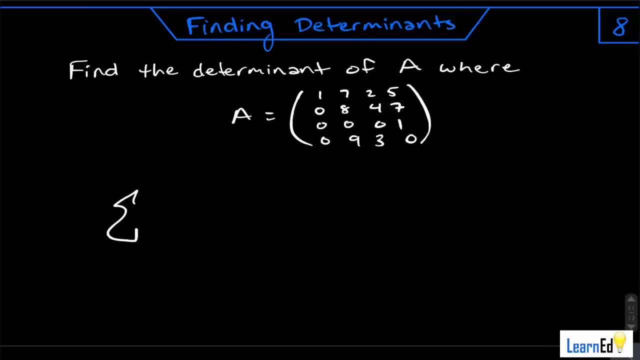 expansion right? is you basically just expansion, right? is you basically just have a sum okay from the? I'll just write: have a sum okay from the. I'll just write: have a sum okay from the. I'll just write it as a sum okay, I'm not gonna confuse. 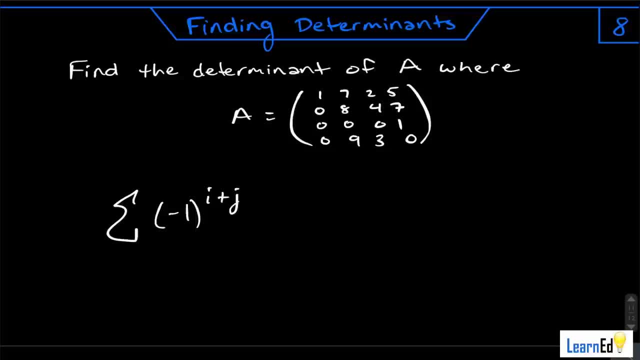 it as a sum. okay, I'm not gonna confuse it as a sum. okay, I'm not gonna confuse you with any other notation. it's you with any other notation? it's you with any other notation? it's negative 1 to the I plus J, where I is. 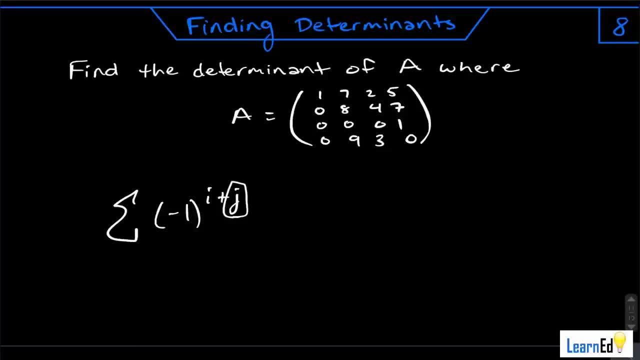 negative. 1 to the I plus J where I is negative. 1 to the I plus J where I is the row entry that you're at, or the the, the row entry that you're at, or the the the row entry that you're at or the the row that you're on in J is the column. 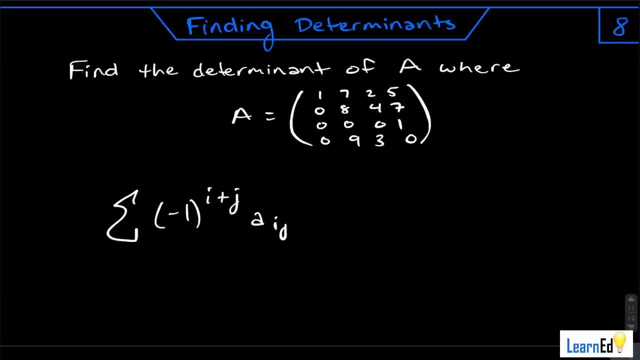 row that you're on in J is the column row that you're on in J is the column that you're on and you have some aij, so that you're on and you have some aij so that you're on and you have some aij. so whatever the value is at the entry that 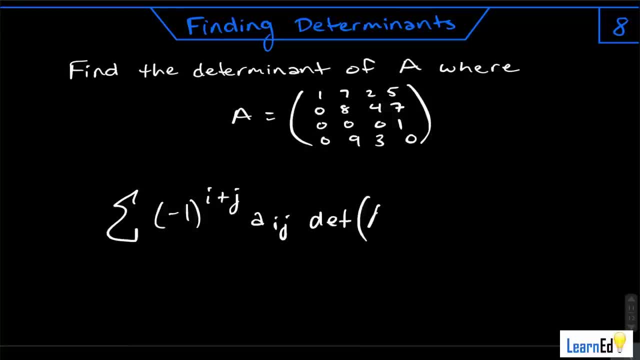 whatever the value is at the entry, that, whatever the value is at the entry, that you're focused on and it's going to be you're focused on and it's going to be you're focused on and it's going to be times the determinant of aij, okay, and 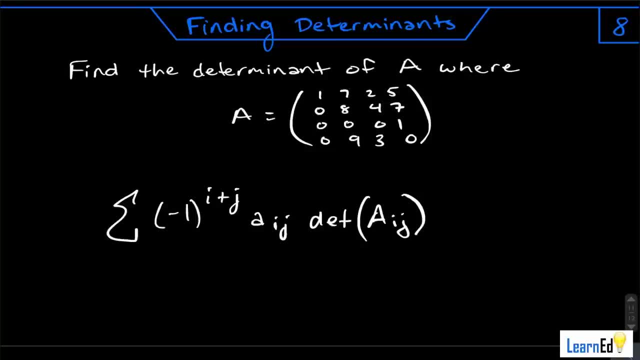 times the determinant of aij okay and times the determinant of aij okay, and that's some really that can be. that's some really that can be. that's some really that can be. definitely some confusing notation, but definitely some confusing notation, but definitely some confusing notation. but what this ends up meaning is that we are 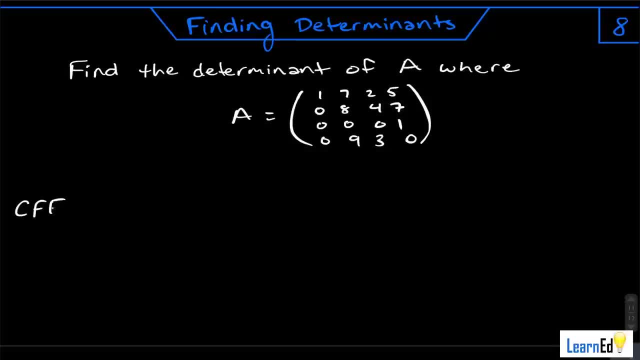 what this ends up meaning is that we are. what this ends up meaning is that we are going to and doing a cofactor expansion. going to and doing a cofactor expansion. going to and doing a cofactor expansion down the first column here what we're, down the first column here, what we're. 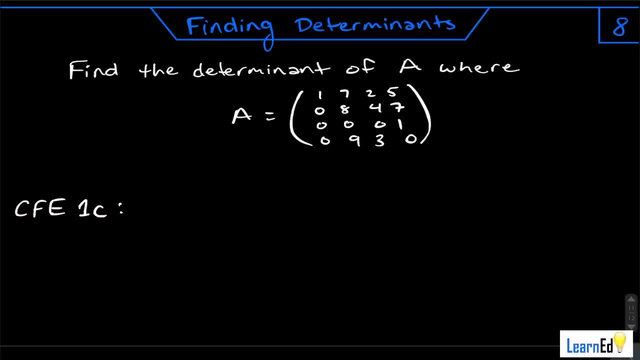 down the first column here. what we're going to do is say that we have a going to do. is say that we have a going to do is say that we have a negative one to the I plus J. we have the negative one to the I plus J, we have the. 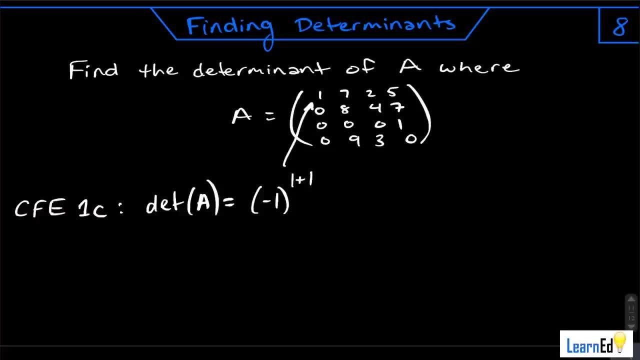 negative one to the I plus J, we have the entry at the position. this is at one one. entry at the position. this is at one one. entry at the position. this is at one one right. we're at the first row in the right. we're at the first row in the. 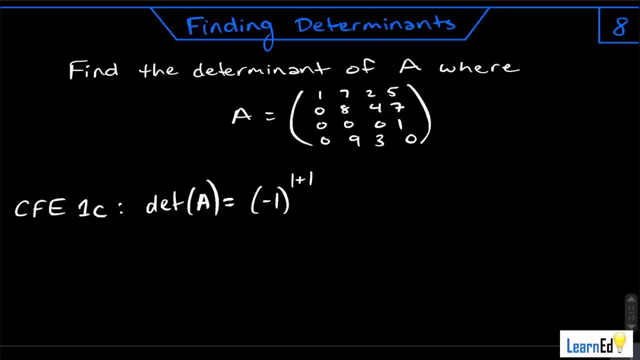 right, we're at the first row in the first column and that's our entry there, first column, and that's our entry there, first column, and that's our entry there. so we have a negative one to the one. so we have a negative one to the one. 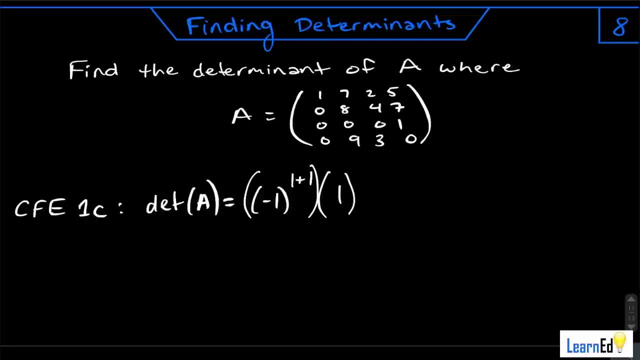 so we have a negative one to the one plus one times a one right, which is the plus one times a one right, which is the plus one times a one right, which is the actual entry and the position: okay, actual entry and the position. okay, actual entry and the position okay, that's the AI J, and then we have the 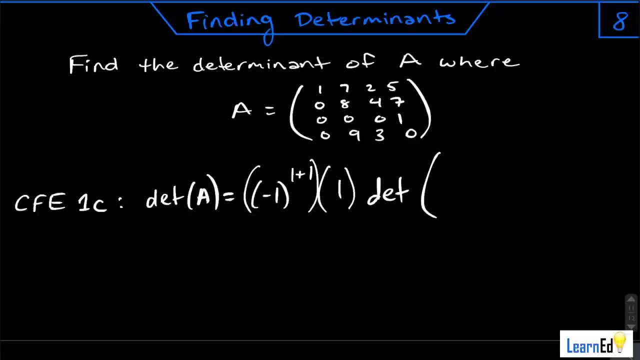 that's the AI J. and then we have the. that's the AI J. and then we have the determinant of that big AI J. which determinant of that big AI J, which determinant of that big AI J which basically just means every entry is, basically just means every entry is. 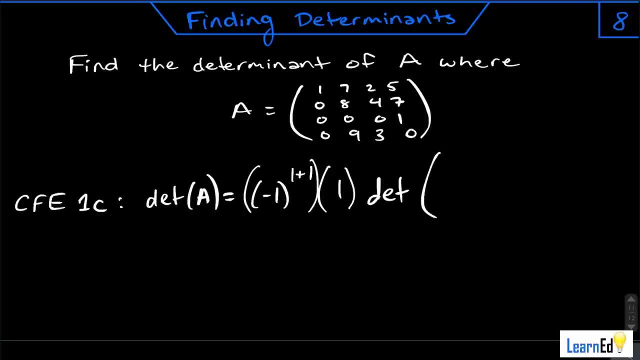 basically just means every entry is going to be included in this. that's not going to be included in this. that's not going to be included in this. that's not in the same row or column as that value. in the same row or column as that value. 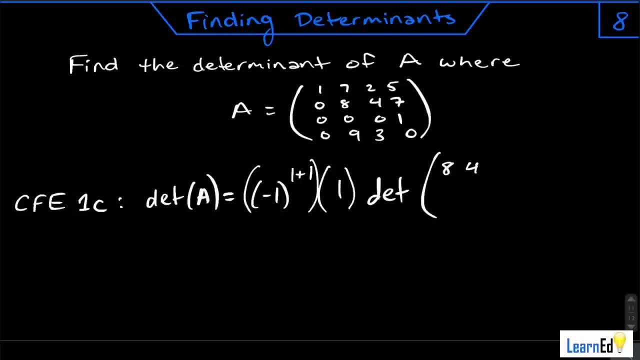 in the same row or column as that value. that. we just took that one. so we have that. we just took that one. so we have that, we just took that one. so we have the determinant of eight four seven zero. the determinant of eight four seven zero. the determinant of eight four seven zero. zero. one nine three zero. okay. and if we 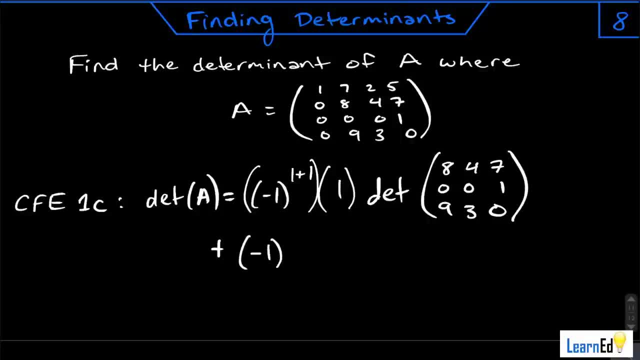 zero one, nine, three, zero, okay. and if we zero one, nine three, zero, okay. and if we kept adding on terms, we'd have you know, kept adding on terms, we'd have you know, kept adding on terms, we'd have you know this would be negative one to the we. 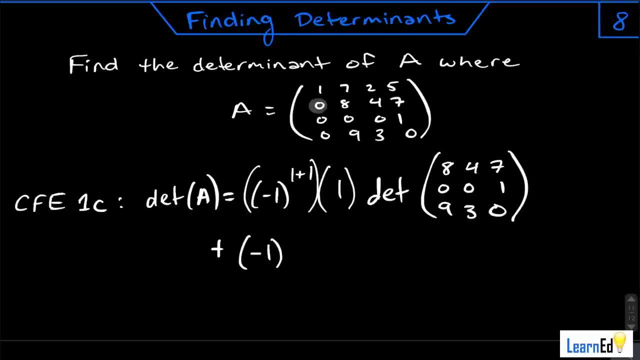 this would be negative one to the we. this would be negative one to the we. could go down to the zero next. okay. could go down to the zero next. okay. could go down to the zero next. okay, cuz we're going down the first column, cuz we're going down the first column. 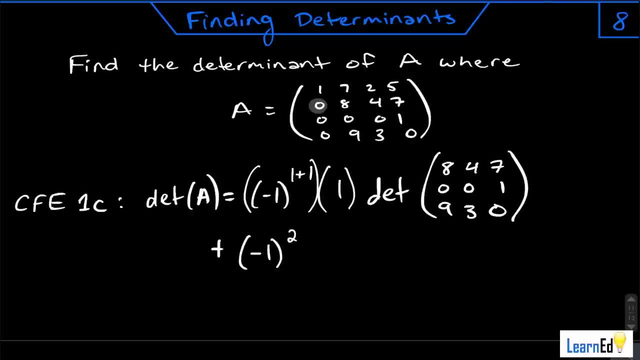 cuz we're going down the first column and we would have negative one to the and we would have negative one to the and we would have negative one to the. we're in the second row now and we're in. we're in the second row now and we're in. 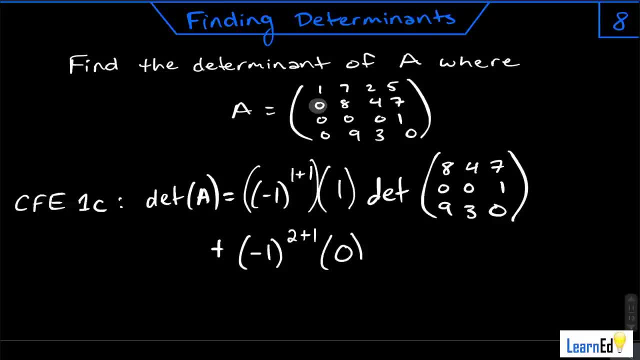 we're in the second row now and we're in the first column still, and now we have the first column still, and now we have the first column still, and now we have a zero okay, and we'll have a determinant. a zero, okay, and we'll have a determinant. 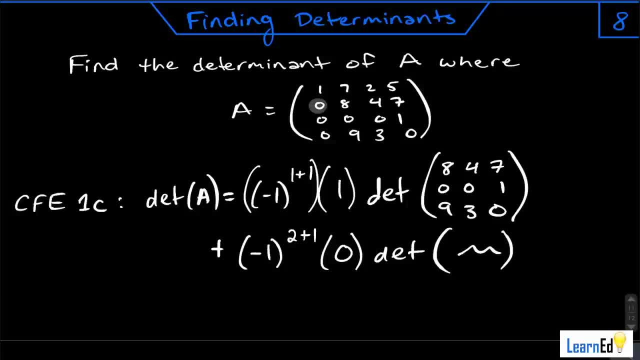 a zero, okay, and we'll have a determinant of something, but it doesn't matter of something, but it doesn't matter of something, but it doesn't matter because we have a zero here, okay, and as because we have a zero here, okay, and as because we have a zero here, okay, and as we keep going down that first column, we 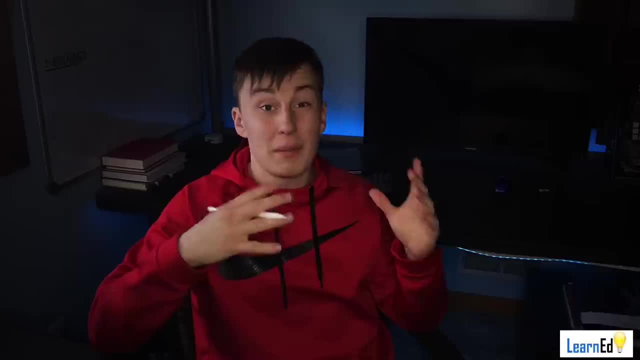 we keep going down that first column, we we keep going down that first column. we keep hitting zeros. again and again, it keep hitting zeros, again and again, it keep hitting zeros, again and again, it again. so the only thing that matters is again. so the only thing that matters is: 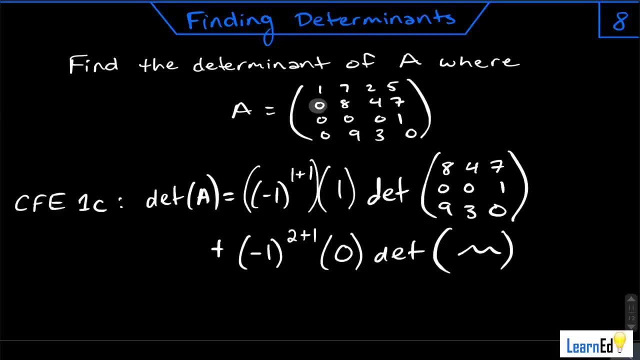 again. so the only thing that matters is that first term that we had. okay, so kind that first term that we had okay, so kind that first term that we had okay, so kind of erasing this because it doesn't, of erasing this because it doesn't. 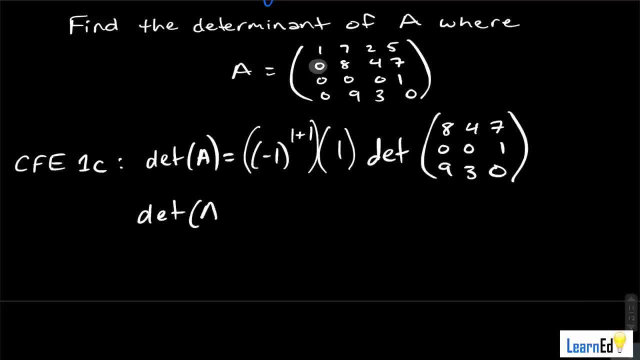 of erasing this because it doesn't matter anymore. we have determinant of a matter anymore. we have determinant of a matter anymore. we have determinant of a. equals a negative 1 to the 1 plus 1. equals a negative 1 to the 1 plus 1. 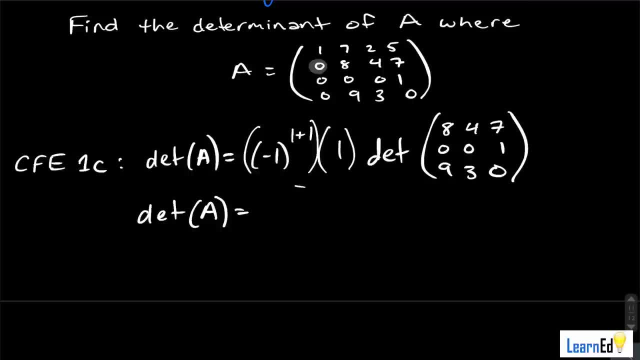 equals a negative 1 to the 1 plus 1 negative 1 squared is 1 and 1 times 1 is negative. 1 squared is 1 and 1 times 1 is negative. 1 squared is 1 and 1 times 1 is 1, so really, we just have the. 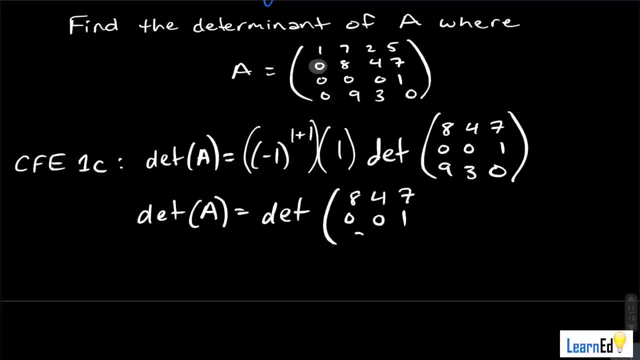 1. so really we just have the 1. so really we just have the determinant of 8, 4, 7, 0 0, 1, 9, 3 0. now. determinant of 8, 4, 7, 0 0, 1, 9, 3 0 now. determinant of 8, 4, 7, 0, 0, 1, 9, 3, 0. now you could go through and compute this. you could go through and compute this. you could go through and compute this. determinant here: right. cut your losses. determinant here: right, cut your losses. 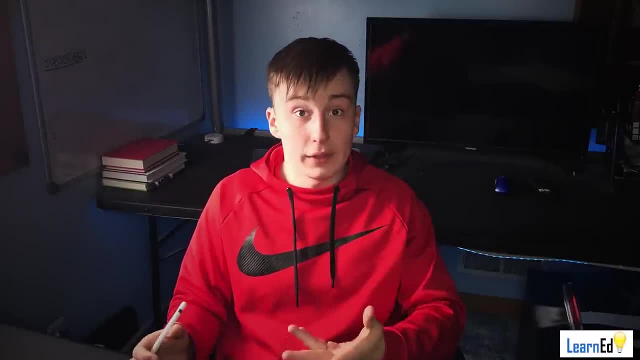 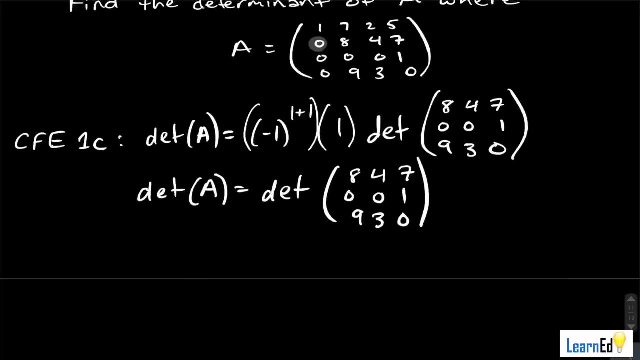 determinant here: right, cut your losses. but what I would do is another cofactor. but what I would do is another cofactor. but what I would do is another cofactor: expansion- okay, and do this one on the expansion. okay, and do this one on the expansion. okay, and do this one on the the second row- okay, so we do a cofactor. 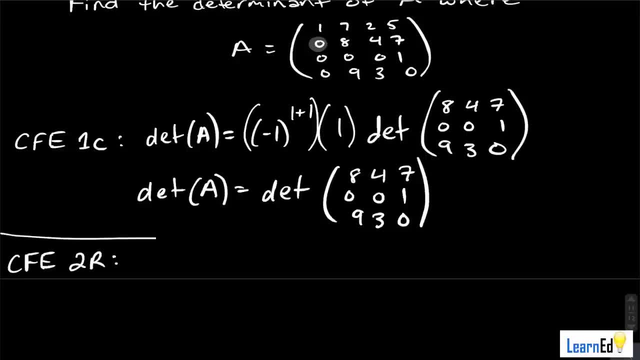 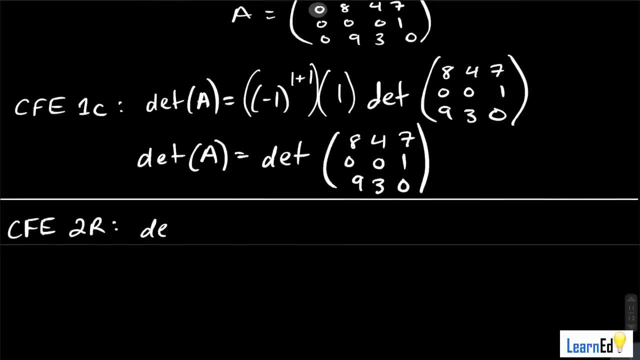 the second row. okay, so we do a cofactor the second row. okay, so we do a cofactor. expansion on the second row. we have a expansion on the second row. we have a expansion on the second row. we have a that the determinant of a is equal to. 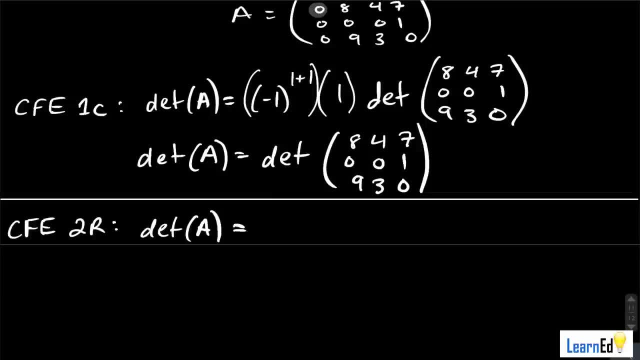 that the determinant of a is equal to that. the determinant of a is equal to now. we'll have now, we'll have now, we'll have first off our first two terms of this. first off, our first two terms of this, first off, our first two terms of this cofactor expansion are going to be zero. cofactor expansion are going to be zero. cofactor expansion are going to be zero. so the only thing that we actually care, so the only thing that we actually care, so the only thing that we actually care about is this one, so we have a negative about- is this one, so we have a negative. 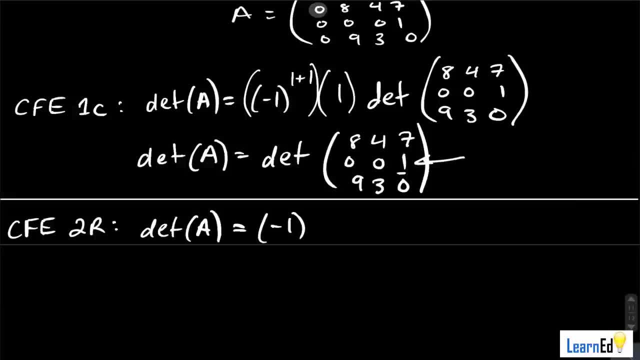 about is this one. so we have a negative one to the. this one is on the second row. one to the. this one is on the second row. one to the. this one is on the second row, in the third column. so we have a in the third column. so we have a. 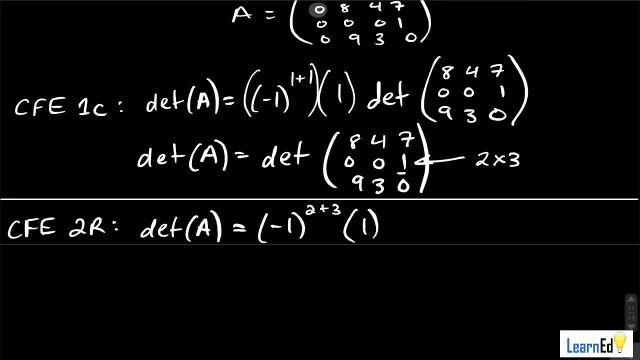 in the third column. so we have a negative one to the two plus three times, negative one to the two plus three times, negative one to the two plus three times the actual value at that entry, which is the actual value at that entry, which is the actual value at that entry which is in the matrix. that are not in the same. 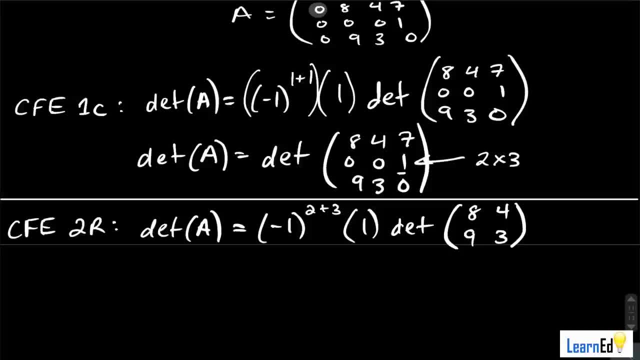 in the matrix that are not in the same in the matrix that are not in the same row or column as the entry that we're row or column, as the entry that we're row or column, as the entry that we're talking about, so determinant of a 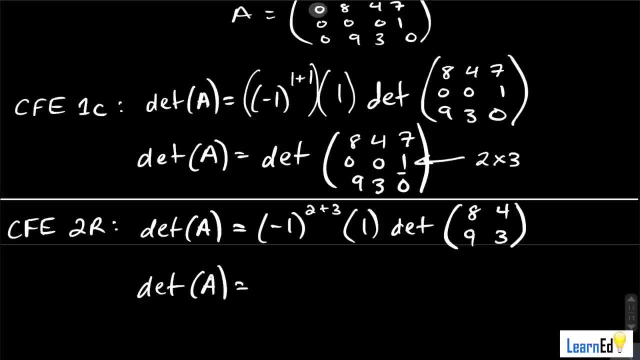 talking about so determinant, of a talking about so determinant, of a negative one to the two plus three. it's negative one to the two plus three. it's negative one to the two plus three. it's an odd power, so we're going to get a, an odd power. so we're going to get a. an odd power, so we're going to get a negative one out here. that's why we have negative one out here. that's why we have negative one out here. that's why we have that negative one to the I plus J and that negative one to the I plus J, and 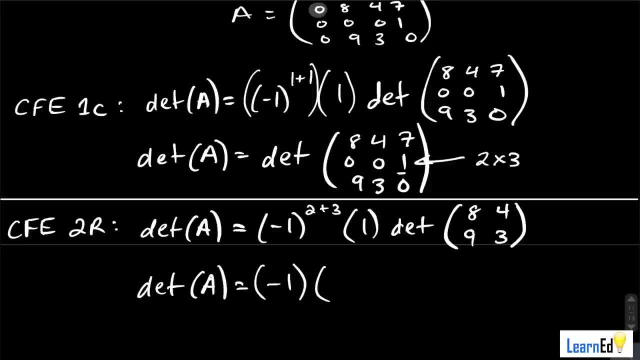 that negative one to the I plus J, and then the determinant of this 2x2 matrix, then the determinant of this 2x2 matrix, then the determinant of this 2x2 matrix is going to be 8 times 3 minus 9 times. 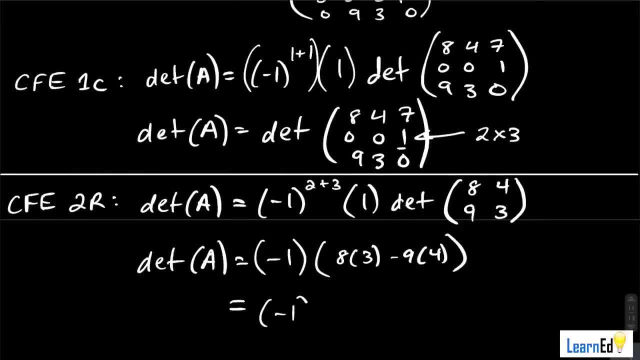 is going to be 8 times 3 minus 9 times is going to be 8 times 3 minus 9 times 4. so it's equal to negative 1 times 24- 4. so it's equal to negative 1 times 24. 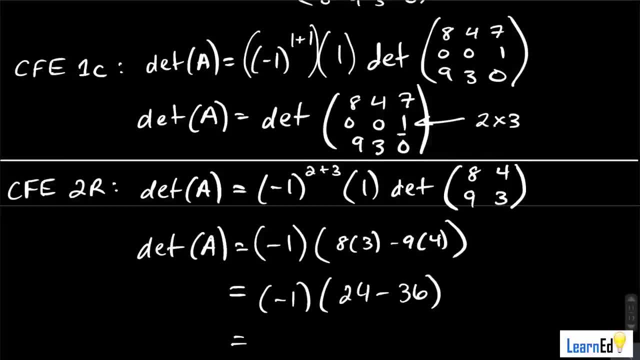 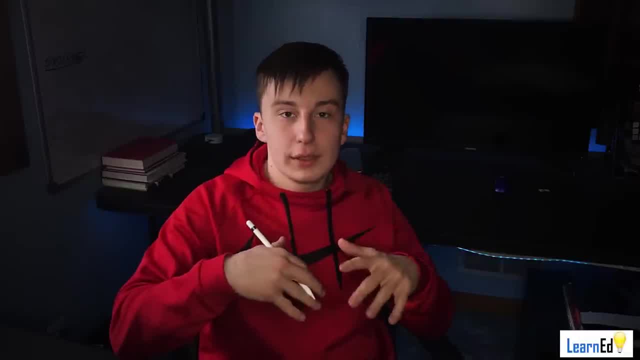 4, so it's equal to negative 1 times 24 minus a 36, and so we get 12. okay, so minus a 36, and so we get 12. okay, so minus a 36, and so we get 12. okay, so cofactor expansions, you know honestly. 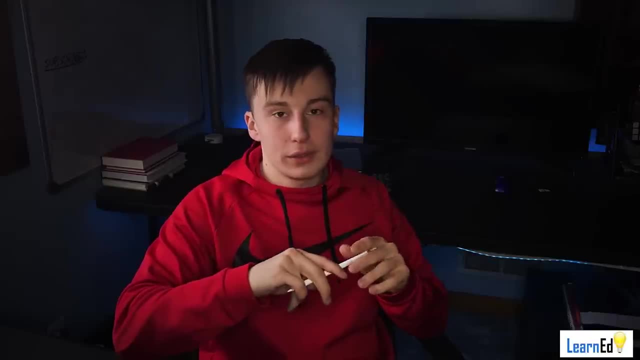 cofactor expansions. you know, honestly, cofactor expansions, you know, honestly, they're very, very, very nice and I think they're very, very, very nice and I think they're very, very, very nice and I think that I'm almost 100% sure that you'll that I'm almost 100% sure that you'll. 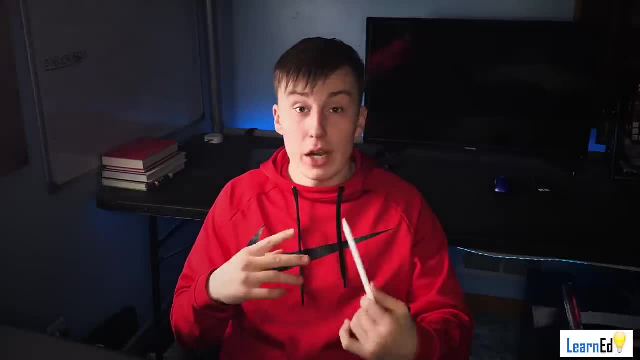 that I'm almost 100% sure that you'll have a cofactor expansion somewhere on. have a cofactor expansion somewhere on. have a cofactor expansion somewhere on your linear algebra final. I know I had your linear algebra final. I know I had your linear algebra final. I know I had one on mine and I think it's very. 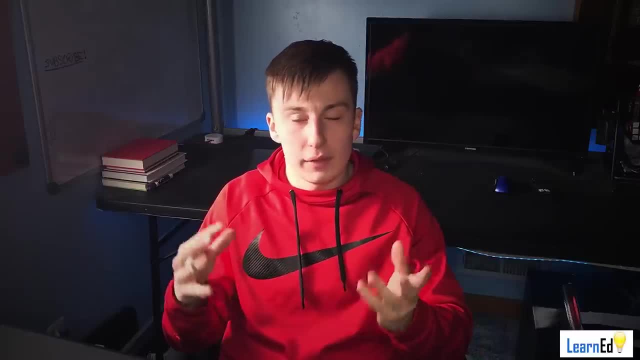 one on mine and I think it's very one on mine and I think it's very popular on on most files. I've seen a popular on on most files. I've seen a popular on on most files. I've seen a couple others. they all seem to have a. 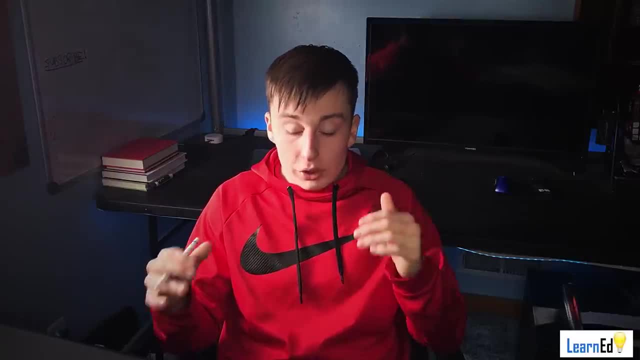 couple others. they all seem to have a couple others. they all seem to have a one cofactor expansion problem. okay. so one cofactor expansion problem okay. so one cofactor expansion problem, okay. so this is definitely very, very important. this is definitely very, very important. this is definitely very, very important review and I hope I explained it in a 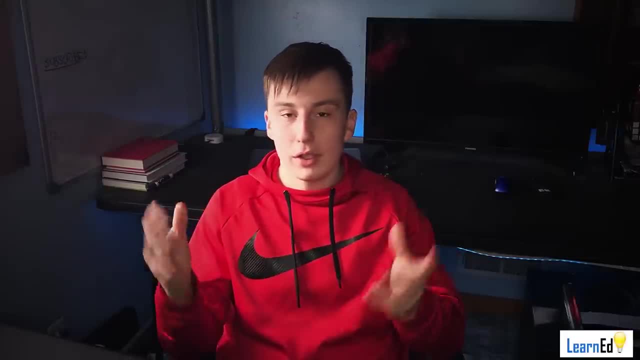 review and I hope I explained it in a review and I hope I explained it in a way that was kind of like down-to-earth way. that was kind of like down-to-earth way, that was kind of like down-to-earth, because I know that when you start because I know that when you start, because I know that when you start throwing in all that notation, and I get throwing in all that notation and I get throwing in all that notation and I get confused with this as well in the math, confused with this as well in the math. 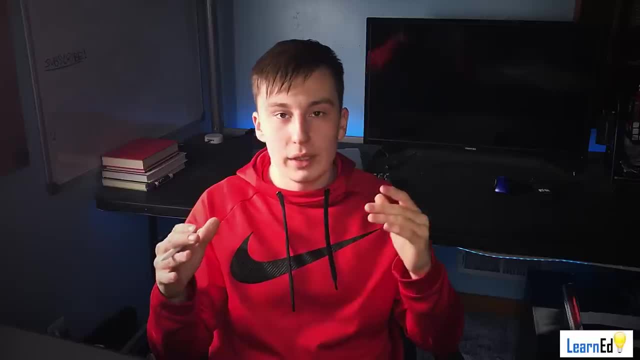 confused with this as well in the math classes that I take. when you start classes that I take, when you start classes that I take, when you start throwing in all that notation- it really throwing in all that notation, it really throwing in all that notation- it really gets confusing and it's easy to get. 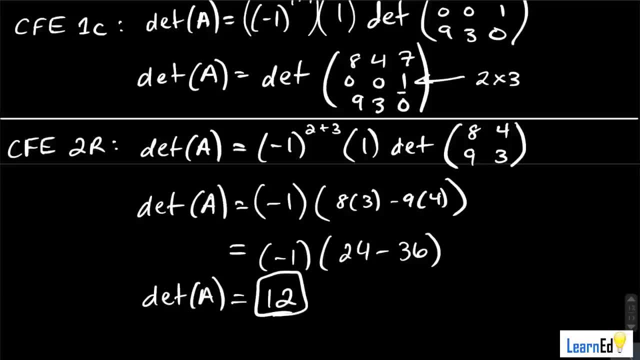 gets confusing and it's easy to get gets confusing and it's easy to get lost pretty quick. so moving on to our next lost pretty quick. so moving on to our next lost pretty quick. so moving on to our next problem. we are being asked to find problem we are being asked to find. 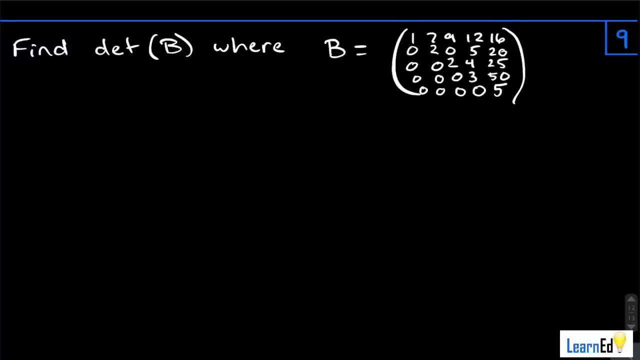 problem. we are being asked to find the determinant of B where B is some now. we the determinant of B where B is some now. we the determinant of B where B is some now we have a five by five matrix- okay, and have a five by five matrix, okay, and 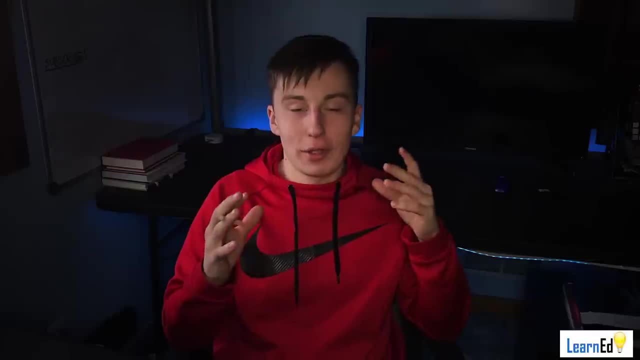 have a five by five matrix, okay, and before you, before you ask no, I'm not before you. before you ask no, I'm not before you. before you ask no, I'm not going to make you do like three. going to make you do like three, going to make you do like three cofactor expansions or anything like. 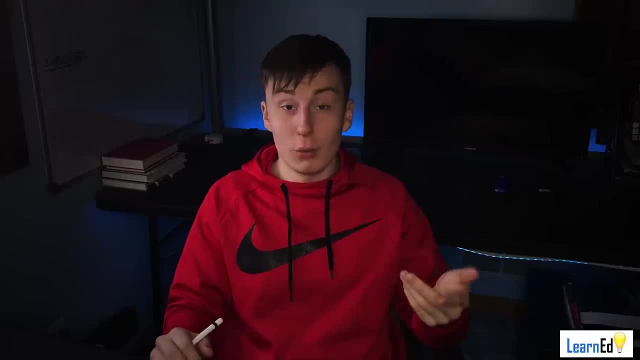 cofactor expansions or anything like cofactor expansions or anything like that. that's not what this problem is. that that's not what this problem is. that that's not what this problem is about. although you could solve it that about, although you could solve it that about, although you could solve it that way if you wanted to, it would just be a. 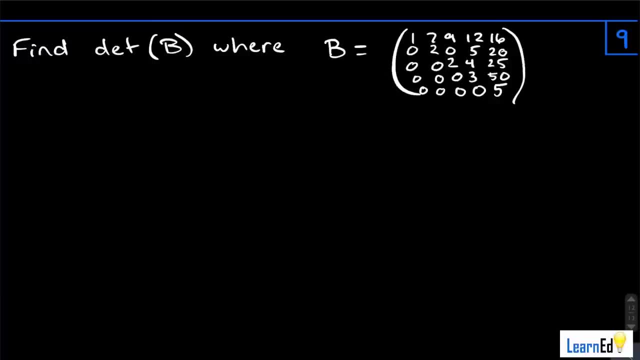 way if you wanted to. it would just be a way. if you wanted to, it would just be a kind of a mess. so how we're actually kind of a mess, so how we're actually kind of a mess, so how we're actually going to find the determinant of this is 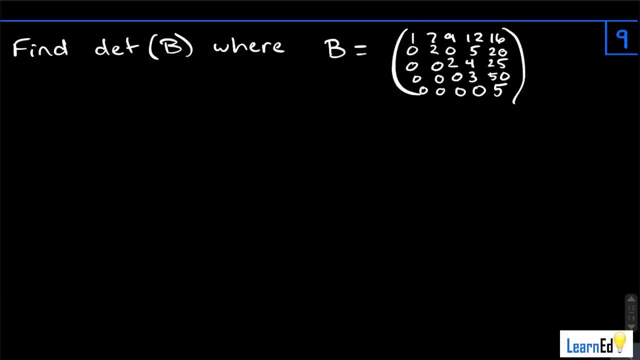 going to find the determinant of this is going to find the determinant of this is a lot simpler. okay, this is actually a a lot simpler. okay, this is actually a a lot simpler. okay, this is actually a pretty quick problem and the reason why pretty quick problem and the reason why. 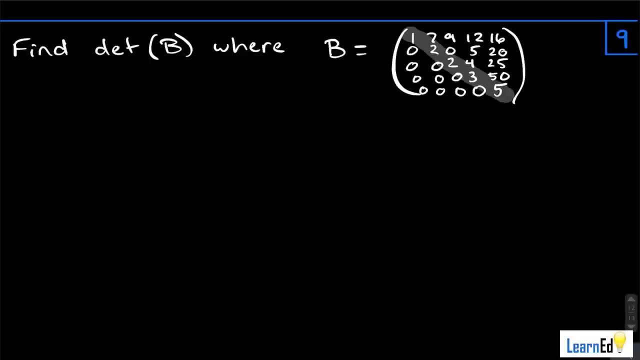 pretty quick problem, and the reason why is because, as you can see, I'll draw a. is because, as you can see, I'll draw a, is because, as you can see, I'll draw a. I'll highlight down the main diagonal. you, I'll highlight down the main diagonal, you. 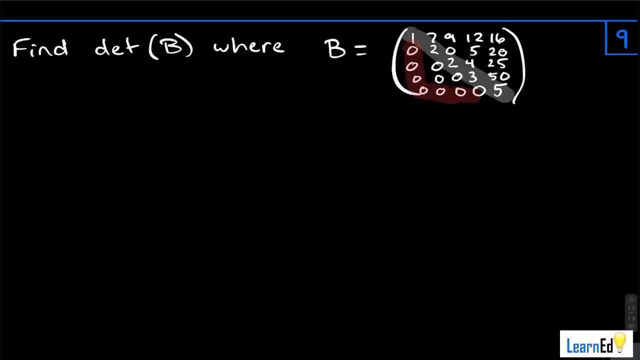 I'll highlight down the main diagonal. you can see that, all the other entries can see that, all the other entries can see that, all the other entries that are below the main diagonal or zero, that are below the main diagonal or zero, that are below the main diagonal or zero. what does that mean? well, it means that 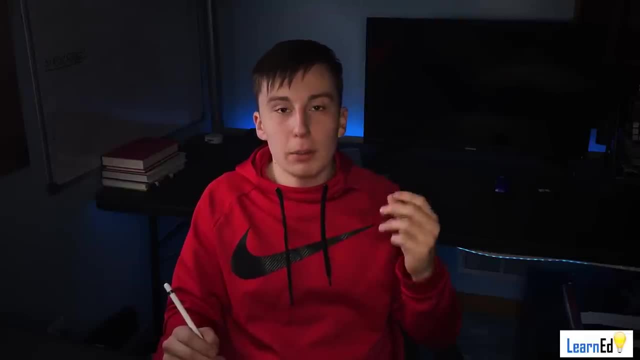 what does that mean? well, it means that. what does that mean? well, it means that this matrix is upper triangular. if it's, this matrix is upper triangular. if it's, this matrix is upper triangular. if it's upper triangular, then that means that upper triangular, then that means that. 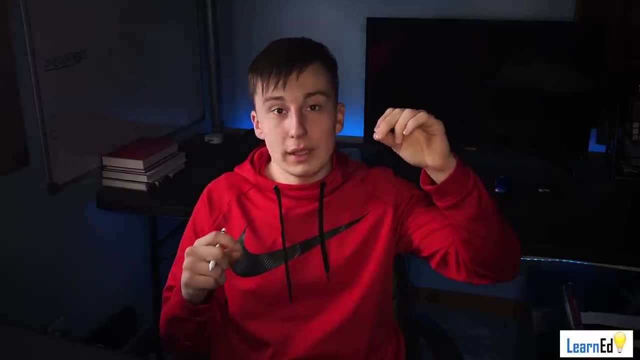 upper triangular, then that means that the determinant is just going to be all the determinant is just going to be all. the determinant is just going to be all the values down the diagonal multiplied, the values down the diagonal multiplied, the values down the diagonal multiplied together, and that's how you find the 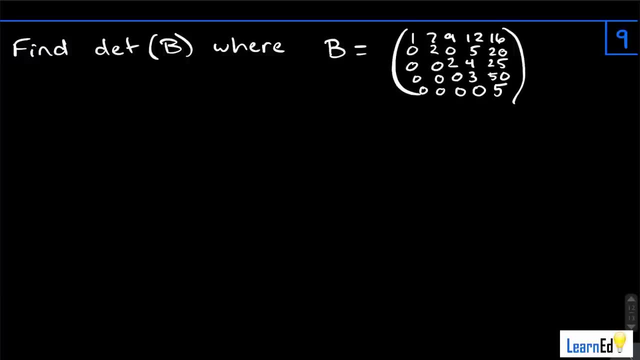 together and that's how you find the together and that's how you find the determinant. okay, so really nice, and I determinant. okay, so really nice, and I determinant. okay, so really nice. and I actually did have one of these problems, actually did have one of these problems. 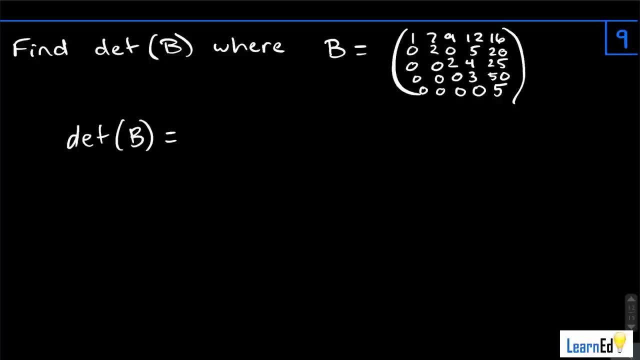 actually did have one of these problems on my final. so either the determinant of on my final so, either the determinant of on my final, so either the determinant of B is just going to be the values of the, B is just going to be the values of the. 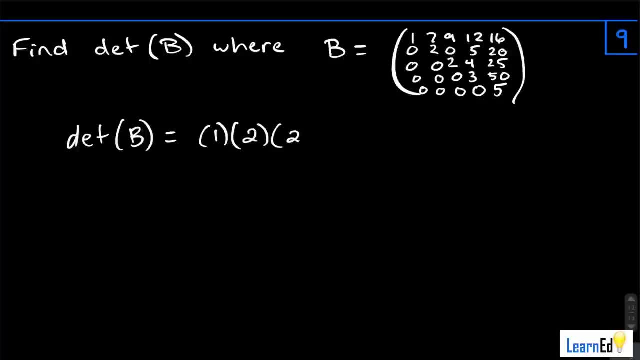 B is just going to be the values of the diagonal multiplied together. so we have a diagonal multiplied together. so we have a diagonal multiplied together. so we have a 1, 2, 2, 3 and a 5, right? so we have. we have 1, 2, 2, 3 and a 5, right? so we have. we have. 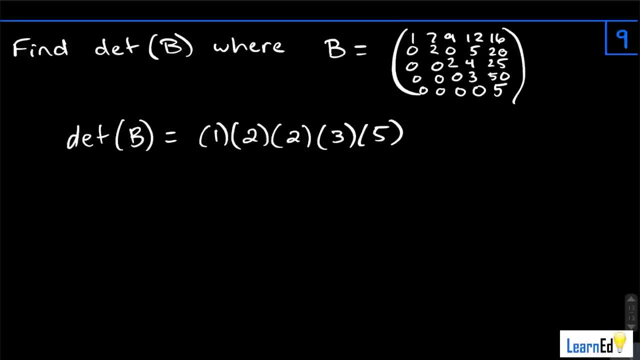 1, 2, 2, 3 and a 5, right? so we have: we have 5 values because we have a 5 by 5 matrix, 5 values, because we have a 5 by 5 matrix, 5 values because we have a 5 by 5 matrix, right, so we have 5, 5 pivots. you can. 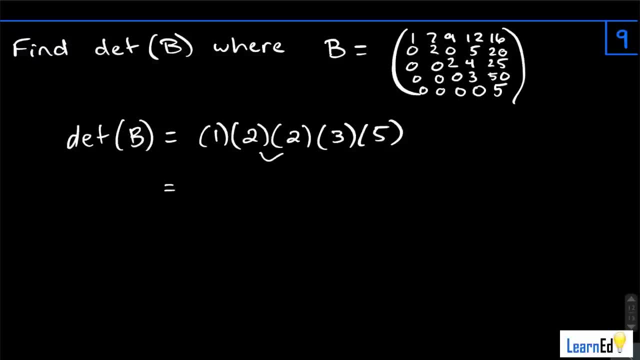 right, so we have 5, 5 pivots. you can right, so we have 5, 5 pivots. you can think of it that way, right, and so this think of it that way, right, and so this think of it that way, right, and so this is going to be 4 times. this 3 is going. 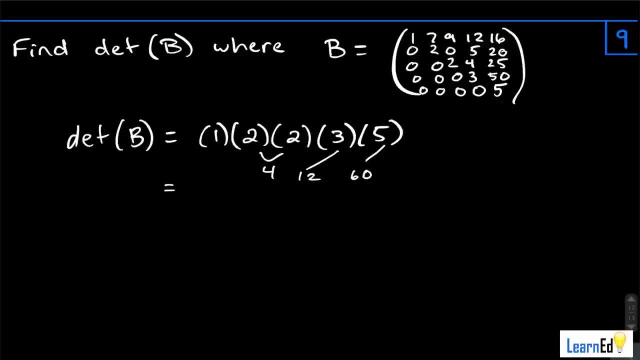 is going to be 4 times this 3 is going is going to be 4 times this 3 is going to be 12, and then times this 5 is going to be 12, and then times this 5 is going to be 12, and then times this 5 is going to be 60. okay, so we get our determinant. 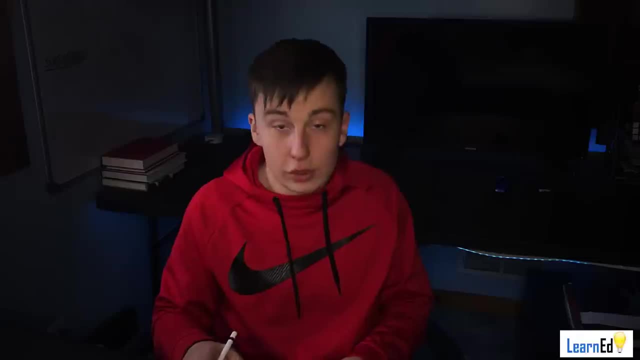 to be 60: okay, so we get our determinant to be 60: okay, so we get our determinant to be 60 okay, so really really nice. when to be 60: okay, so really really nice. when to be 60: okay, so really really nice when you have an upper triangular matrix and you have an upper triangular matrix and you have an upper triangular matrix and that's definitely something you want to, that's definitely something you want to. that's definitely something you want to check for before you go and do like three, check for before you go and do like three. 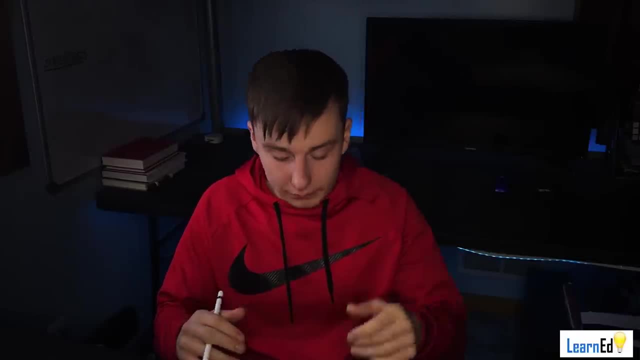 check for before you go and do like three cofactor expansions or even any cofactor expansions, or even any cofactor expansions, or even any cofactor expansions at all. so moving on, cofactor expansions at all. so moving on cofactor expansions at all. so moving on to our next problem, we're gonna shift. 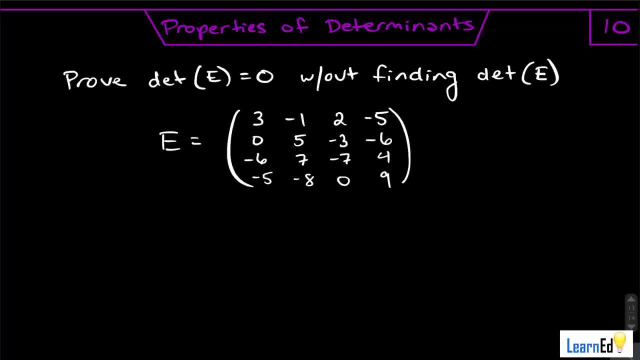 to our next problem. we're gonna shift to our next problem. we're gonna shift our focus to the properties of our focus, to the properties of our focus, to the properties of determinants. and for problem 10 we're determinants and for problem 10, we're. 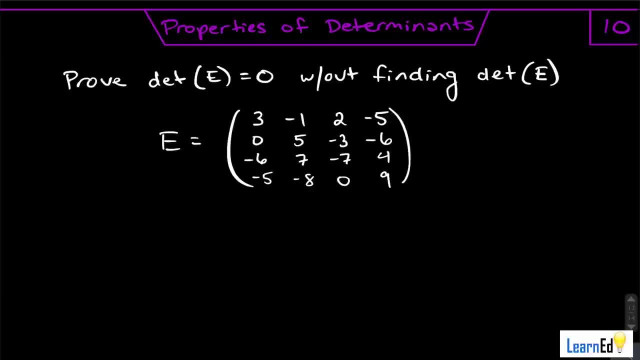 determinants and for problem 10, we're being asked to prove that the being asked to prove that the being asked to prove that the determinant of E equals zero without determinant of E equals zero, without determinant of E equals zero, without finding the actual determinant of E. okay, 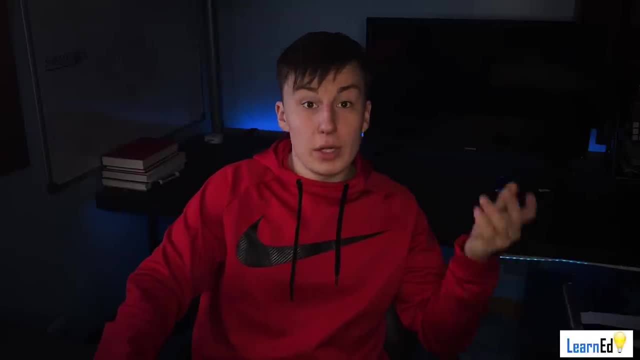 finding the actual determinant of E? okay. finding the actual determinant of E? okay. so how do we end up doing something like so? how do we end up doing something like so? how do we end up doing something like this? well, we know that. if a matrix is this, well, we know that if a matrix is: 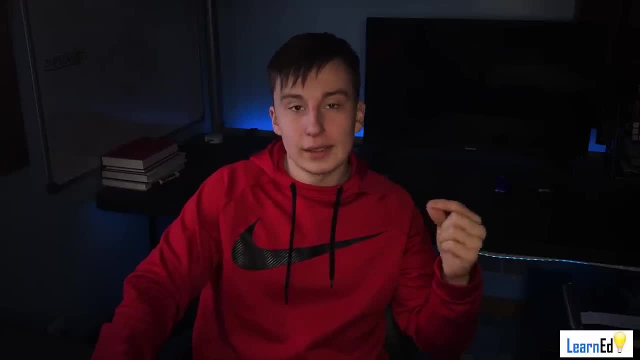 this. well, we know that if a matrix is linearly independent, its determinant is linearly independent. its determinant is linearly independent, its determinant is nonzero. and if it is linearly dependent, nonzero. and if it is linearly dependent- nonzero and if it is linearly dependent, the determinant of that matrix will be. 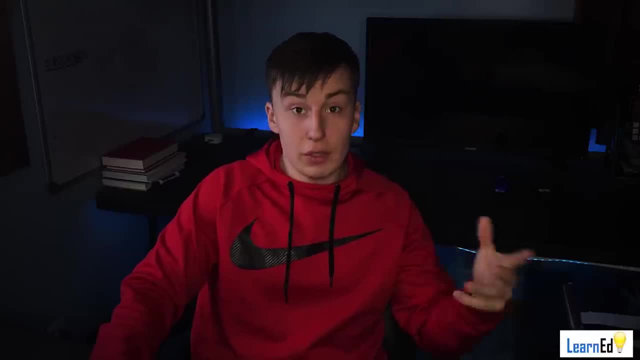 the determinant of that matrix will be. the determinant of that matrix will be zero, okay, and so all we have to do if we zero, okay, and so all we have to do if we zero, okay, and so all we have to do if we prove this matrix is linearly dependent. 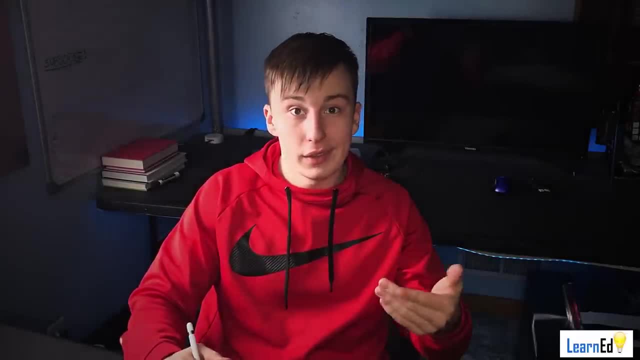 prove this matrix is linearly dependent. prove this matrix is linearly dependent. okay then, the determinant of it is zero. okay then, the determinant of it is zero. okay then, the determinant of it is zero. okay, so let's go to work on row. okay, so let's go to work on row. 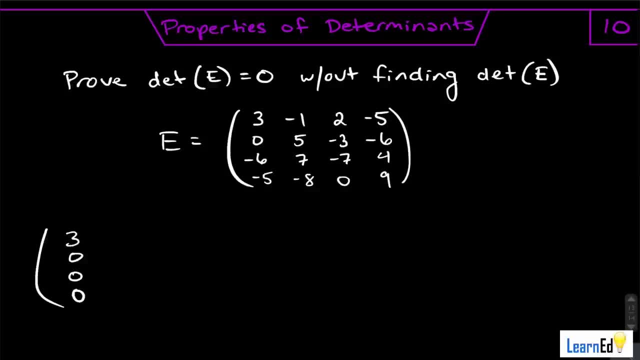 okay, so let's go to work on row. reducing right: that's how we prove that. reducing right: that's how we prove that. reducing right: that's how we prove that this thing is linearly dependent. okay, this thing is linearly dependent. okay, this thing is linearly dependent. okay. so we zero out all the entries below. 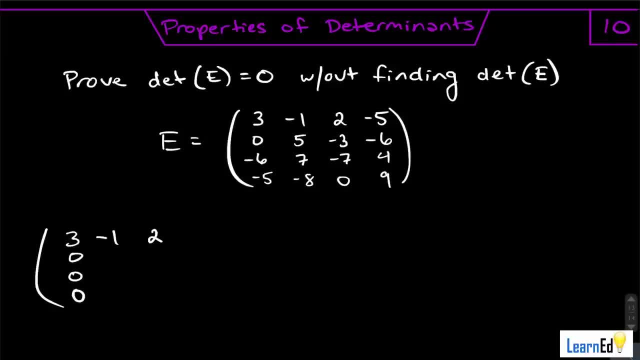 so we zero out all the entries below. so we zero out all the entries below our first pivot. and since that does not our first pivot, and since that does not our first pivot, and since that does not take any work to do that in the second, take any work to do that in the second. take any work to do that. in the second row, we can just keep all these values row. we can just keep all these values row. we can just keep all these values the same. so we have a 5 negative 3 the same. so we have a 5 negative 3. 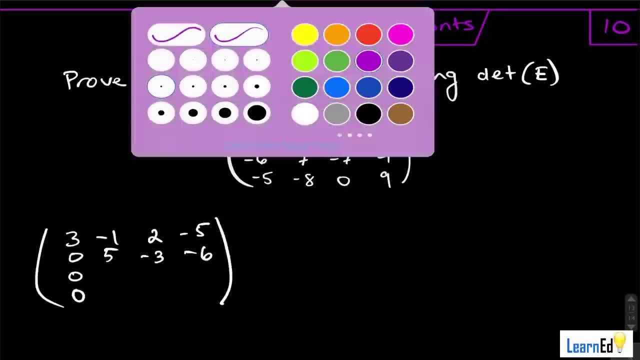 the same. so we have a 5 negative 3, negative, 6 and the only values will have negative 6 and the only values will have negative 6 and the only values will have to worry about changing are in the third. to worry about changing are in the third. 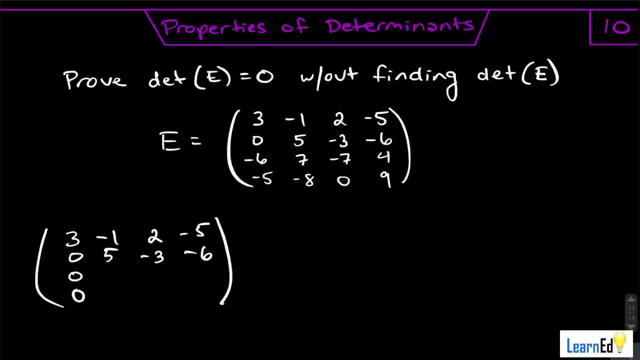 to worry about changing are in the third row, in the fourth row, so we have to row in the fourth row. so we have to row in the fourth row. so we have to multiply the first row by what. when we multiply the first row by what? when we 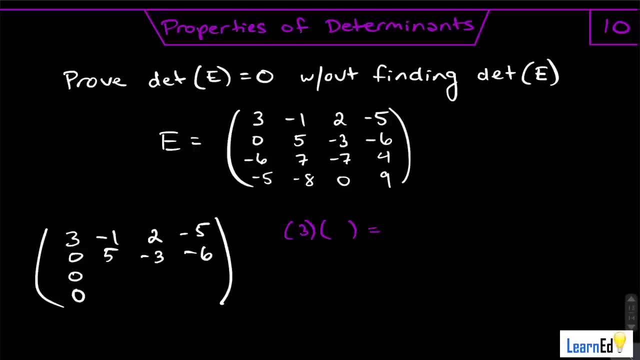 multiply the first row by what when we add negative 6, so equals what, and minus add negative 6, so equals what, and minus add negative 6, so equals what, and minus 6 equals 0. well, that value is going to. 6 equals 0. well, that value is going to. 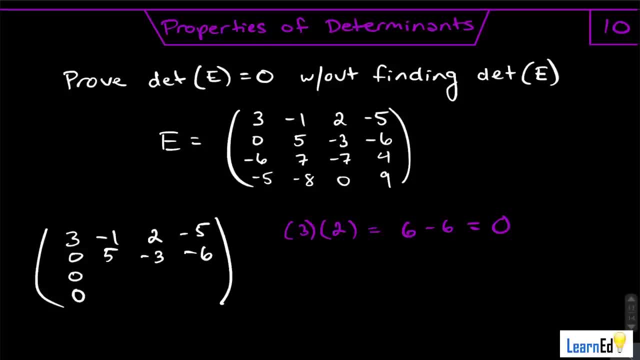 6 equals 0. well, that value is going to be 2, because then we get a 6 and 6 minus be 2, because then we get a 6 and 6 minus be 2, because then we get a 6 and 6 minus 6 is 0. so our multiplying factor is 2. we. 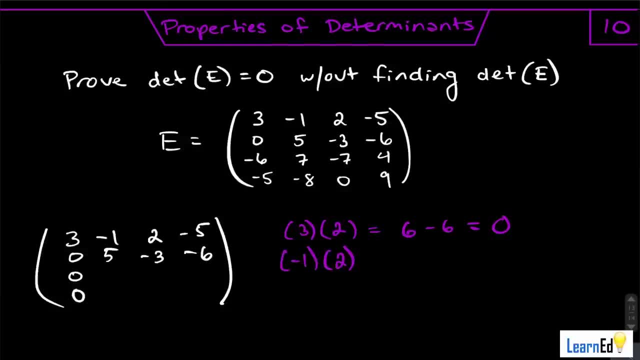 6 is 0, so our multiplying factor is 2. we 6 is 0, so our multiplying factor is 2. we multiply the first row by 2 negative 1. multiply the first row by 2 negative 1. multiply the first row by 2 negative 1 times 2 is negative 2. we add the 5 or. 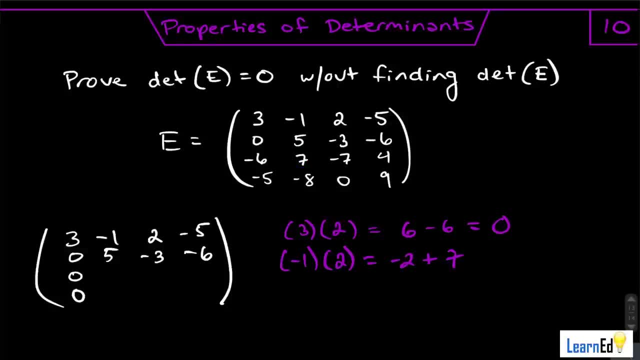 times 2 is negative 2, we add the 5. or times 2 is negative 2, we add the 5. or sorry, not at 5. we had these 7. that's sorry, not at 5. we had these 7. that's sorry, not at 5, we had these 7. that's right here. and we get 5. so we get a 5. 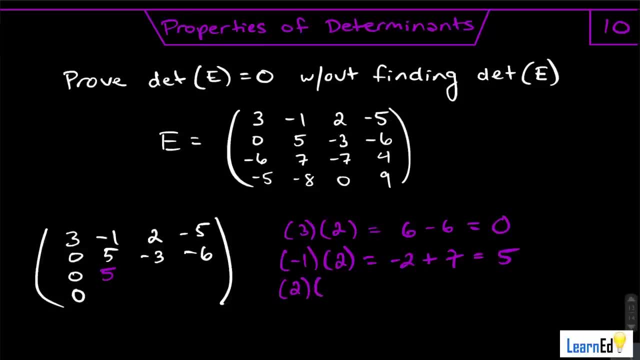 right here and we get 5. so we get a 5. right here and we get 5, so we get a 5 here. we do the same for the 2 to get 4 here. we do the same for the 2 to get 4. 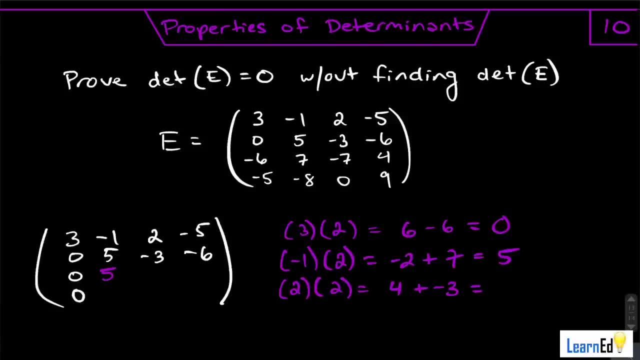 here we do the same for the 2 to get 4, and then we're going to add the negative, and then we're going to add the negative, and then we're going to add the negative. 3- that was there, and again I've looked. 3- that was there, and again I've looked. 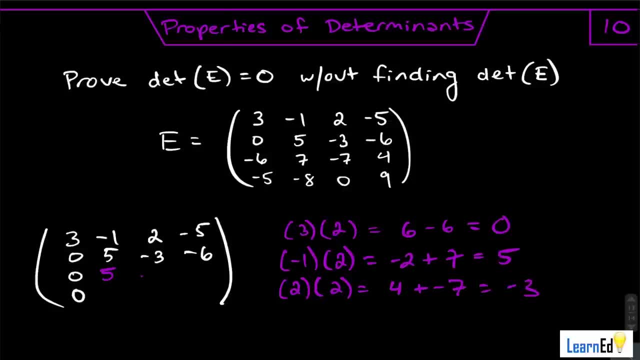 3. that was there. and again I've looked at the wrong row: negative 7: negative 3. at the wrong row: negative 7- negative 3. at the wrong row: negative 7: negative 3: great, all right starting off solid with. great, all right, starting off solid with. 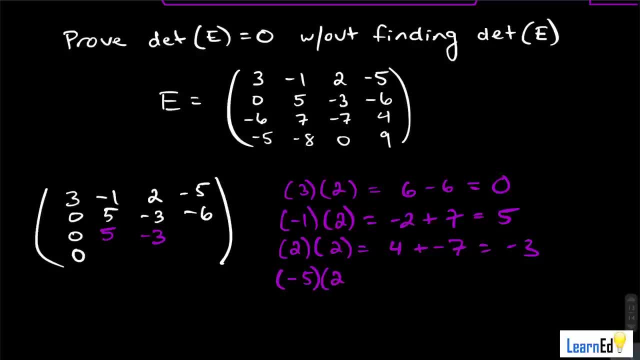 great, all right. starting off solid with this problem, I'll tell you so negative this problem. I'll tell you so negative this problem, I'll tell you so negative. 5 times 2 is negative 10, and then we add: 5 times 2 is negative 10, and then we add: 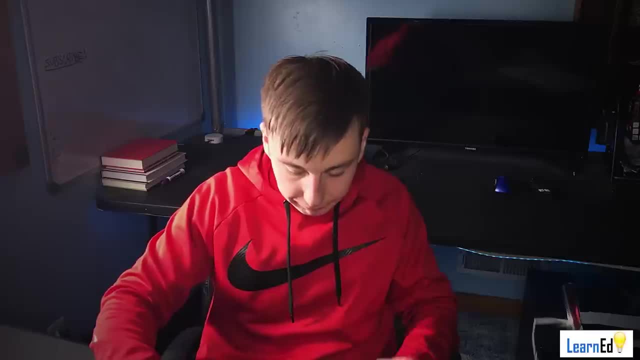 5 times 2 is negative 10. and then we add on 4 and we get negative 6. so what on 4 and we get negative 6. so what on 4 and we get negative 6. so what you'll notice here is that, well, our 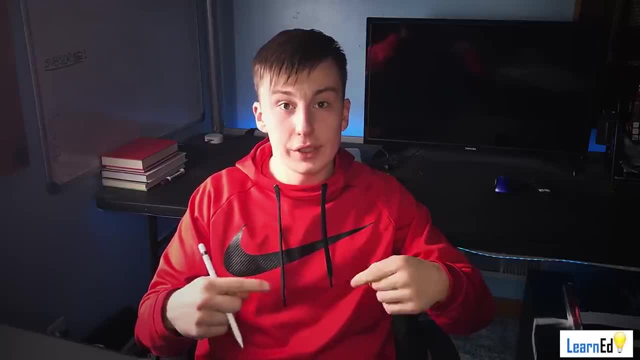 you'll notice here is that, well, our you'll notice here is that, well, our third bro is an exact copy of our second third bro is an exact copy of our second third bro is an exact copy of our second row. so we can just zero one of those. 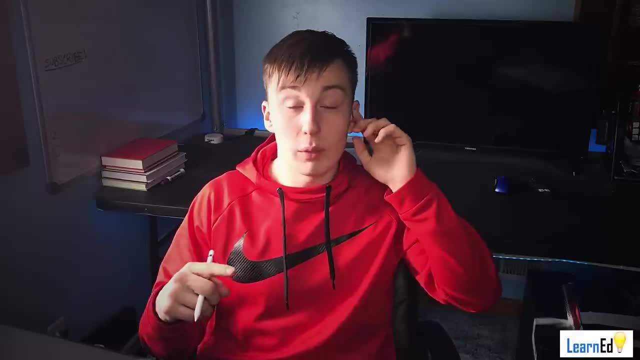 row so we can just zero one of those row. so we can just zero one of those rows off right by multiplying one of the rows off right, by multiplying one of the rows off right, by multiplying one of the rows by negative 1 and adding it to. 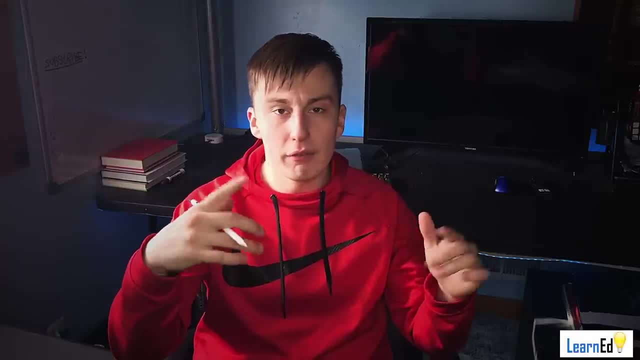 rows by negative 1, and adding it to rows by negative 1, and adding it to the other row, and then we have our zero row, the other row, and then we have our zero row, the other row, and then we have our zero row, and so this matrix will end up being: 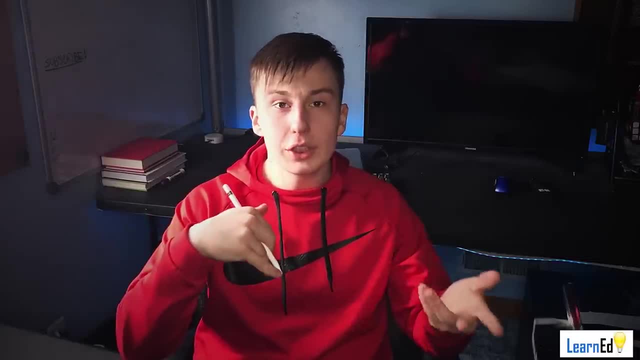 and so this matrix will end up being, and so this matrix will end up being linearly dependent. and so we know the linearly dependent, and so we know the linearly dependent. and so we know the determinant is zero. so let's just show. determinant is zero. so let's just show. 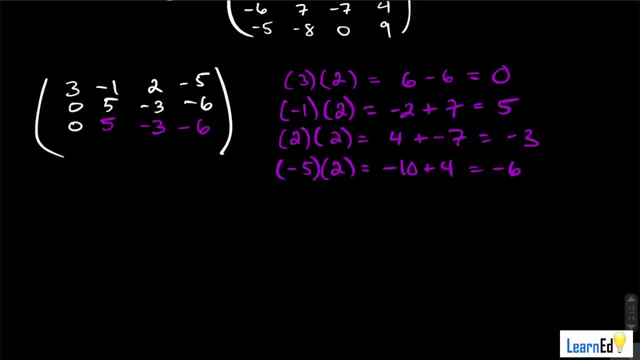 determinant is zero. so let's just show that quick and actually what we can do that quick and actually what we can do that quick and actually what we can do is make so we don't have to end up row is make so we don't have to end up row. 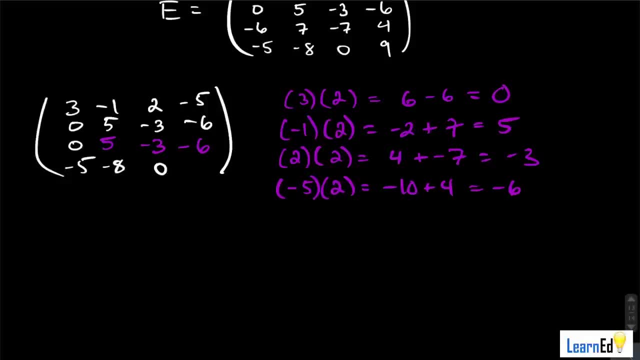 is make, so we don't have to end up row reducing anymore. we can just keep this reducing anymore. we can just keep this reducing anymore. we can just keep this row, row for the same. okay, so, we'd never row. row for the same. okay, so we'd never. 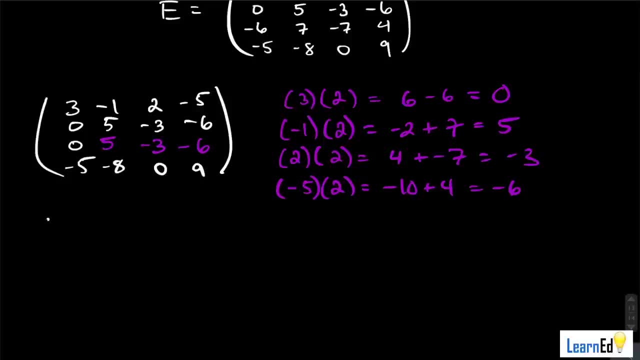 row. row for the same. okay, so we'd never even touched it, okay, and that's fine. even touched it, okay, and that's fine. even touched it, okay, and that's fine, because we know that we can represent, because we know that we can represent, because we know that we can represent this as a 3 negative, 1 2 negative, 5 0, 5. 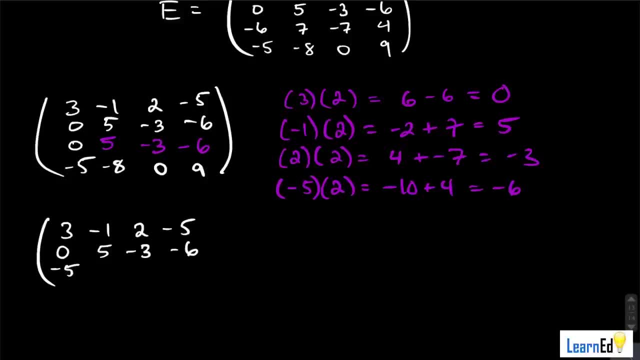 this as a 3 negative, 1 2 negative, 5 0, 5. this as a 3 negative, 1 2 negative. 5 0, 5 negative. 3 negative, 6. we can row swap. negative 3 negative, 6: we can row swap. 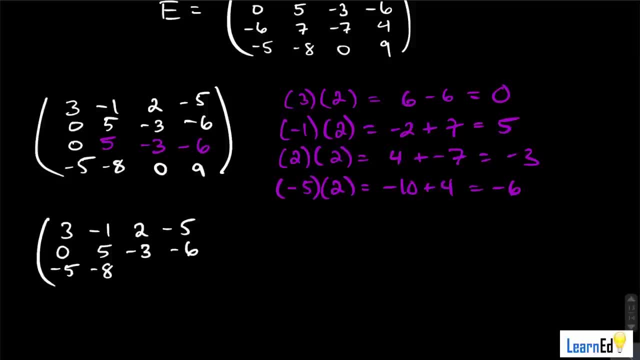 negative 3, negative 6. we can row swap because you know, I know, that most people, because you know, I know that most people, because you know, I know that most people will like to put the zeros to the bottom, will like to put the zeros to the bottom. 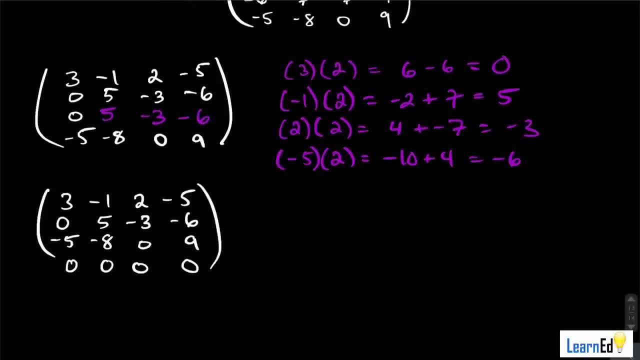 will like to put the zeros to the bottom, and that's exactly what we'll do. okay, so, and that's exactly what we'll do. okay, so, and that's exactly what we'll do. okay, so we can say, since this matrix is, we can say: since this matrix is, 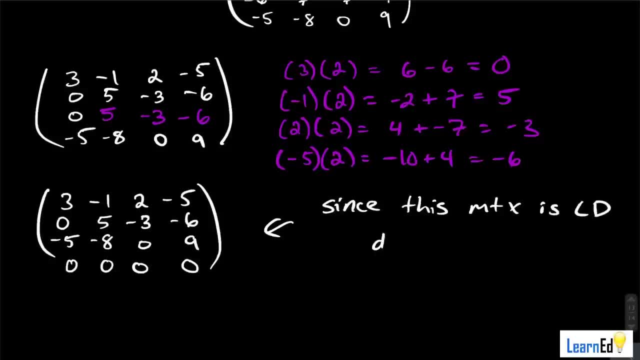 we can say: since this matrix is linearly dependent, the determinant of E linearly dependent, the determinant of E linearly dependent. the determinant of E equals 0. okay, and that's all you have to. equals 0: okay, and that's all you have to. equals 0. okay, and that's all you have to do for that problem. so now, moving on to 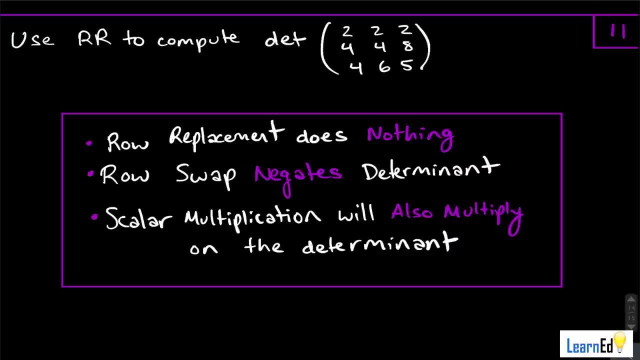 do for that problem. so now moving on to do for that problem. so now moving on to problem 11. we're going to be asked to problem 11. we're going to be asked to problem 11. we're going to be asked to use row reduction to compute the. 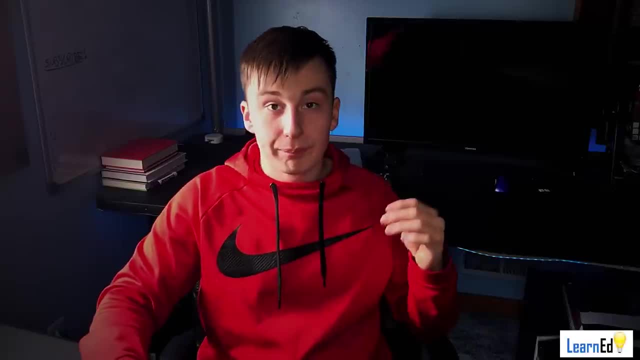 use row reduction to compute the. use row reduction to compute the determinant of this: 3 by 3 matrix: okay. determinant of this: 3 by 3 matrix- okay. determinant of this: 3 by 3 matrix: okay. and a big note about row reduction to. and a big note about row reduction to. 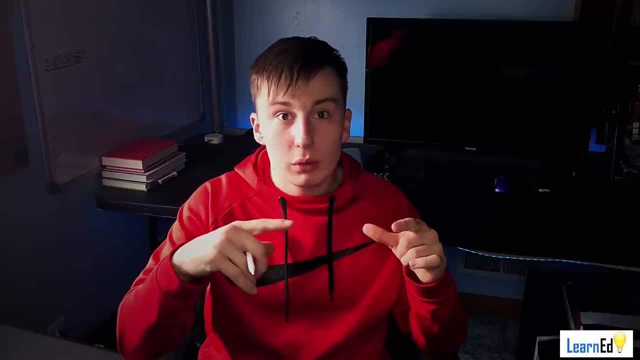 and a big note about row reduction to compute determinants. it actually can be compute determinants. it actually can be compute determinants. it actually can be really helpful when you don't well, when really helpful when you don't well, when really helpful when you don't well, when you have like a matrix, that's gonna be. you have like a matrix that's gonna be. you have like a matrix that's gonna be really ugly to do a cofactor expansion- really ugly to do a cofactor expansion- really ugly to do a cofactor expansion with. sometimes it's just easier to get with, sometimes it's just easier to get. 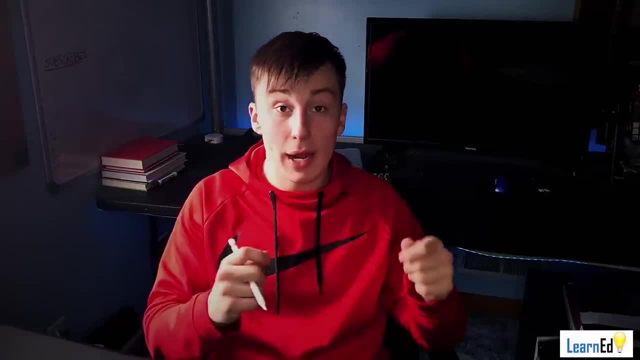 with. sometimes it's just easier to get your determinant okay. and how does that your determinant okay? and how does that your determinant okay? and how does that determinant relate back to your determinant, relate back to your determinant, relate back to your determinant of this matrix that we have? 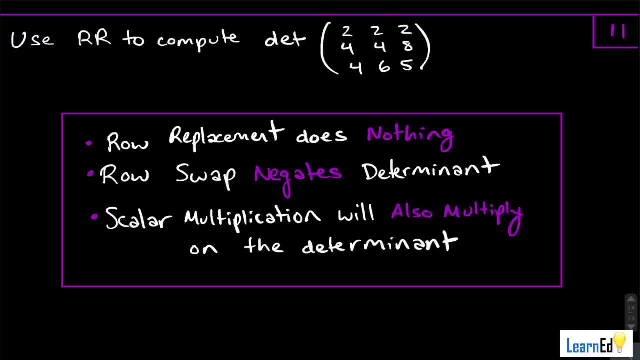 determinant of this matrix that we have, determinant of this matrix that we have here. well, here, here's how. if you perform here. well, here, here's how. if you perform here. well, here, here's how. if you perform a row replacement, as you will reduce, okay, a row replacement as you will reduce, okay. 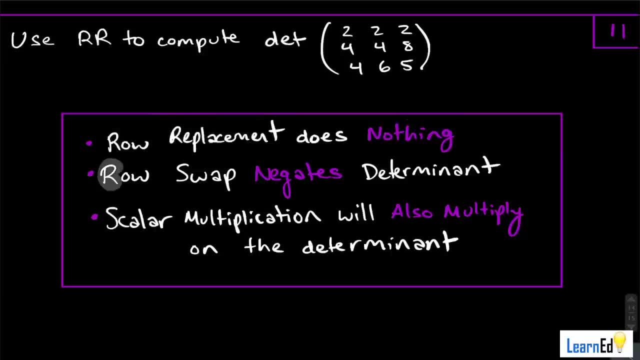 a row replacement as you will reduce. okay, that will do nothing to change the. that will do nothing to change the. that will do nothing to change the determinant. if you do a row swap, you determinant. if you do a row swap, you determinant. if you do a row swap, you will negate the determinant. okay, and if 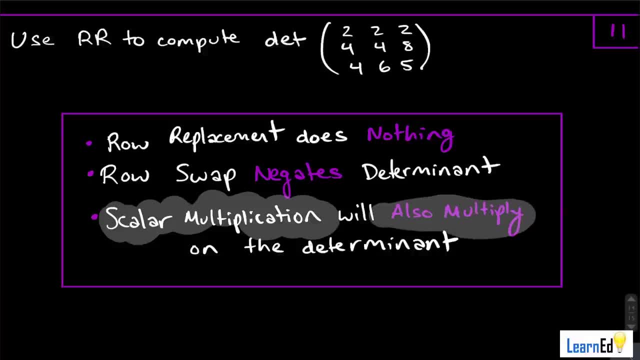 will negate the determinant okay, and if will negate the determinant okay, and if you perform a scalar multiplication, you, you perform a scalar multiplication, you, you perform a scalar multiplication. you will also multiply that on to the will also multiply that on to the will also multiply that on to the determinant okay, and the scalar. 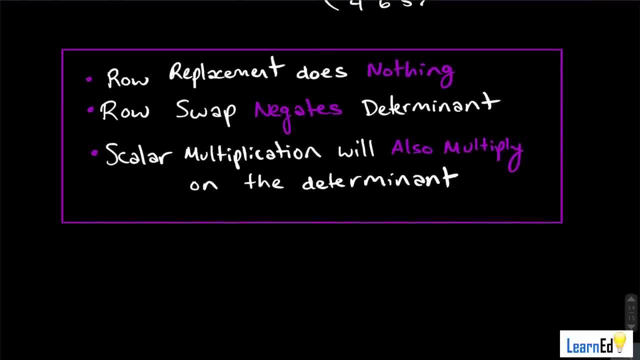 determinant okay, and the scalar determinant okay, and the scalar multiplication one there. I kind of made multiplication one there. I kind of made multiplication one there. I kind of made that a little bit vague, so what? I'm that a little bit vague, so what? I'm that a little bit vague. so what I'm going to do is actually show you that. 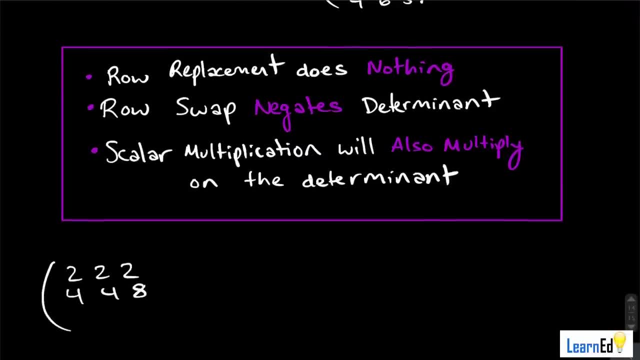 going to do is actually show you that. going to do is actually show you that, right now, we're going to call this. right now, we're going to call this. right now, we're going to call this matrix a and what we're going to do: matrix a and what we're going to do. 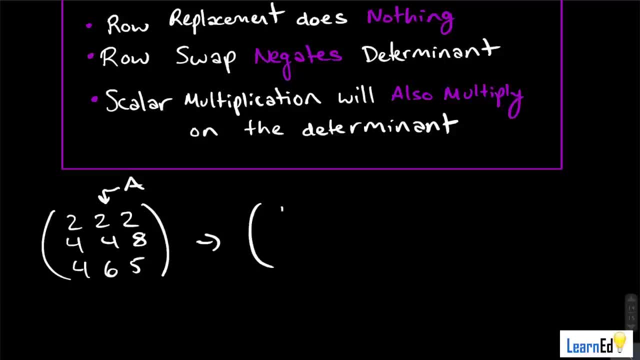 matrix a. and what we're going to do right now is perform a scalar. right now is perform a scalar right now is perform a scalar multiplication. so we're going to just multiplication, so we're going to just multiplication, so we're going to just multiply by 1 half on the top, okay, and 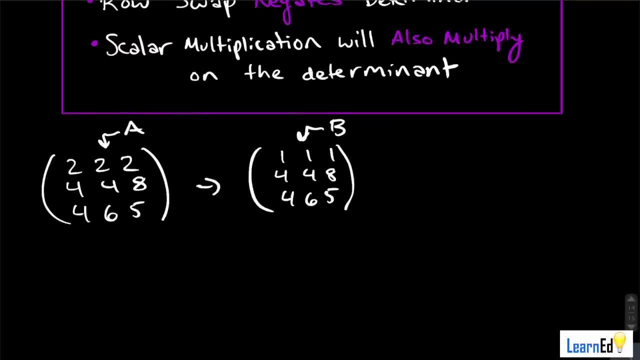 multiply by 1 half on the top, okay, and multiply by 1 half on the top, okay. and so now we get a matrix B, okay and here. so now we get a matrix B, okay and here. so now we get a matrix B, okay, and here, since we did a scalar multiplication, we 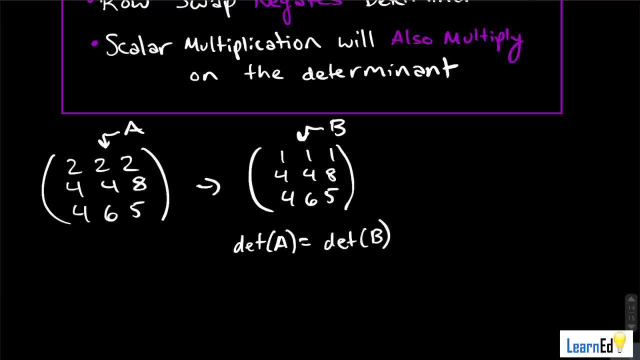 since we did a scalar multiplication, we, since we did a scalar multiplication, we get that instead of the determinant of a. get that instead of the determinant of a. get that instead of the determinant of a. equaling the determinant of B. it's going, equaling the determinant of B. it's going. 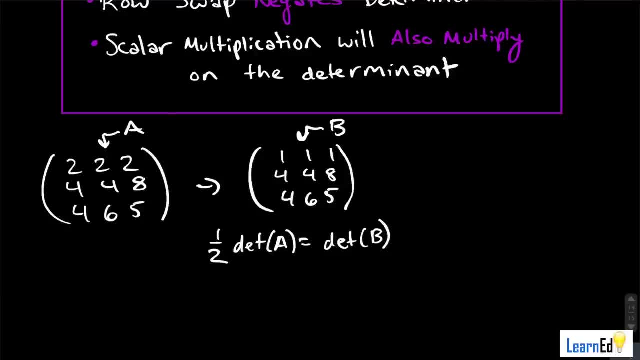 equaling the determinant of B. it's going to be 1 half of the determinant of a. to be 1 half of the determinant of a equals the determinant of B. okay, so we equals the determinant of B. okay, so we equals the determinant of B. okay, so we just pull out a 1 half. okay, meaning that: 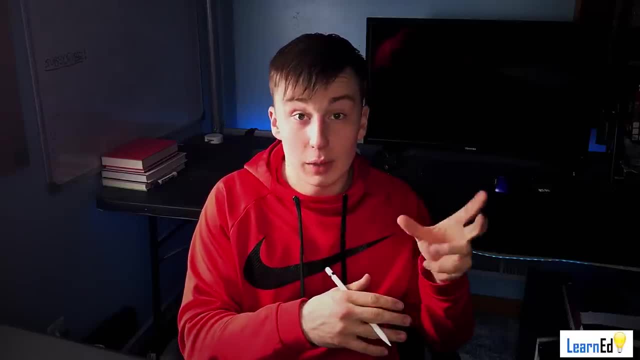 just pull out a 1 half okay. meaning that: just pull out a 1 half okay. meaning that we now have ones in our top row and we, we now have ones in our top row and we, we now have ones in our top row and we just multiply that onto the determinant. 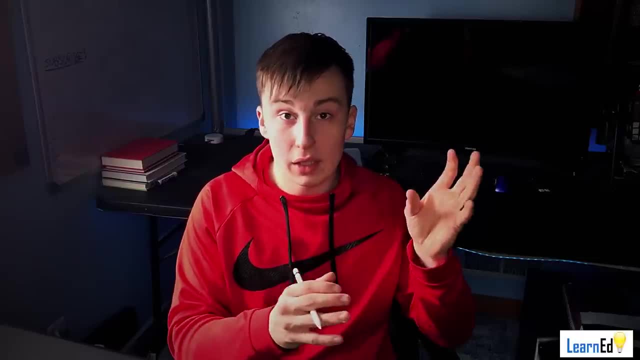 just multiply that onto the determinant. just multiply that onto the determinant of our original matrix. okay, you got to of our original matrix. okay, you got to of our original matrix. okay, you got to remember. that's the the turn we're remember, that's the the turn we're. 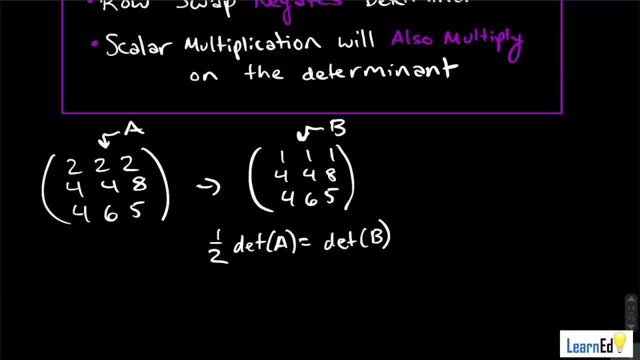 remember, that's the the turn. we're doing all that stuff to the determinant, doing all that stuff to the determinant, doing all that stuff to the determinant of the original matrix. okay, so now of the determinant of the original matrix. okay, so now of the determinant of the original matrix. okay, so now moving on to the next step. 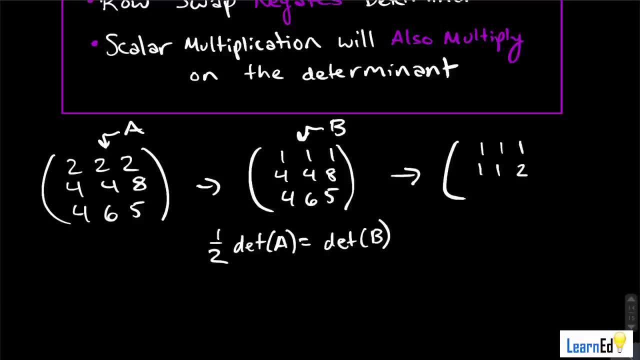 moving on to the next step. moving on to the next step. we're just going to do the same exact. we're just going to do the same exact. we're just going to do the same exact thing, but for the second row, so we're thing. but for the second row, so we're. 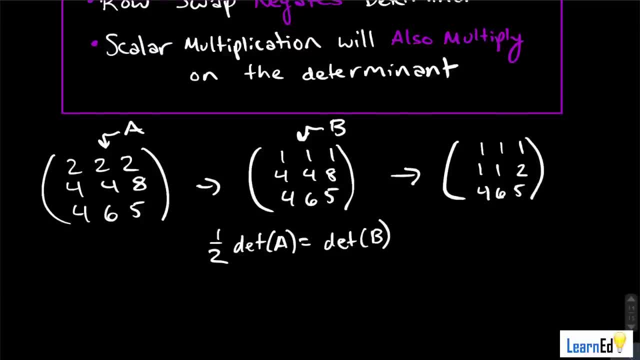 thing, but for the second row. so we're gonna take out a 1 4th, okay, and we'll gonna take out a 1 4th, okay, and we'll gonna take out a 1 4th, okay, and we'll call this matrix C. so now we get that 1. 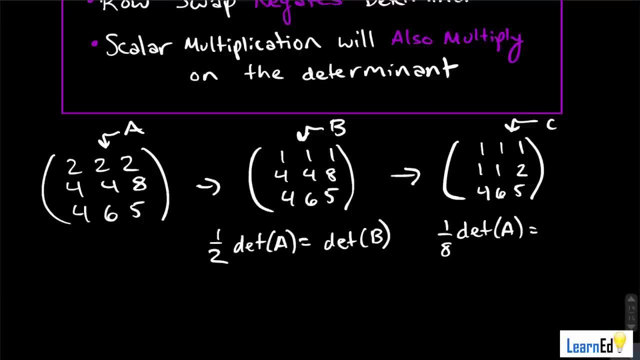 call this matrix C, so now we get that. 1. call this matrix C, so now we get that 1, 8th times the determinant of a equals 8th times the determinant of a equals 8th times the determinant of a equals the determinant of C. okay, because we 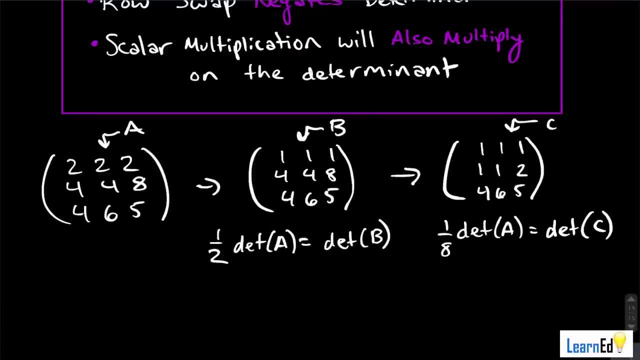 the determinant of a equals C. okay, because we the determinant of a equals C. okay, because we already had a 1 half there. we take already had a 1 half there. we take already had a 1 half there, we take out a 1- 4th and now that becomes 1- 8th, all. out a 1 4th, and now that becomes 1 8th. all out a 1 4th, and now that becomes 1 8th. all we have to do now is row reduce, and we have to do now is row reduce and. 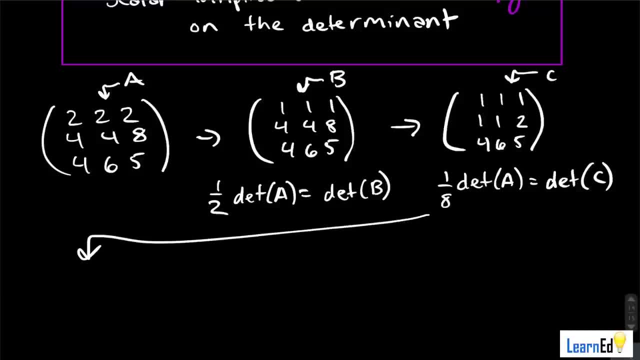 we have to do now is row reduce and we will get much closer to a row echelon. we will get much closer to a row echelon. we will get much closer to a row echelon. form okay, so we have a. we have ones on. form okay, so we have a, we have ones on. 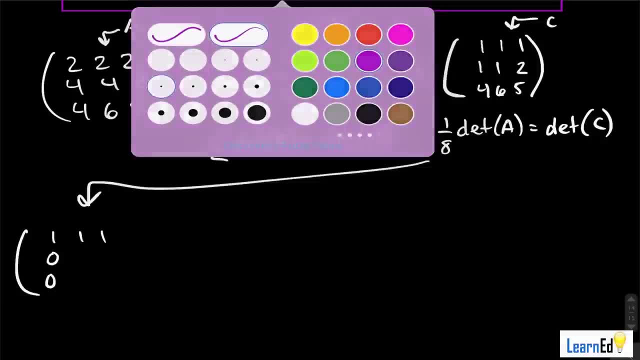 form: okay. so we have a. we have ones on the top. we're going to zero out the the top. we're going to zero out the the top. we're going to zero out the entries below the first pivot and to do entries below the first pivot and to do. 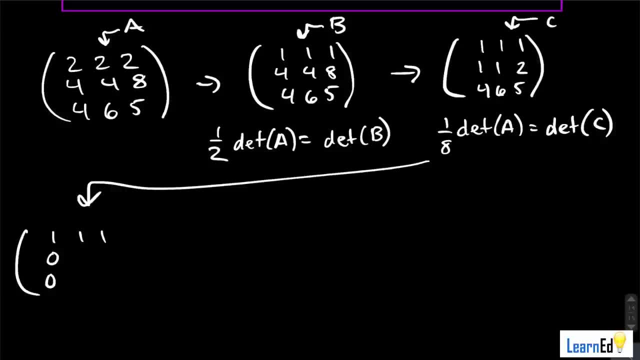 entries below the first pivot. and to do that first off, to get the second row to that first off, to get the second row to that first off, to get the second row to be 0 in the first column, we have to be 0 in the first column, we have to. 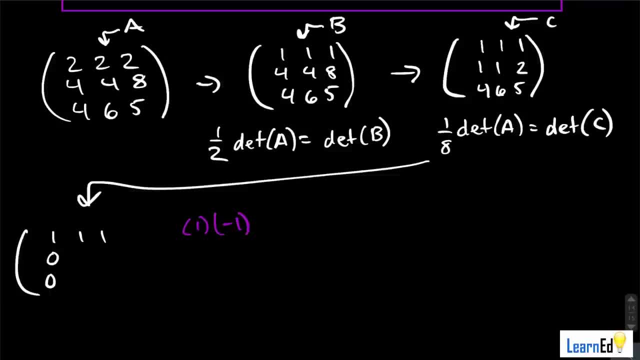 be 0 in the first column, we have to multiply the top row by negative 1- okay. multiply the top row by negative 1- okay. multiply the top row by negative 1- okay, and we'll get negative 1. here we add to and we'll get negative 1. here we add to. 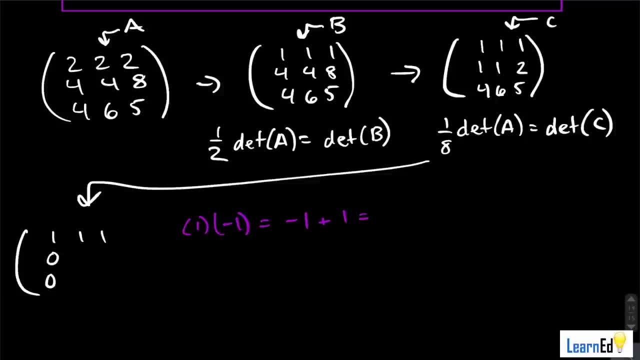 and we'll get negative 1 here. we add to that one that was already in the second, that one that was already in the second, that one that was already in the second row, first column, and we get 0 now since row first column and we get 0 now since. 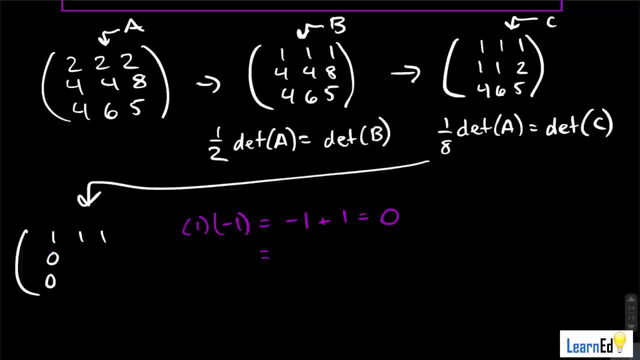 row, first column, and we get 0. now, since all of these values are 1, every single, all of these values are 1, every single, all of these values are 1, every single time. we do this, it's going to be time we do this, it's going to be. time we do this, it's going to be negative 1 and we're just gonna add on negative 1 and we're just gonna add on negative 1 and we're just gonna add on. so basically, we're just going to be. so, basically, we're just going to be. 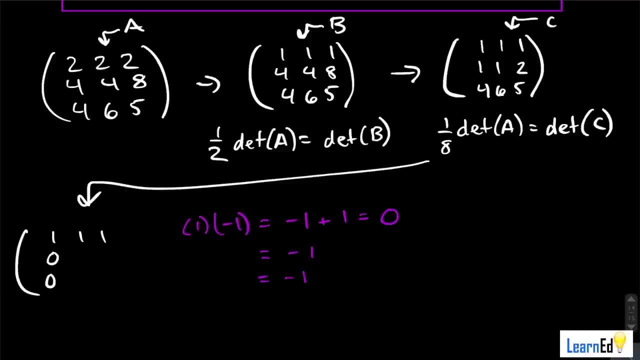 so basically, we're just going to be subtracting negative 1 from the from the subtracting negative 1 from the from the subtracting negative 1 from the from the second row. so we'll get a 0 here and a second row. so we'll get a 0 here and a. 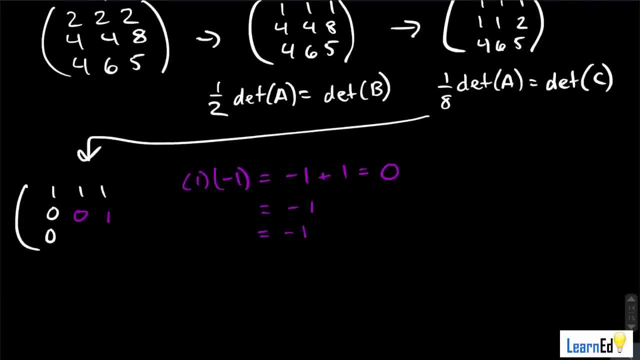 second row. so we'll get a 0 here and a 1 here. okay, so next we will do the same 1 here. okay, so next we will do the same 1 here. okay, so next we will do the same exact thing, but for row 3 and there. 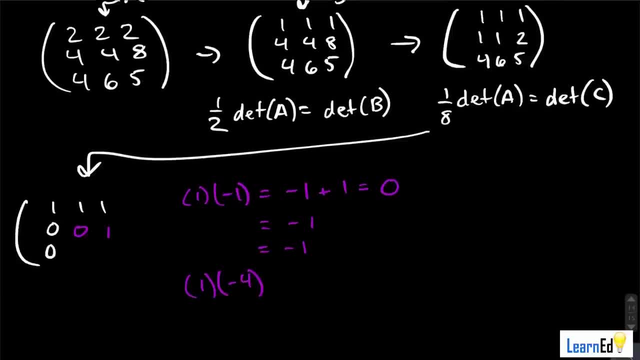 exact thing but for row 3. and there: exact thing but for row 3. and there we'll have to multiply by negative 4 on. we'll have to multiply by negative 4 on. we'll have to multiply by negative 4 on our first row. okay, so we're just going. 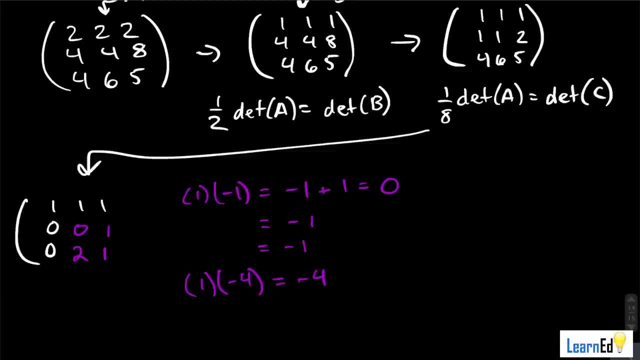 our first row. okay, so we're just going. our first row. okay, so we're just going to be subtracting by negative 4, and so to be subtracting by negative 4, and so to be subtracting by negative 4, and so we get 2 and 1. okay, so here, since we 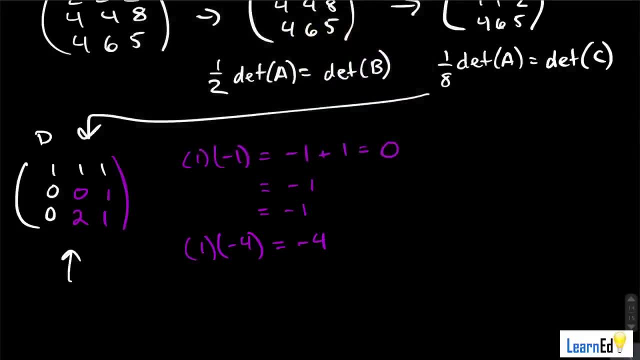 we get 2 and 1. okay. so here, since we we get 2 and 1. okay. so here, since we just did a row replacement, we know that, just did a row replacement. we know that just did a row replacement. we know that if we call this matrix D, the 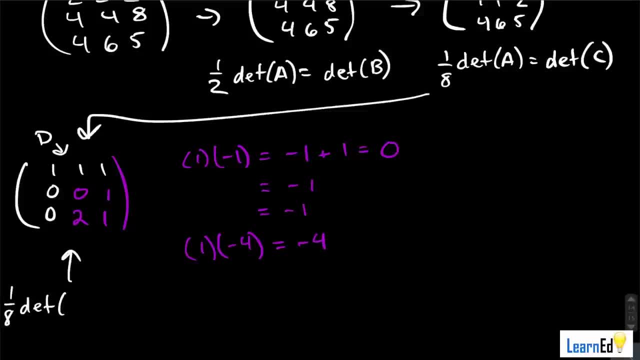 if we call this matrix D, the. if we call this matrix D, the determinant 1 half sorry, 1, 8 times the determinant 1 half sorry, 1, 8 times the determinant 1 half sorry, 1, 8 times the determinant of a is equal to the. 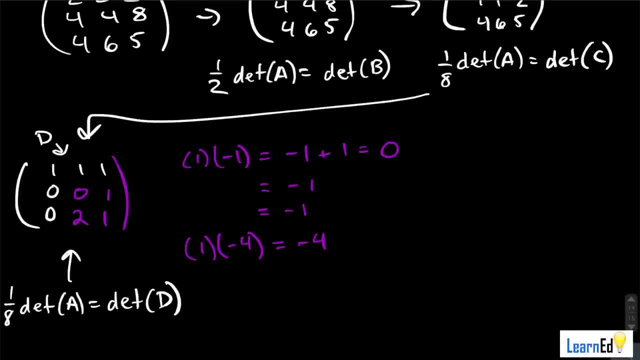 determinant of a is equal to the determinant of a is equal to the determinant of D, and then performing a determinant of D, and then performing a determinant of D, and then performing a row swap. okay, and this is gonna get a row swap. okay, and this is gonna get a. 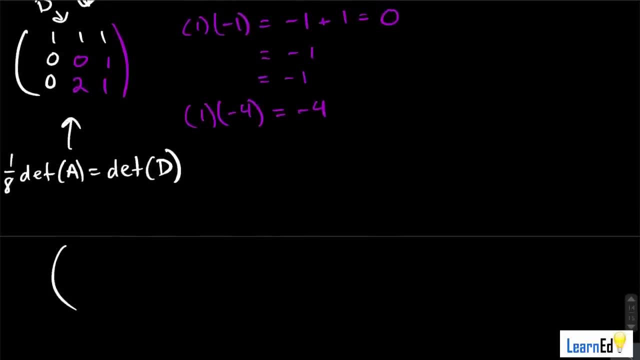 row swap. okay, and this is gonna get a little bit messy, so I'll just actually little bit messy, so I'll just actually little bit messy, so I'll just actually go down here. we'll go 1: 1 1 0 2. 1 0 0 1. go down here we'll go 1 1 1 0 2, 1 0 0 1. go down here, we'll go 1 1 1 0 2 1 0 0 1. so we did a row swap and what that's going. 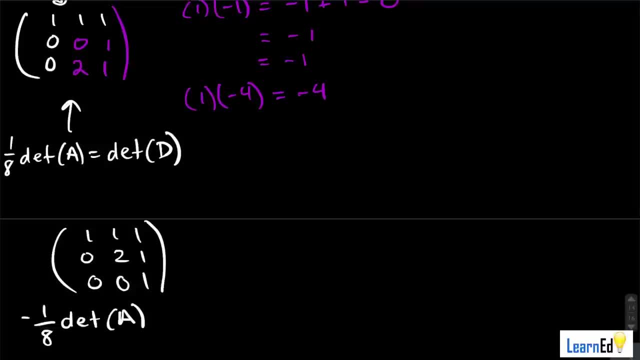 so we did a row swap and what that's going. so we did a row swap and what that's going to do is make it so negative. 1 8 to do is make it so negative. 1 8 to do is make it so negative. 1, 8 times. the determinant of a is equal to the. 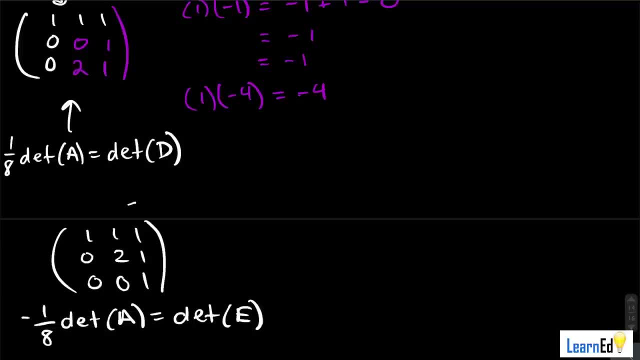 times the determinant of a is equal to the times the determinant of a is equal to the determinants of e, and we'll call determinants of e and we'll call determinants of e, and we'll call this matrix e, and now we have the upper. 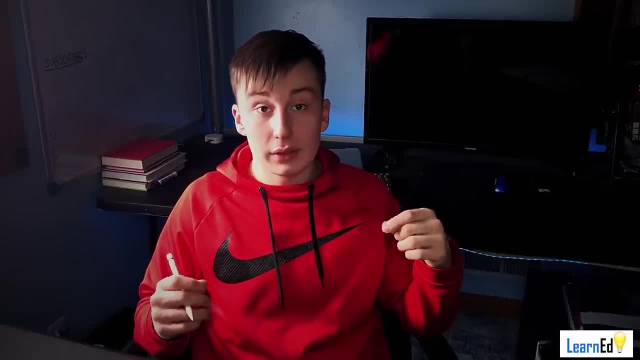 this matrix e, and now we have the upper, this matrix e, and now we have the upper triangular matrix. if we multiply the triangular matrix, if we multiply the triangular matrix, if we multiply the entries in the diagonal together, we end entries in the diagonal together. we end entries in the diagonal together. we end up getting our determinant of e. okay so, 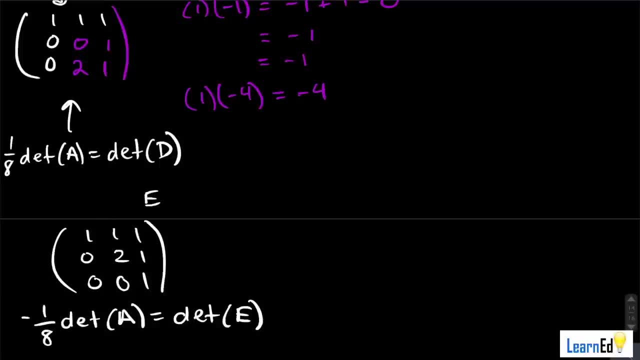 up getting our determinant of e- okay, so up getting our determinant of e- okay, so and sorry. I've been drawing some pretty and sorry. I've been drawing some pretty and sorry. I've been drawing some pretty cruddy arrows. that's still bad. hang on, cruddy arrows. that's still bad, hang on. 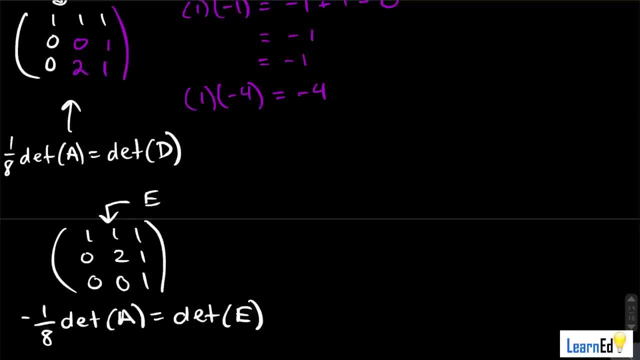 cruddy arrows. that's still bad. hang on, I'm gonna fix, there we go. so the I'm gonna fix there we go. so the I'm gonna fix there we go. so the determinant of e is equal to 1 times 2. determinant of e is equal to 1 times 2. 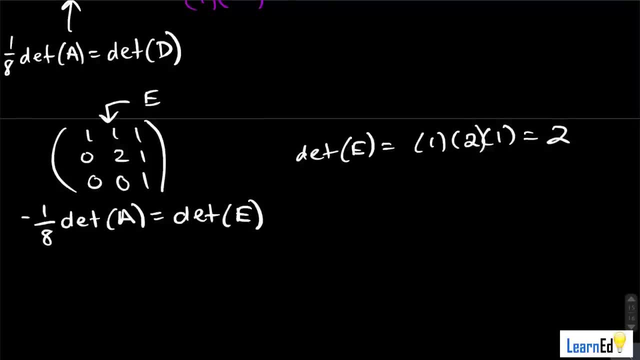 determinant of e is equal to 1 times 2 times 1 and that's equal to 2. so now we times 1 and that's equal to 2. so now we times 1 and that's equal to 2. so now we have that negative 1 8 times the. 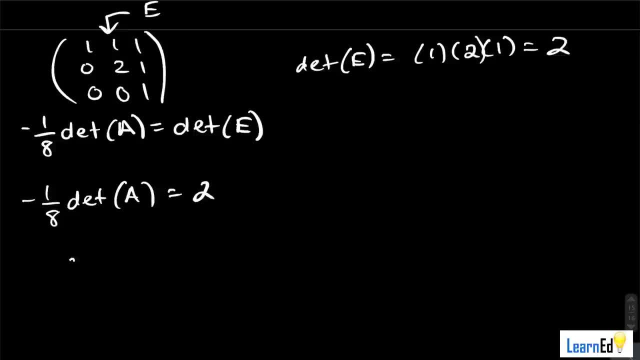 have that negative 1, 8 times. the have that negative 1, 8 times the determinant of a is equal to 2, and so we determinant of a is equal to 2, and so we determinant of a is equal to 2, and so we get that the determinant of a is equal. 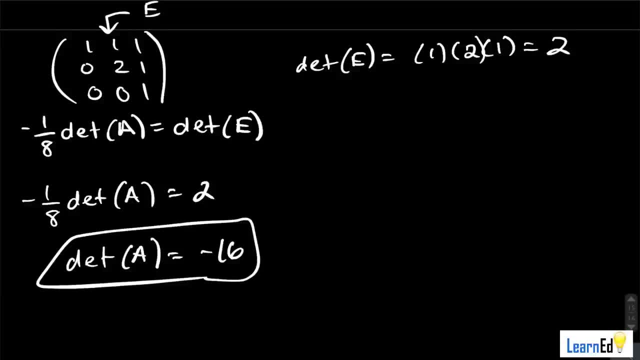 get that the determinant of a is equal to negative 16. okay, so it can be a bit to negative 16. okay so it can be a bit to negative 16. okay so it can be a bit of a process, but as you get better at of a process, but as you get better at. 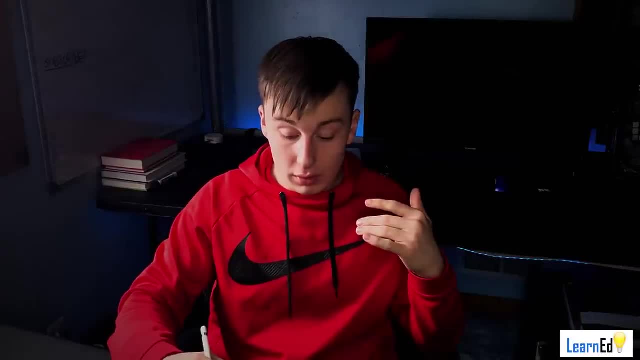 of a process. but as you get better at this and you start, you know skipping this and you start, you know skipping this and you start, you know skipping more steps like you could have done, the more steps like you could have done, the more steps like you could have done, the scalar multiplication steps. we did two. 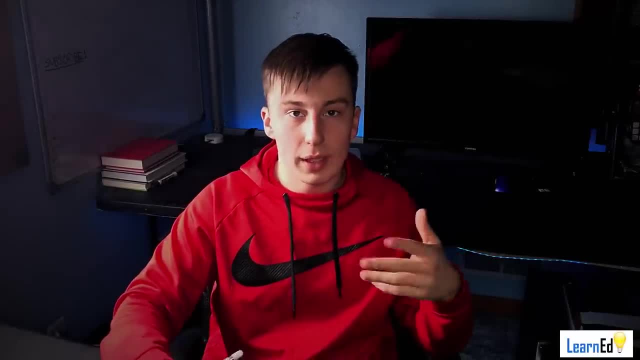 scalar multiplication steps. we did two scalar multiplication steps. we did two of those. you could have done those, all of those. you could have done those, all of those. you could have done those all at once. and you know the row swap kind at once, and you know the row swap kind. 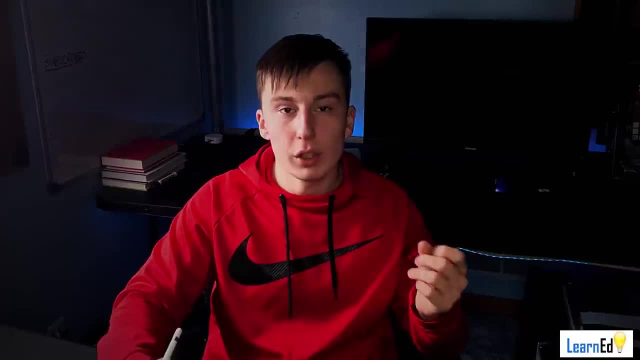 at once and you know the row swap kind of just throws your through your head a of those. you could have done those all at once and you know the row swap kind of just throws your through your head a lot quicker than I did it. so as you start, 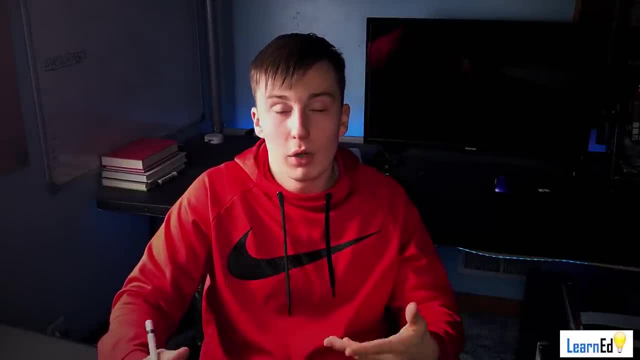 lot quicker than I did it. so as you start lot quicker than I did it, so as you start to do that faster and faster, this to do that faster and faster, this to do that faster and faster, this actually becomes more of and more, and actually becomes more of and more, and. 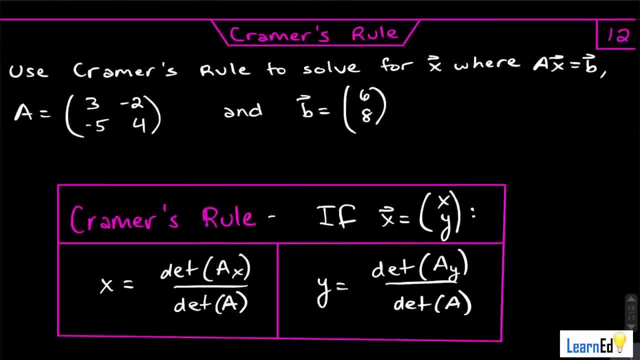 actually becomes more of and more and more of a feasible method. so now we're more of a feasible method. so now we're more of a feasible method. so now we're going to move on to our final problem. going to move on to our final problem, going to move on to our final problem, which is on Kramer's rule. okay, so for. 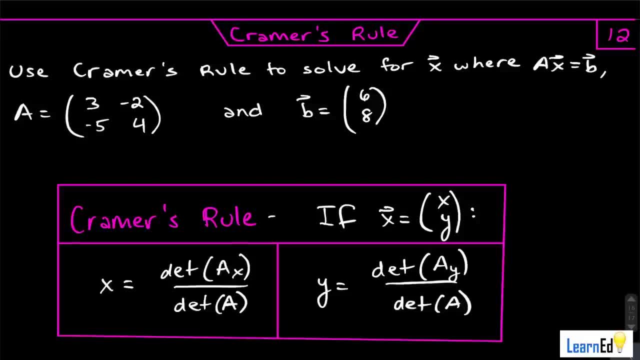 which is on Kramer's rule, okay. so for which is on Kramer's rule, okay. so for problem 12, we're being asked to use problem 12. we're being asked to use problem 12. we're being asked to use Kramer's rule to solve for the vector X. 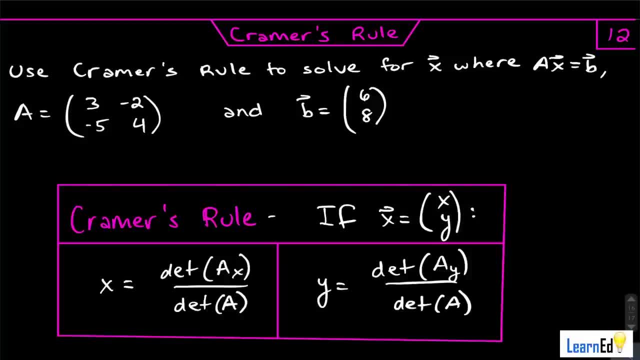 Kramer's rule to solve for the vector X. Kramer's rule to solve for the vector X, where ax equals B and we have our a where ax equals B and we have our a where ax equals B and we have our a, which is a 2 by 2 matrix, and B, which is: 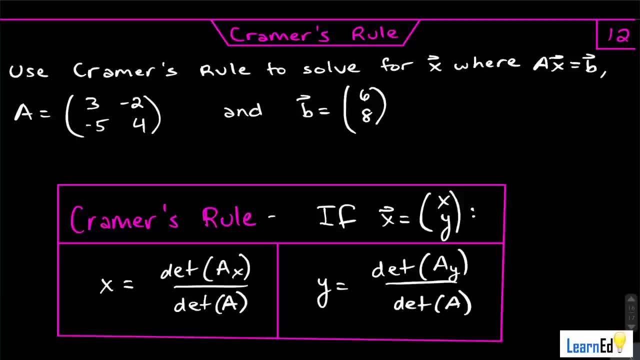 which is a 2 by 2 matrix and B, which is, which is a 2 by 2 matrix and B, which is a two-dimensional vector. so Kramer's a two-dimensional vector. so Kramer's a two-dimensional vector. so Kramer's rule. Kramer's rule is something that 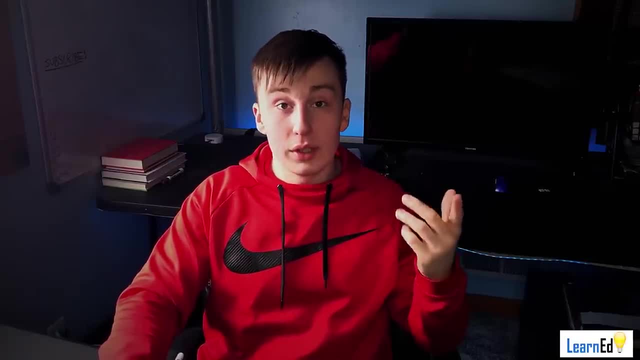 rule Kramer's rule is something. that rule Kramer's rule is something that we're actually doing right now in my. we're actually doing right now in my. we're actually doing right now in my ordinary differential equations class. ordinary differential equations class. ordinary differential equations class. we're actually using Kramer's rule to 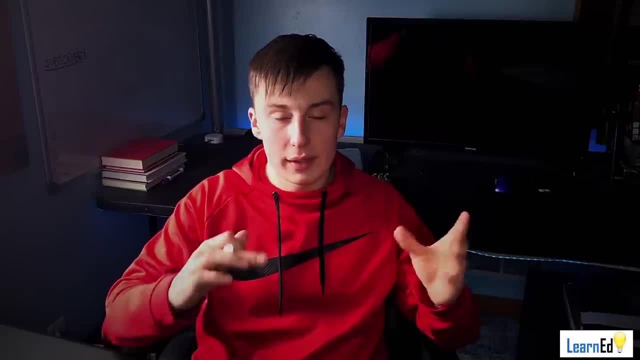 we're actually using Kramer's rule to. we're actually using Kramer's rule to solve a system of linear equations. solve a system of linear equations, solve a system of linear equations- that's really really gross. and this, that's really really gross. and this, that's really really gross. and this system of linear equations actually ties. 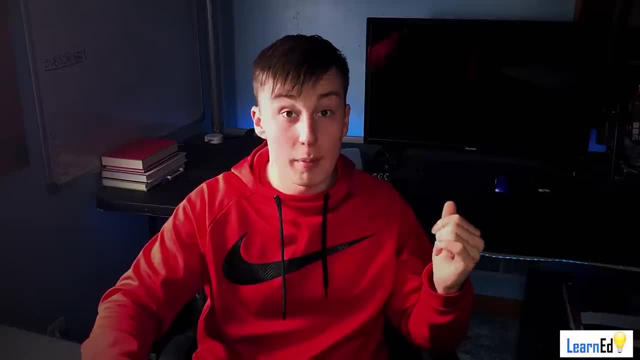 system of linear equations actually ties, system of linear equations actually ties into differential equations. so that's a into differential equations, so that's a into differential equations. so that's a whole nother topic, which I am definitely whole nother topic, which I am definitely whole nother topic, which I am definitely not going to explain right now because 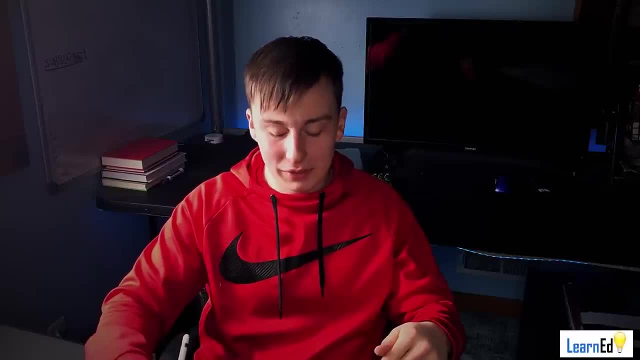 not going to explain right now. because not going to explain right now? because I'm learning it myself, and because this I'm learning it myself, and because this I'm learning it myself, and because this is a linear algebra final review, so is a linear algebra final review. so 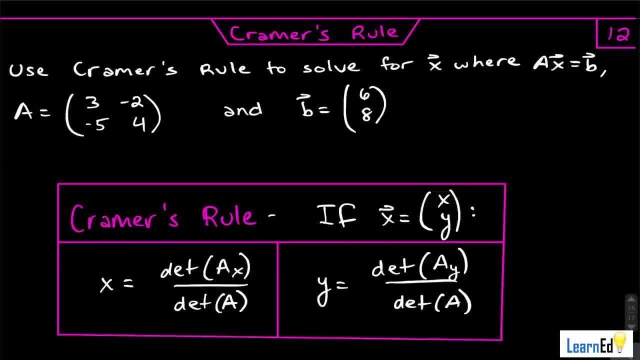 is a linear algebra, final review. so anyways, let's get into what Kramer's. anyways, let's get into what Kramer's. anyways, let's get into what Kramer's rule actually is telling you. so rule actually is telling you so rule actually is telling you so. Kramer's rule basically says that if you 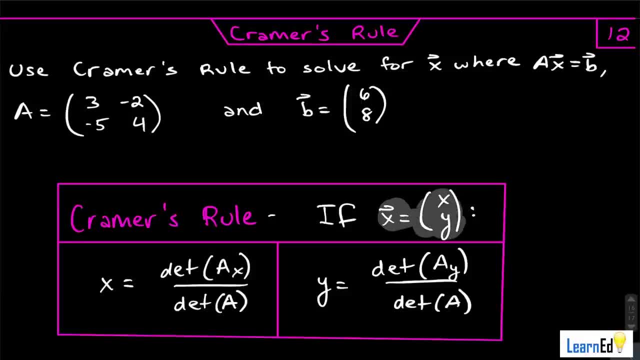 Kramer's rule basically says that if you Kramer's rule basically says that if you have a vector X and it is components, have a vector X and it is components, have a vector X and it is components, its components are X and Y. okay, and this. its components are X and Y. okay, and this. 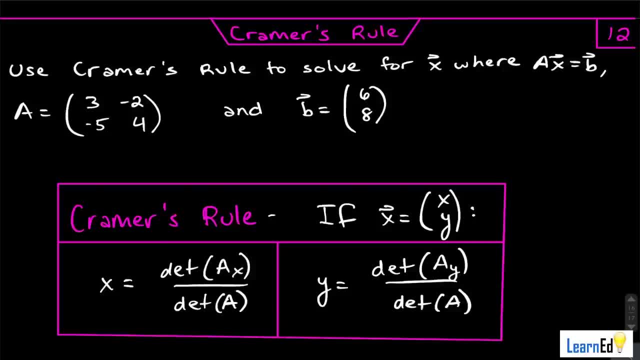 its components are X and Y. okay, and this works for two-dimensional or first, works for two-dimensional or first, works for two-dimensional or first for three-dimensional, and extra for three-dimensional and extra for three-dimensional and extra dimensional vectors, as well that your dimensional vectors, as well that your. 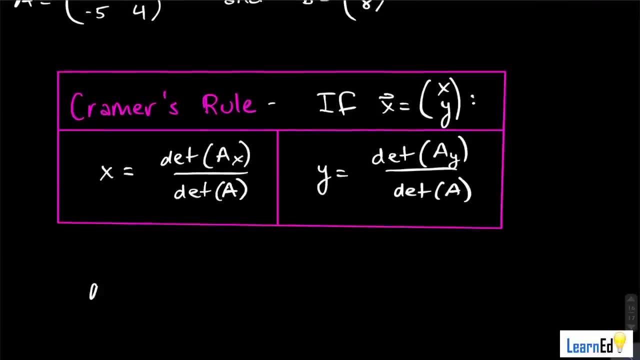 dimensional vectors as well, that your determinant of a. now, you're probably determinant of a. now, you're probably determinant of a. now, you're probably wondering, well, what is this determinant? wondering well, what is this determinant? wondering, well, what is this determinant of ax? mean, okay, what is this ax? even. 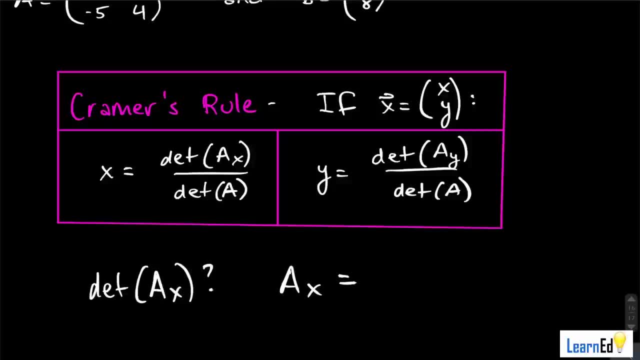 of ax mean: okay, what is this ax? even of ax mean okay, what is this ax even standing for? well, basically, what ax standing for well, basically what ax standing for well, basically, what ax means is that you have your matrix. a means is that you have your matrix a. 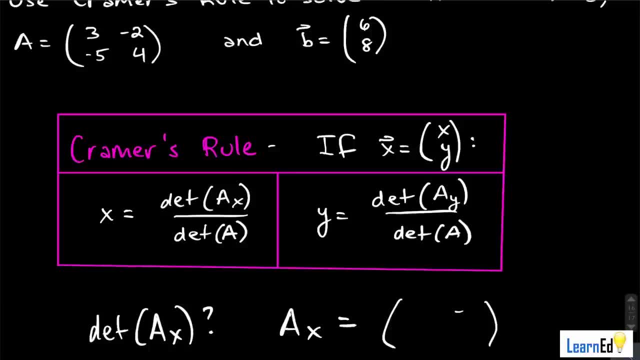 means is that you have your matrix a okay and you have your regular Y column okay and you have your regular Y column okay and you have your regular Y column. in this case, our Y column is negative 2. in this case, our Y column is negative 2. 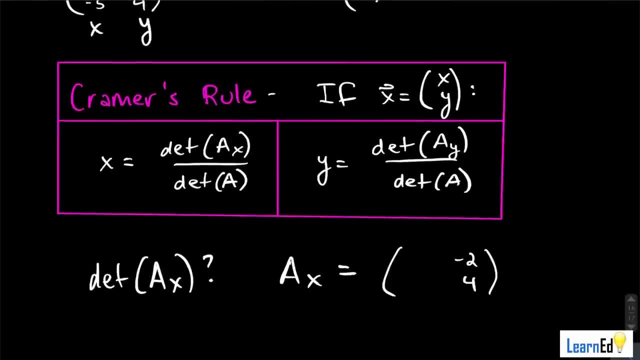 in this case, our Y column is negative. 2, 4 right- this is our Y column, but our X- 4 right- this is our Y column, but our X- 4 right- this is our Y column, but our X column gets replaced with the actual column. gets replaced with the actual. 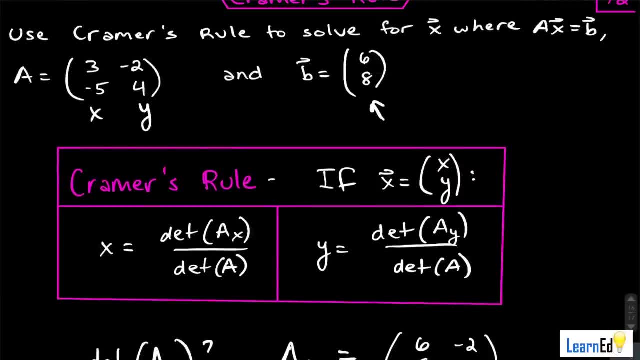 column gets replaced with the actual two-dimensional vector that we're using two-dimensional vector, that we're using two-dimensional vector that we're using to solve this system of linear equations, to solve this system of linear equations, to solve this system of linear equations. right, so that's our B vector and our B. 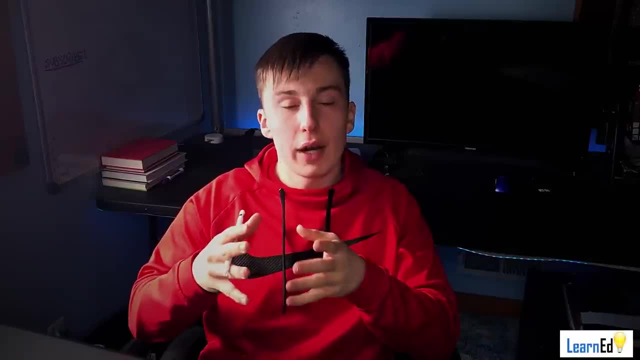 right. so that's our B vector and our B right. so that's our B vector. and our B vector gets replaced for the X column vector. gets replaced for the X column vector. gets replaced for the X column. similarly for a Y: our, our B vector gets. similarly for a Y. our, our B vector gets: 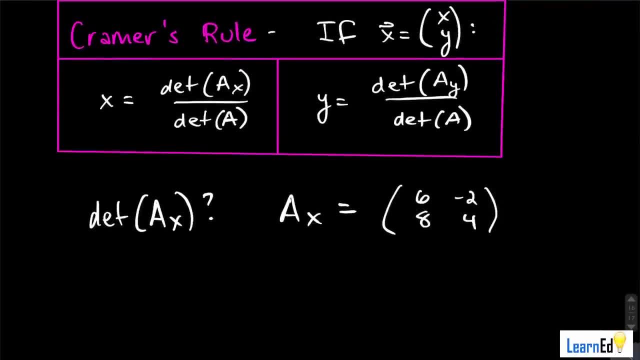 similarly for a Y, our, our B vector gets replaced in the Y column, and then we find replaced in the Y column, and then we find replaced in the Y column, and then we find the determinant like that, okay, so we the determinant like that. okay, so we, the determinant like that. okay, so we would get the a Y equals, not 68, we would. 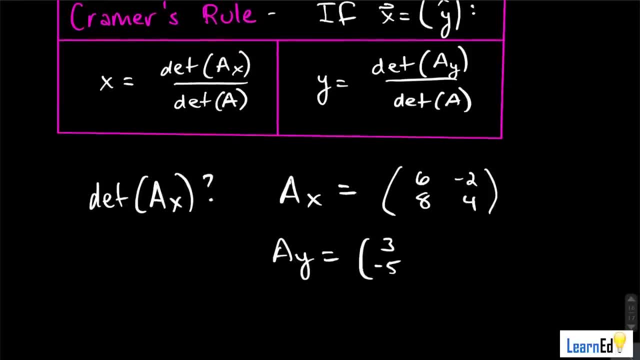 would get the a Y equals, not 68, we would would get the a Y equals, not 68. we would get 3 negative 5, which is our original X, get 3 negative 5, which is our original X, get 3 negative 5, which is our original X column. and then we put our solution or: 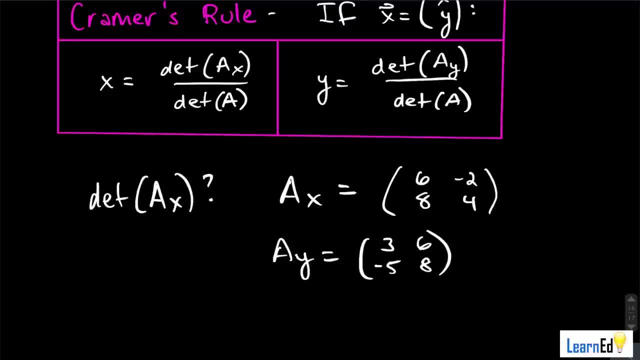 column and then we put our solution or column and then we put our solution or not our solution, our B vector in our Y, not our solution, our B vector in our Y, not our solution, our B vector in our Y column. so let's actually go through and 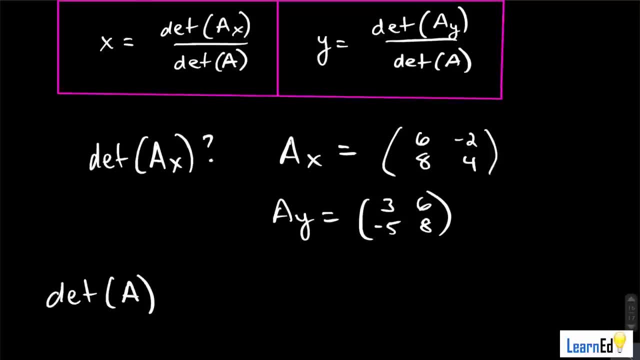 column. so let's actually go through and column. so let's actually go through and compute these determinants. so, first off, compute these determinants. so first off, compute these determinants. so first off, the determinant of a: well, remember that a the determinant of a: well, remember that a. 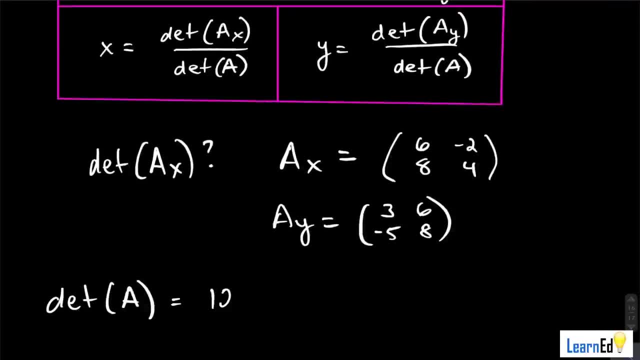 the determinant of a. well, remember that a is 3: 4, so we'll have 12, minus a is 3: 4, so we'll have 12, minus a is 3: 4, so we'll have 12, minus a negative 2 times negative, 5 is 10, so we. 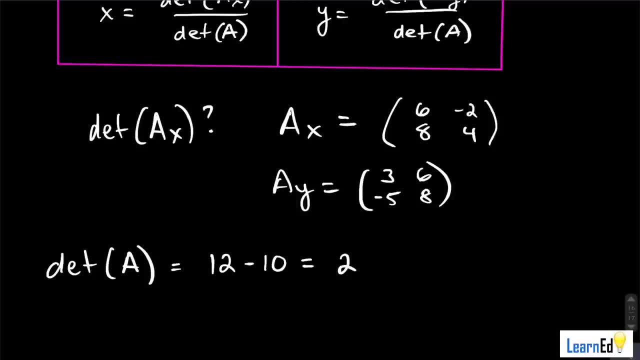 negative 2 times negative, 5 is 10. so we negative 2 times negative, 5 is 10. so we get minus 10, and then that is 2, so get minus 10, and then that is 2, so get minus 10, and then that is 2. so that's the determinant of a, the 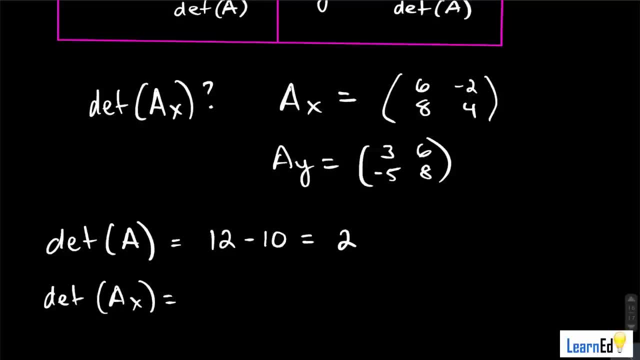 that's the determinant of a. the. that's the determinant of a. the determinant of ax will be: we have 6 times determinant of ax will be: we have 6 times determinant of ax will be: we have 6 times 4 is 24 minus a. 8 times negative. 2 is. 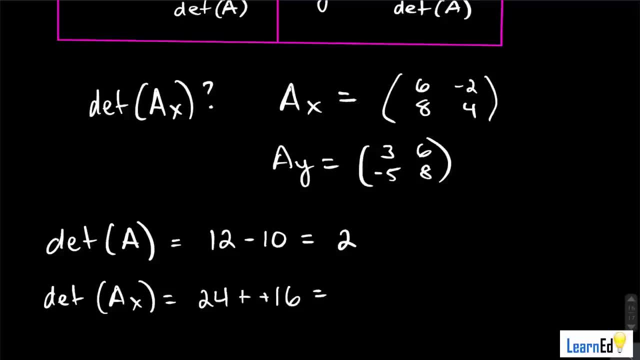 4 is 24 minus a 8 times negative 2 is 4 is 24 minus a 8 times negative. 2 is negative 16, and that will give us a 40 negative 16, and that will give us a 40 negative 16, and that will give us a 40. yeah, 40 okay, and then we have: 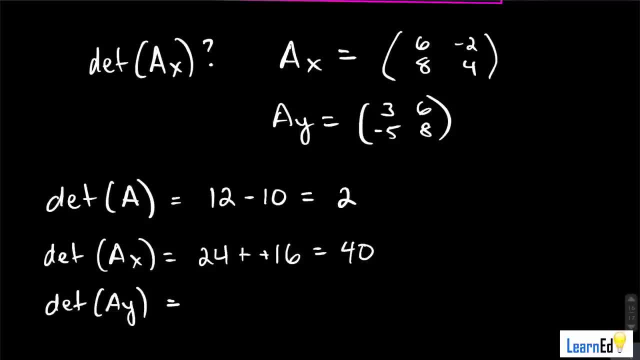 yeah, 40, okay. and then we have yeah, 40, okay. and then we have determinant of a Y which is going to be determinant of a Y, which is going to be determinant of a Y which is going to be 3 times 8, which is 24, okay. and then we 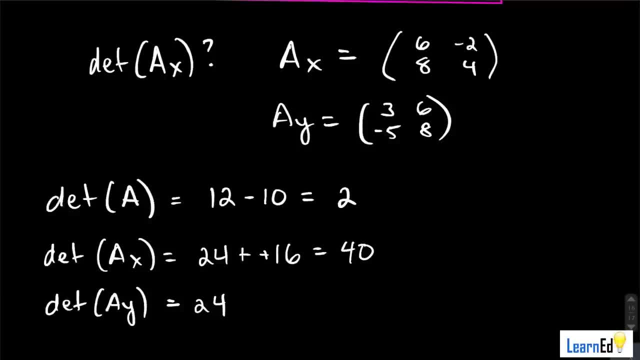 3 times 8, which is 24, okay. and then we 3 times 8, which is 24, okay. and then we have a negative 6- no, sorry, negative 5. have a negative 6. no sorry, negative 5. have a negative 6- no, sorry, negative 5 times 6, which is negative 30. so we get. 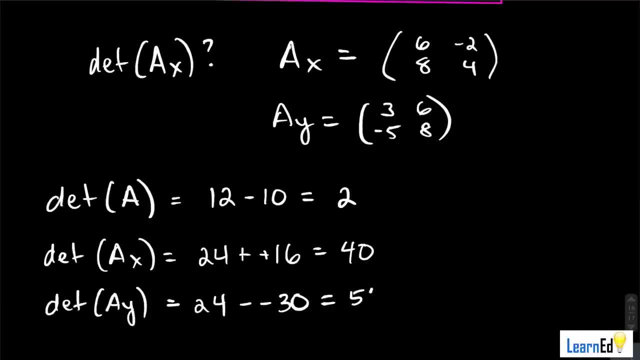 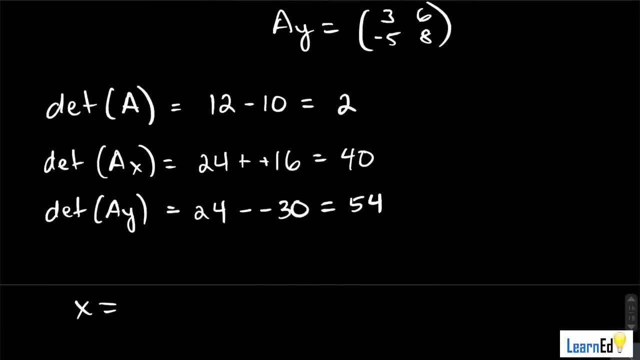 times 6, which is negative 30, so we get times 6, which is negative 30, so we get minus, minus, and then we have a 54- okay, minus, minus. and then we have a 54- okay, minus, minus, and then we have a 54- okay, so we just for 4x. that's determinant of. 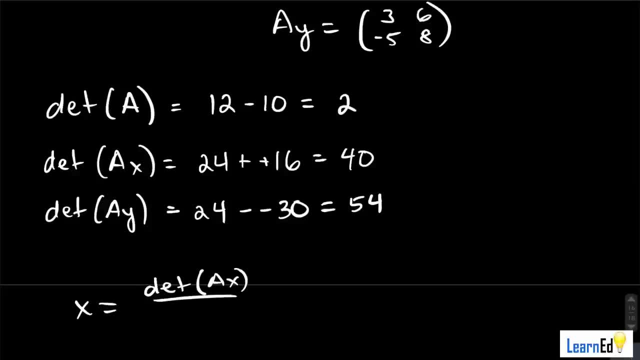 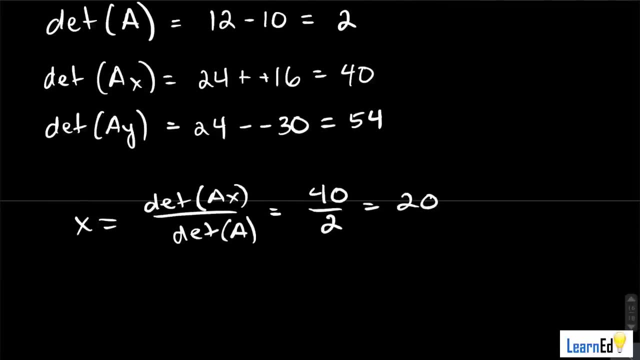 so we just for 4x, that's determinant of. so we just for 4x, that's determinant of a, X over the determinant of a. so we have a X over the determinant of a, so we have a X over the determinant of a. so we have 40 over 2, and that is 20, and then for Y: 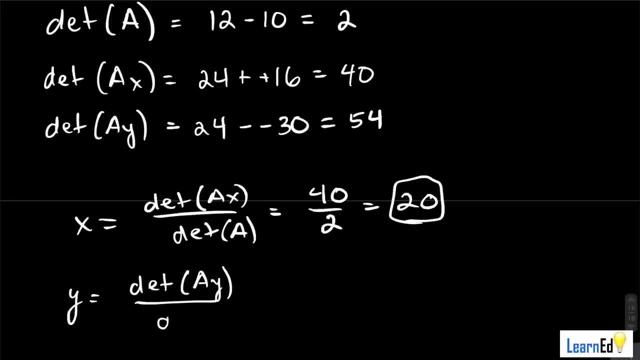 40 over 2, and that is 20. and then for Y, 40 over 2, and that is 20. and then, for Y, we have the determinant of a Y over the, we have the determinant of a Y over the, we have the determinant of a Y over the determinant of a which is equal to 54. 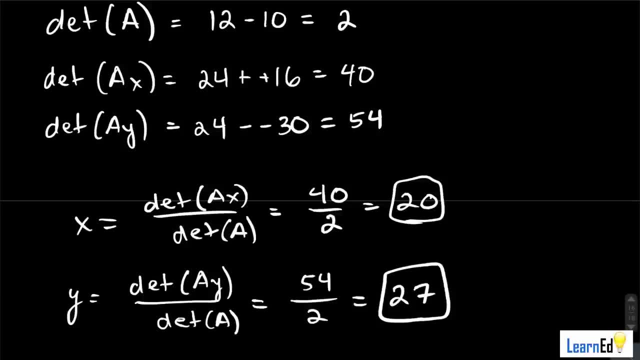 determinant of a which is equal to 54. determinant of a which is equal to 54, over 2, which is 27. okay, and so that is over 2, which is 27, okay, and so that is over 2, which is 27. okay, and so that is what our X vector is, so we can say that.